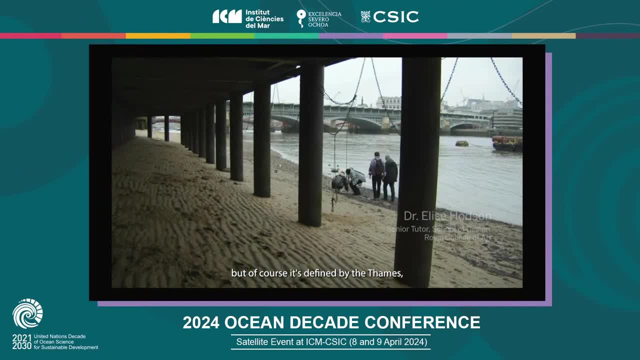 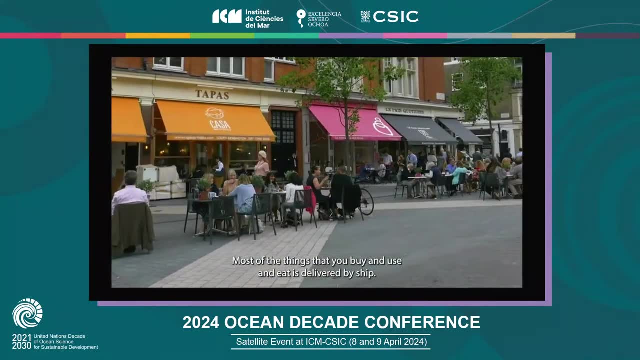 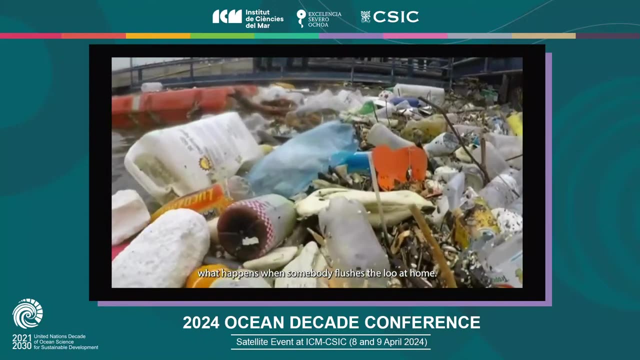 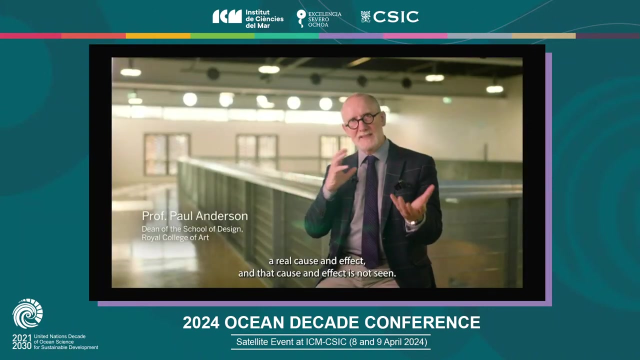 We're able to do this much for our students. We're able to do this much for our students. It's this landscape that we take for granted, but this is producing a real cause and effect, and that cause and effect is not seen. It's very easy to feel far removed from the ocean at times. 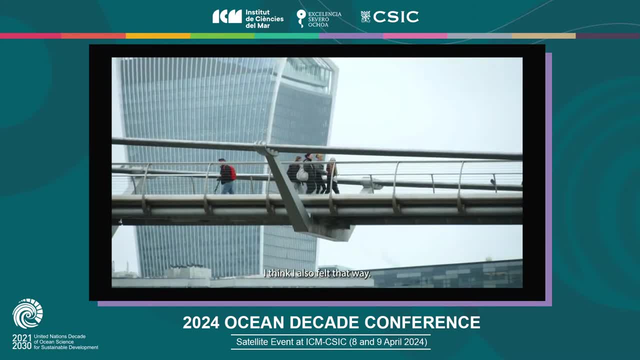 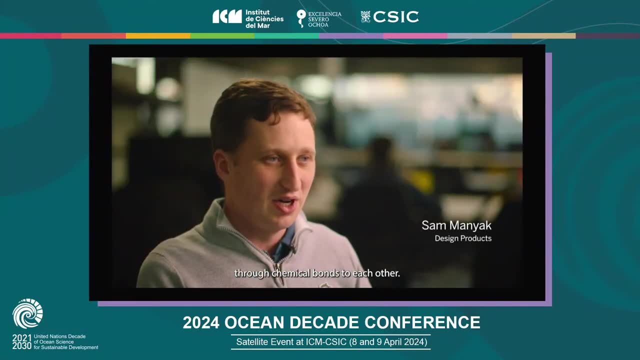 Like there's a sense of diminished responsibility. I think I also felt that way. Finding those connections is important. If you look at it chemically, every water molecule is connected through chemical bonds to each other, So you know everything from here to the ocean. 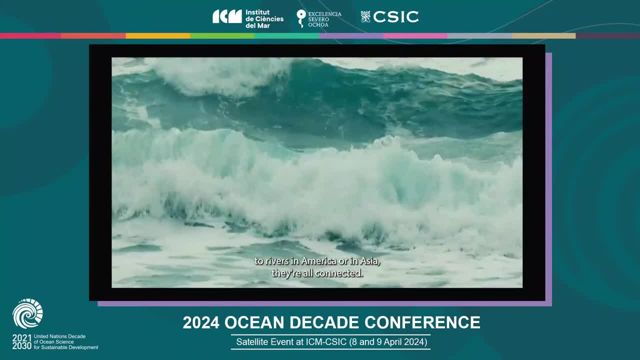 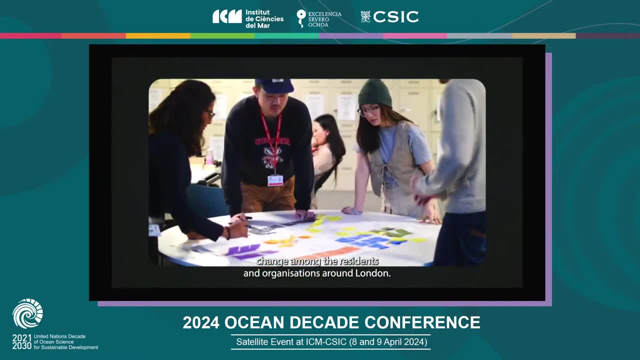 to rivers in America or in Asia. they're all connected. The goal of the Grand Challenge is to support action and behavior change among residents and organizations around London. We want to raise awareness, but more than that, make sure people feel empowered to do something. 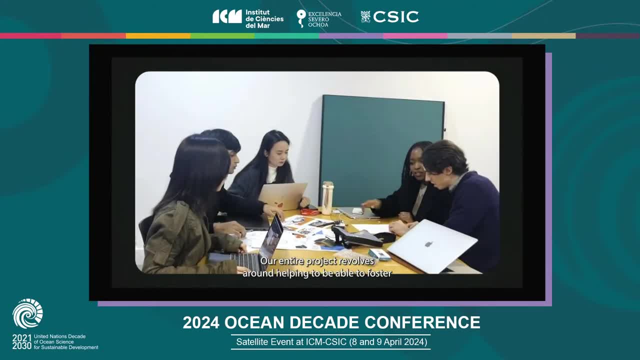 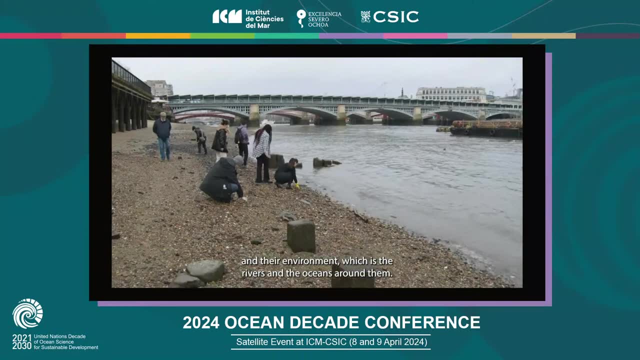 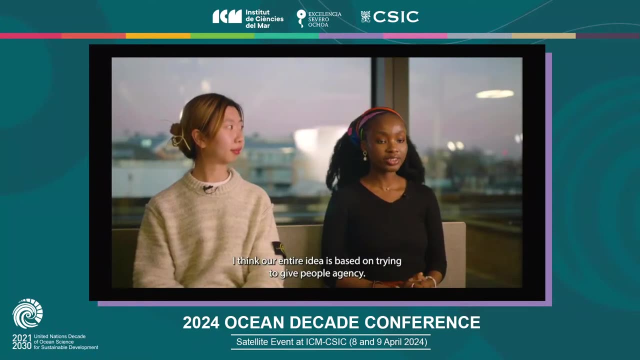 to protect their cities and the ocean. Our entire project revolved around helping able to like foster a more stronger relationship between the community and their environment, which is the river and the oceans around them. I think our entire idea is based on trying to give people agency. 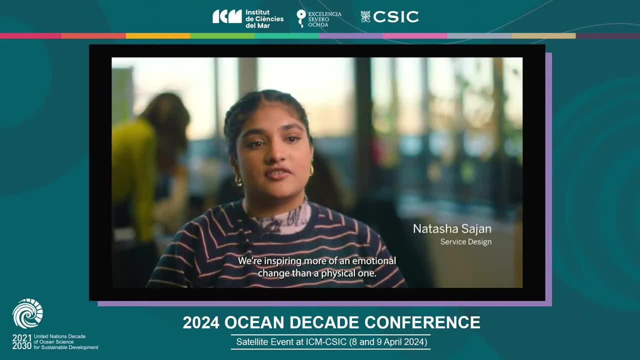 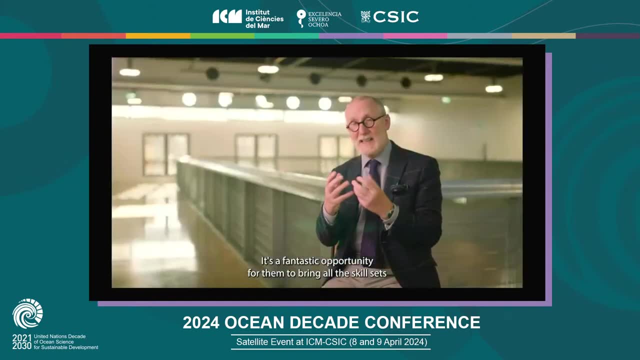 We're inspiring more of an emotional change than a physical one. Students are working with people they've never worked with before, with disciplines They've never worked with before. It's a fantastic opportunity for them to bring all the skill sets and work together. 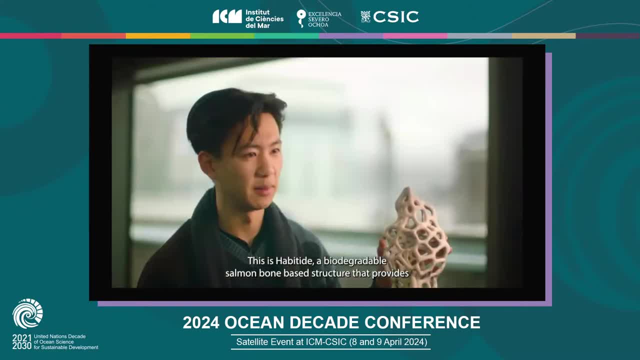 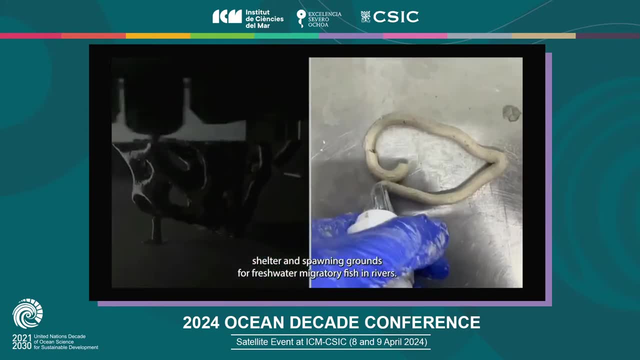 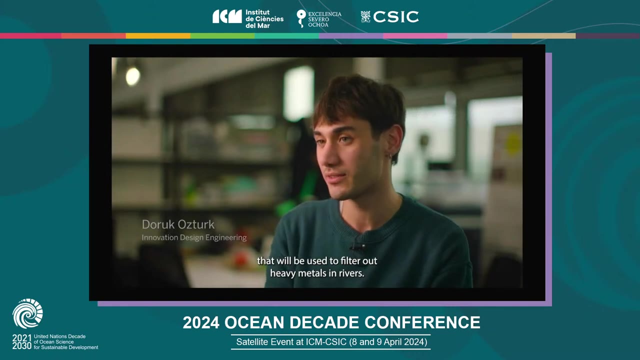 in solving the brief. This is Habitide, a biodegradable salmon bone-based structure that provides shelter and spawning grounds for freshwater migratory fish in rivers. We've collected pigeon poo and then converted into a material that will be used to filter out heavy metals in rivers. 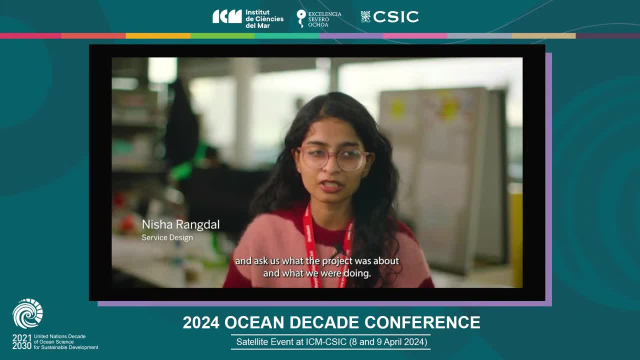 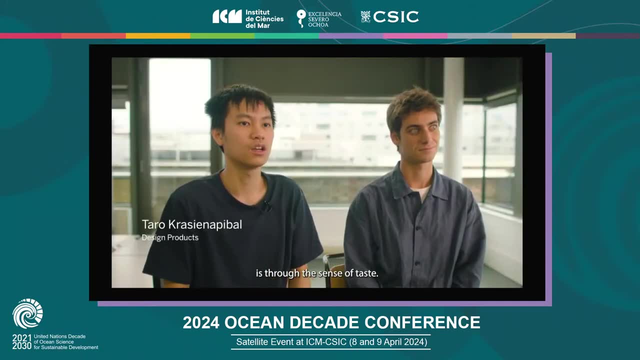 A lot of people did stop us and ask us what the project was about and what we were doing. We saw children running around the wetlands and we realized that one of the ways children explore is to the sense of taste. We were wondering: can we take that and apply it? 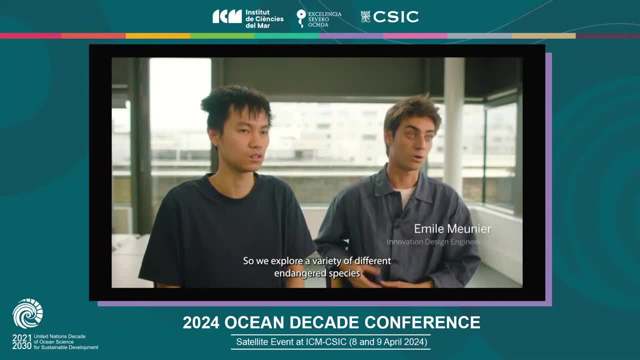 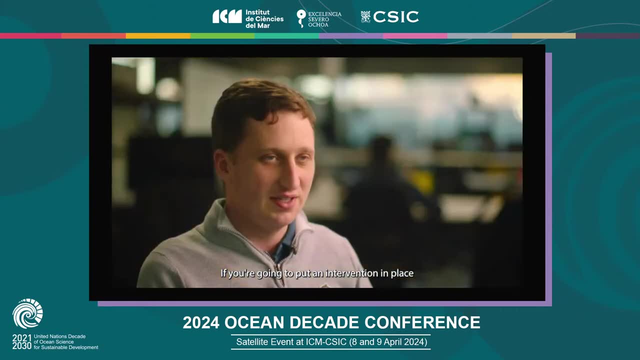 to other parts of the community, like adults as well. So we explore a variety of different endangered species through the box of chocolate. If you're going to put an intervention in place into any sort of ecosystem or interaction, it has to be simple, it has to be easy. 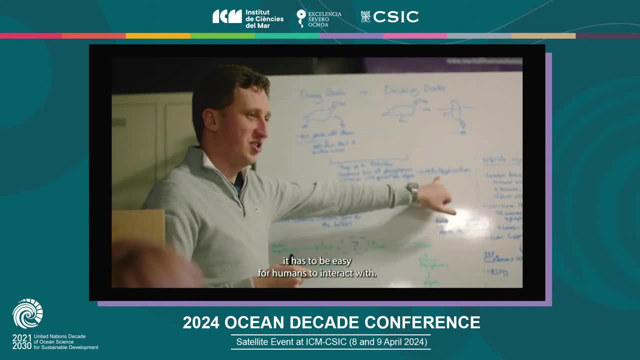 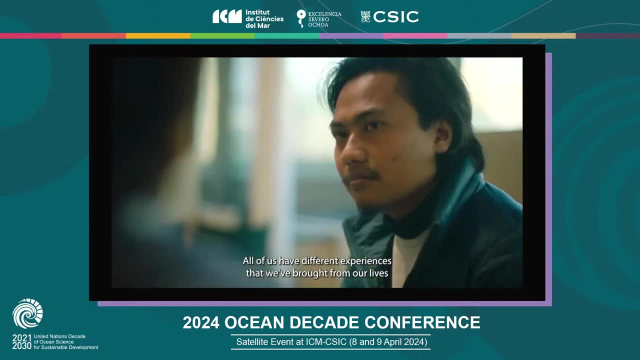 And especially within this theme, where it's human centered, it has to be easy for just children- humans- to interact with. so that was something that was important to all of us. All of us have different experiences that we've brought from our lives and being from different parts of the world. My background is in mechanical 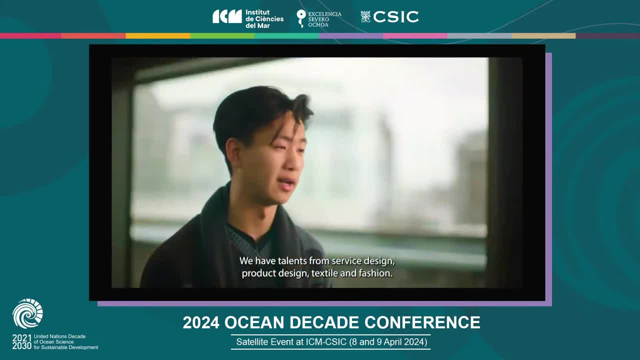 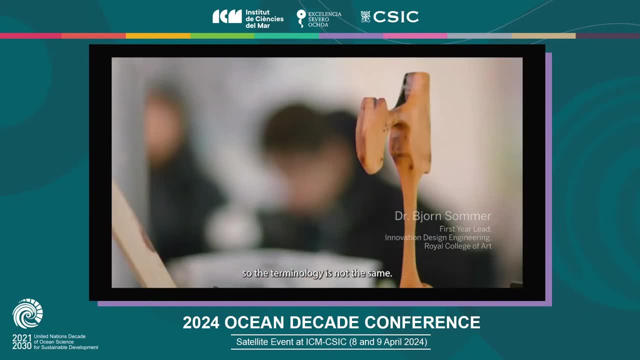 engineering. I'm especially interested in design research. We have talents from service design, product design, textile and fashion. You have a lot of different design languages, in a way, so the terminology is not the same. I think it is really important for each discipline to have a say, to have a voice in the 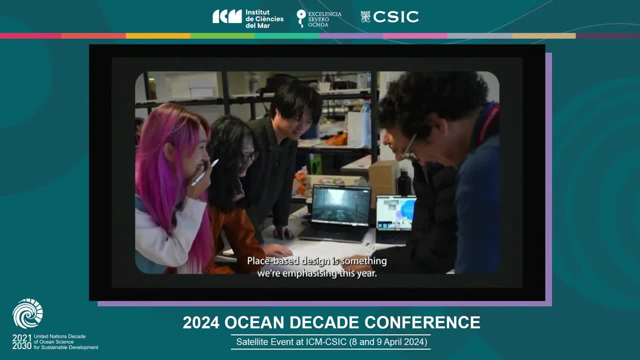 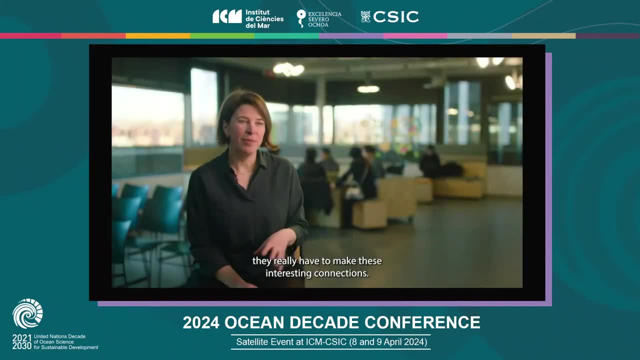 outcome. Place-based design is something we're emphasizing this year. Some of them are right on the Thames and for them it's maybe a bit more obvious, but for the students who are outside of that core, they really have to make these interesting connections. Do we focus at the street? Do we focus at a park? Do we? 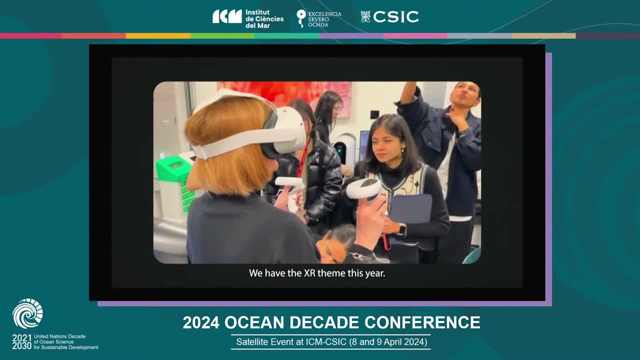 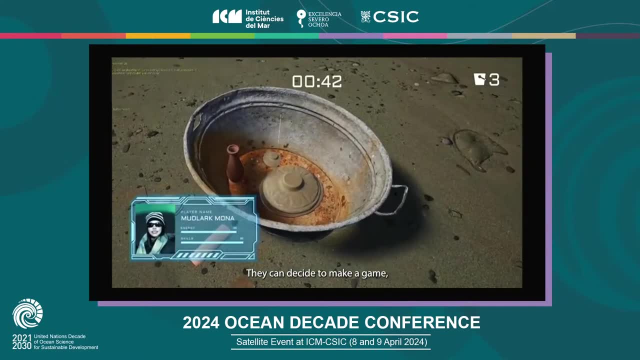 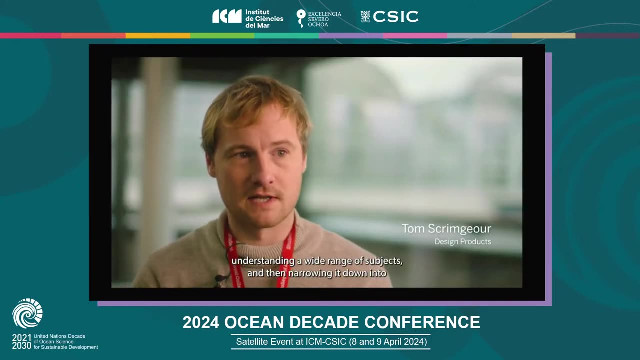 focus more on a global view. We have the XR theme this year. You can use virtual reality, augmented reality, mixed reality. They can decide to make a game which has, of course, educative components which are trying to raise awareness. It's a process of going incredibly broad, understanding a wide. 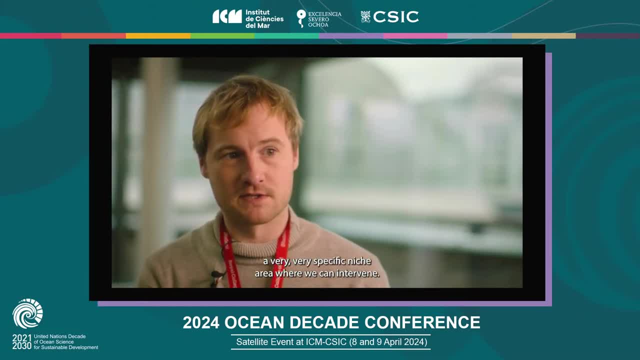 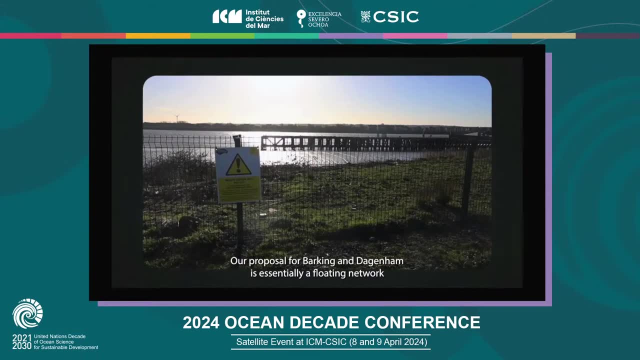 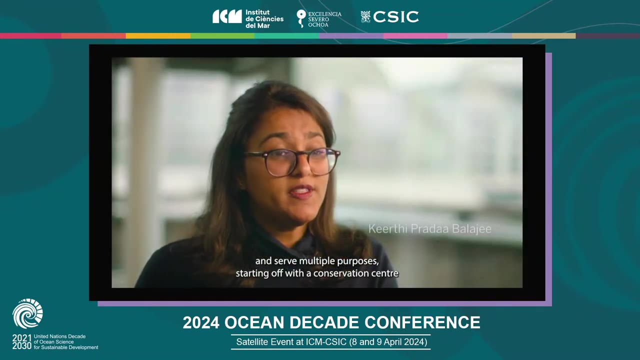 range of subjects and then narrowing it down into a very, very, very specific niche area where we can intervene. Our proposal for Barking and Dagenham is essentially a floating network of decommissioned, end-of-life river barges that are being upcycled and serve multiple purposes, starting off with a conservation center. 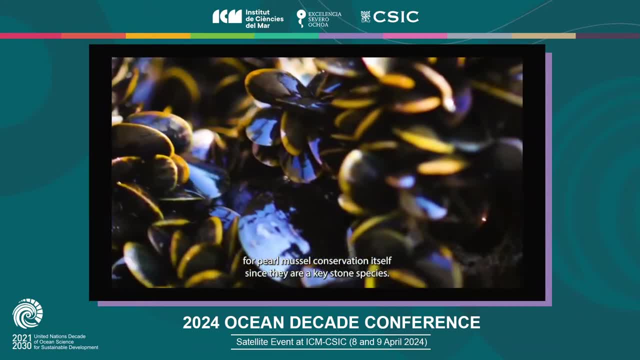 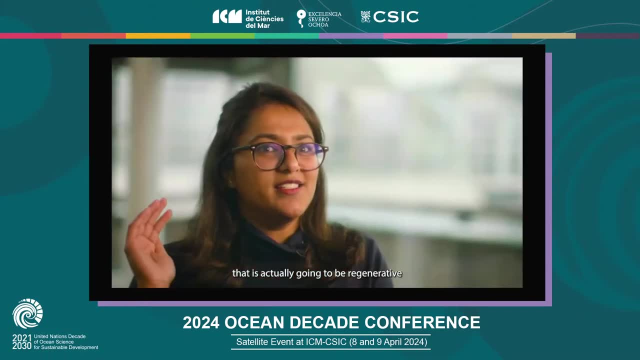 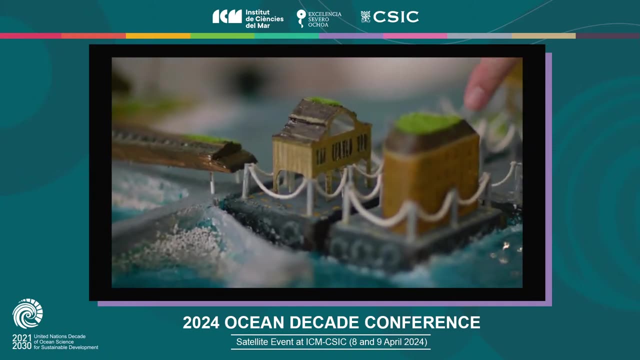 for pearl mussel conservation itself, since they are keystone species. We were really keeping in mind, like, how can we design something that is long-lasting, that is actually going to, you know, be regenerative in the way that it functions and not just self-sufficient? In terms of co-design, we have, first, 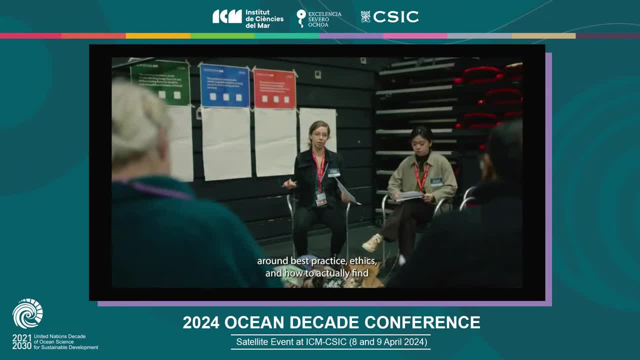 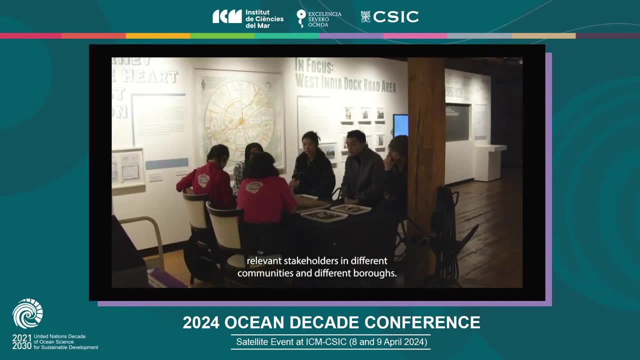 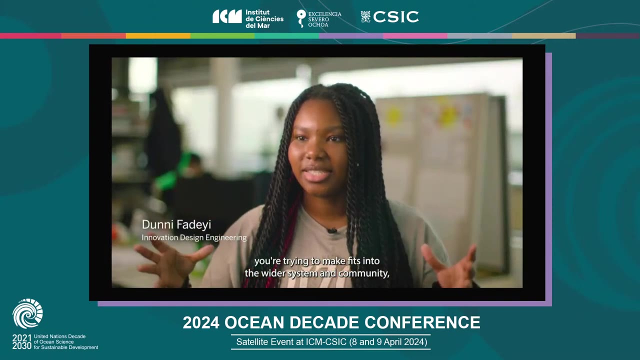 discussed with students some strategies for community engagement around best practices, ethics and how to actually find relevant stakeholders in different communities and different boroughs. You're kind of understanding the system you're trying to make fits into like the wider system and community. making sure that you know what we're creating isn't just about like what we think is cool, but 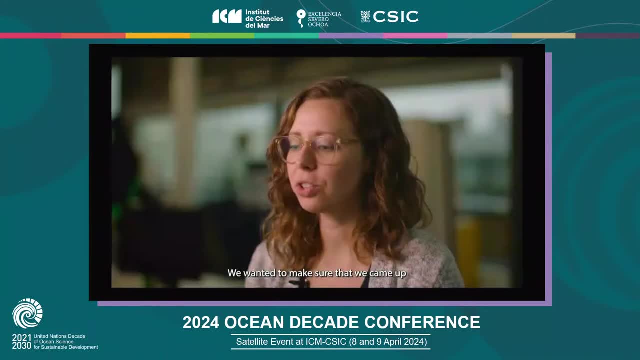 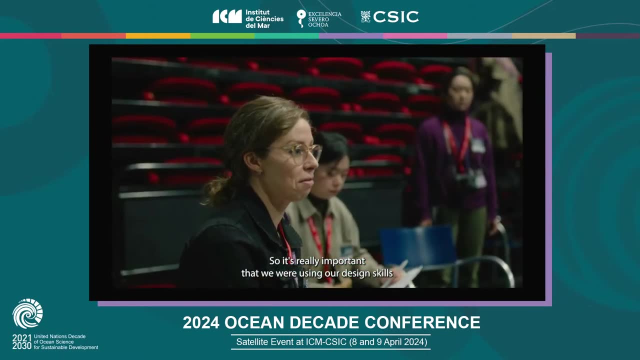 it's actually beneficial to the people we're trying to create. for We wanted to make sure that we came up with something that wasn't forced on the communities of Enfield, so it was really important that we were using our design skills to bring forth their voices and what they wanted, but we wanted to make it, so it was a 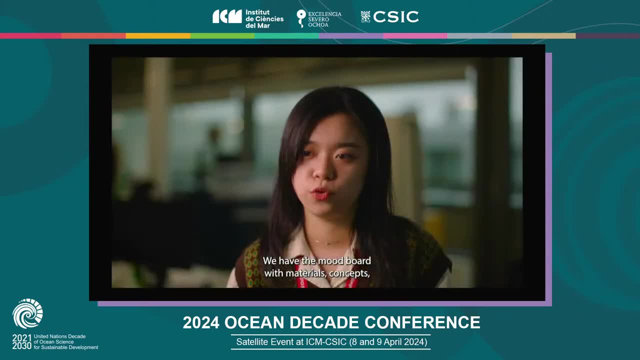 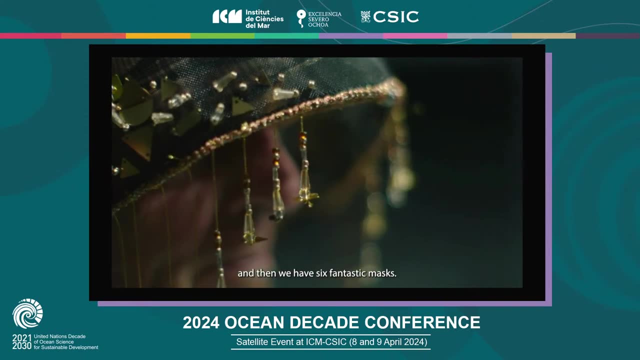 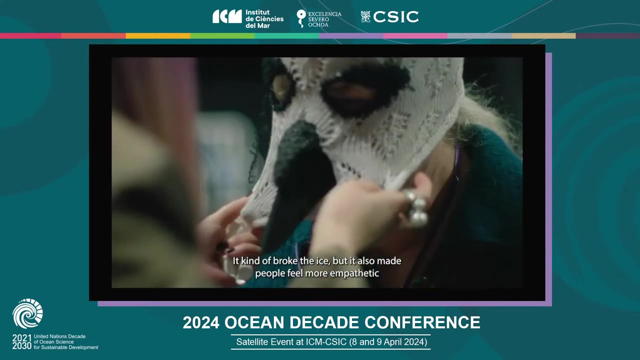 little silly. so we introduced this idea of masks. We have the mood board with materials, concepts, and then we have six fantastic masks. The idea of bringing masks was twofold. you know, it kind of broke the ice, but it also made people feel more empathetic to different parts of their borough. so, thinking about how, 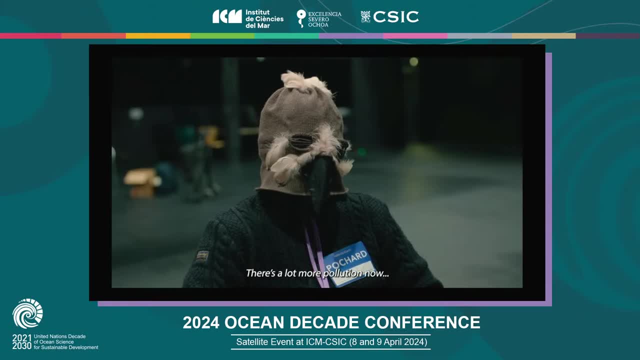 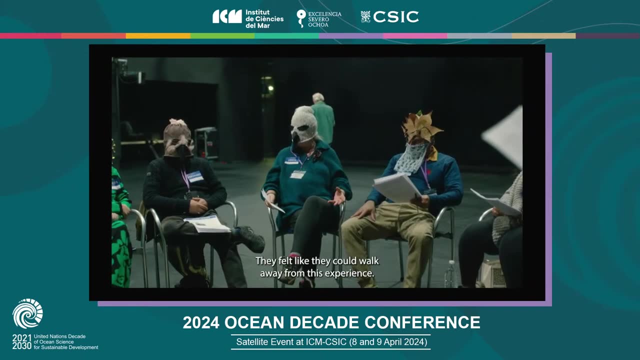 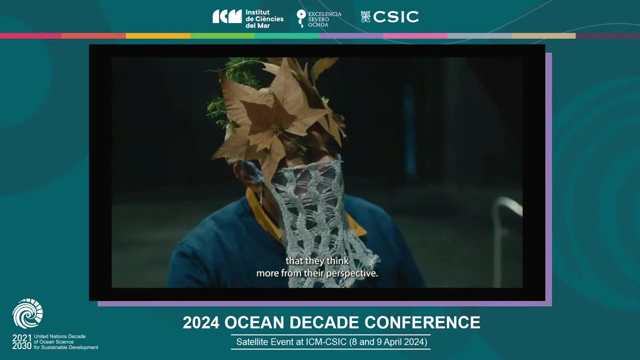 do the birds feel? how do the rivers feel? There's a lot more pollution now, so we fly a long way and we fish out the fish. They felt like they could walk away from this experience, and when they encounter a duck, a river or whatever, it is that they think more from their. 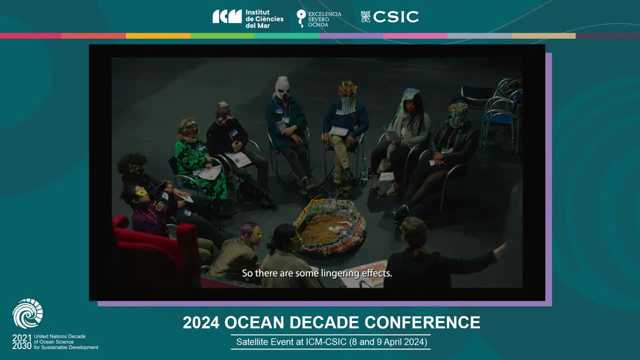 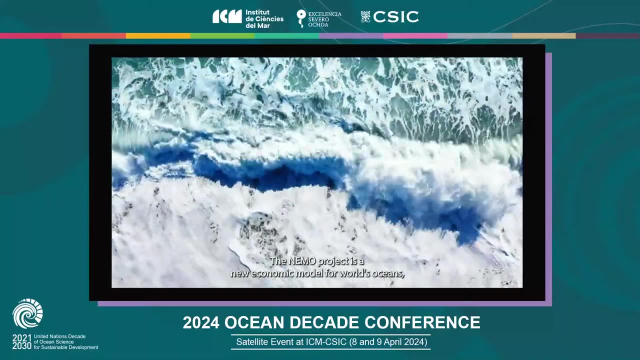 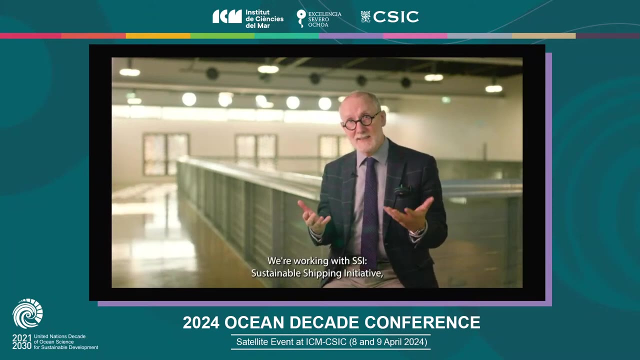 perspective, so there are some lingering effects. The NEEMO project is a new economic model for World's Oceans and we're working with partners like the National Oceanographic Centre in Southampton. we're working with SSI- Sustainable Shipping Initiative and, as a decade implementing partner with UNESCO, we're 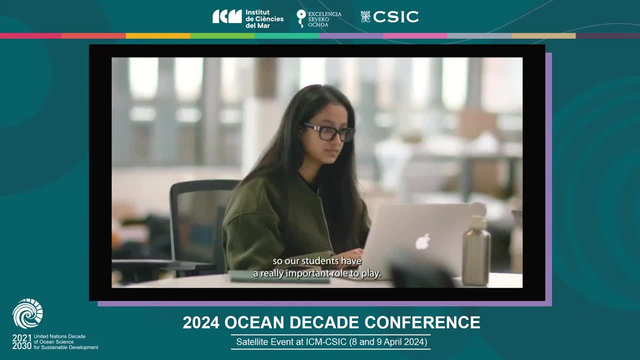 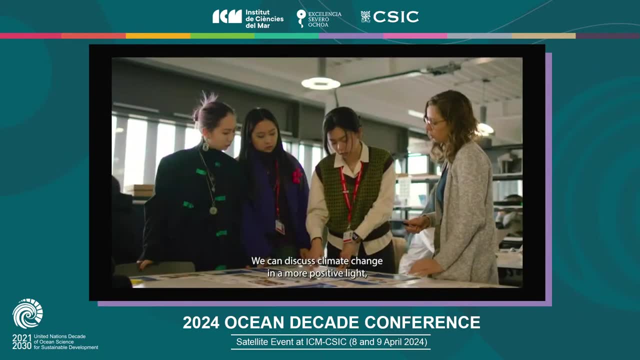 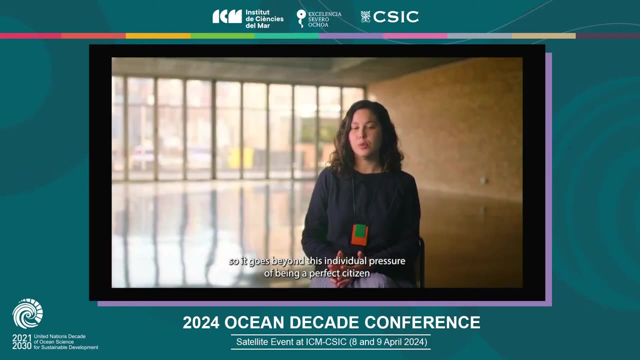 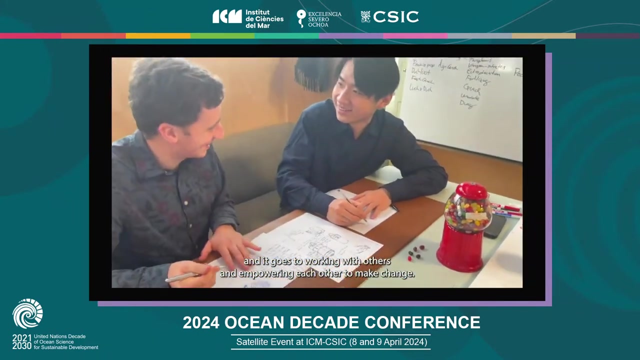 working with them and other partners around the world. so our students have a really important rule to play: We can discuss climate change in a more positive light. so it goes beyond this individual pressure of being a perfect citizen and it goes to working with others and empowering each other to make. 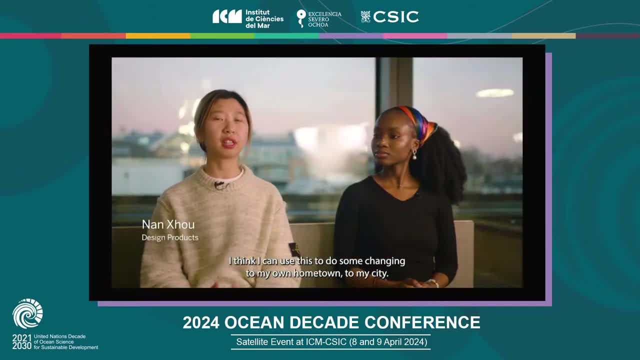 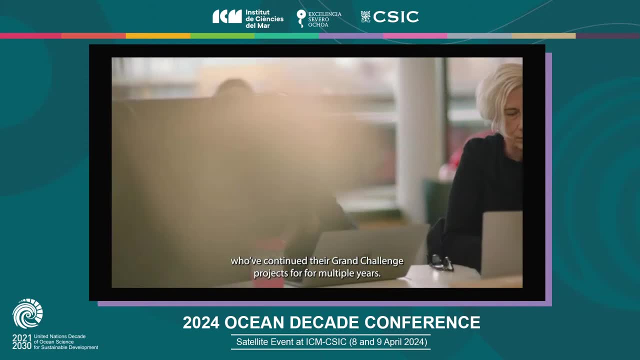 change. I'm thinking I can use this to do some changing to my own hometown, my own city. Just truly great learning experience. all in all, We have seen students who've continued their Grand Challenge projects for for multiple years. They are thinking, their creativity and their 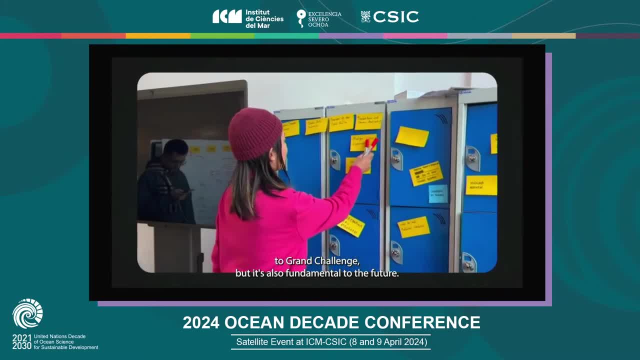 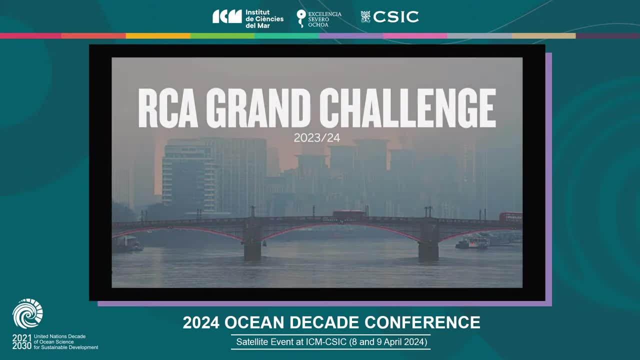 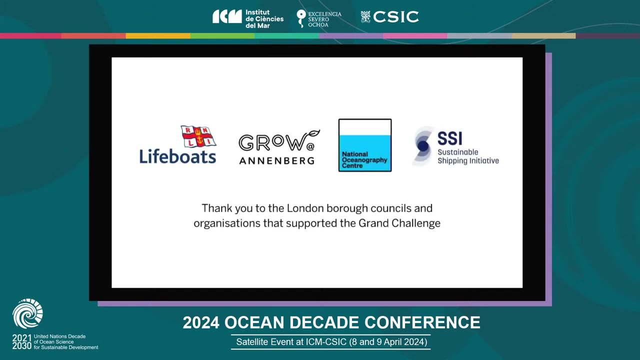 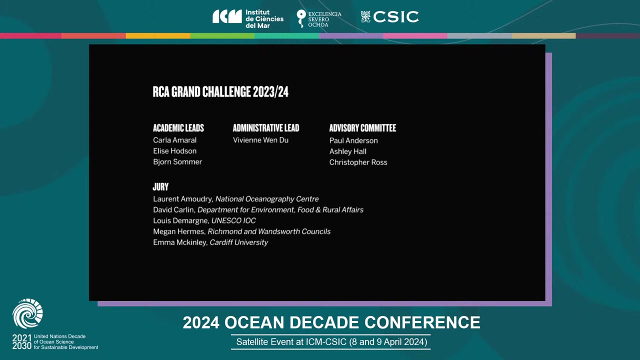 innovation is fundamental to Grand Challenge, but it's also fundamental to the future. It's possible to change. We see it's natural in our world, but also possible in others. We feel like people in Government can change. We are educated to really think. dashboard style. 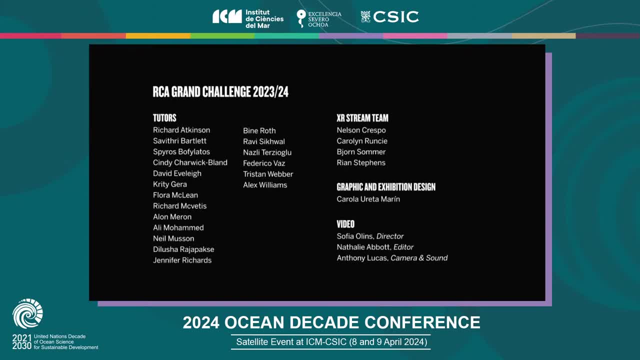 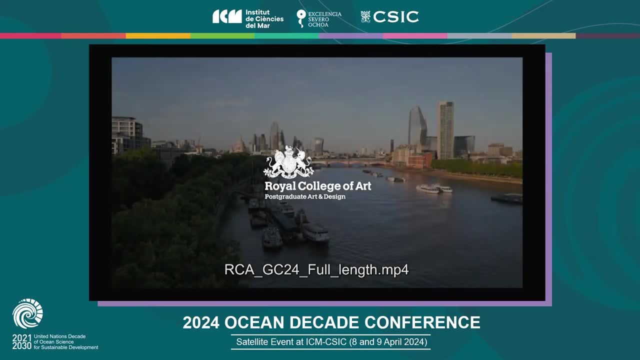 I grew up thinking that everyone lived in a vehicle. I knew that I was able to do really phenomenal things in my life. I grew up expecting that people like like me will change when they turn on the light. The entire journey has been quite interesting because we didn't get into it. 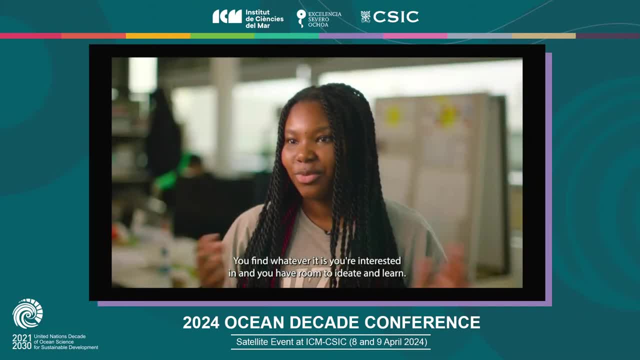 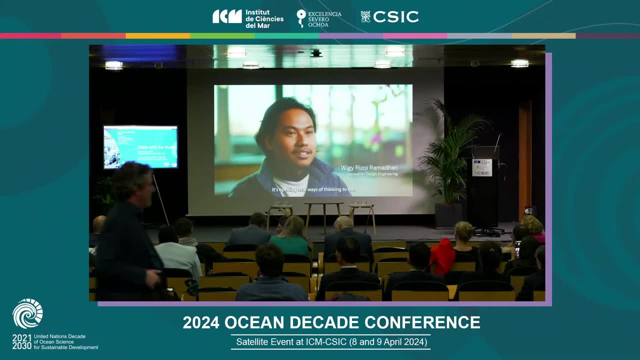 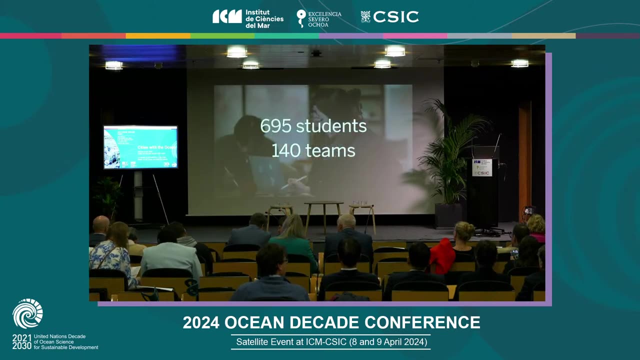 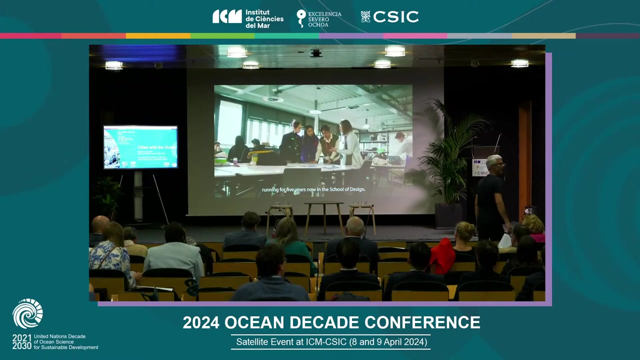 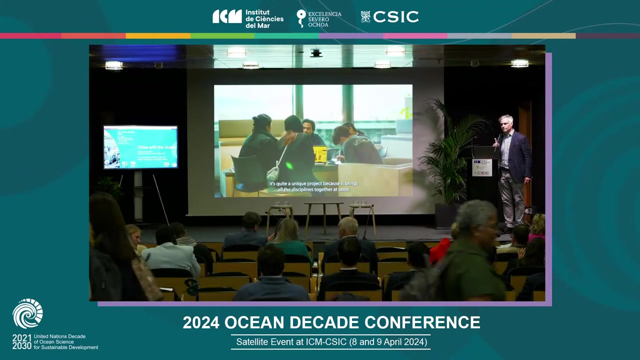 with any sort of preconceived notions. It's almost like a playground in a way. you find whatever it is you're interested in and you: Hello, good afternoon. We're going to get started very shortly, but I just wanted to make a message, send out a message. 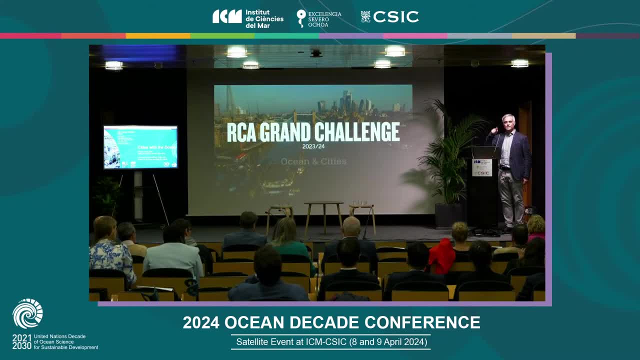 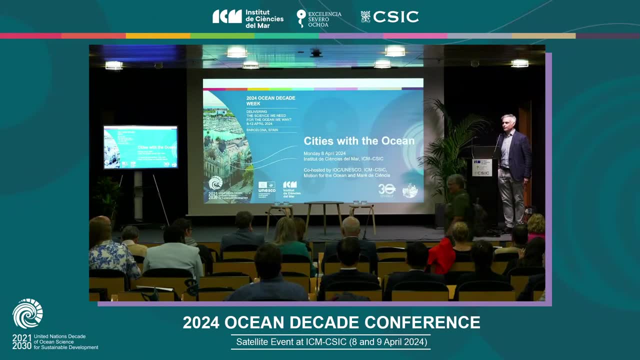 If you are speaking at this event, could you please come forward and sit your? You have names on the seats there for you. Please come forward and sit down at the front so we can make it a little bit easier when we're doing the panel discussion. 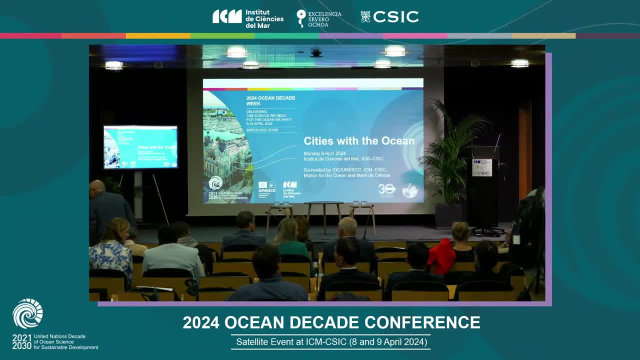 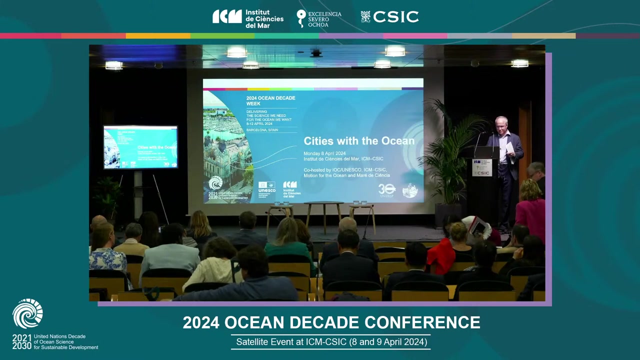 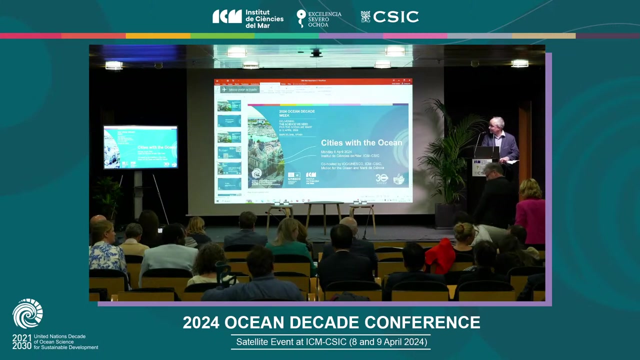 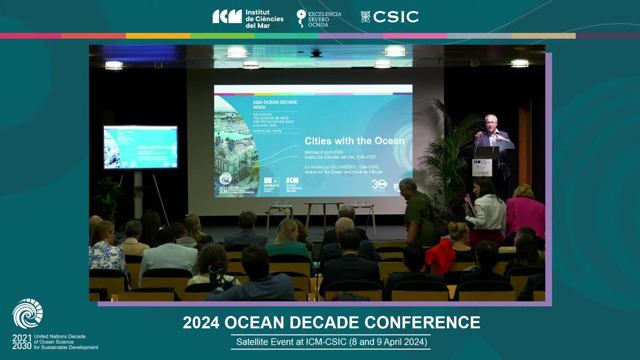 Thank you. Thank you Good afternoon, ladies and gentlemen. Thanks a lot for attending the Cities with the Ocean satellite event today. This event will take us deep into the connections between ocean, ocean science, coastal cities and ports, And we will reflect on how to strengthen this connection. 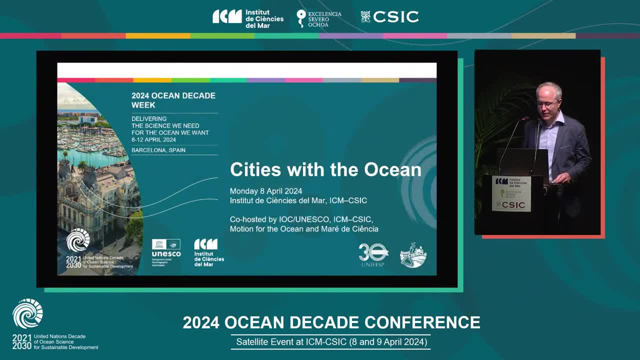 and build a more inclusive, more sustainable world on the ocean decade, to increase the way the ocean can contribute to the sustainable development of coastal territories. So, without further ado, it is my pleasure today to leave the floor to Mr Vidar Helgesen. 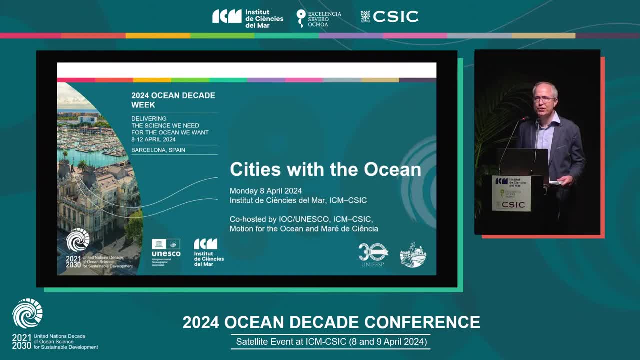 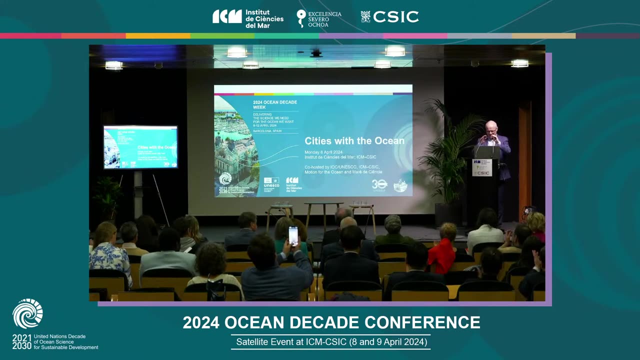 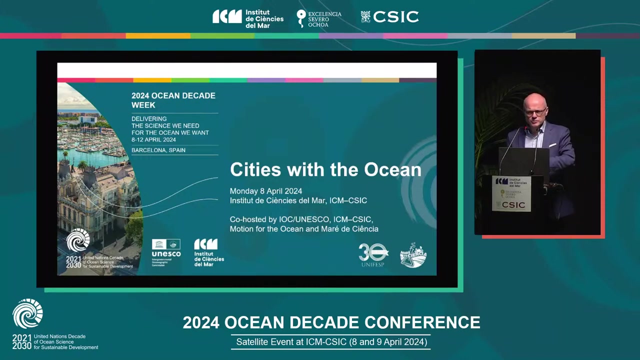 the Executive Secretary of the Intergovernmental Traffic Commission of UNESCO to deliver the introduction to this event. Mr Helgesen, please Thank you, dear city leaders, ocean leaders, city dwellers, ocean dwellers. It's such a delight that we 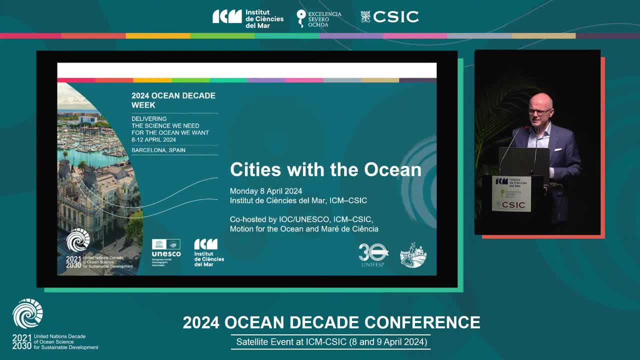 Thank. you have now kicked off the Ocean Decade Week in Barcelona, after my team has, with partners in Barcelona and around the world, spent enormous effort putting this all together, And it's also exciting to start with cities and cities' relationship to the ocean. 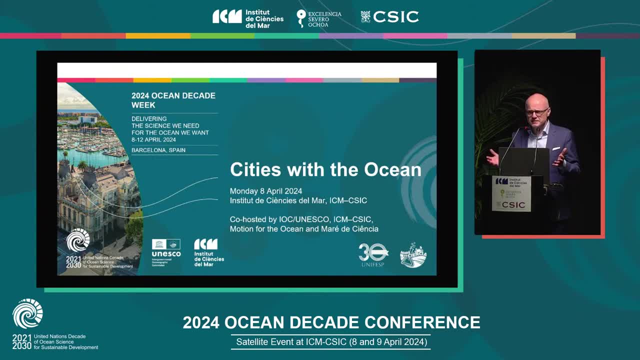 Cities are attractive. We're in a very attractive city, the second biggest cruise port city in the world, Barcelona, And that attraction of cities, that dynamism of cities is what makes them grow, And the hope and aspiration that comes with cities. 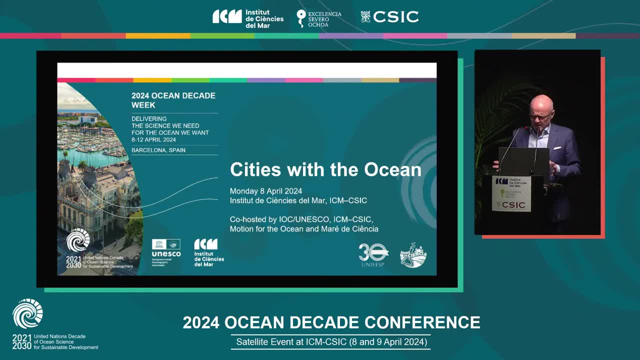 is also what makes them grow. About 37% of the global population live within 100 kilometers of the ocean, with twice the population of the world- The density of the global average. So there is much pressure on the coastal areas and not least on cities. 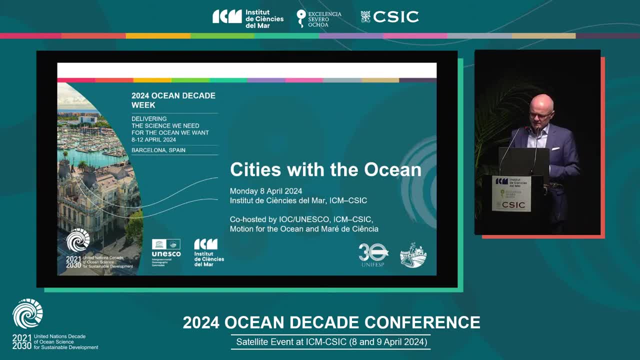 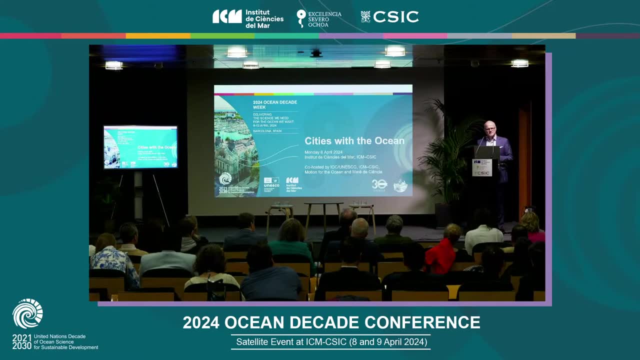 15 of the 23 megacities globally are in low-lying coastal areas And these bustling, attractive places are at risk. And they're at risk partly because the ocean is at risk, Sea level rise, Storms are at risk. 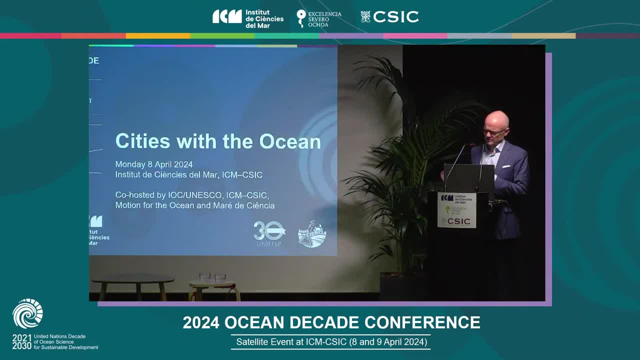 The ocean is at risk: Storms and floods prompted or at least reinforced and strengthened by warmer oceans, Coastal erosions, tsunami, a lot of other hazards that put these enormous population centers at risk. And not only the enormous population centers: There are many smaller and medium-sized and big cities. 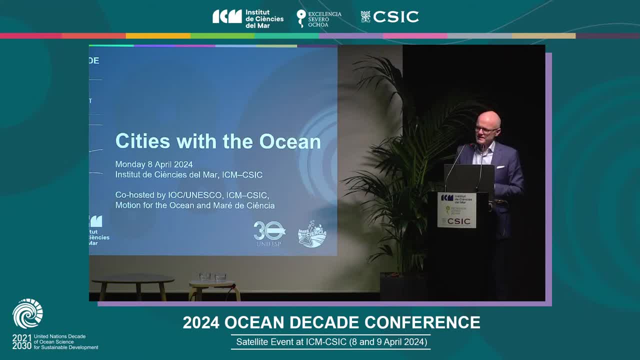 that aren't megacities along coasts. globally And, as it happens, because of the global warming, because these oceans are symbols of hope for many people, cities have often a fairly high proportion of poor people. that are those that are the most at risk. 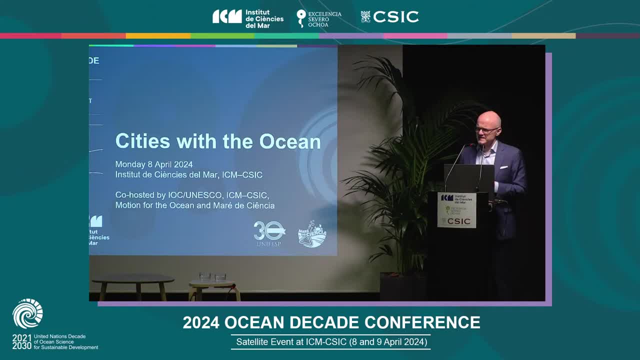 As many of us know, the ocean has a lot of capacity to mitigate problems, mitigate disasters, But many of the mitigating factors that the ocean ecosystems provide have been destroyed In the development of these coastal areas and population centers. So we're at a stage where new thinking is necessary. 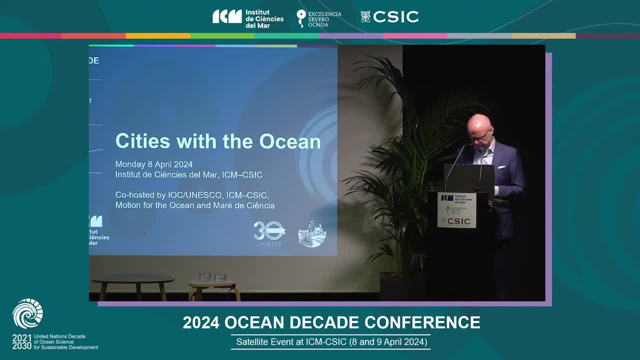 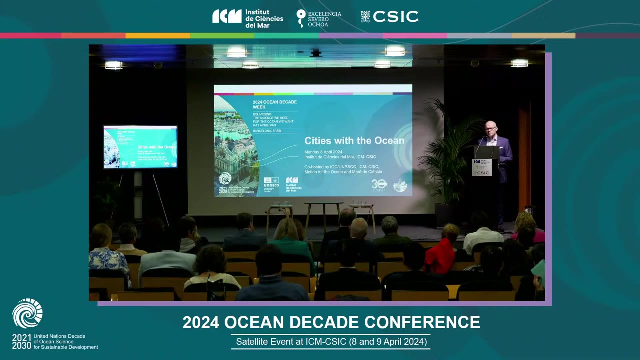 when it comes to the relationship between cities and the ocean, And there's hope in the fact that cities are actually hubs of dynamism and innovation. It's a place of a lot of innovative spirit and places where we can work together to find the solutions. we need to adapt and build resilience. 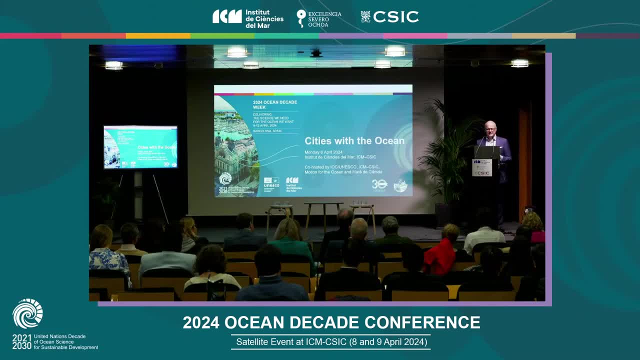 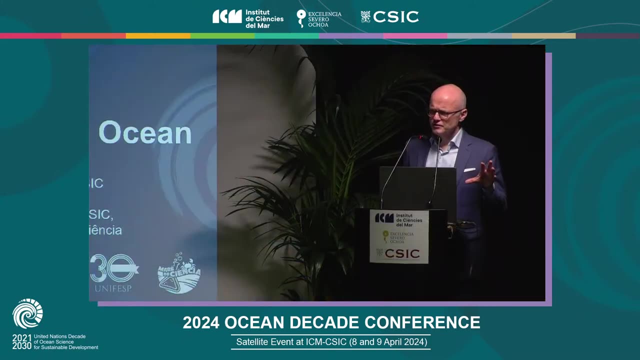 So what we need is knowledge and engagement. There's actually been some research done into cities and floods, And one of the observations made in that research is that there's a need for more knowledge of how you can build resilience, For example, through infrastructure, how you can make better use. 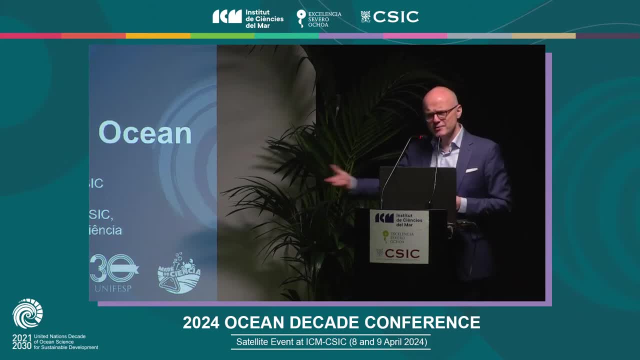 of green and blue infrastructure and not only the engineering gray infrastructure, and that often that knowledge is lacking locally. And another key conclusion from that research is that you need engagement, You need industry, decision makers, communities to work together. You need to tap into the wisdom of those who live and have lived in cities. 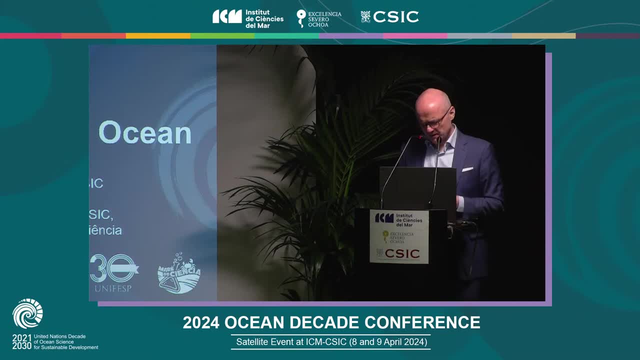 for a long time to make the right decisions. So knowledge and engagement: That's actually also what the ocean decade is about. It's about generation. It's about generating knowledge, but not only to generate knowledge for its own sake, but for the ocean we want and the sustainable development that the planet needs. 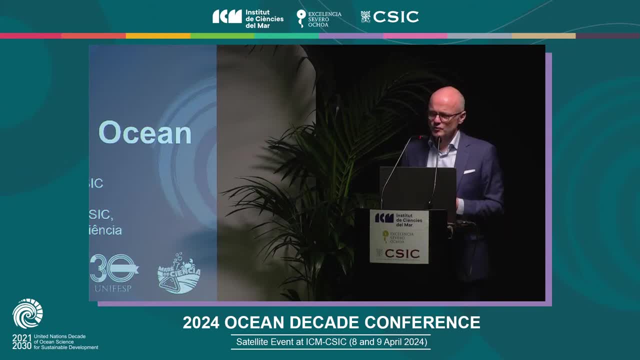 So cities with the ocean, the ocean cities, have a critical role to play in contributing to that knowledge and that engagement that we want with the ocean decade. And we've seen that in the preparations of this decade, ocean decade program, A platform has been developed. 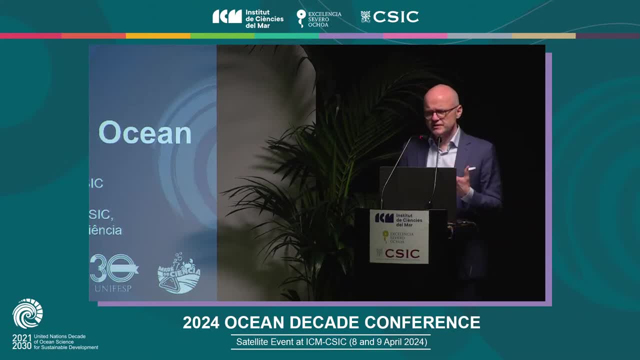 A call to action has been developed. A shared vision has been developed on how cities can continue benefiting from oceans and contribute to restoring oceans in order to benefit even more going forward. I'd like to thank the working group and the scoping group that has been working to prepare the agenda for cities with the ocean. 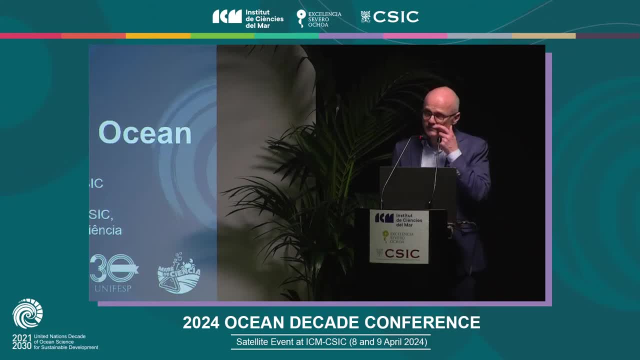 not leaving the ocean behind, And I'd like to thank all the partners that have been involved in this work. We've released Basil Angaga from Mombasa and Marco Talone from Barcelona, who have been the co-chairs of this work. 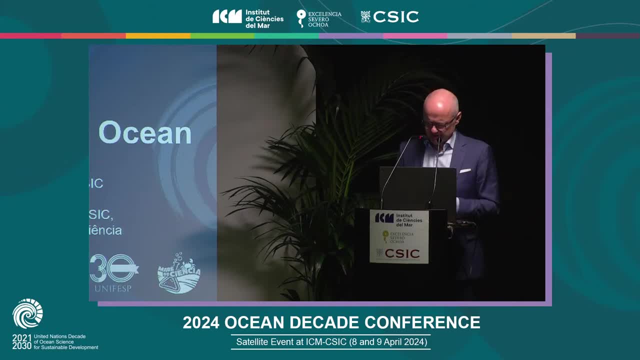 They have demonstrated through this process that we can create engagement, We can bring people together and tap into all those experiences that cities and ports and city activity entail, And that engagement, those partnerships, is what we need going forward as well. Thank you, 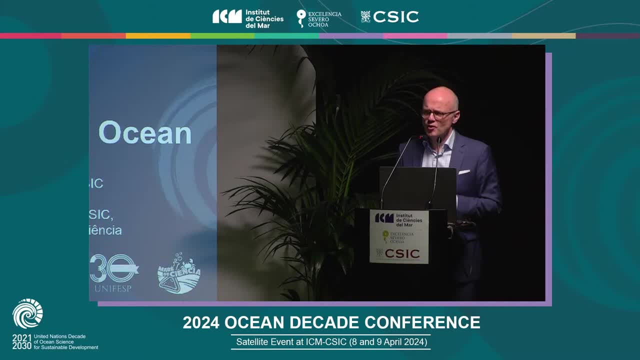 And this is therefore a start of a process that will hopefully bring more cities on board, more ocean scientists on board, in that critical partnership and engagement. Let me thank our partners in organizing this event as well: Our host institution, Institut de Ciências del Mar, Motion for Ocean and the Brazilian Ocean Literacy Commission. 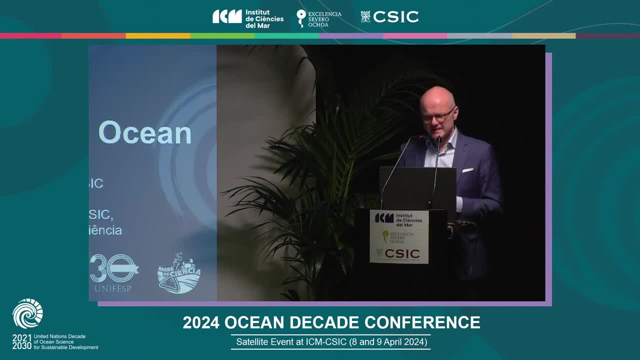 Thank you. Thank you And I'd like to thank all the partners in the Alliance that have been critical partners in this event. I wish you an event and a process going forward with this decade program of knowledge and engagement and a lot of learning over the next couple of hours. 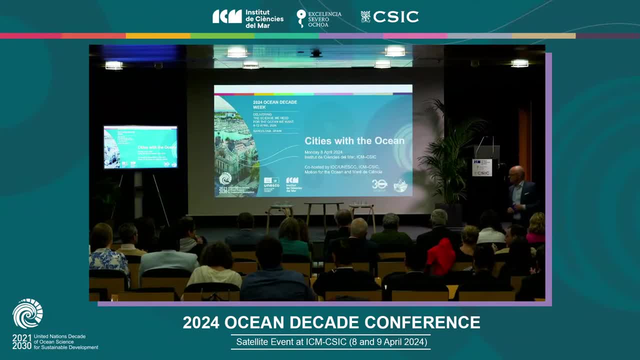 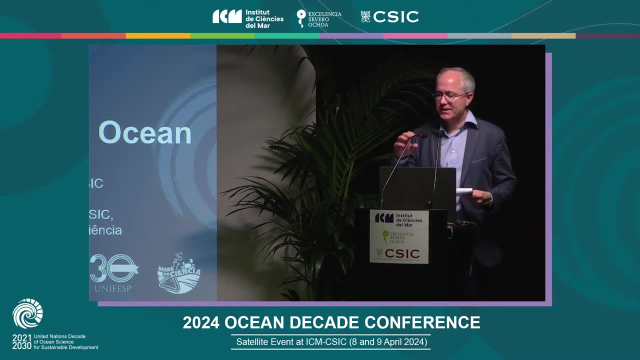 Thank you very much. Thank you very much. Thanks a lot, Mr Helgesen, for this very inspiring opening, And it is now time to set sail and go around the world to explore the existing connections of ocean science and cities. And to start this, it is my pleasure to welcome Mrs Marta Pontes from the city of Matosinos in Portugal. 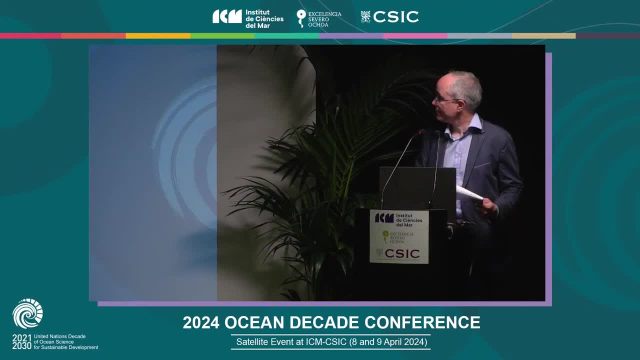 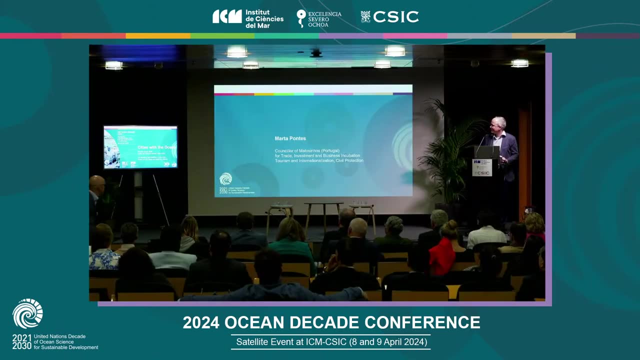 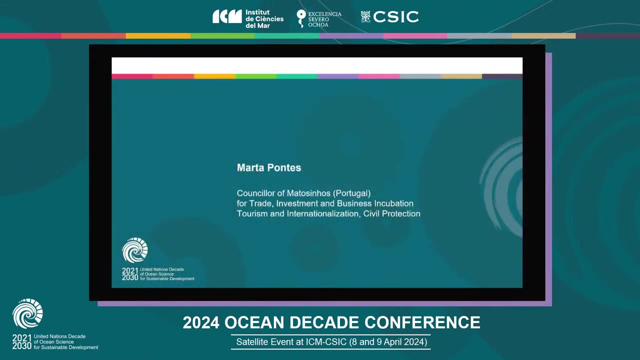 As the counselor for trade, investment and business, tourism and also civil protection, Marta Pontes is well aware of all the opportunities and threats of the ocean for her city. Thank you very much. Thank you very much, Thank you. 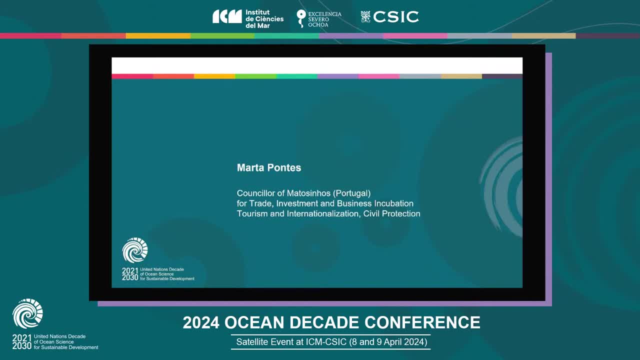 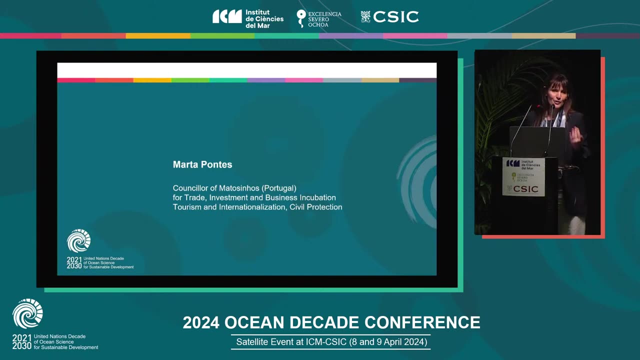 First of all, we would like to say thank you for the invitation, not only to be present at this event, but for all the work that we have been doing in this scoping group, which has been very important. I thank Oliver, because Olivier is the soul of the work and we have been working, sharing and learning, which, in fact, 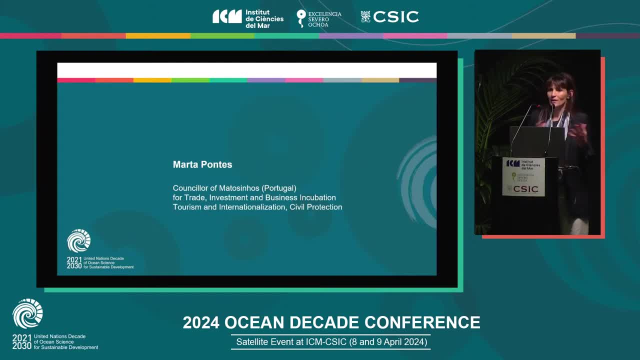 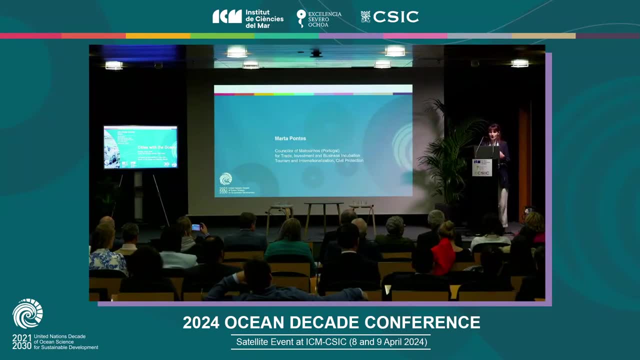 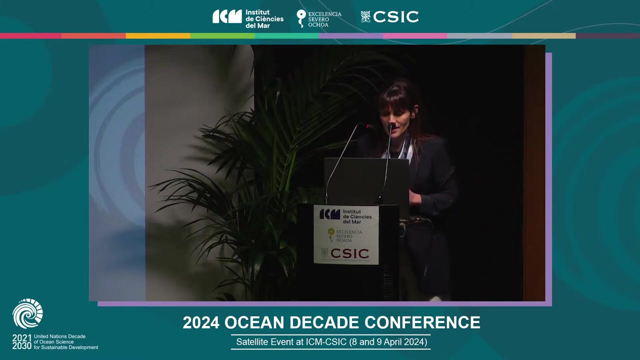 is the reason why I think we are all here, being technical or political sharing nowadays what we have been doing and inspiring each other is the main goal for us to be here. Matosinos is in Portugal. It is a city with 15 kilometers of coastline, of which 90% is covered by beaches and the rest occupied by the second. largest shipping port of Portugal, which integrates cargo transportation, fishing port cruises and also a marina. It is a city with an economic and cultural history connected since the early times to the sea Through its fishing history, fresh fish markets, canary industry, port activity, tourism and tourism. it is a city that has been connected since the early times to the sea through its fishing history, fresh fish markets, canary industry, port activity, tourism and tourism. 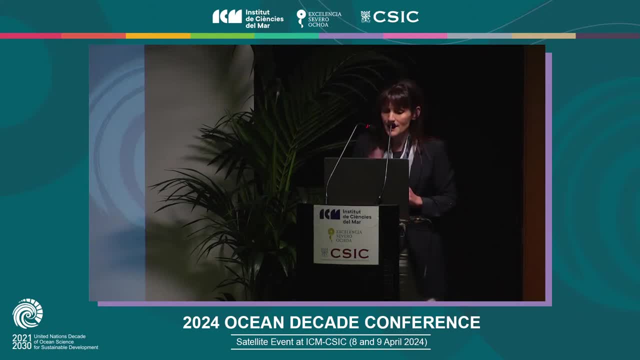 And that nowadays affirms itself as one of the most broader and complete references on the blue economy. in Portugal, and I believe, not only in Portugal, Climate change leads the city to understand the necessity of comprehending the coastline evolution. To achieve that, we did cartographic research. 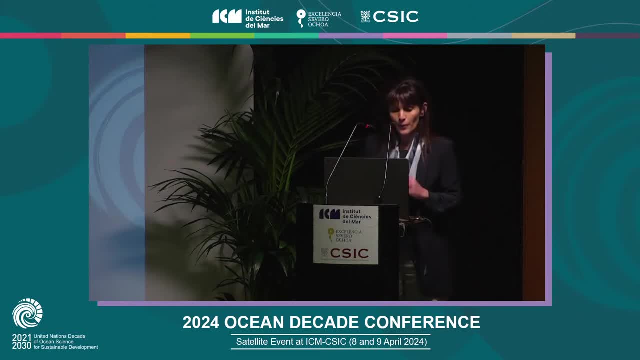 Since then we have been working on a map of the coastline. Since then we have been working on a map of the coastline. Since then we have been working on a map of the coastline. It was around the year 1944, comparing it every 10 years to this year, with the fact that we are still doing it, 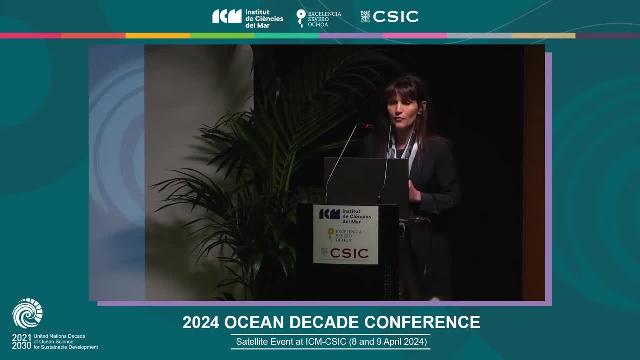 Through such research and with the help of the Municipal Geographic Information System, we were able to image coastal gains or losses and therefore define the zones of vulnerability and non-climatic areas in the coast and Arctic zone or risk, With the help of a vast 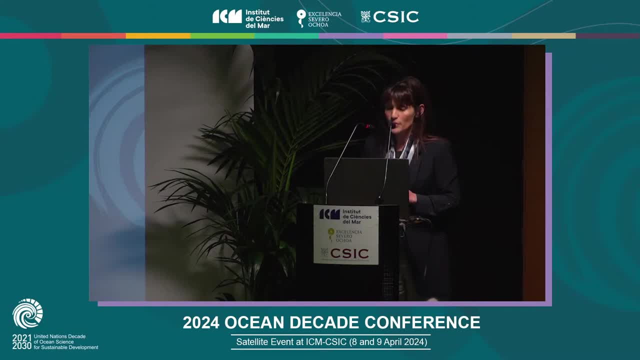 network of more than 2,000 researchers from the University of Porto working on Matizinhos-Cimar installation and dedicated only to marine ecosystem. we are conducting studies on sediments and nature-based solutions to minimize the impact of coastal overtopping. 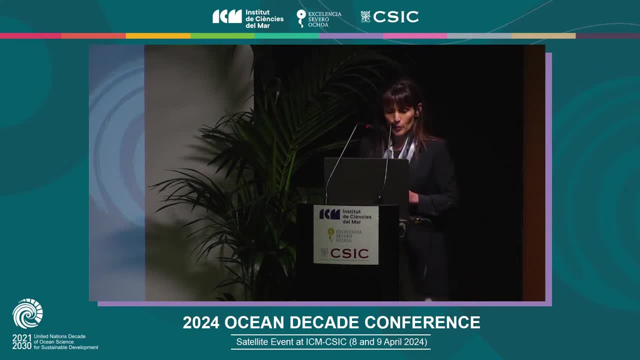 therefore protecting our communities In this compensation of sediments, especially on the areas that have been most affected. we are trying to have the process being done exclusively with elements of our own ecosystem, making the last impact possible on biodiversity. Still with CIMART, this research center, 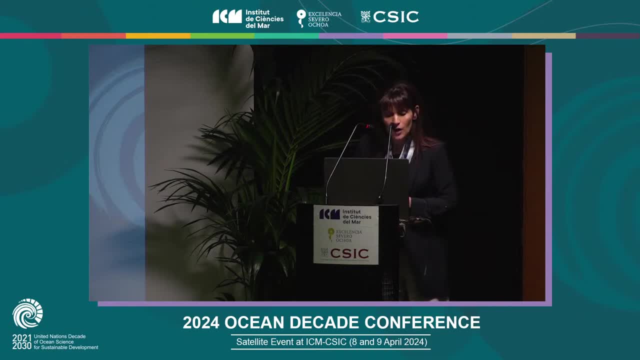 of the University of Porto, we are now integrating the ocean, its flora, in the strategy for carbon neutrality defined in the 2030 Agenda. mapping the sources of capture and storage of carbon in the ocean. Matizinhos has already reached the proposed goal. 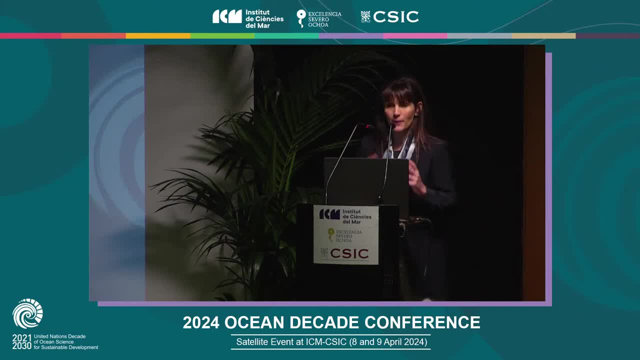 for 2030, working now on anticipating the goals for 2050.. With SAEA, that is the another research center in Matosinhos that is dedicated to investigation and engineering, and they have more than 4,000 engineers. 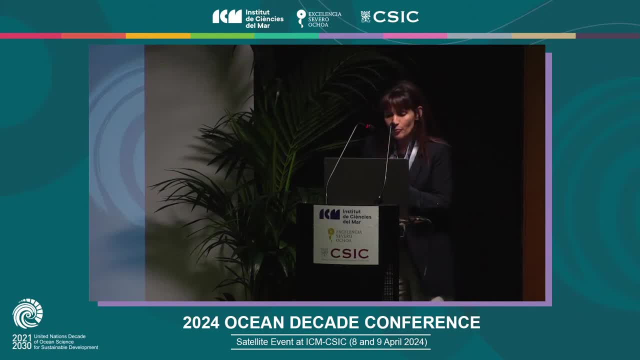 which is also located in Matosinhos. We have been developing deep ocean reading solutions with recently acquired technology implemented from Matosinhos to the Portuguese Navy, which use them on all countries. The investment in knowledge centers and interface institutions has been in the center of the political decision. 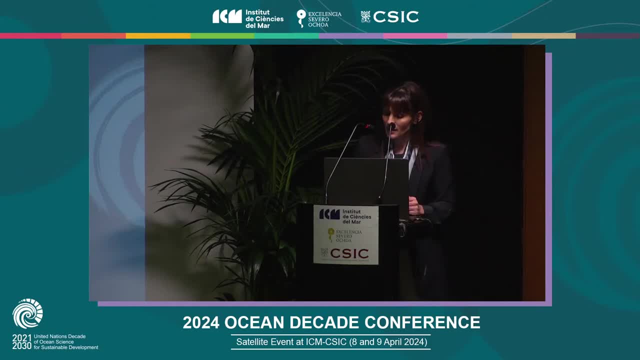 As for 2024,, we are expecting the beginning of the constructions of one more research unit with a budget of 12 million euros. Protecting the oceans, protecting marine and coastal biodiversity, protecting community and the stakeholders that foster blue economy has been one of the crucial points of Matosinhos' political agenda. 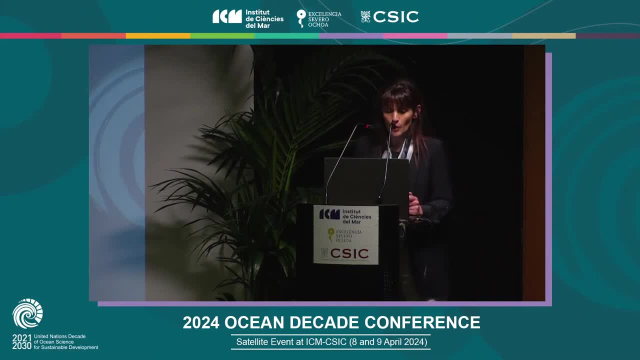 and one of the most significant commitments we have assumed as a United Nations Resilience Hub city, which we are. By participating in this project, we have been able to improve the quality of life in Matosinhos and we are happy to share our experiences with you. 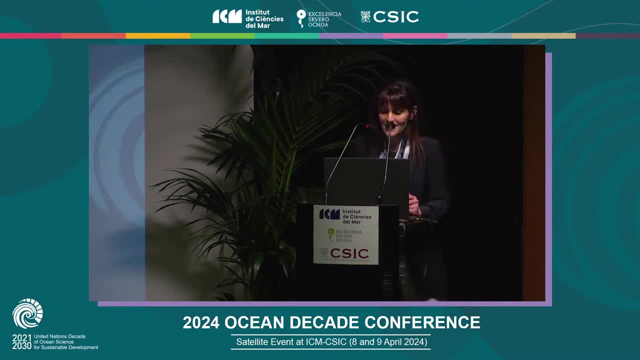 By participating in this Cities with the Ocean platform and integrating this call for action. we pretend to add value, sharing our experiences based on the diversity of the sea-connected sites we manage, but we have big expectations of learning and creating synergies that can connect our communities. 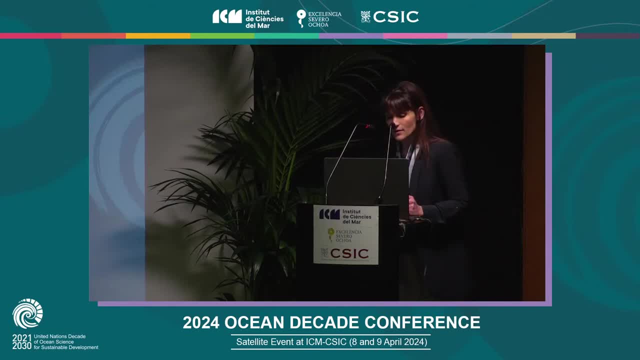 integrating policies and collectively answer to our questions. This is a global challenge, So we are available for everything that we need and we have big expectations on this work, on the sharing, on this project that we are building together. Thank you very much. 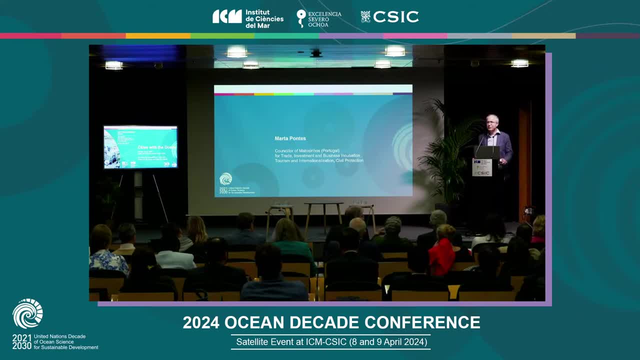 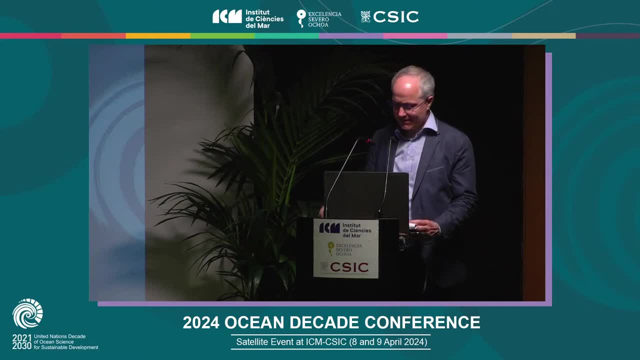 Thank you very much, Mrs Pontes, And now I'd like to invite Mrs Zhang Wei to join the scene As the executive director of the Ocean Decade International Cooperation Center and Qingdao Working Group on Cities with the Ocean platform. Mrs Wei will tell us how Qingdao carried out eight major marine actions. 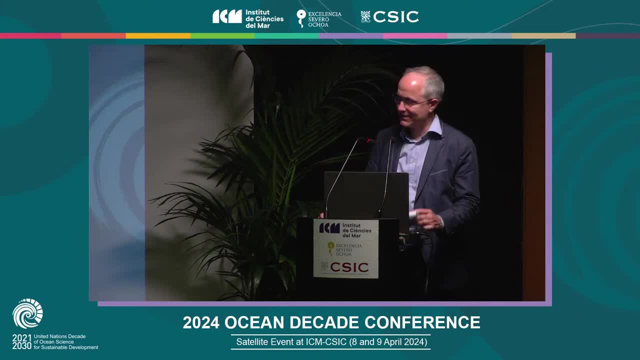 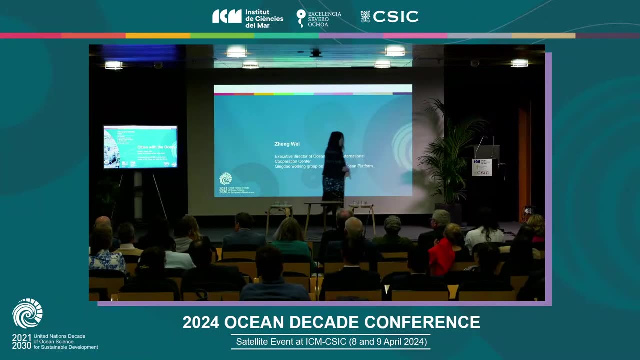 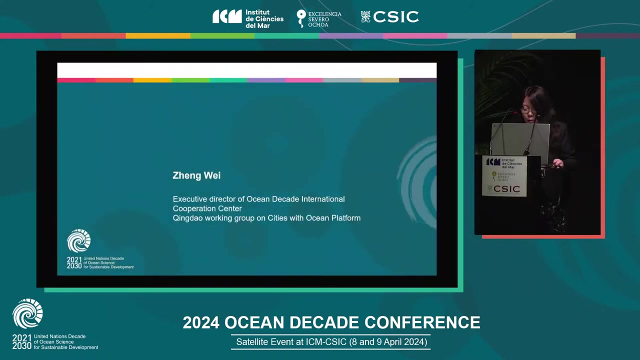 to create Ocean Decade best practices. Thank you, Thank you. Okay, thank you, Chair Distinguished guests, ladies and gentlemen, good afternoon. I'm Zhang Wei from Qingdao. It's my pleasure, it's my great pleasure to meet you all here in Barcelona. 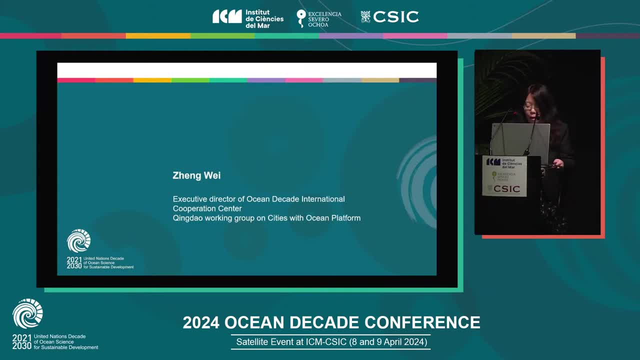 for the launching event of the Cities with the Ocean platform. On behalf of our Qingdao delegation, I would like to extend my warmest congratulations on the launch of the Cities with the Ocean platform. Qingdao is honored to be one of the founding members of the platform. 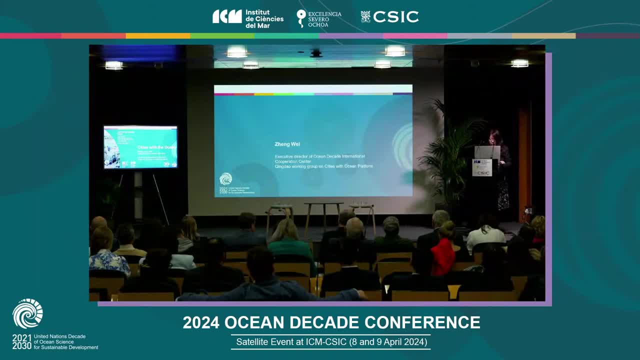 Qingdao has been an active participant in the Ocean Decade since its inception. A year ago, Qingdao established the Ocean Decade International Cooperation, ODCC. together with the Ministry of Natural Resources, Shandong Province, It has been providing a broad range of activities, including the development. 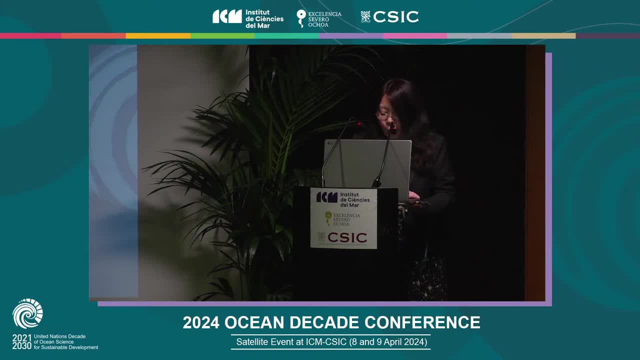 of marine concluding research facilities, community development and poi exploration, by providing a platform for exchange and cooperating among government bodies, international organizations, ocean-related research institute and other stakeholders to promote the in-depth integration of marine science with comprehensive governance and ultimately, to catalyze the transformative science solution. 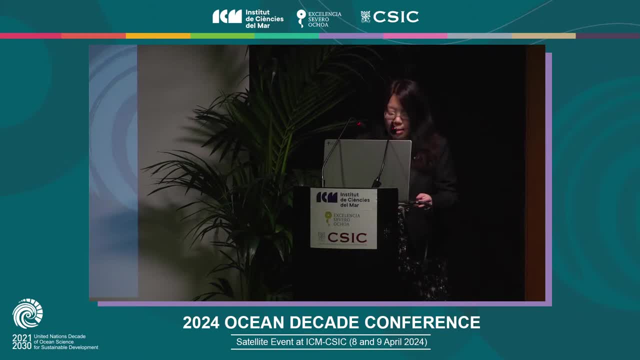 for sustainable development. In the future, ODCC will carry out eight major marine actions Aimed towards the escape of global warming. China has realized the potential of marine science and also including the these Western countries to promote the development of our best practice of China for the ocean decade. 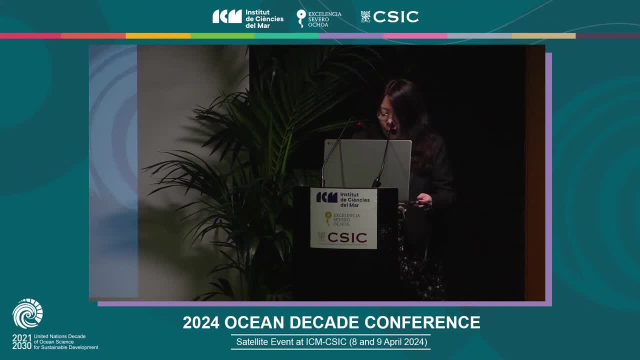 and carry out international demonstration and popularization. The first major marine action is contributing wisdom to the ocean decade. With this action, we will launch the Ocean Decade, China Action and YANSH program, promote the marine science and technology innovation and propose science-based ocean governance solution. The second action is 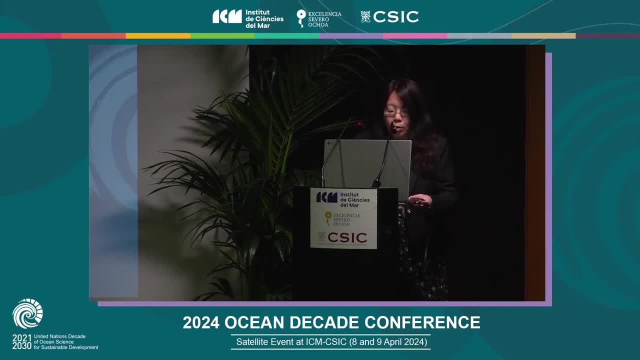 competing climate change. We will support the operation of DCC-OCC, promote the implementation of the Decade program, Ocean to Climate Simility Forecasting System, OSF. We aim to provide an ocean-based solution to global climate change With the third major marine action. 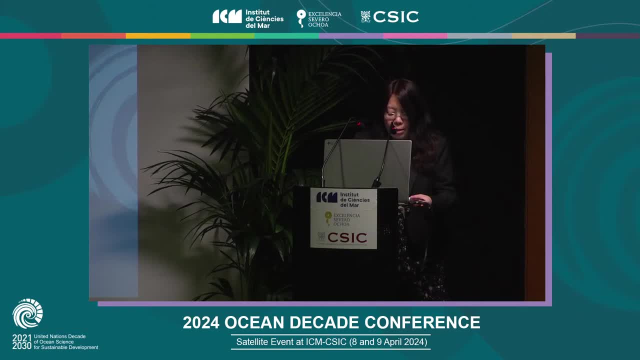 Fighting for a Healthy Ocean. we will organize a series of marine environmental practices and ecological restoration actions. We will also promote the implementation of the Dimension Tracing Project on ocean-negative carbon emissions- marine ecological practices and promote them globally. Energy-energized marine industry is our fourth marine action. We will provide an 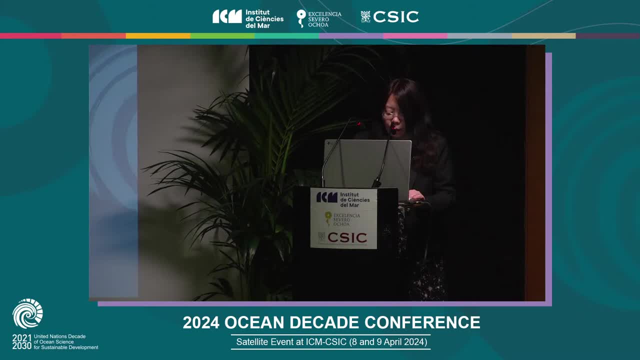 international cooperation and exchange platform for the marine industry through forum exhibition project roadshow. The fifth action is named Fostering Global Dialogue. Through organizing a series of international forums, seminars and exchanges, we aim to promote marine international cooperation and. 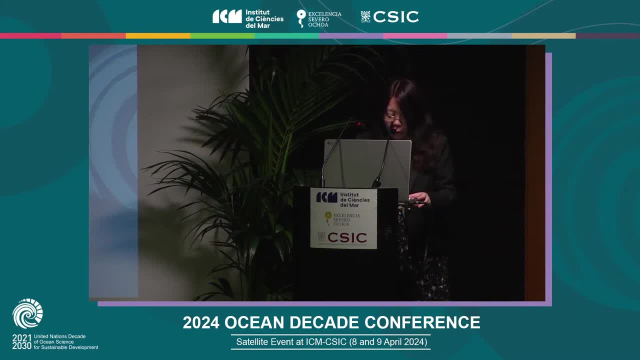 communication and deepen the linkage between marine science and governance and policy. With the third major marine action we will promote the 6-axis stimulating blue partnership. We will facilitate the process of building partnership with the World Economic Forum, the International Union for Conservation of. 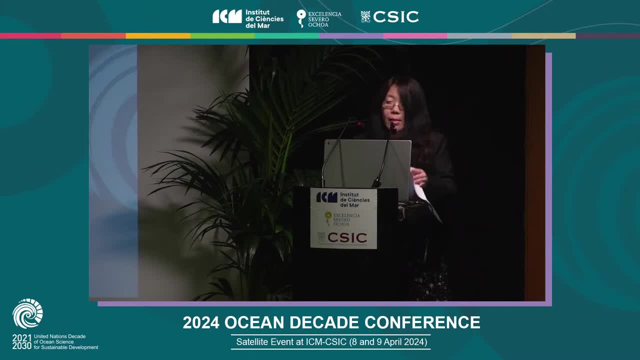 the Nature and other organizations with shared vision. We will plan to host several international organizations, including the Pogo Regional Node and the China Pemex Center, to build an international cooperation network for the ocean decade. For me, the marine think tank is the seventh major marine action. 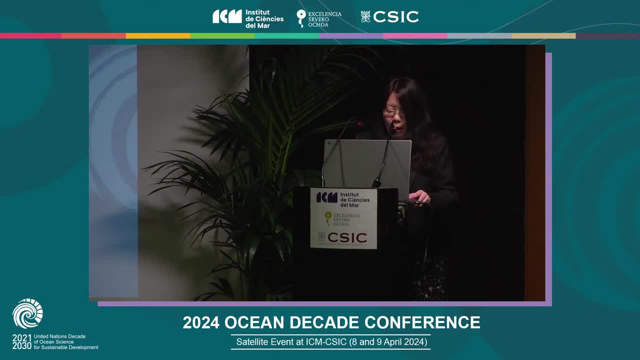 We will build a think tank to support implementation of the eight major actions. Finally, the eighth action is the facilitated capacity development. We will organize international training course on marine science and technology and the ocean governance to build the capacity for the young generation, especially for the ecops from the small island developing. 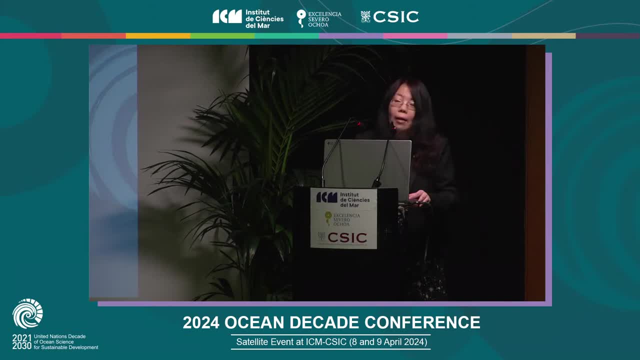 states and the least developed countries. Ladies and gentlemen, Qingdao, China and the Ocean Decade International Cooperation Center would like to join hands with all partners to embrace the ocean, care for the ocean, protect the ocean and turn the ocean we have into the ocean we want. Thank you. 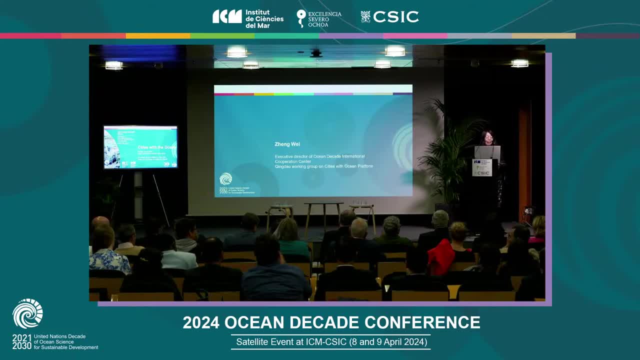 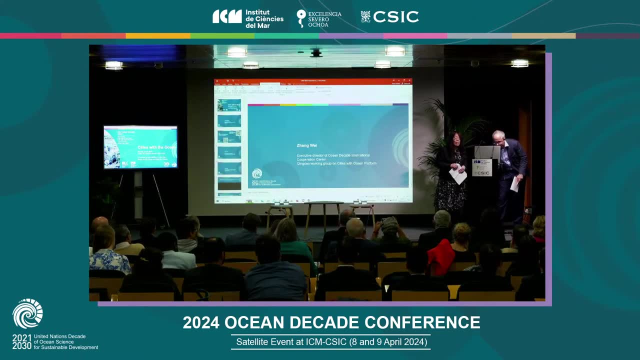 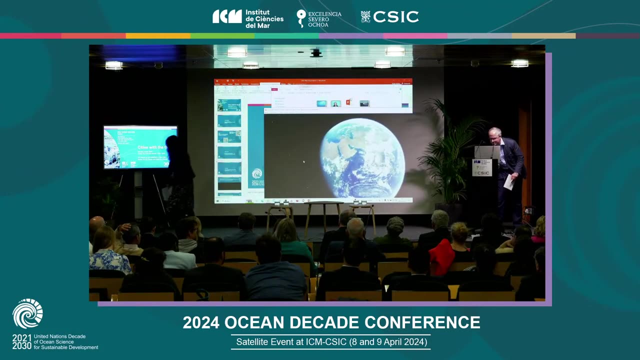 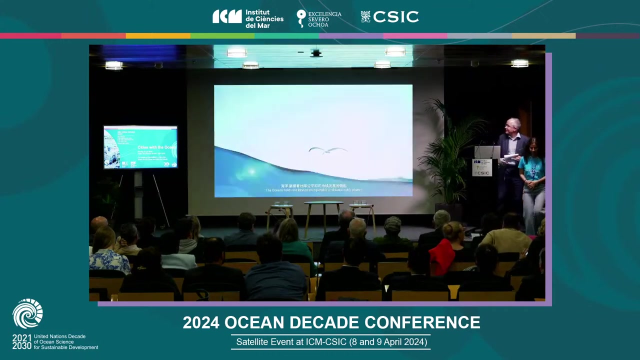 And we also prepared a video of how Qingdao engaged in the ocean decade. Yes, let's watch the video together. The oceans holds the keys to an equitable and sustainable planet. Launched in June of this year, the ocean has been a key to the development of the ocean. 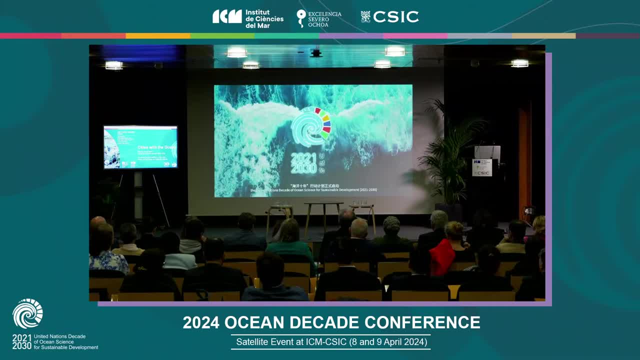 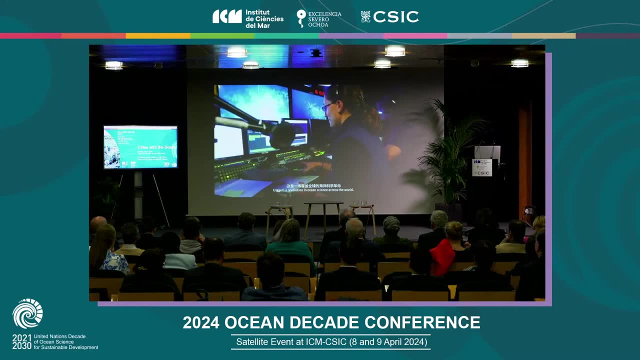 The ocean has been a key to the development of the ocean. The ocean has been a key to the development of the ocean. In January 2021, the United Nations Decade of Ocean Science for Sustainable Development- 2021 to 2030, triggers a revolution in ocean science across the world. 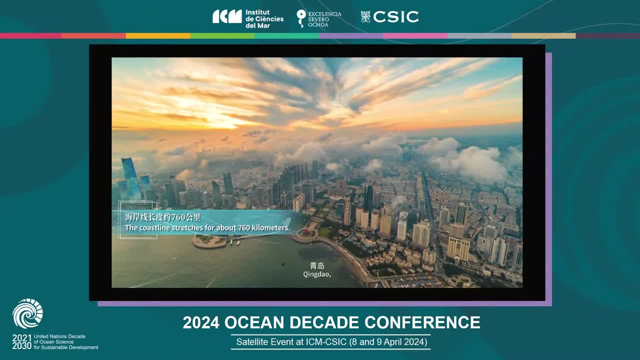 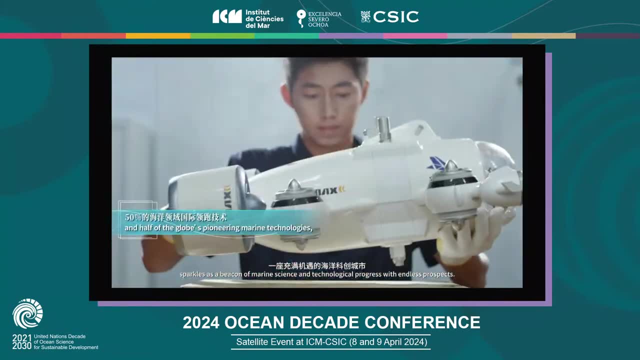 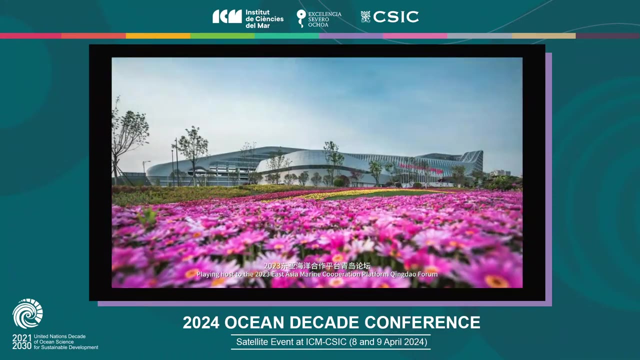 Qingdao, the gem on China's coastline, sparkles as a beacon of marine science and technological progress, with endless prospects. Playing host to the China's Coastline, Qingdao is the world's largest ocean science and technology center. Qingdao is the world's largest ocean science and technology center. 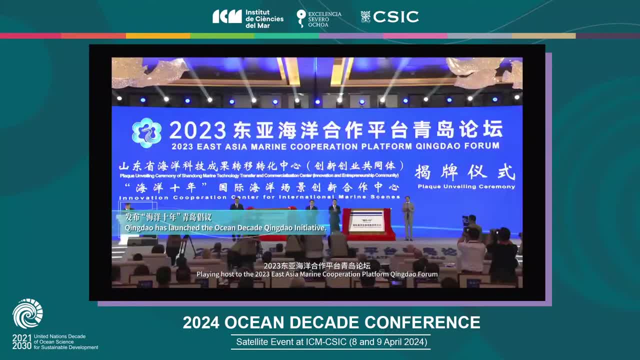 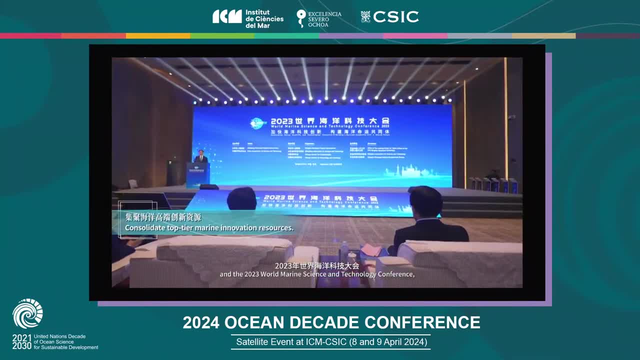 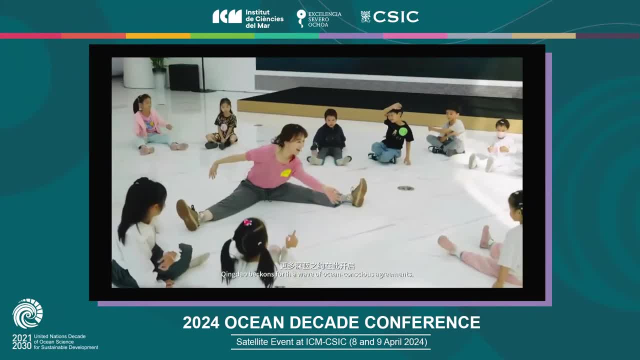 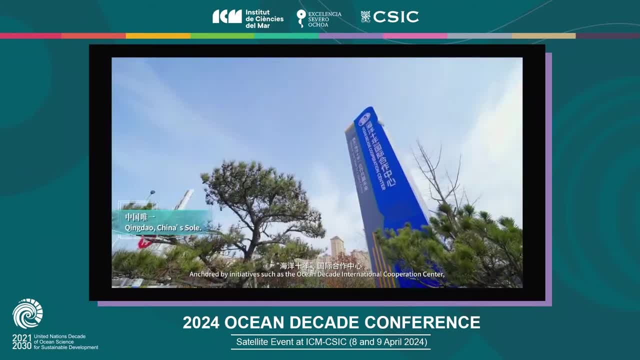 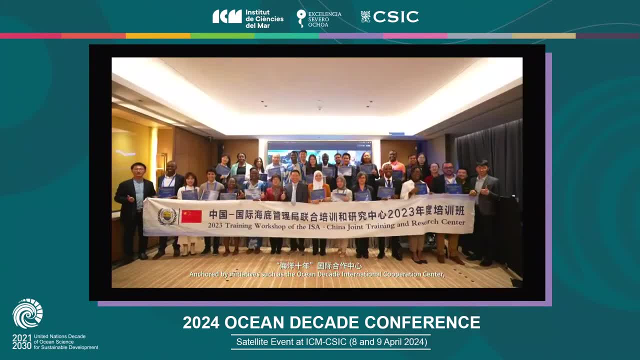 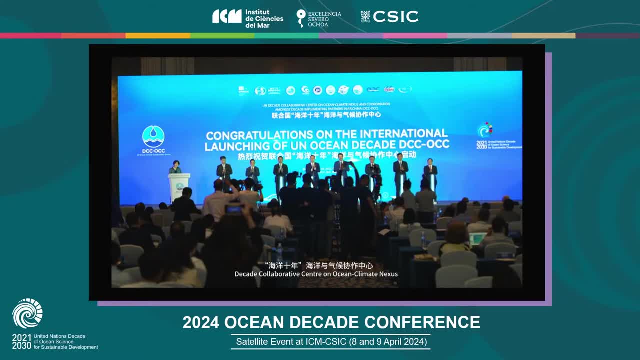 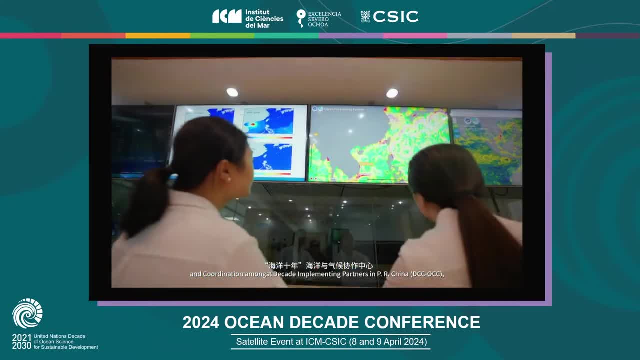 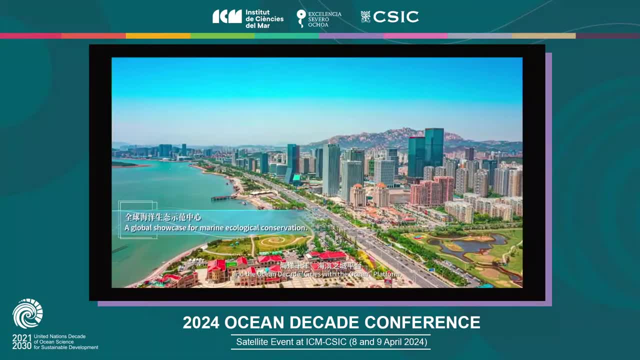 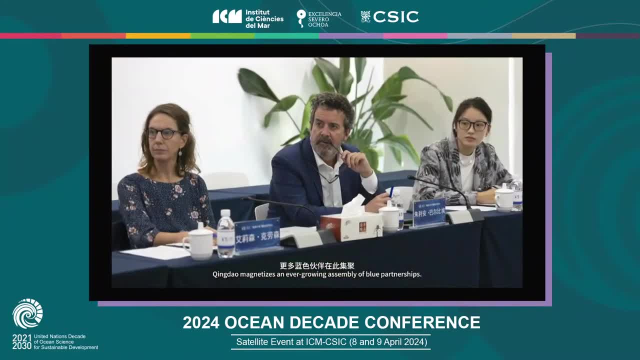 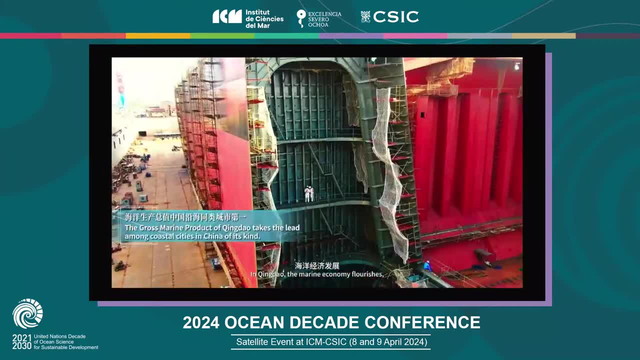 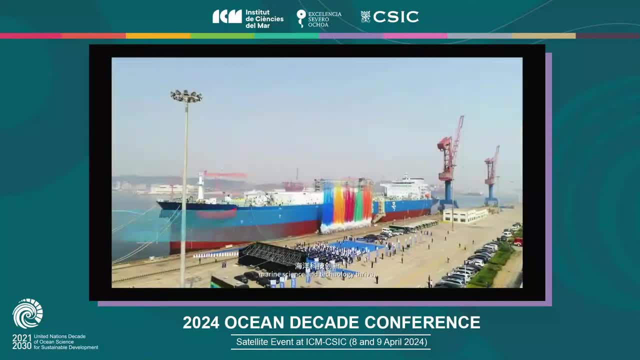 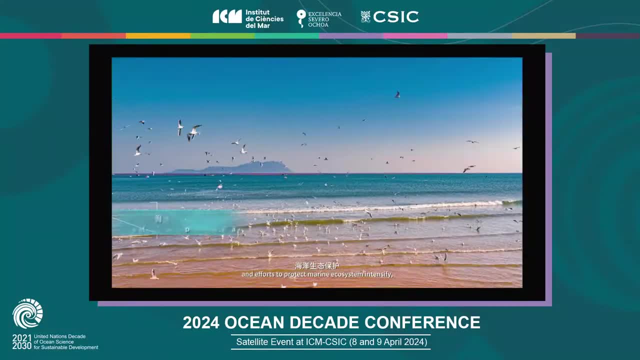 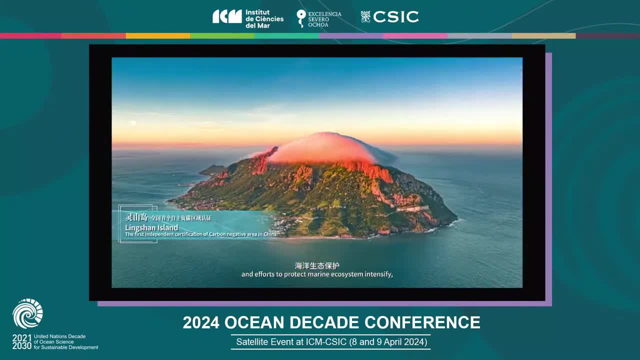 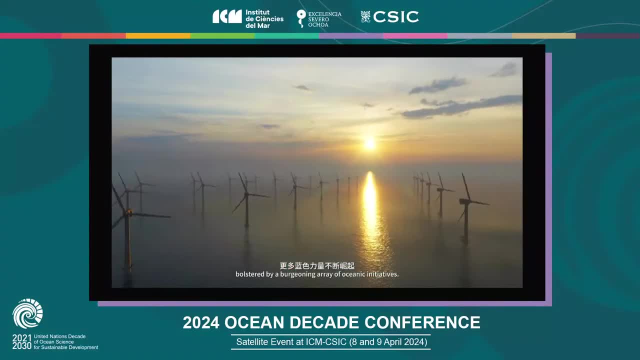 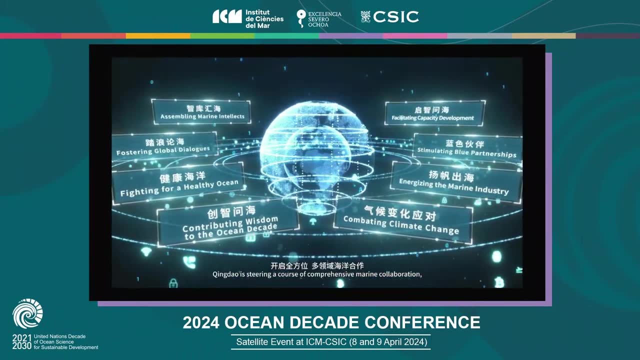 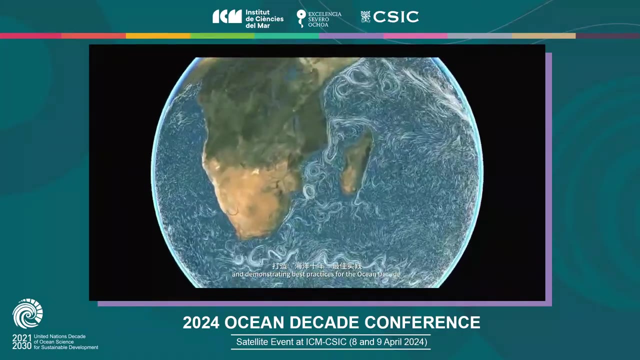 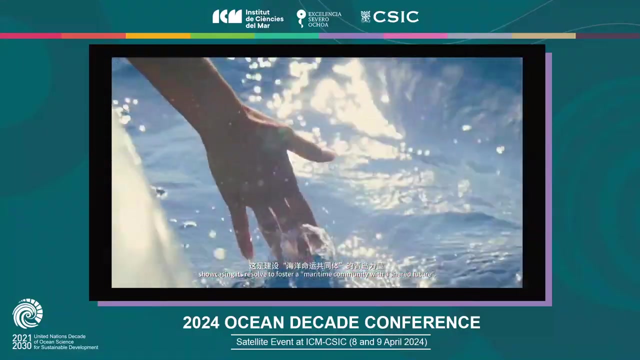 fostered by a burgeoning array of oceanic initiatives. With the eight major marine actions, Qingdao is steering a course of comprehensive marine collaboration and demonstrating best practices for the ocean decade. This movement echoes Qingdao's call for the ocean decade, showcasing its resolve to foster a maritime community with a shared future. 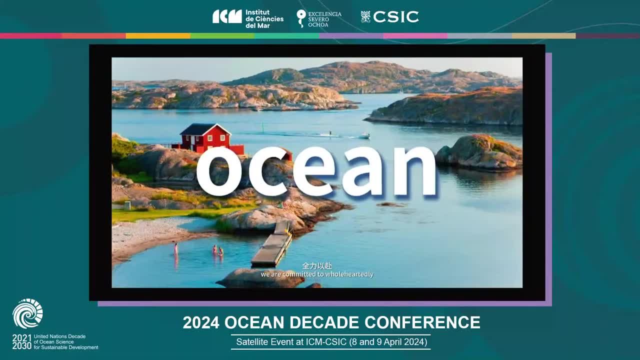 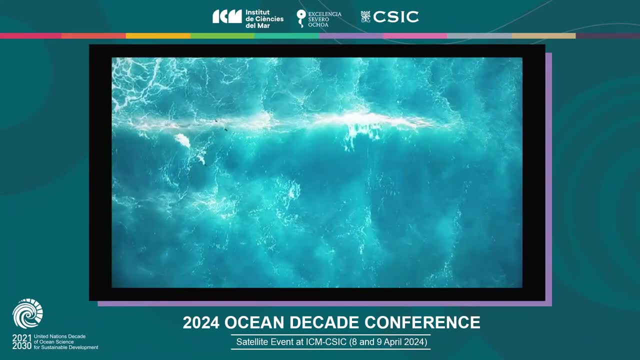 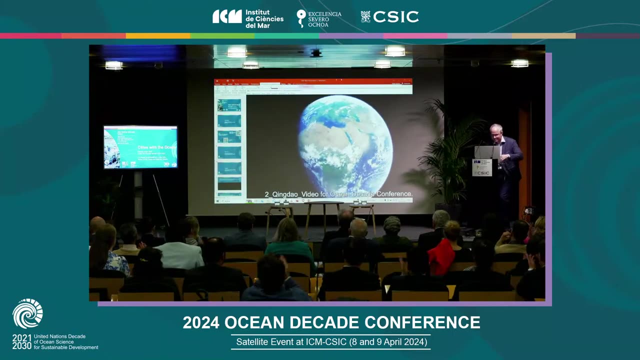 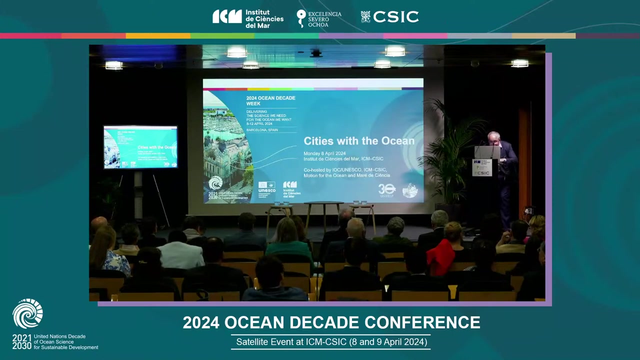 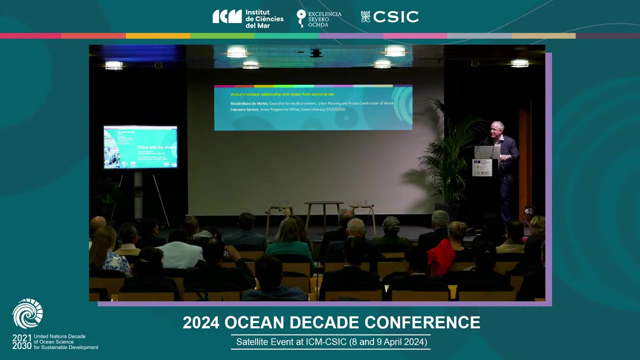 Armed by a shared future. we are committed to wholeheartedly delivering the science we need for the ocean we want. Now it's time to start a series of panels, or I would rather say dialogues, between cities and ocean science, And to start with, 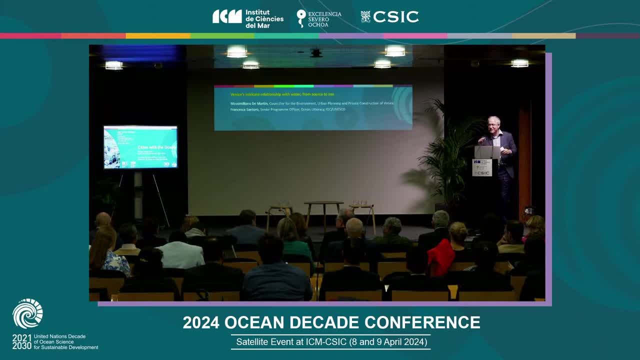 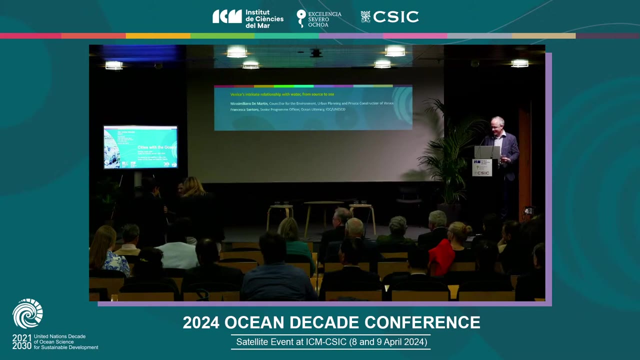 we'll get back to the Mediterranean and to the city of Venice, well known for its connection with water, both salty and fresh water, and they will share the vision of Venice on this relation And it's my pleasure to welcome Massilia Miliano de Martin. 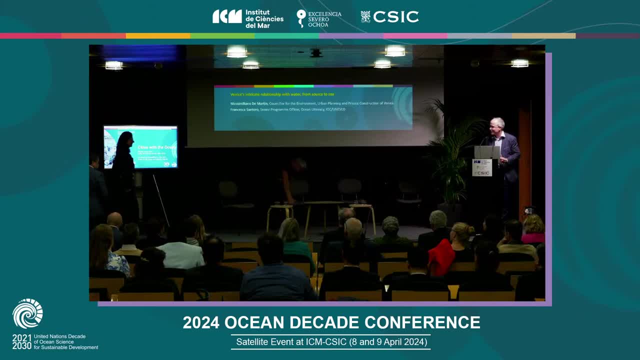 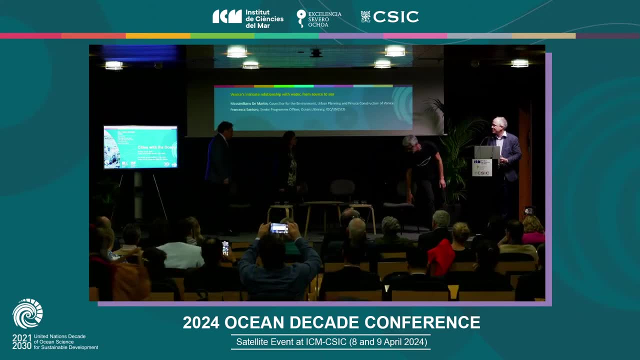 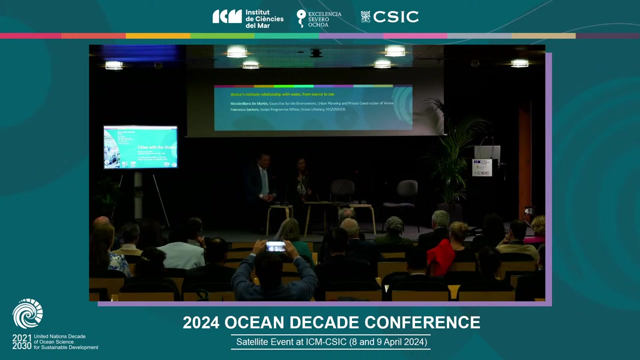 the Councilor for the Environment, Urban Planning and Private Construction, together with Francesca Santoro, Senior Program Officer for Ocean Literacy at the IOC, UNESCO and based in Venice too. Thank you, It's a great pleasure to be here. Thanks to Olivier for the invitation. 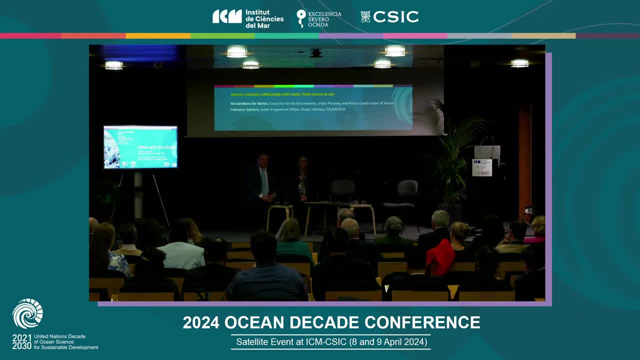 and to be here with the Councilor for the Environment of the City of Venice, but also seeing all friends, because I we organize a summer school with the city of Matusinius and we also brought our ocean and climate village to Cindao. 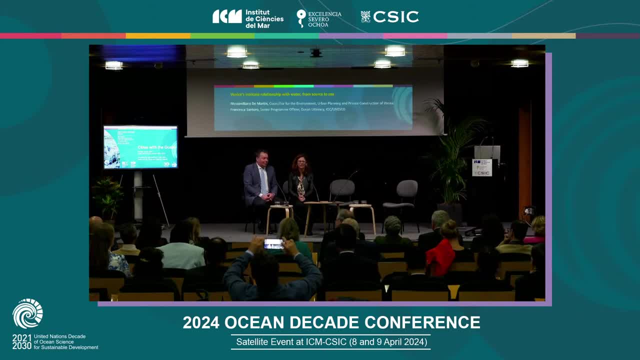 so it's a kind of connection already existing and probably the thread is ocean literacy here. So I'm based in the city of Venice, at the UNESCO Regional Bureau for Science and Culture in Europe, where we have an IOC project office, and of course we work very closely with the city of Venice. 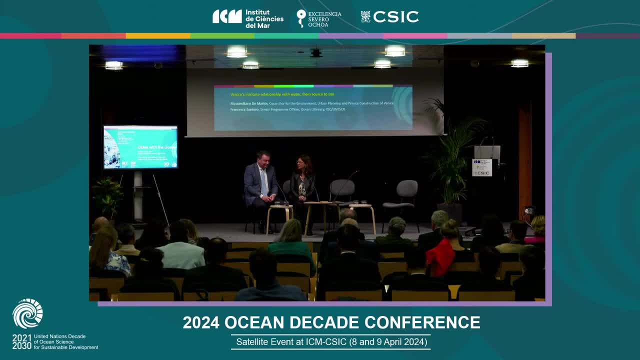 and in particular with the Councilor for the Environment, and with him we're going to tell you a little bit some initiatives that we have been developing together. So I'm going to also play the role of interpreter here for Massimiliano, so I will have this jewel hat. 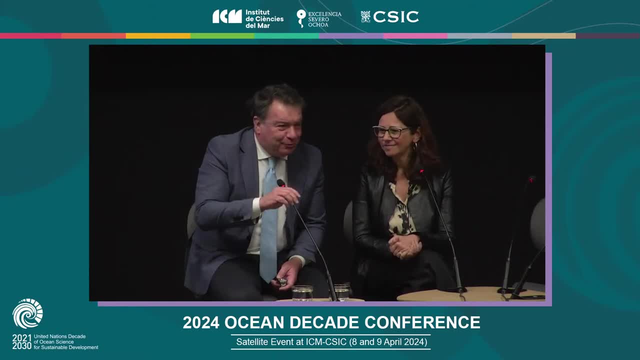 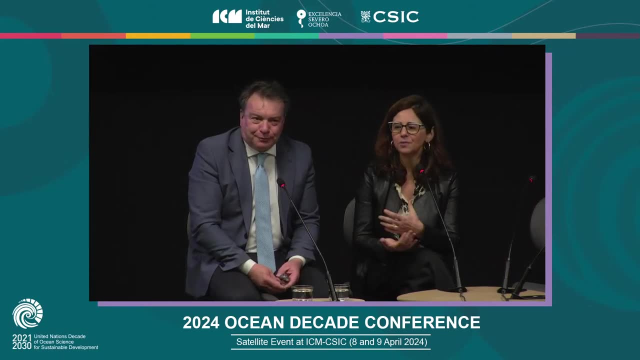 Thank you, Francesca. Through my voice, first of all, I bring the greeting of the city of Venice to all of you, and we also thank you for the invitation. So through myself, here, I'm bringing all the wishes from the city of Venice to all of you. 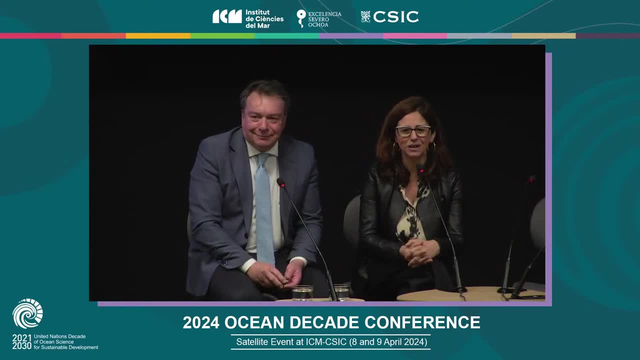 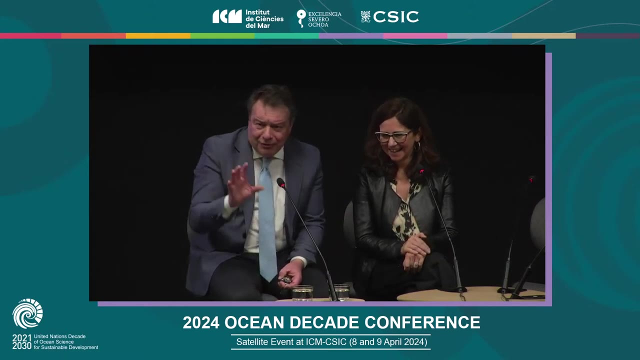 So I know that I have to stay in the minutes that were given to me, so I'm going to speak half of the time of the rest of the colleagues to allow for the translation. Then, when you face it from a cognitive point of view, 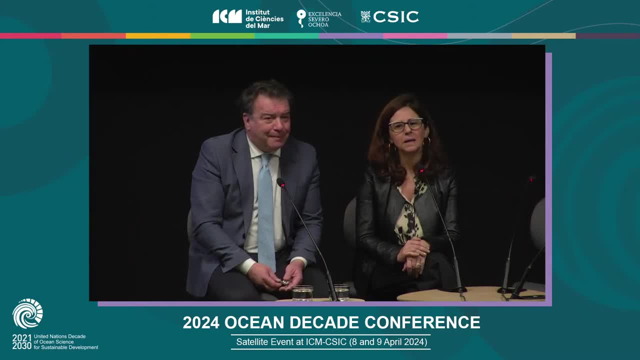 it's a very complex city. So it might seem easy to talk about Venice because everybody knows about Venice, we have all images about the city, but when we start talking about the problems and the issues of the city, it's really a very complex environment. 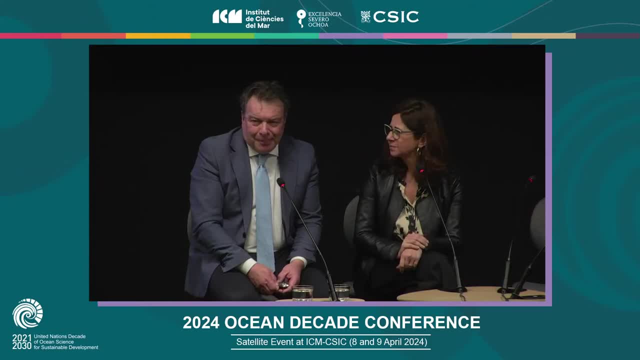 and a lot of things that are interacting with each other. It's a great city for its history, for its culture, for its knowledge, but from an urbanistic, administrative point of view it's very small. So it's a big city for the history. 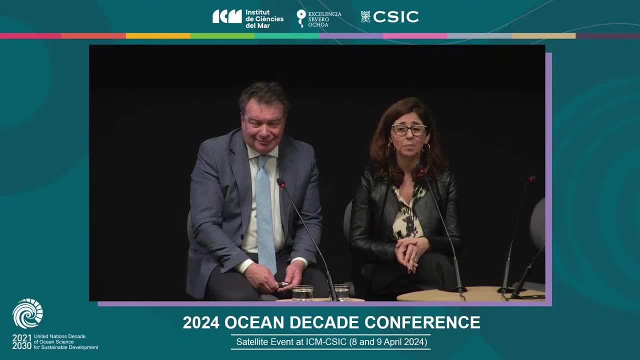 for the cultural heritage, but actually the actual space that it covers is quite limited. So I want to make it clear right away from a point of view: When we talk about Venice, often those who come to the city think of Venice and look at the sea. 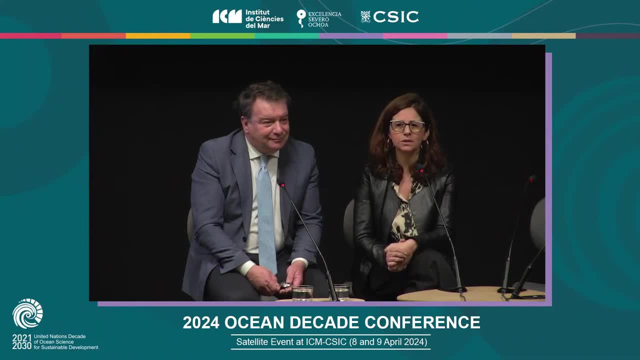 I want to start by saying something very important: that all the people that are coming to Venice, they are in the city but they look towards the sea. For this reason, in Venice we have the biggest engineering infrastructure of the world. It's a dam that defends the city of Venice. 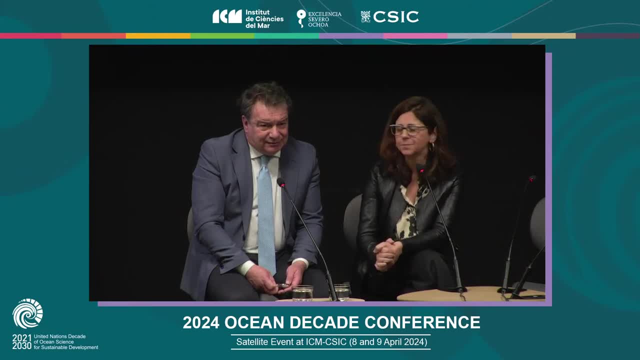 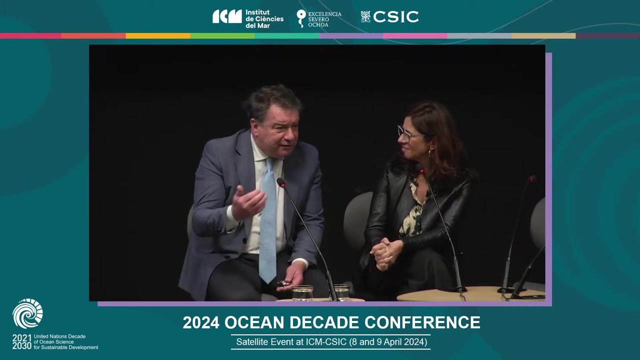 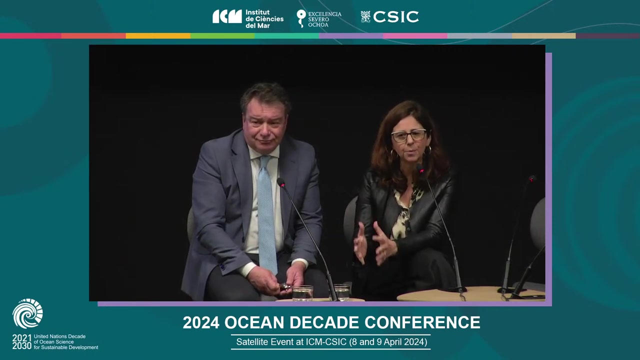 from sea level rise, and its name is Mose. So this engineering work has been designed in order to last for more than 100 years. But we also need to look backwards and think that we need to connect what is happening in the lagoon and in the sea. 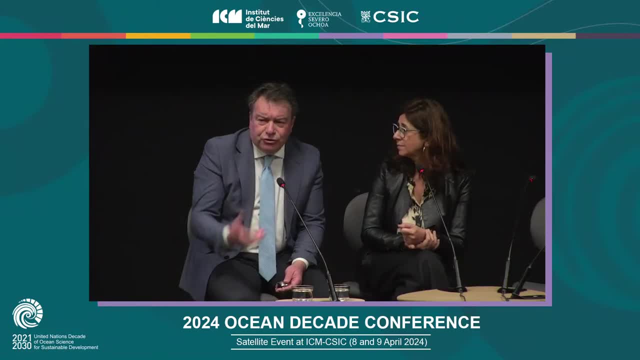 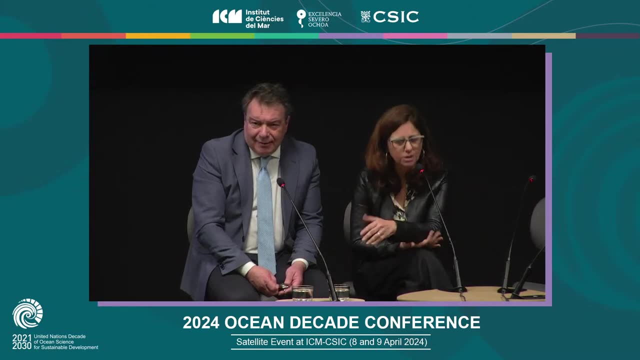 connected to what happens in the rivers, And there are six rivers that are connecting the land part to the sea part through the lagoon of Venice, And they were always the biggest threat for the city. The enemies came through the sea, the nature came through the river to attack it. So the first engineering works of the city to defend itself from the sea- not from the sea but from the waters, especially the river ones- started in 1350.. So in 1350, the first hydraulic and engineering infrastructure started. just to control actually. 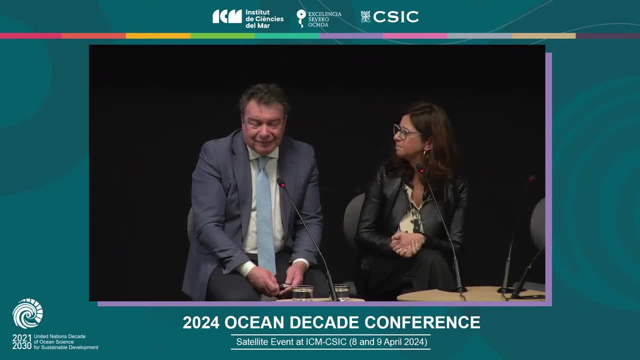 the rivers that were coming into the lagoon. So it's a paradox, but the rivers were bringing all the sediment into the lagoon, and so they were threatening the lagoon to actually become all land part. Per questo motivo, dal 1350, la città si difende della natura. 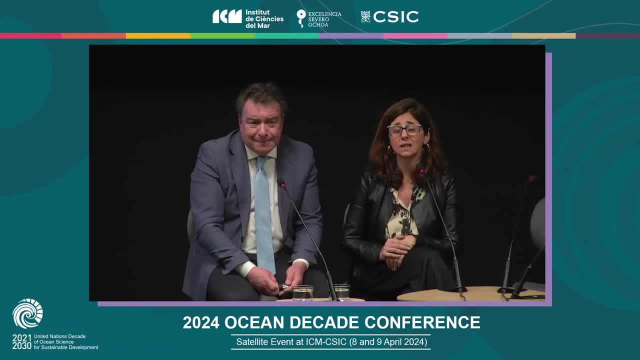 e la sta sfidando. So it's since 1350 that the city protects itself from nature and from natural risks. Queste poche parole per dirvi anche solo due dati, perché poi entriamo invece nell'aspetto, quello importante. 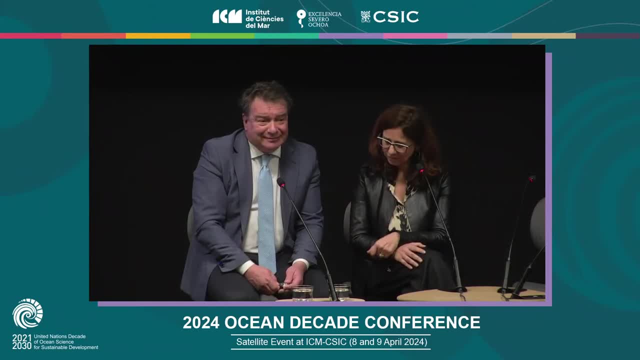 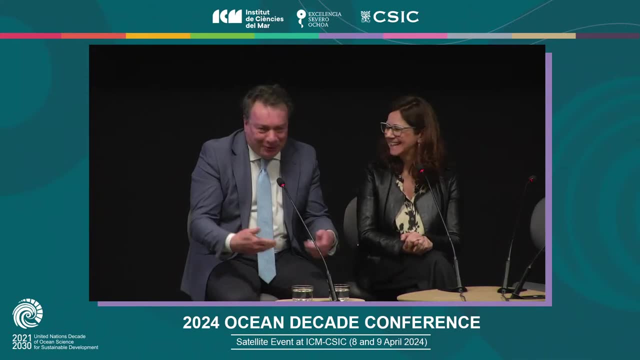 quello educativo e formativo. Ah, so I thought you wanted to continue. Non abbiamo il copione, parliamo a braccio. So just two numbers to set the scene, and then I'm going to talk about some concrete examples. 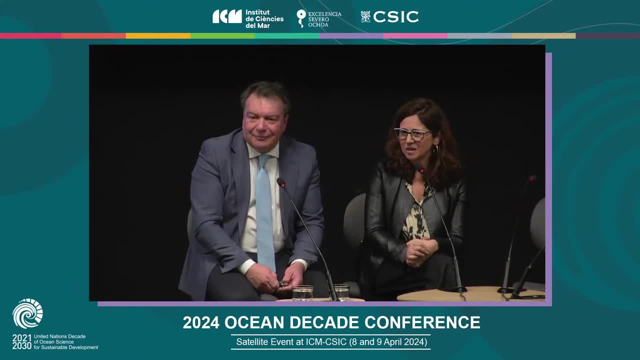 Cosa fa la città di Venezia oggi per difendersi dalle acque? What the city of Venice does today to defend itself from waters? Sta investendo più di 100 milioni di euro per difendersi proprio dei fiumi della terraferma. 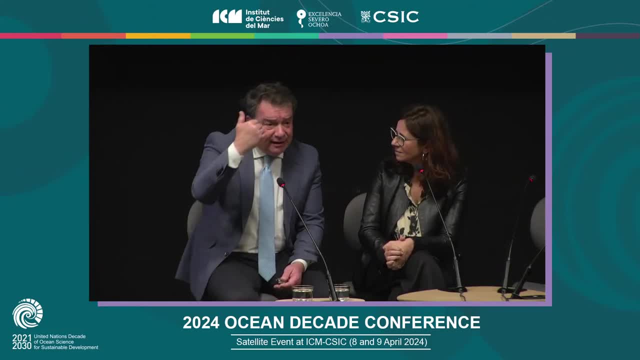 Se vogliamo difendere la città, bisogna pensare a investire e progettare nella terraferma. So the city is investing more than 100 million euros to protect itself from rivers Per due motivi. Il primo è difendersi dai rischi idrogeologici. 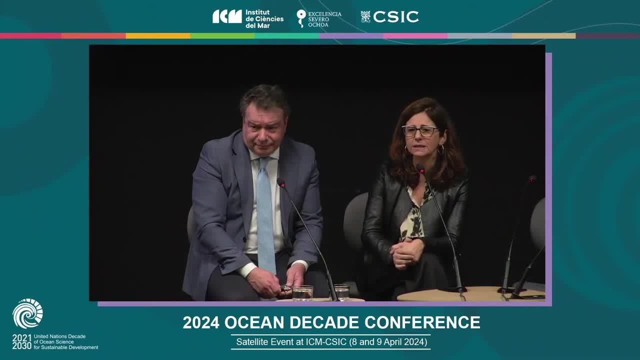 So for two reasons: The first one is to protect itself from hydrogeological risks, Il secondo per rimettere nella laguna delle acque sempre più pulite gestendo i nutrienti, And the second one is to make sure. 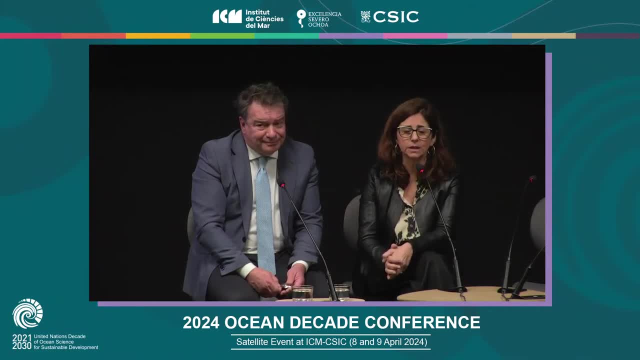 that the inputs into the laguna is cleaner and cleaner and with less nutrients than possible. Ecco perché nel nostro piano di azione del clima noi stiamo anche gestendo i dati che ci vengono da 130 km di distanza della città. 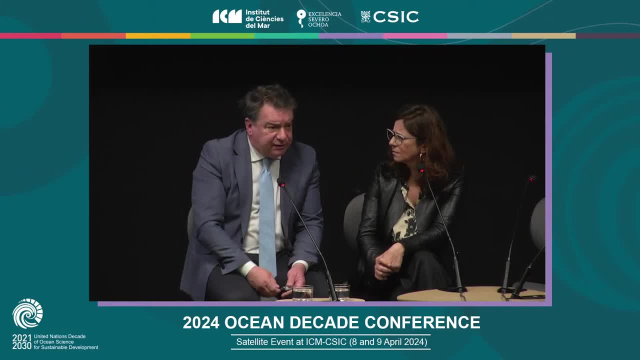 che sono i ghiacciai e i nevai delle Dolomiti. That's why, into the climate adaptation plan of the city of Venice, we are including data coming from 130 km from the city itself, so from the mountains. 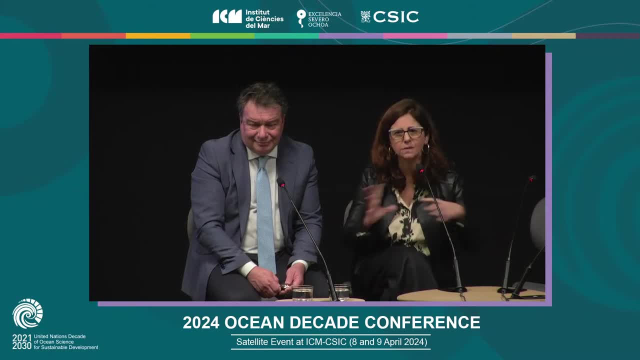 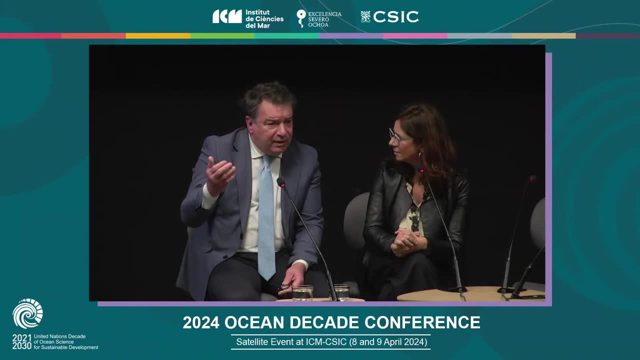 because we are well aware that we need to have this integrated and holistic approach to water management. Questi 100 milioni servono proprio per gestire le acque e per mettere in sicurezza il territorio. So these 100 million euros are invested. 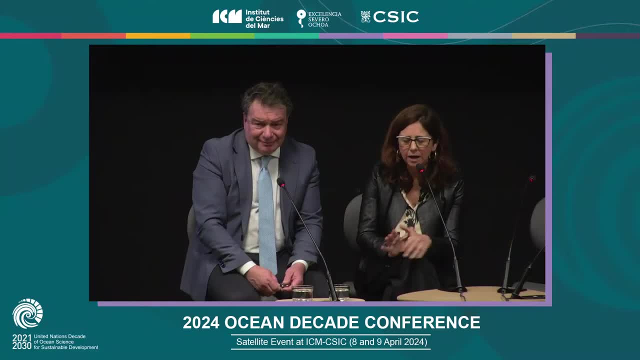 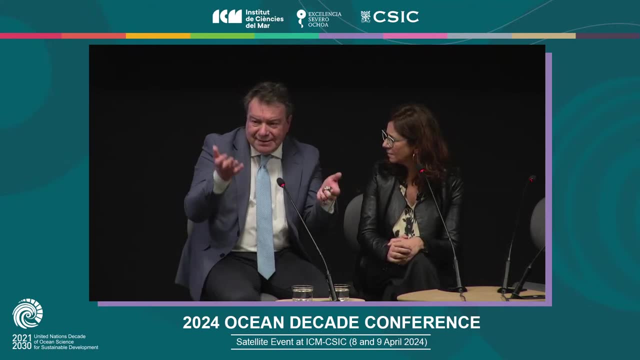 to protect the city of Venice from hydrological risks. Quindi, in sintesi, MOSE, Interventi di Opera di Ingegneria Idraulica, Terraferma, gestiamo l'innalzamento dei mari. 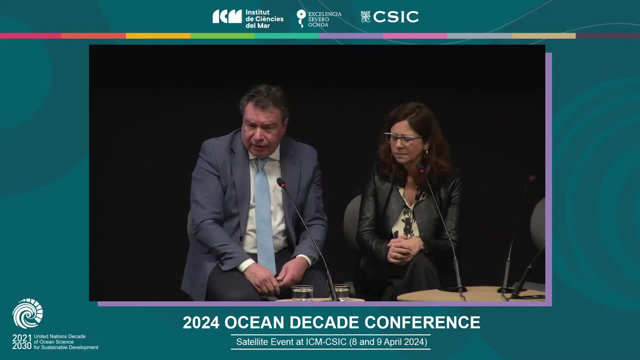 e l'innalzamento anche dei sedimenti della laguna. So, in a nutshell, there is MOSE, which is this hydrological, huge hydrological engineering work that protects the city of Venice from sea level rise, so seaward. 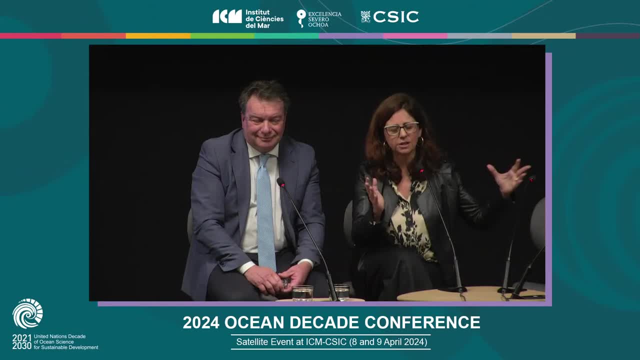 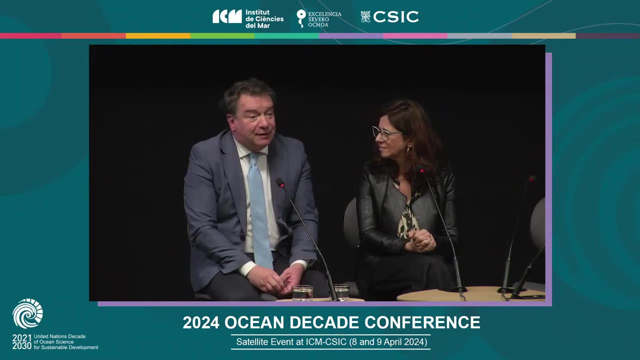 and also 100 million euros invested in the land, part from the rivers to the city. Ora, oggi, i progetti più attuali, invece, che riusciamo a fare dal punto di vista metodologico ed educativo, riusciamo a farli proprio con dei partner come UNESCO. 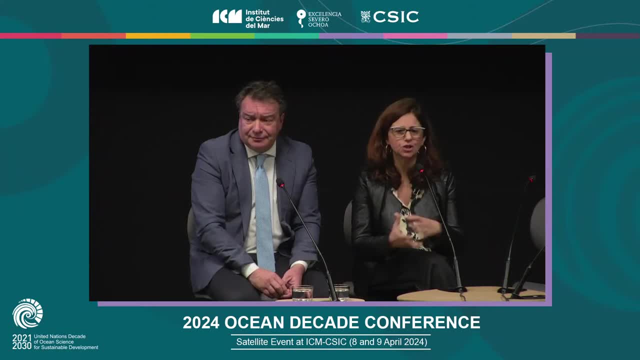 Nowadays, the most operational and concrete and educational activities that we are putting in place in the city of Venice are being done with partners like UNESCO. Da tre anni stiamo lavorando in montagna, duemila metri di altezza, per tre giorni. 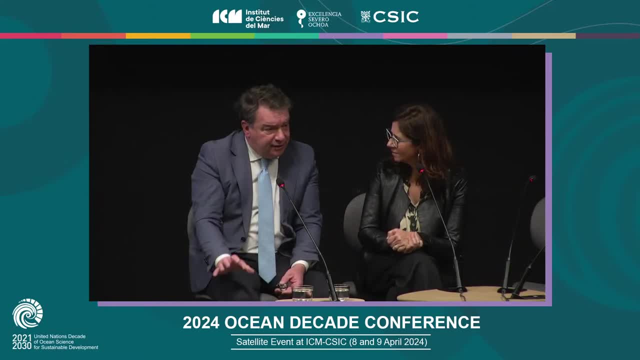 proprio per parlare della qualità dell'acqua dalle sorgenti alle foci. It's been three years that we started to work together on the idea of organizing a workshop that we call From the Source to the Sea. So we organize this workshop together in the mountains. 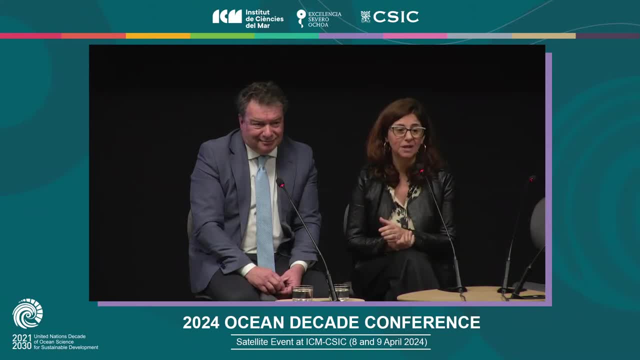 in the Dolomites, in the Alps, to talk about what is happening in the lagoon and in the sea, Assieme anche al Consiglio Nazionale delle Ricerche, Together with the Italian National Council of Research, E l'anno scorso per la prima volta, 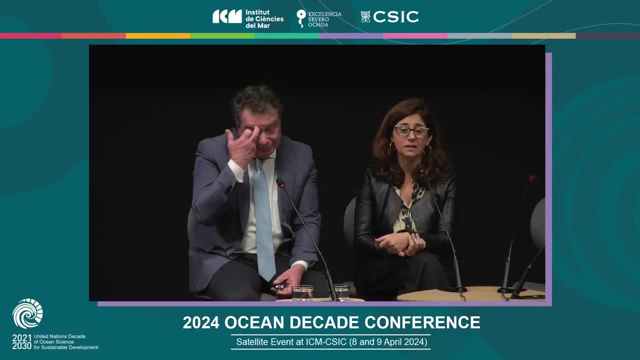 anche il Gran Teatro, La Fenice, And also with the Lyric Theater of the city of Venice, La Fenice. Pensiamo che le politiche ambientali passino anche attraverso la conoscenza dell'arte e della cultura, So we think that environmental policies 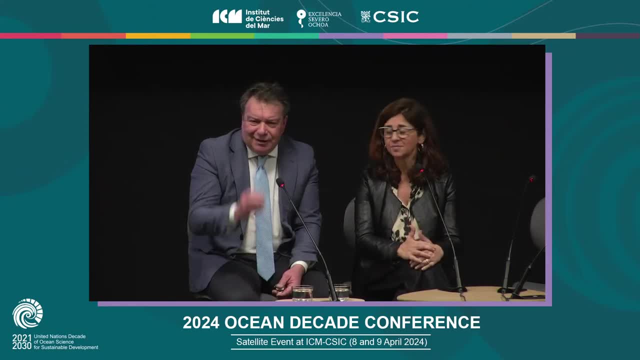 can also be developed through art and through culture. Al Galassi, il Gran Teatro, La Fenice mi ha fatto pensare sopraintendente quando mi ha detto: ma tu sai quante volte la nostra orchestra ripercorre il suono dell'acqua? 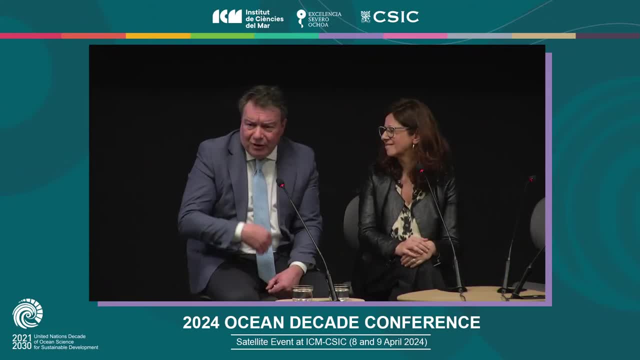 dalle grandine alle tempeste a Ruscello, al mare mosso al mare fermo alle tempeste. So the president of the foundation of the theater made me think. you know, do you know how many times we actually reproduce with music and with instruments? 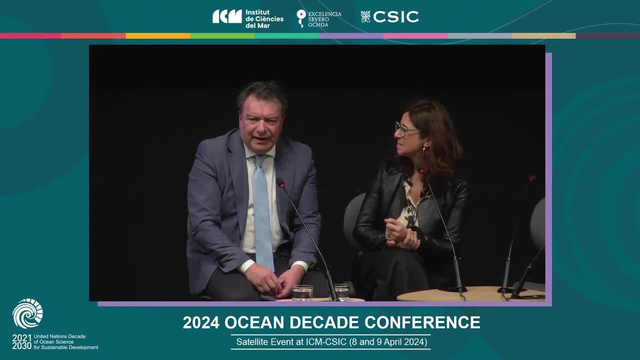 all the sounds of water, E così anche i testi delle parole delle opere. ripercorrono anche molte condizioni ambientali dei secoli passati, And even the words of the operas are talking about environmental topics, Quindi l'ambiente non è solo materia scientifica. 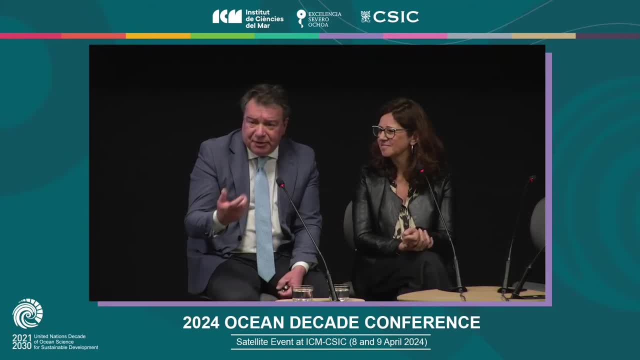 ma è materia che ha espresso sempre un tema che è sempre espresso le possibilità alle persone di esprimere le loro arti. So environmental issues are not only a scientific topic, but also a cultural, artistic topic, and this is a good way for letting everybody express. 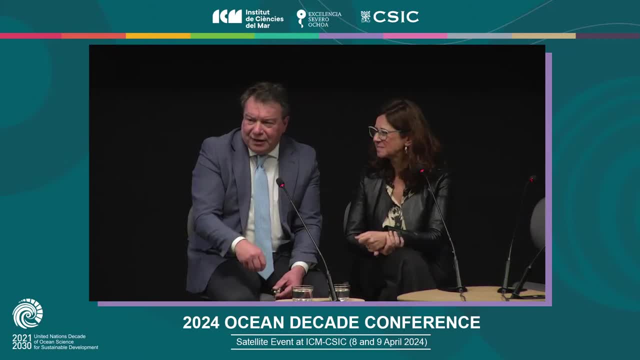 what they think about those topics. Quindi, in questo caso, il Gran Teatro La Fenice con il suo coro, ha suonato e cantato in rifugio temi che riguardavano l'acqua. 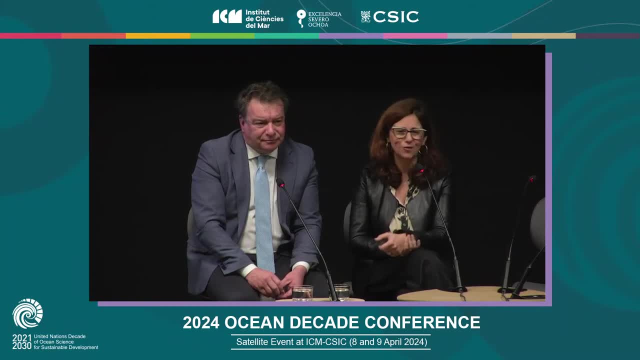 So in last year the choir, the choir of the theater, they came up in the mountain to sing a song about water and environmental issues in the mountain. Poi un altro progetto bellissimo è quello che stiamo portando avanti con UNESCO. 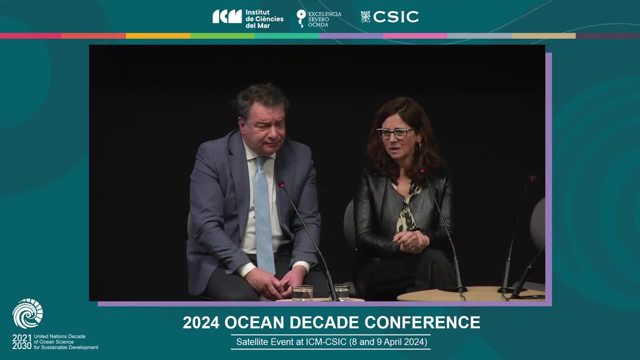 è il gruppo Prada, l'Asilo della Laguna. Another project that we are implementing in the city of Venice is done with UNESCO and with the Prada group, and it's called the Kindergarten of the Lagoon. Abbiamo capito che i nostri bambini 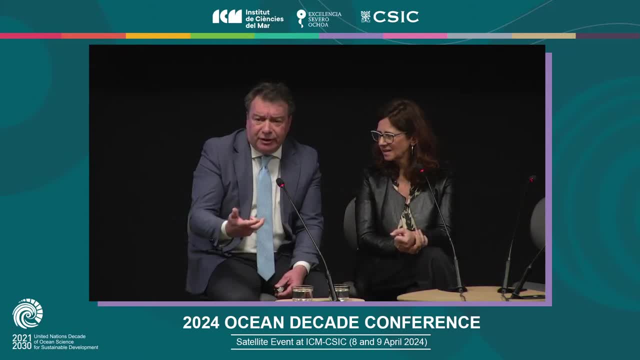 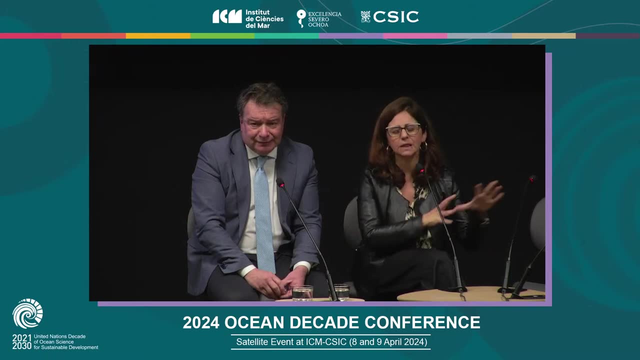 sia quelli dell'isola, del centro storico, delle isole della terraferma, non conoscono il loro territorio. We realized that the kids, both the kids living in the city and those living in the mainland, were not knowing actually their environment. 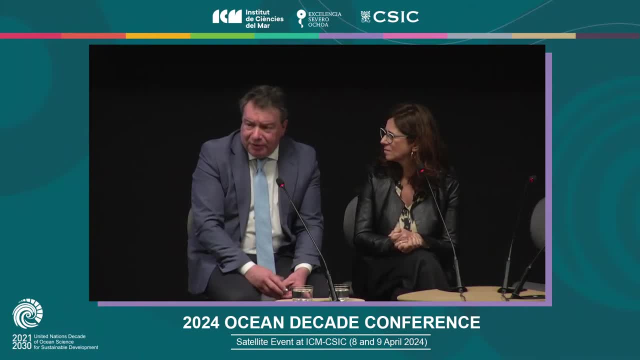 Genitori e famiglie che non hanno mai accompagnato i bambini a scoprire la nostra città. dal punto di vista ambientale, So families, parents that never brought their kids to know better their natural environment. Quindi, grazie a UNESCO e il gruppo Prada. 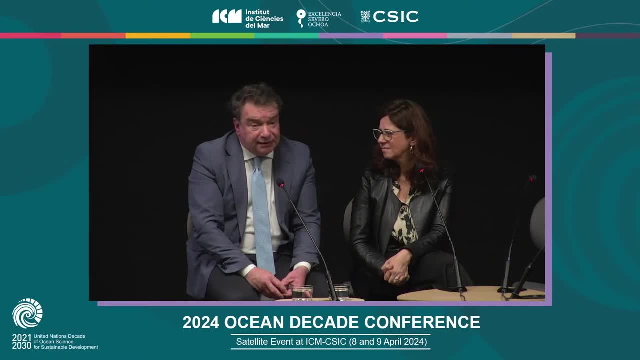 è stato creato un percorso metodologico, didattico e formativo, non solo per i bambini, ma anche per gli insegnanti. So, through the help of UNESCO and the Prada group, we were able to create a training, a capacity development program. 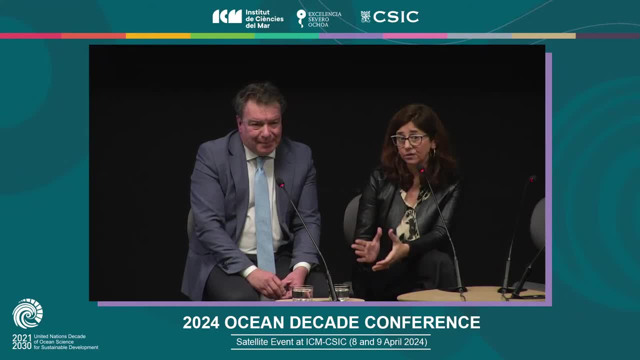 not only for the kids, but also for the teachers and for the families, E questa è stata un'occasione, soprattutto per i bambini, di parlare a casa della propria città, And so the kids that were learning in the field. 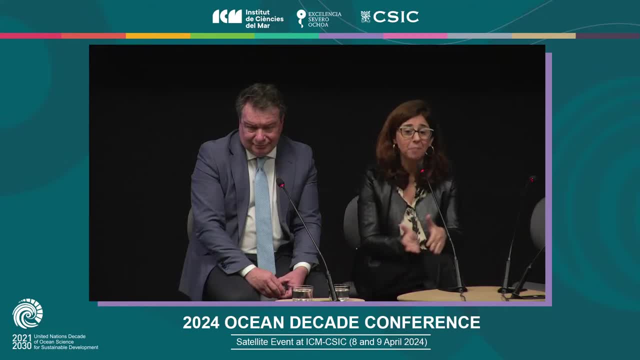 about their lagoon and their environment were then bringing back what they learned to their families, their parents and their relatives. Ed è stata anche occasione per formare in un modo diverso il nostro corpo insegnante delle nostre scuole. 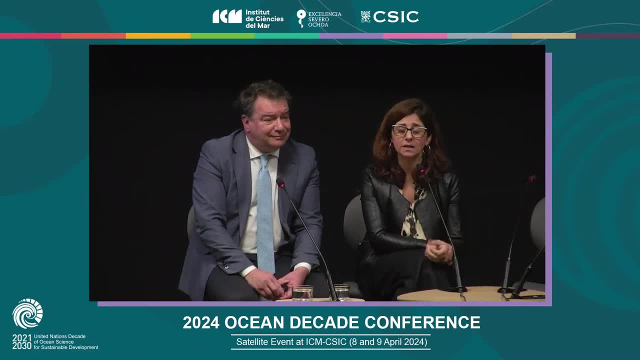 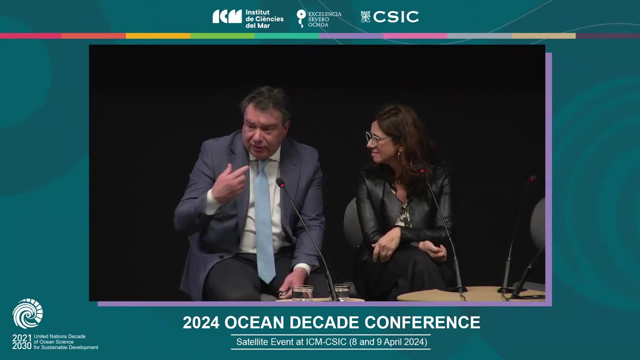 And so the teachers were also trained in ocean literacy, in outdoor education, and so they really learned a new way of teaching and a new way of educating the young For the younger generations. Pensiamo che sia molto importante parlare in più lingue. io che parlo italiano e basta. 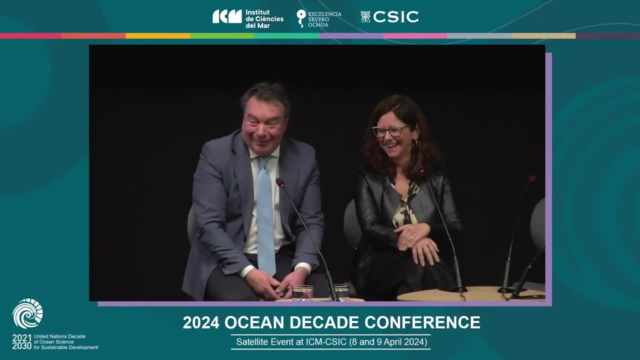 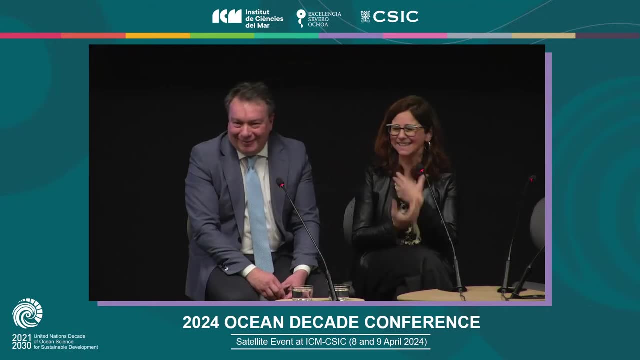 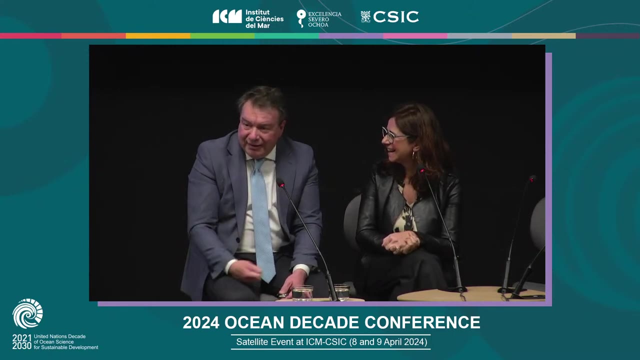 Però ridete, mi avete capito. So we know that it's important to speak many languages. and said by me that I only speak Italian. is quite strange, Perché è importante che i bambini di oggi diventino a breve i dirigenti delle nostre città. 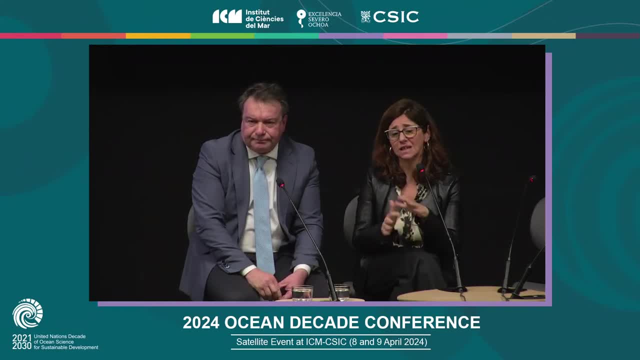 e dei nostri territori, Because it's important that the kids of today. they will become the managers and the policy makers of our cities in the future. Chi è cresciuto con la mia età, con l'obiettivo dell'economia e dello sviluppo dei territori? 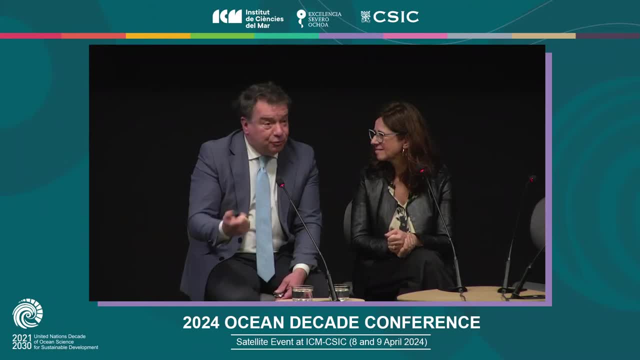 ha portato tante cose buone, ma abbiamo anche sporcato molto. People of my generation were. you know we were raised in thinking more about economic development, so we brought some good economic development, but we also brought some problems and environmental issues. 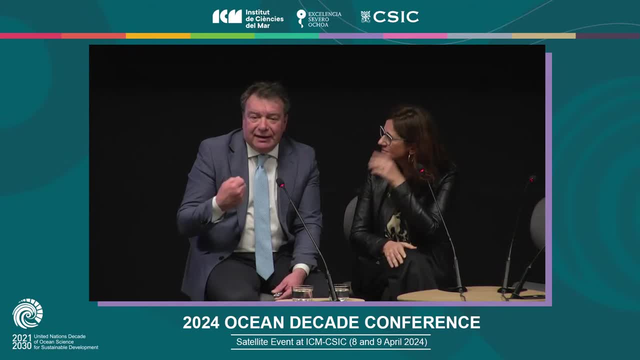 E' importante che oggi noi riusciamo a capire che abbiamo anche la responsabilità di pulire e di far crescere delle persone che rispettino un po' più del territorio rispetto a noi, And therefore it's now our responsibility. 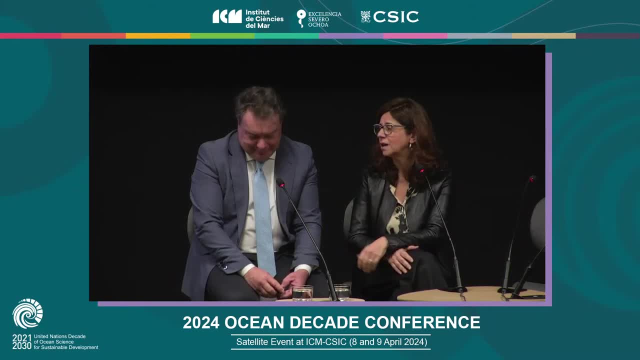 to help the new generations to change the way in which they behave and in the way in which they protect and take care of their environment. Ho promesso che sarei rimasto nei tempi, quindi vi vorrei dirvi tantissime altre cose. 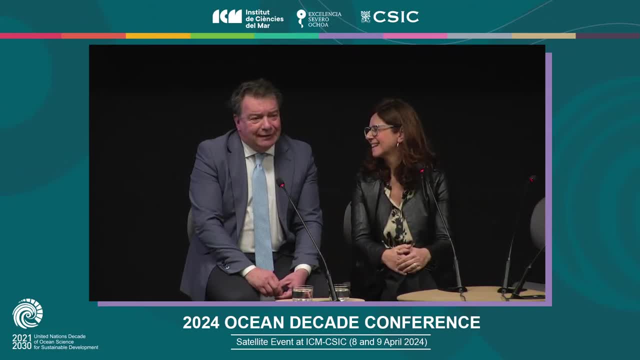 Però il tempo è questo E vi auguro una cosa: di poter venire a trovare la nostra città al più presto, nel più breve tempo possibile. I would like to say many more other things, but I know I have to stay in the minutes that were given to me. 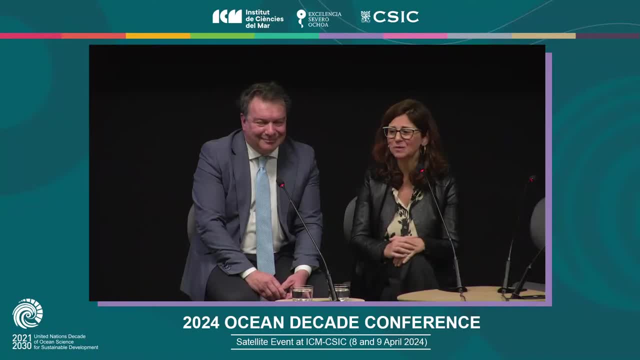 so, to conclude, I just would like to invite you all to come to Venice, and I also add also my invitation to come to Venice and to see the work that we are doing together, especially with this kindergarten of the Lagunis- three to five years old kids. 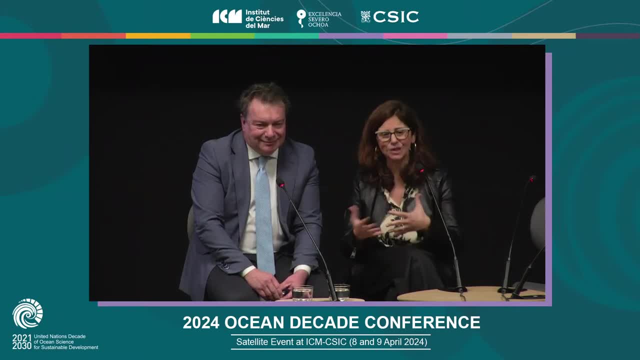 that we bring every Thursday, every Wednesday and Thursday in the nature to learn about their environment and also about their culture and their tradition. Sembra che non abbia capito, ma la seguo. mi ha tradotto di più di quello che dice. 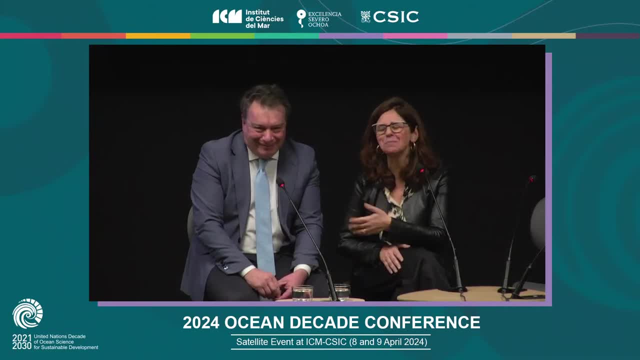 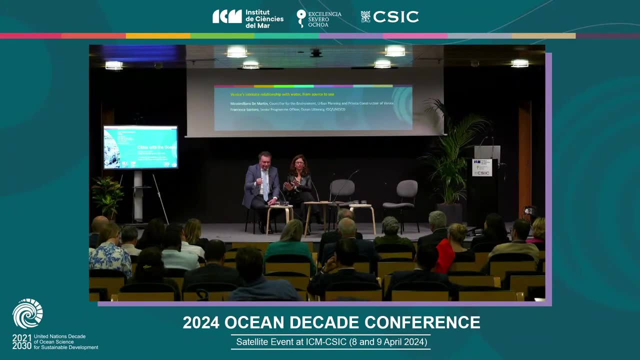 It seems that I don't know what she's saying, but I know she's saying more than I said. Confermo quello che ha detto lei, Però se venite, vi auguro una cosa che potrebbe apparire brutta per come ve l'auguro, ma così non è. 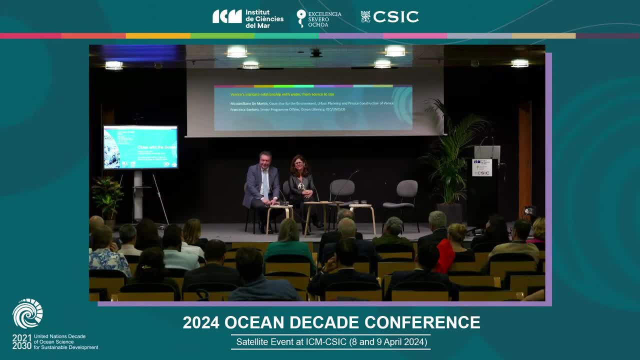 I'm telling you something which might sound strange, but it's not like that. Se venite in città, l'augurio più bello che vi posso fare è perdervi. So the best wish I can tell you, if you come to Venice, is to get lost. 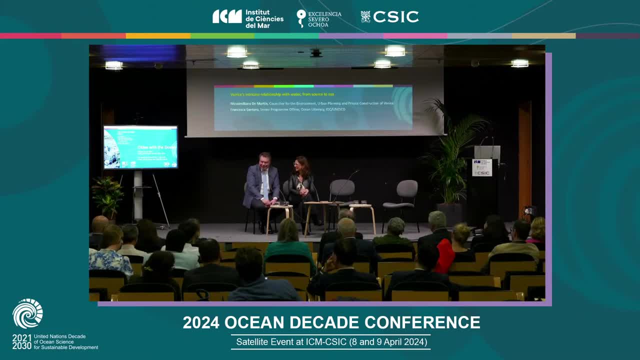 E, se riuscite, tornate nel vostro hotel, nella vostra casa, ma senza GPS, And you need to go back to your hotel apartment that you rented without using your GPS. Scoprirete cose fantastiche che nessuna guida vi farà vedere. 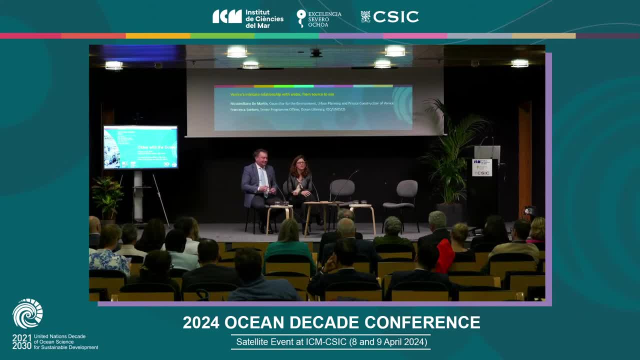 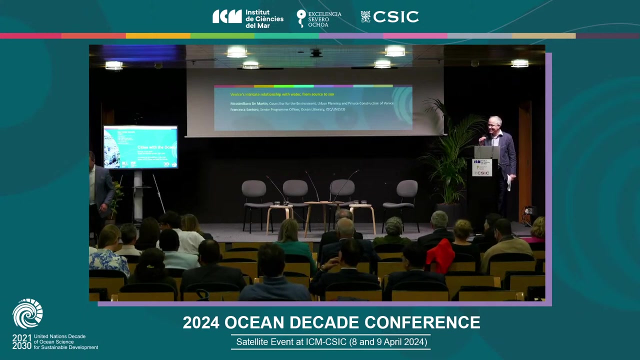 You will find out amazing things: that there is no guide or no book, no GPS that can tell you about Venice. It's territorial marketing. Thank you so much for this great advice And we'll be happy to follow it And now to maybe to build again on this ocean literacy. 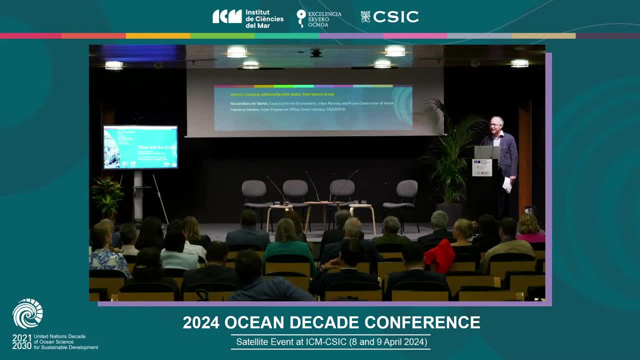 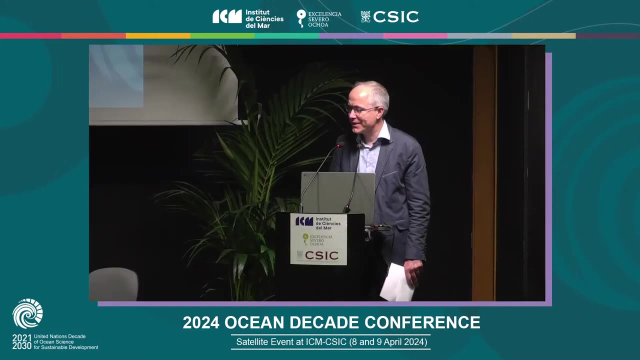 we'll cross the Atlantic to Brazil and hear how Brazilian cities have developed a strong ocean literacy approach to build really the blue cities of the future. There's a slight change and this panel will be moderated by Ronaldo Cristofoletti from the University of Sao Paulo. 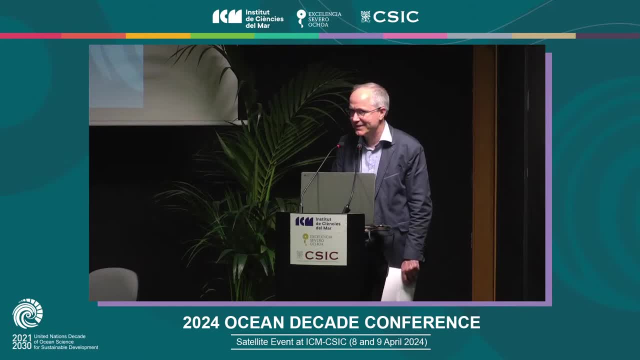 and the Brazilian Ocean Literacy Alliance, with Mrs Ivana Ramos Nascimento and representing the city of Barca Arena, and Axel Greil, the mayor of Niterói, and Carolina Goncalves Pinheiro, from the Brazilian Ministry of Cities. Please 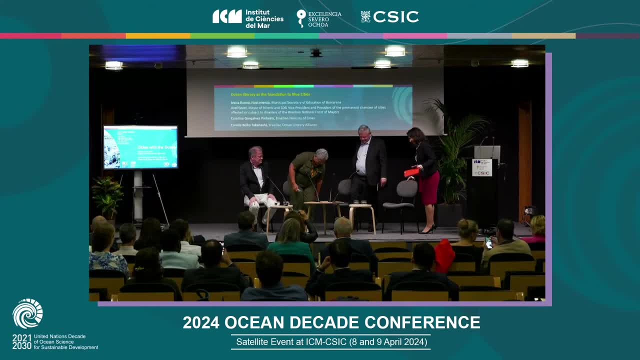 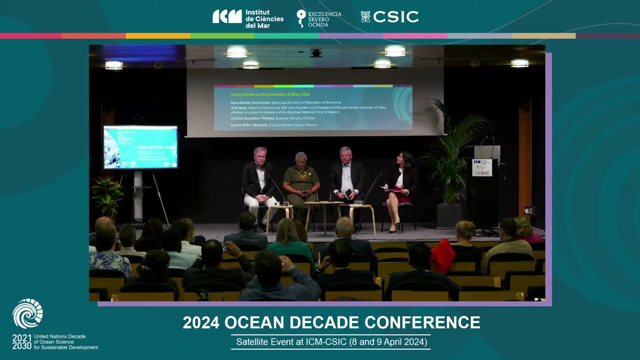 Okay, Hello everyone. So I'm Ronaldo Cristofoletti. I'm replacing Keiko. I'm from the Federal University of Sao Paulo and also the chair of the group of experts in Ocean Literacy for the IOC UNESCO, So it's a huge pleasure to be here with my colleagues. 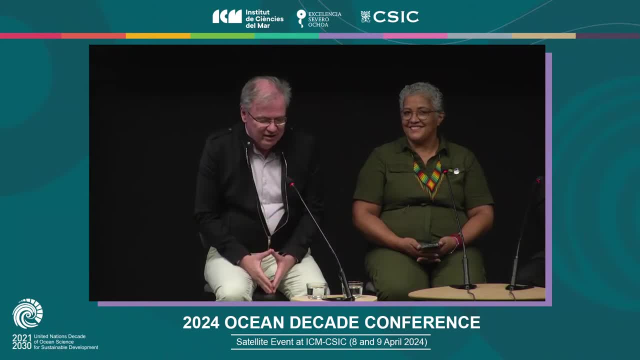 We also will be short, We will split the conversation, But just to let you know where our history come on this in Brazil, So, with the beginning of the ocean decade- and understand that while all the decisions are taking globally, it's locally and at the cities that everything happens. 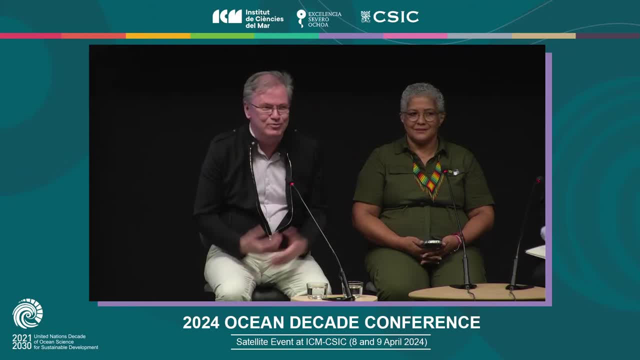 So that's why the importance of the City of the Ocean platform- Congratulations, Olivier and all the team in IOC We have created- and also understanding that for governments- most of them they do not really understand sometimes their relationship with the ocean. 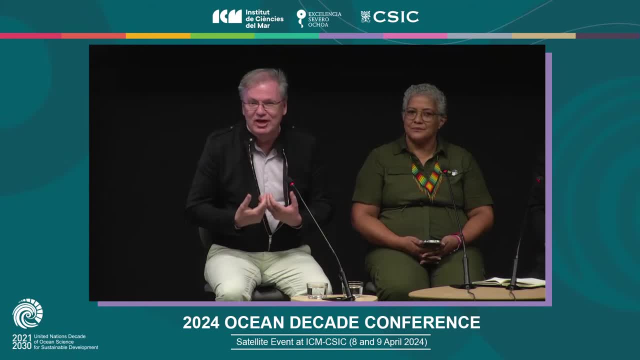 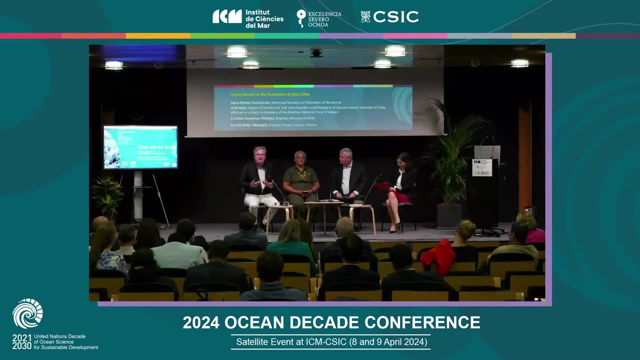 But they have the power in their hands. So that is the basis of the Ocean Literacy. So we created the Brazilian Ocean Literacy Alliance. This alliance links governments from municipalities, states and private sectors, especially ports, for them to understand what is their role. 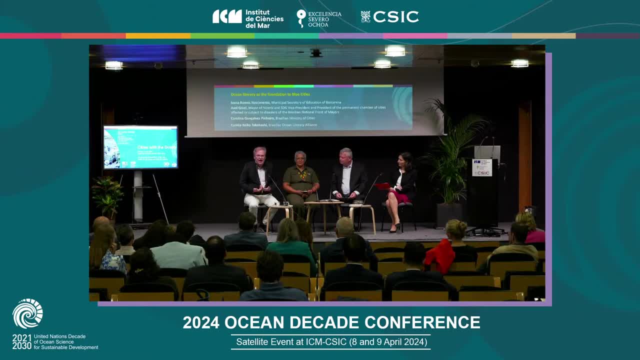 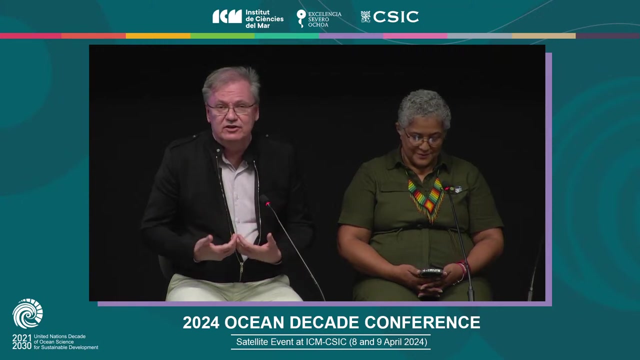 for ocean sustainability. It was created in 2021. And we have had some steps of that. that led, for example, for Brazil having, at the moment, 19 laws for ocean literacy for schools in 19 cities and three states, But also last year in COP. 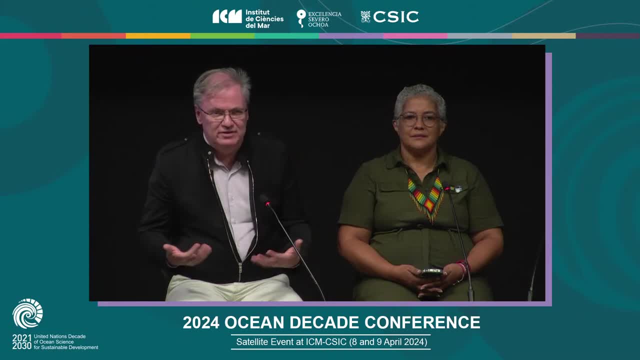 we launched the Building Blue Cities document. There was document to support different secretaries within a city. What could they do for sustainability? And here we have a few examples of this. considering our scale of our country as the size of Brazil that has more than 5,500 cities in the country. 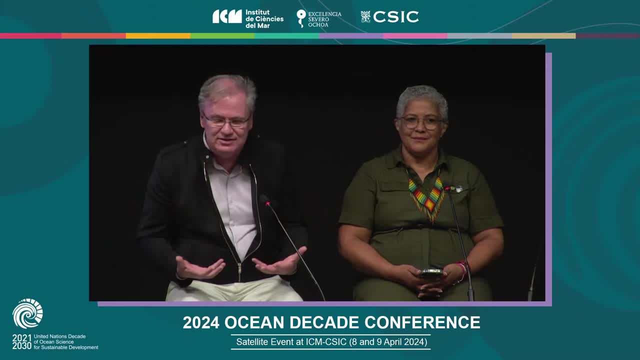 So how can we lead with that diversity? So, to start that, we go for the Amazon. So I invite the secretary, Ivana Ramos Nascimento. and just for you to understand, Barca Arena is a city that is next to Belém. 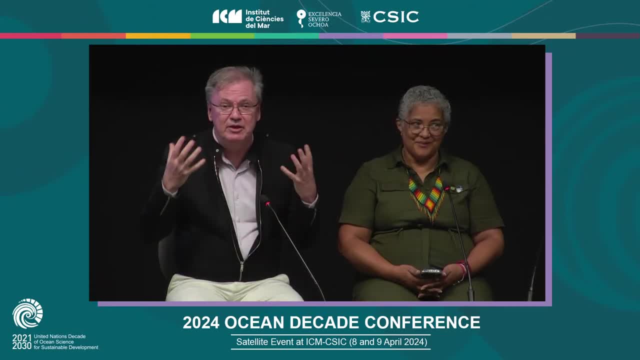 where COP 30 will happen next year. So it's in the Pará states and it's in the forest, And that would be a nice story because, although they have a port, at some moment they did not understand they were related to the ocean. 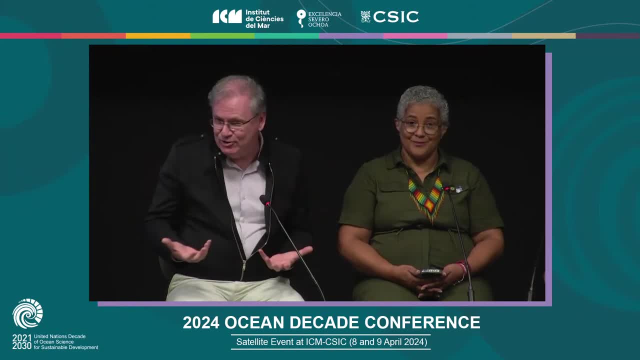 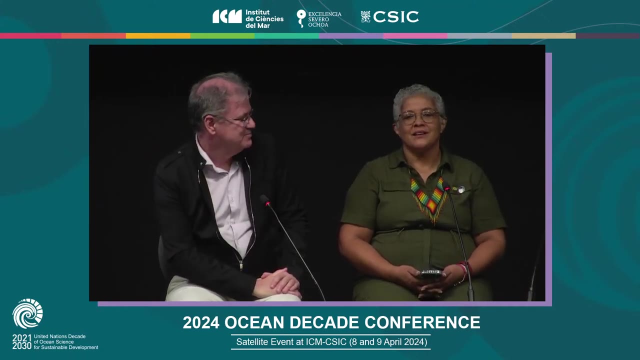 because they are in the Amazon River and they are in the forest. So I used ask the secretary- and I also will work as interpreter here- for her to bring her experience Secretary please. So she said that. hello everyone. 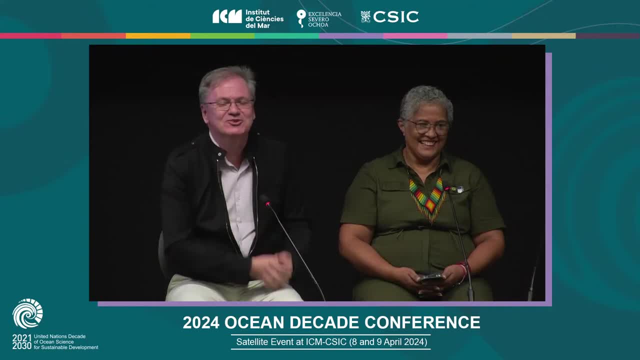 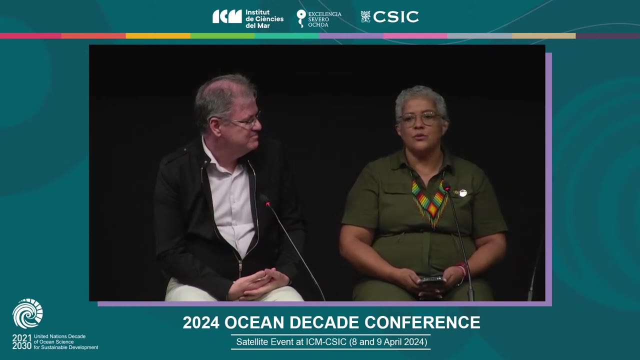 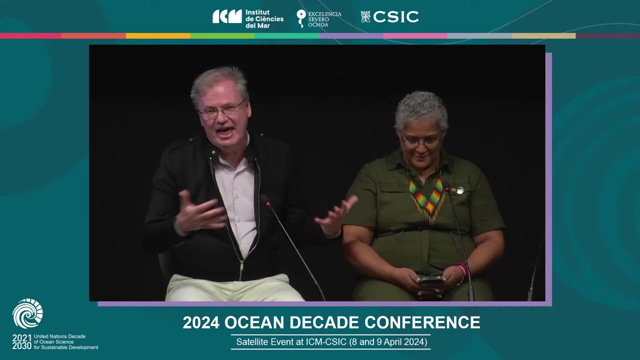 She doesn't speak English as Maximiliano, but she understood by what I was saying that she's the woman from the forest. So Barca Arena. she's from Barca Arena, the city that is in the estuarine zone. 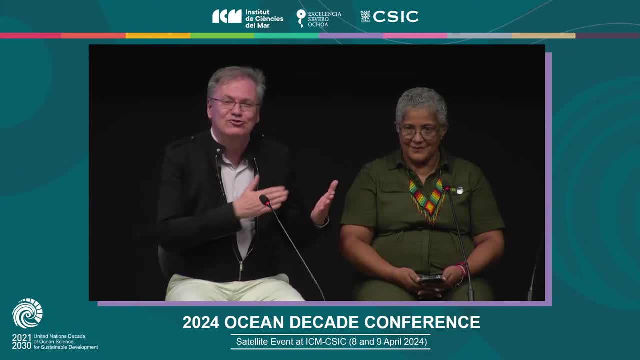 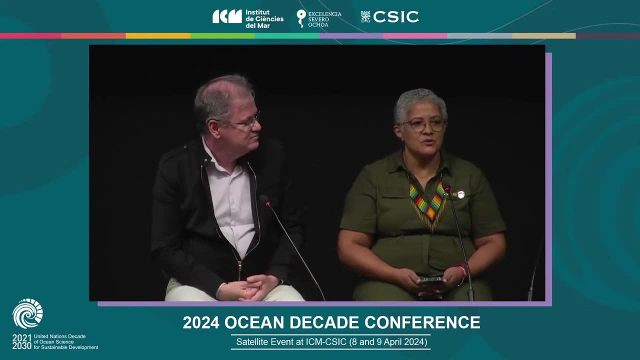 considering the estuary of Amazon. okay, so it's very large. So, in the transition from the Amazon River to the ocean, Before that, we are susceptible to the change in the sea level, And before that, Barca Arena also decided to sign several. 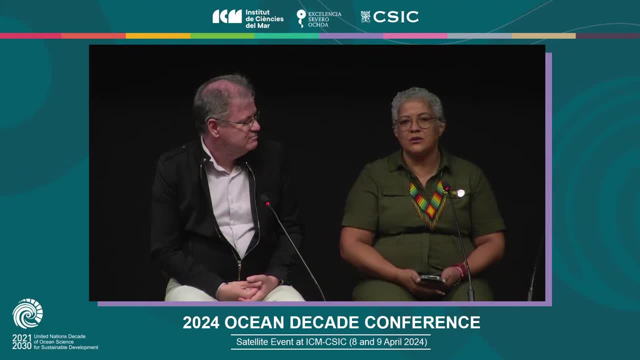 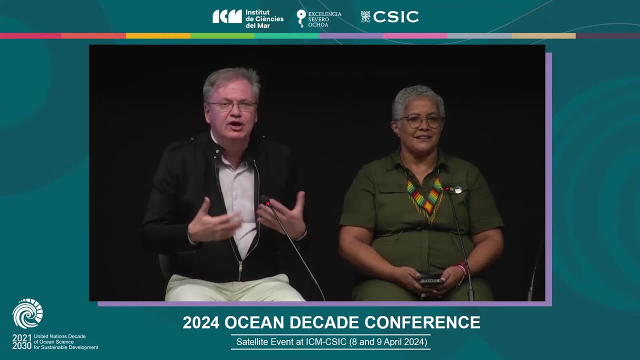 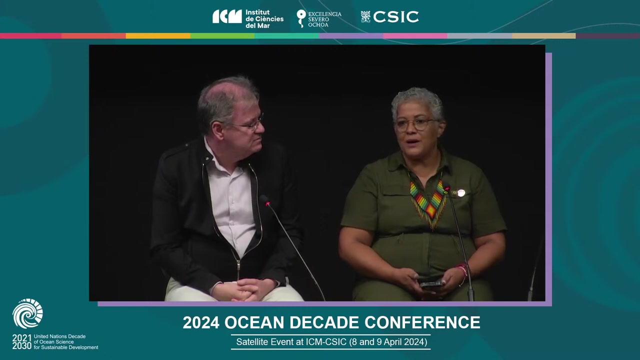 global themes as a governance purpose, So doing to be in this transition zone. they are affected by a lot of impacts from climate change, and so they have been accepting to sign many agreements globally for sustainability and climate resilience. To have one idea from where she comes: 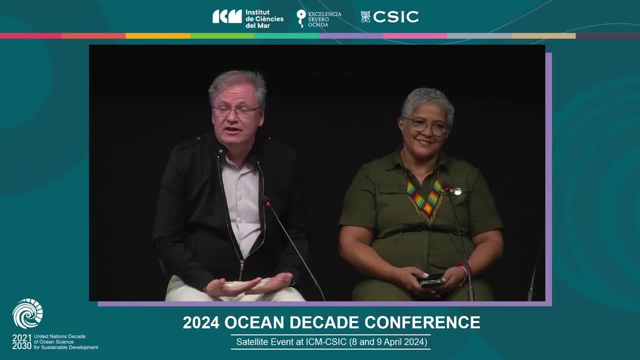 the city, the population in the city. their ocean is brown. The ocean that we use in our photos- multi-color green, blue- they only see in photos, because where she lives it's brown. So when the UN Ocean Decade was launched, 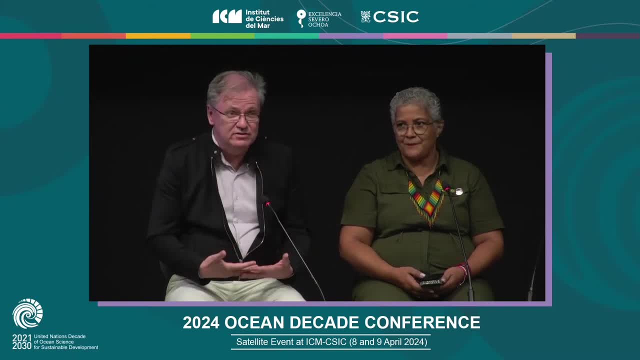 the government understand the importance for bringing the ocean, and so the secretary of education assumed the position to bring the ocean literacy for the society. With that we started to discuss oceanic culture in an Amazonian context, different from what oceanic culture is. 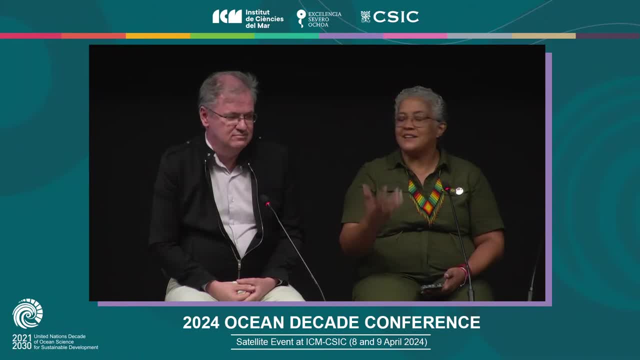 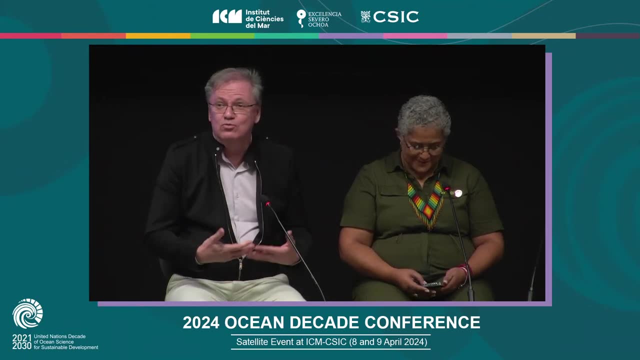 in the global context And we 100% joined our network to the blue school project. So, based on that, they started to work: ocean literacy in their reality, the Amazon reality, the Amazon River reality, And as first step- and here I'll make an addition from me- 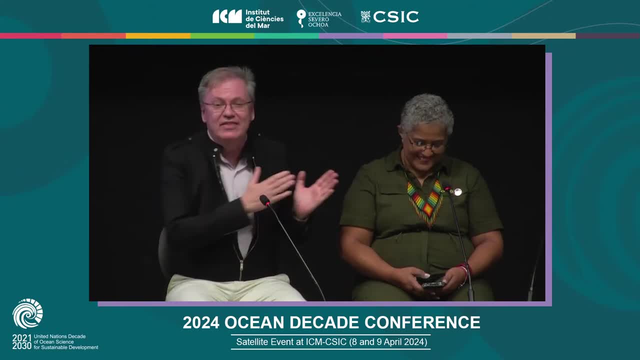 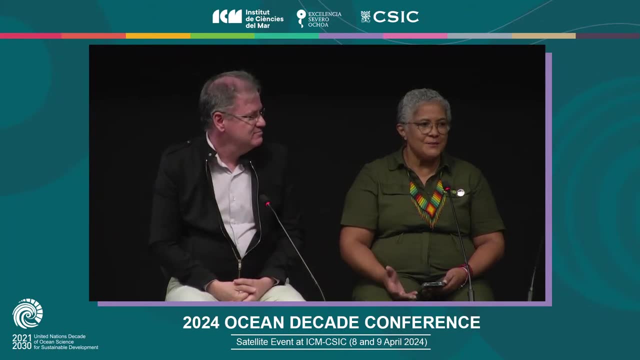 was the first city in Brazil, and actually in the world, that added 100% of their schools in the blue school's network. So in that, they are working to bring together concepts like oceanic culture, resilience and responsible citizenship. So in that, 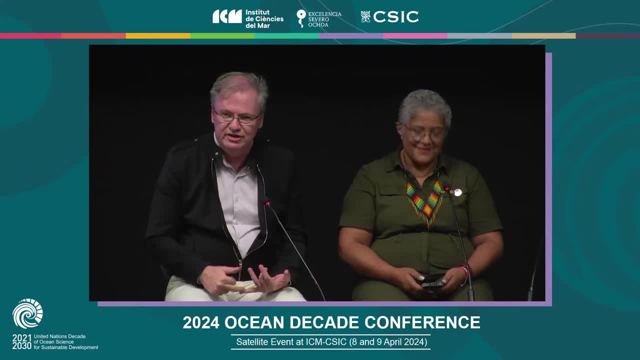 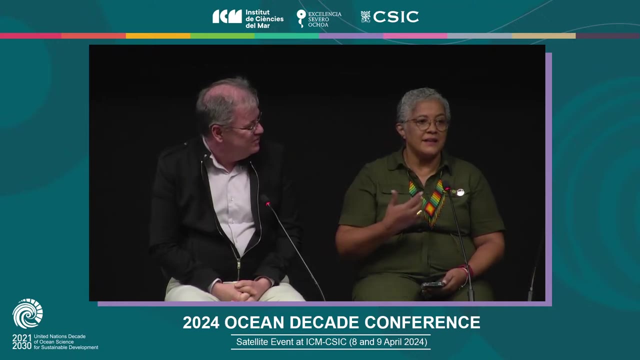 they are working together. ocean literacy, citizenship and climate resilience- Yeah, Sorry. When they started to think about ocean literacy, it was for most of the people talking about mermaids, Nemo or things like that. Hoje, depois de algum tempo, 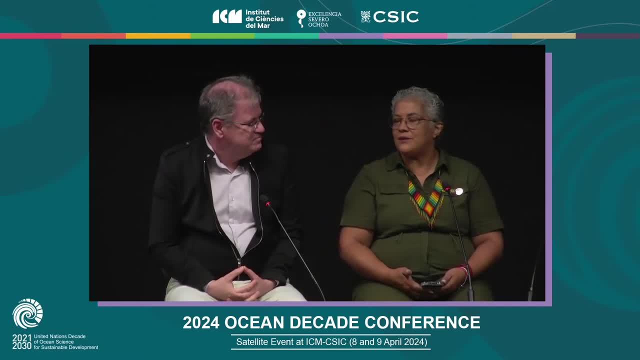 a gente tem a certeza de estar fazendo o trabalho correto. Nowadays, they are sure they are doing the right thing, Porque nossos alunos são capazes de discutir e de entender o conceito e a importância do oceano. 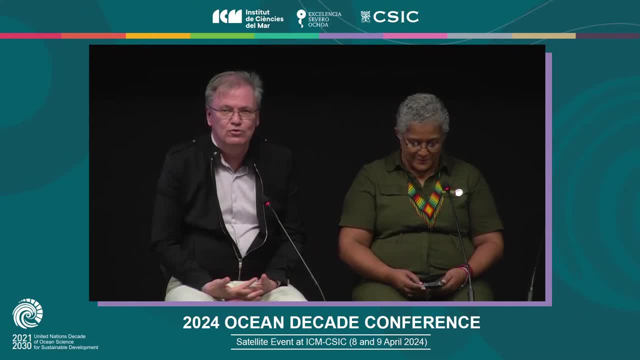 nas nossas vidas, Because now the students in their schools are able to understand and discuss the importance of the ocean in their reality. Somos uma pequena estrela no norte do Brasil, na Amazônia, Mas acreditamos que através 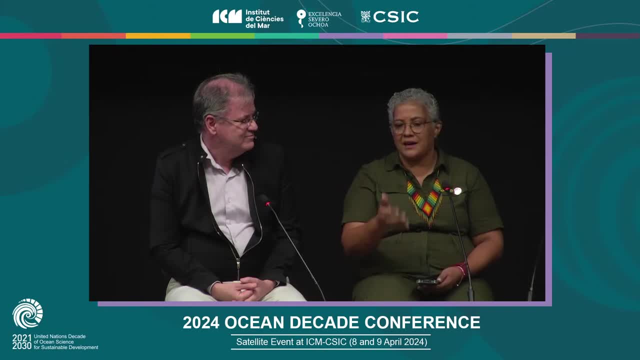 do cooperativismo que chegaremos a essa solução. They are a small star in the heart of the Amazon in the north of Brazil, But they believe that with the collaboration, that they can achieve the change that is needed. E finalmente, 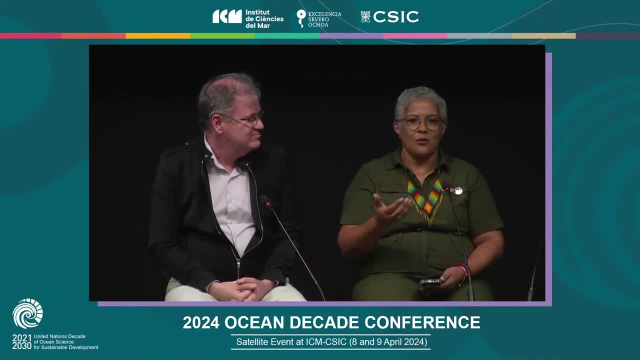 quero agradecer o convite de Olivier do COI UNESCO em participar dessa construção da ideia da plataforma, que nos parece ser de extrema importância para garantir essa aproximação tão necessária entre as cidades costeiras. 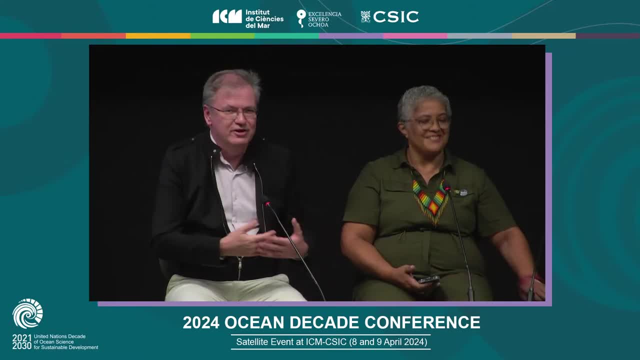 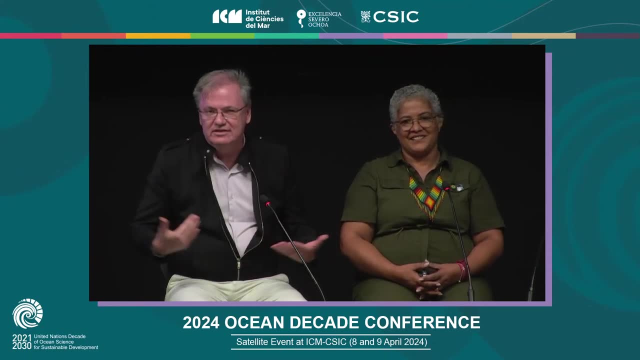 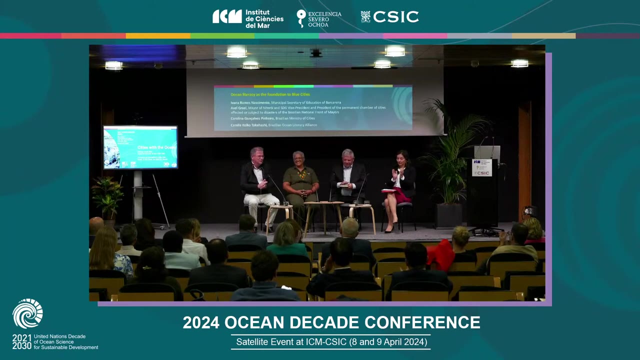 And I would like to acknowledge Olivier, the IOC, for having had the opportunity for Barca Arena, that is part of the scoping group, to help in design this platform from the beginning. Obrigado, Valeu, parabéns. So from there. 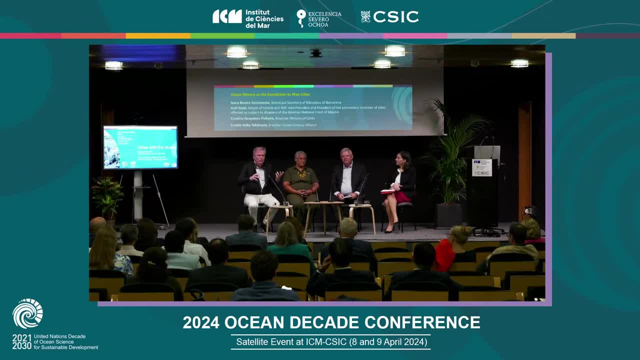 we go from the heart of the Amazon, But then I understand, from the reality of the state of Rio de Janeiro, and especially from Niterói. So we have here the mayor, Axel Graell, And Axel, Well, he's a sailor. 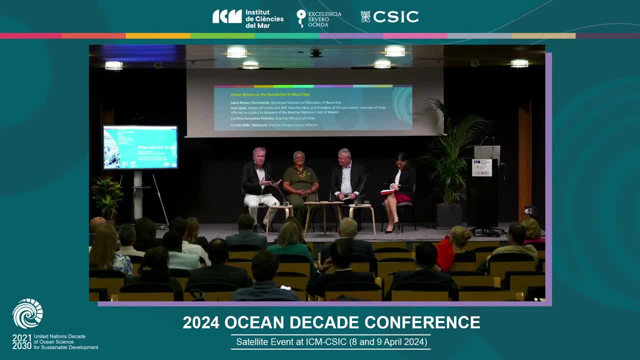 So he comes from a star life with the ocean But, as mayor, one of the most important cities in Brazil, I have to say here is a city- has in there a program for the ocean decade since 2021.. So in the first year they established a program. 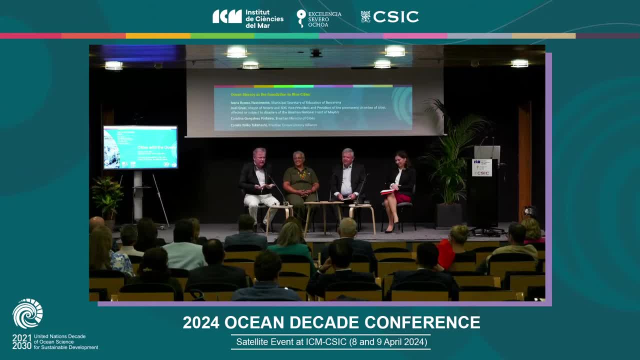 for the decade within the municipality And also he represents here the network of mayors from Brazil. are you saying that in that way? So the five more than 5,000 cities? they have a network of mayors with some working groups. 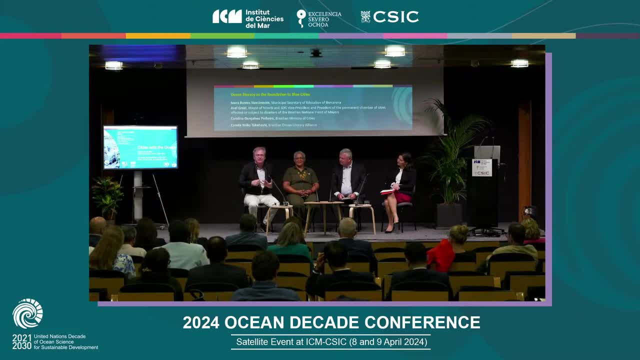 and he leads the working group for SDG and coastal cities, for coastal disasters and resilience. So, Axel, I'd like them to hear from you, based on this experience of establishing or bringing the ocean decade to the municipality agenda, but also if you are viewing this network of mayors. 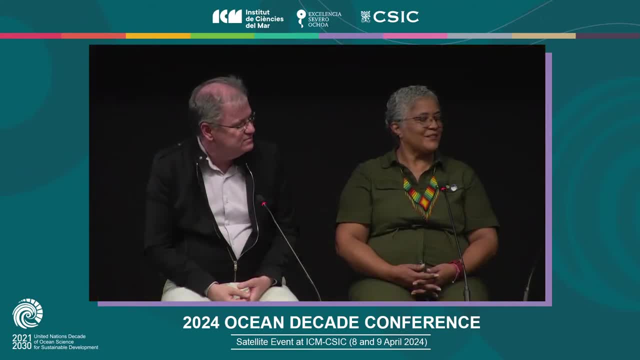 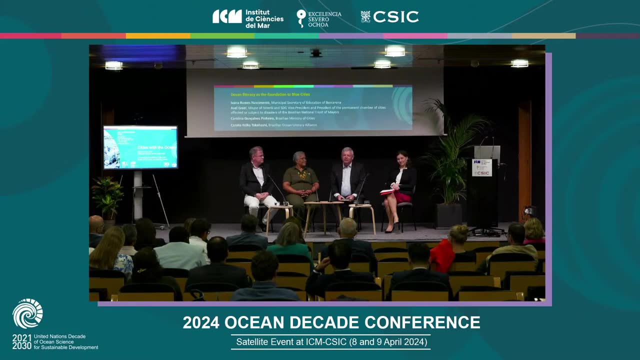 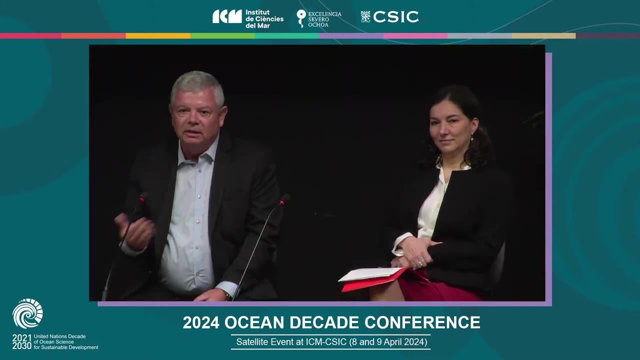 where you see opportunities and challenges for the advances Well, thank you very much. I would like to thank UNESCO for the opportunity to be here And share a little bit about our city with all of you. Niterói is a half a million inhabitants city. For our patterns. it's considered a half size city. We are part of the Rio de Janeiro metropolitan area. The city of Rio de Janeiro is one side of the Guanabara Bay. We are in the other side of the Guanabara Bay. 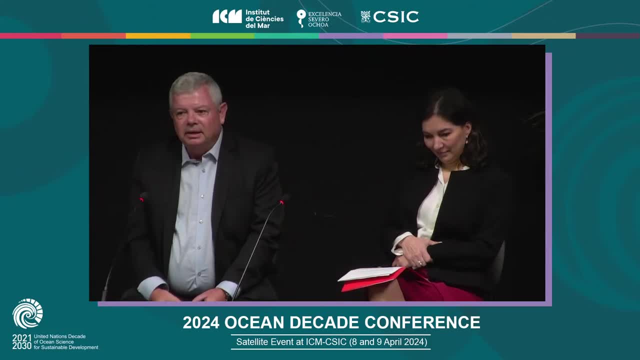 and we're connected by a bridge, And the city of Niterói has a historical connection with the ocean. We are the headquarters of the Brazilian Navy fleet is in Niterói, So we are the most important city for our National Navy. We are the most important city for our National Navy. We are the most important city for our National Navy. We also have the largest shipyards facility in the country. so shipbuilding- One of the first industries in the country- was exactly a shipyard in Niteroi. 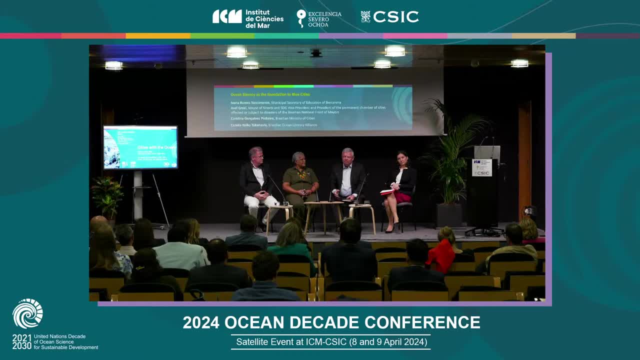 We also have a very strong connection with the water on our everyday life, because 8% of our population goes across on a ferry every day to Rio de Janeiro for work. We also have the largest university in Brazil in number of students. Many of them are from Brazil. 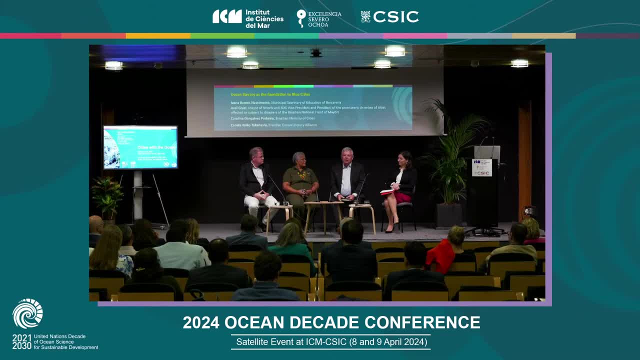 We also have the largest university in Brazil in number of students. Many of the activities are connected to the ocean. We have out in the ocean, in front of the city of Niteroi. we have a large oil production, So 40% of our budget income comes from oil royalties. 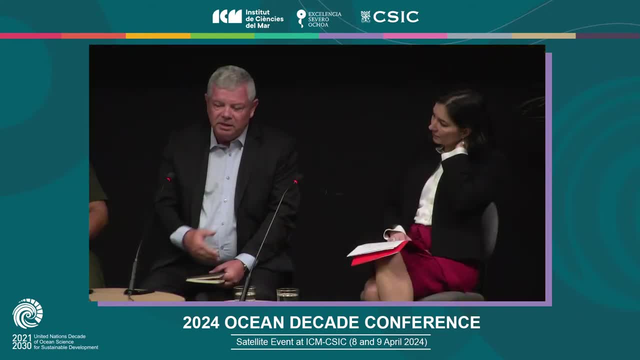 So it's very important in our economy too. So for many reasons we are very connected to the ocean. as Cristofoletti said, we are a city with a long sailing tradition, with ten Olympic medals, We have many connections with the ocean. 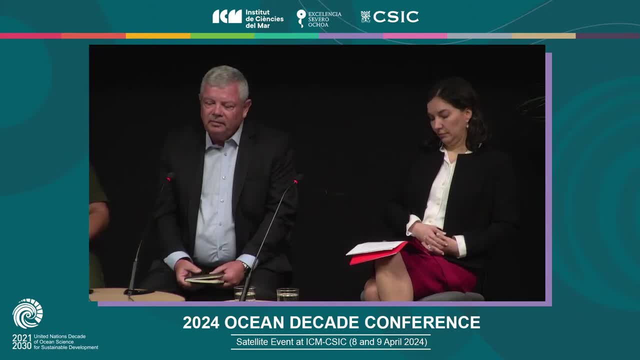 Yeah, we also have the. we have the second largest fishing city in the country. so we decided to connect the ocean- Yeah management, you know, along our shore- into the urban planning of the city. So our city master plan goes beyond our coast and connects the management of the. 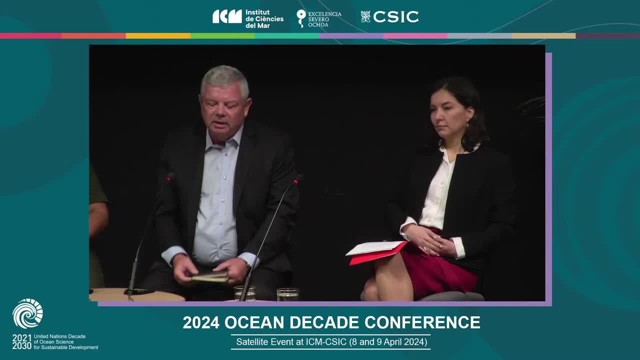 sea ahead of us into our management and into our responsibilities. We – there was an agreement that was made that half of the Guanabara Bay – you know, we divided the Guanabara Bay with the city of Rio de Janeiro, And so most of the ships that are in the Guanabara Bay were all in the Guanabara Bay. 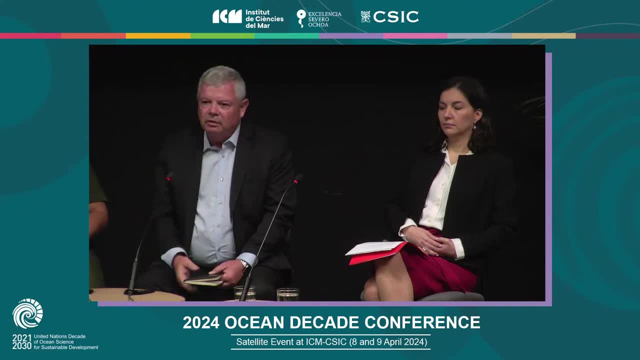 And so most of the ships that are in the Guanabara Bay were all in the Guanabara Bay, there for repair and and for other logistics, before all the taxes were being paid to Rio, and now it's It's, it's shared with, with our 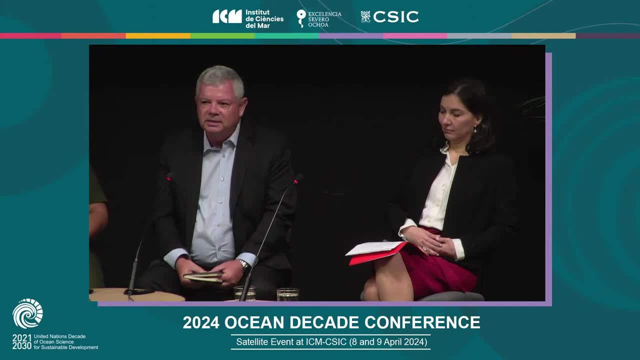 business- offshore built business. so we We also have a protected Area in the ocean, that it was protected by the state government, But it covers a large part of our Coastline and it's important because it protects Traditional fishing activities. so this is also important as 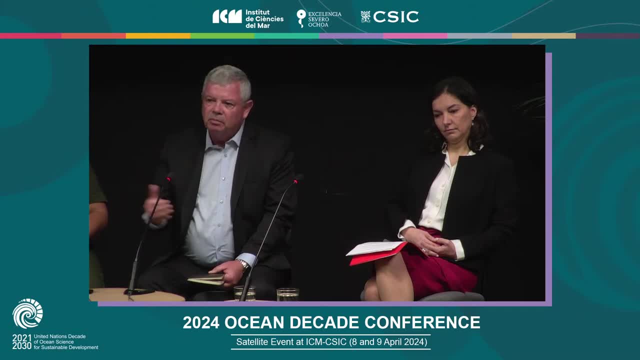 Ship. the ship business is so important to to to Niteroi. We decided to invest with our own funding, on the dredging of the port of Niteroi and that makes Feasible to have a fishing port that was built but was never used because the 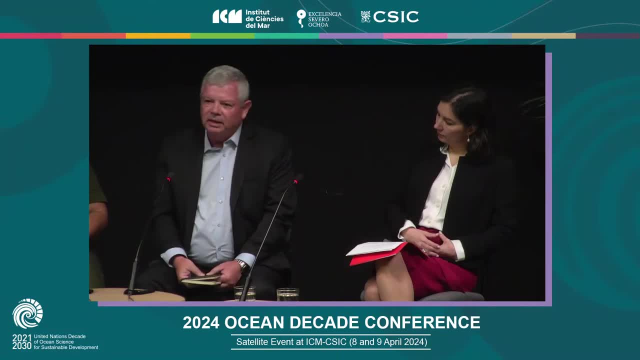 Fishing boats could never reach that place. So now it's going to be running, Which is going to be very important for our economy. So that's basically how we are connected to to the ocean And, Professor Christopher, let it said I'm also the coordinator of this. 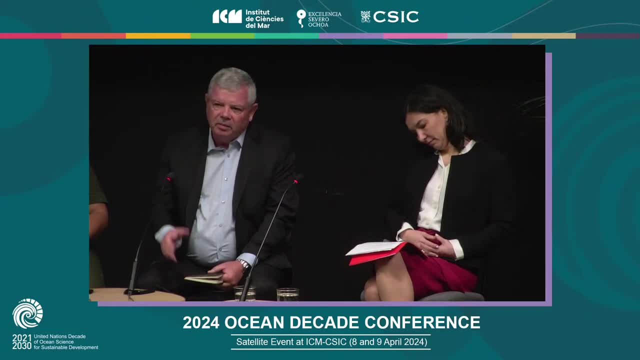 Commission from the, the Brazilian mayor's association related to of cities with with climate threats. so we share experiences and we try to to Lobby for, for new regulations to prevent, like landslides and floods and things like that. it's. It's a very strong issue right now because we've been having 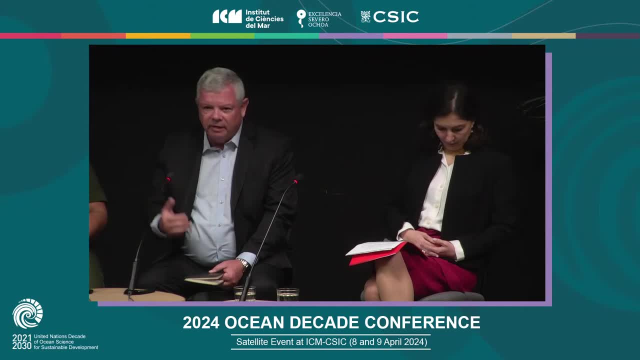 one event after the other, and each event stronger, and Many lives have been lost in in many cities. That happened to the city of Niteroi some years ago. in 2010, we had Heavy rain with a landslide that killed more than 100 people, so this is becoming very 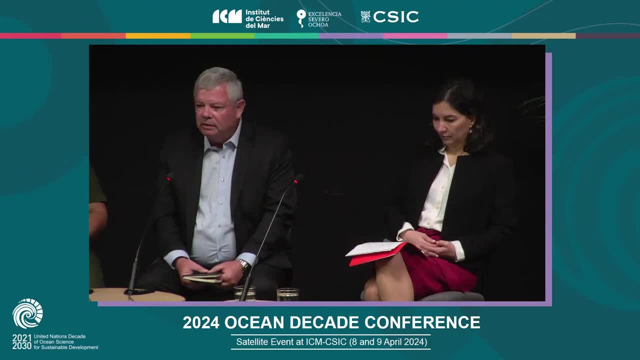 It's a, it's a. it's a big concern, you know, in our country. so This is also what we're doing. So, again, just in short, that that's. that's what I would like to Present you to begin with. so thank you. 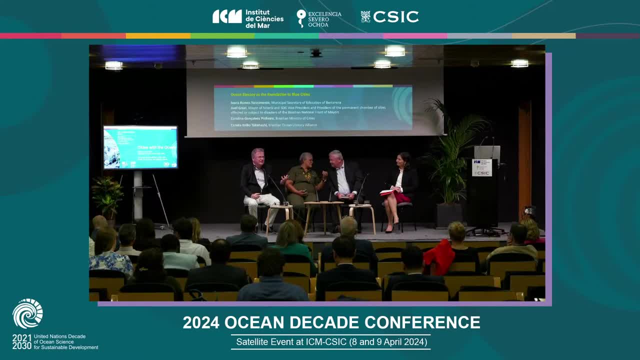 Thank you, Axel, and thanks for bringing us one of his example. as you saw, from the Amazon and and and the other knowledge is, but also seeing almost all the ocean, decades, challenges in his speech, Seen by the view of a mayor and how to lead that and then to finalize this moment. 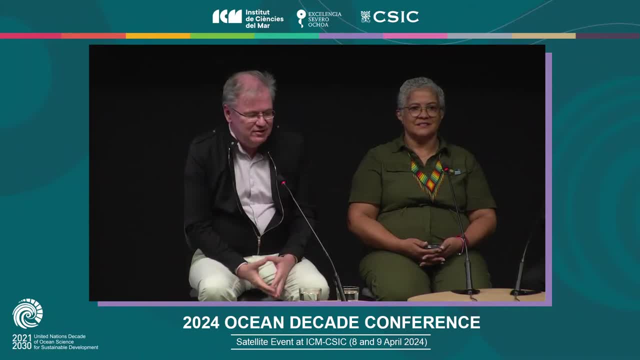 As I mentioned, Brazil was more than five thousand five hundred cities We also have. when we think about linking global to local, of course we need to go through the national, and we have the. We are happy to have a Ministry of Cities in Brazil, and here we have. 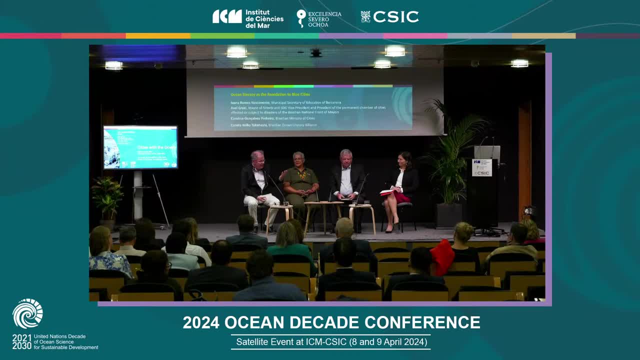 Carolina Piero, representing the Minister of City. So I would ask Carolina to to tell about their job and how they see this link from the global to local In a ministry. Thank you, Carolina. Thank you, I will read, otherwise I won't keep my time and Ronaldo will be mad at me. So 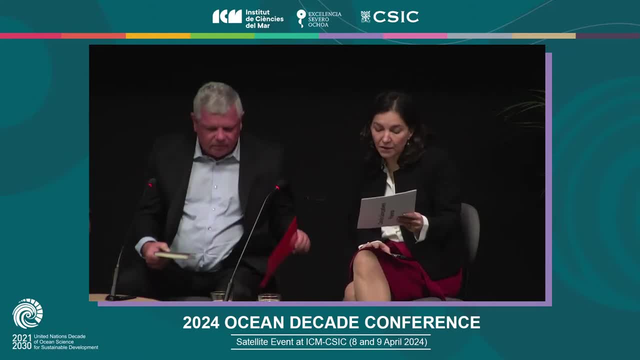 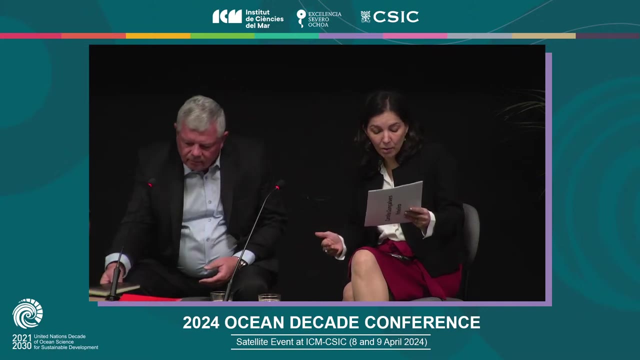 Brazil has reestablished the principles and traditions of our development policy, such as the commitment to dialogue in Multilaterality and the promotion of sustainable development and social social justice. We see in this context the recreation of the Ministry of Cities and the importance of dialogue with local governments. The Ministry of Cities is responsible for public policies on urban development and planification of urban territory housing, urban mobility and environmental sanitation, which in Brazil includes water supply, sewage, urban cleaning and drain rainwater, then drainage and garbage management. Furthermore, specific transverse of urban development actions are included. 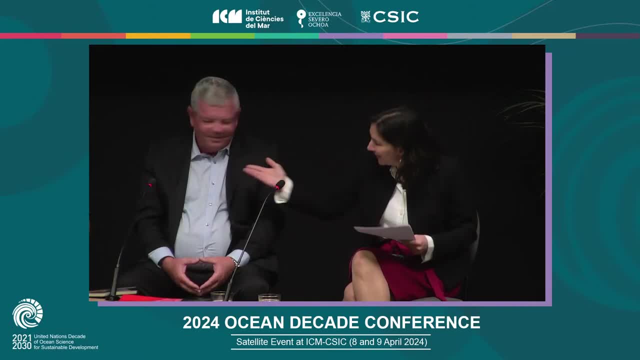 Minister of Cities job their field, who comes from para, Has constantly highlighted that the fight against climate change must begin in cities, Where the majority, the majority of the population lives and where they will withstand the consequences of climate change. statistics in Brazil revealed the gigantic dimensions of urban reality more than 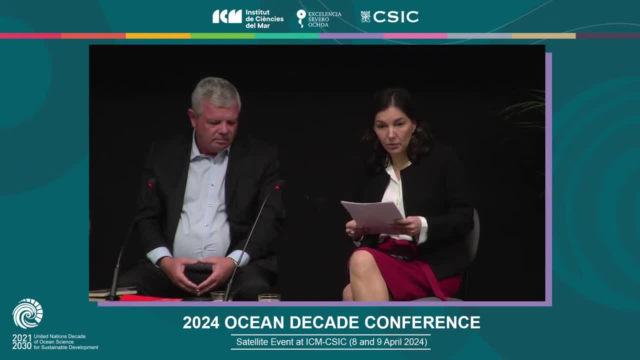 124 million people live in urban areas, which Which highlights the needs to focus efforts on human environment development, including coastal cities. in their peculiarities, all cities face the challenge to build ecologically sustainable approach so as to reinforce the resilience as well as to contribute to environmental preservation. 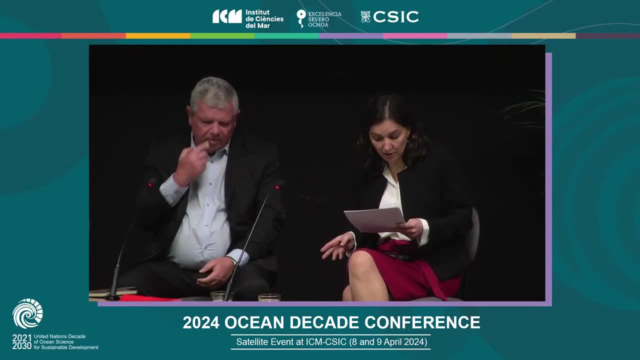 in order to that, To better adapt to climate change. in these contexts, We have the importance of global agendas such as the Alliance, in order to rethink the urban planning of coastal cities and to include the oceanic dimension in the adaptation process of our coastal cities. global agendas such as the ocean decade Alliance and it's ten challenges are: 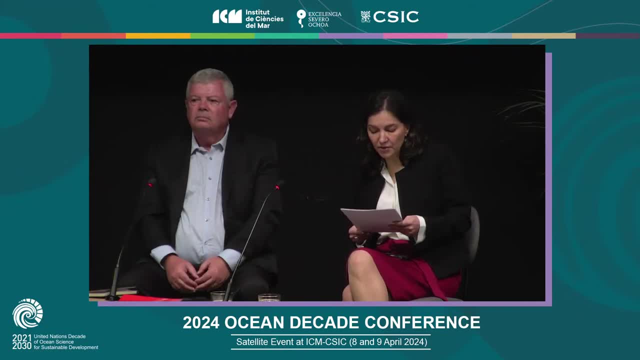 Extremely important, as they discuss challenges with different actors and international experts And plan how to face them. These agendas also highlight challenges to public opinion and place them in the daily routine of our We public managers, Broadly institutionalizing the management of issues related to ocean health, which is, of course, a problem that affects the entire planet. 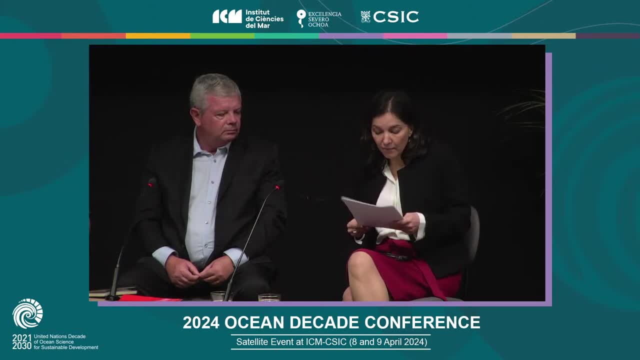 From the Ministry of Cities part, who have been increasingly attentive to these agendas in this, in its in its Structure, the ministry has two transversal national secretariats Working together with local governments on issues directly linked to adaptation in resilience to climate change. the national secretariat for 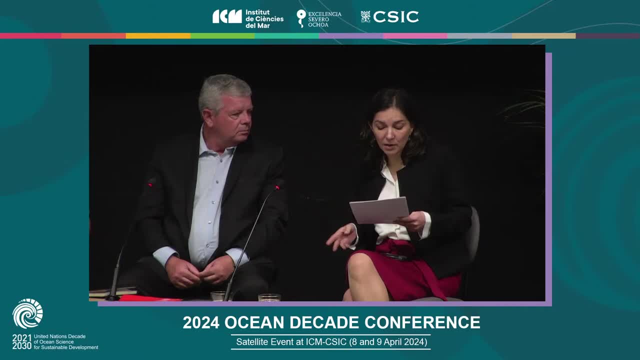 urban and metropolitan development through the Department of Adaptation of cities for climate transition and digital transformation and the National secretariat for peripheries, which is an innovation in Brazil. It's the first time we have a Specific national secretariat for Peripheral areas. It's like slums in Brazil We use this term very fair, which is not. 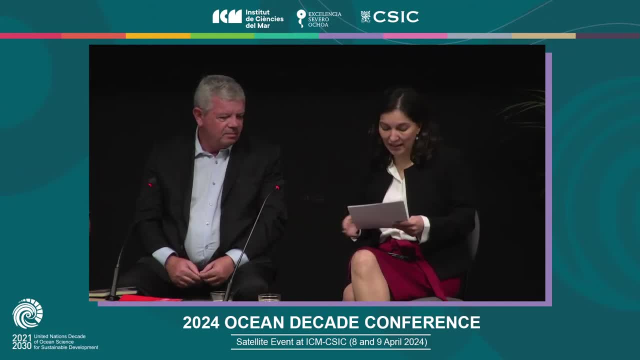 Does not make justice to the what it means in in English. Through the Department of risk mitigation in prevention, Just like the Ministry of Science, Technology and Innovation in the Ministry of Environment, the Ministry of Cities and we at the ministry International Advisory Office, Have been in dialogue with several international partners to bring the oceanic agenda to the ministry and to our policies. 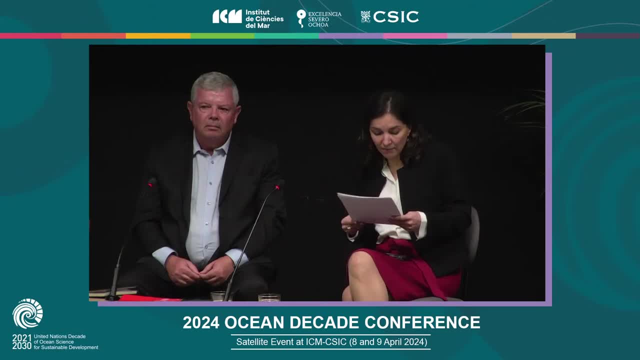 In the several agendas with which with which we have been working, such as breaks subjects me movie, which is the forum of ministers and high authorities of housing and urbanism in Latin America and the Caribbean, Which Brazil presides this year. Minister Jada feel is the president this year. 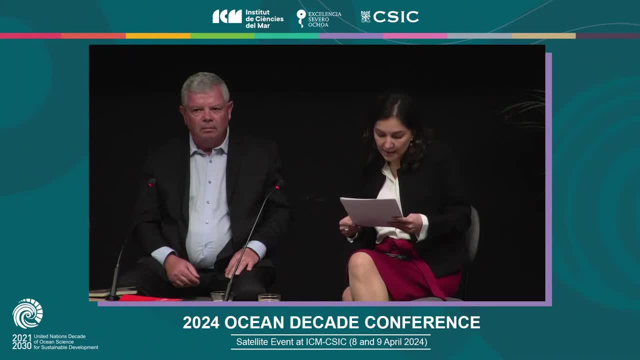 the Amazon cities forum and in the lateral international cooperation with traditional partners. the Environmental agenda is always present. the oceanic agenda is now gain in its space. We cannot do that without dialogue with local governments and with international institutions and experts When we decided to face these challenges. 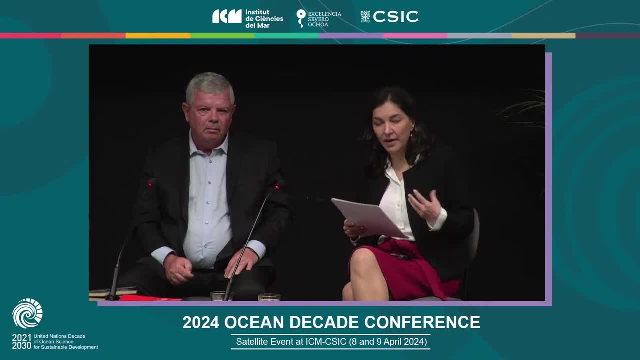 We also have an opportunity to make the country fairer and more Prepared to climate change, and I am going now to borrow and adapt a sentence that is in the UNESCO Constitution, Which is a protagonist of this event here, And I will change it a little bit, since. 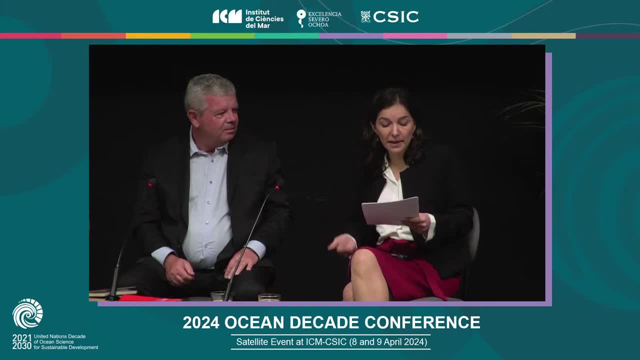 The UNESCO Constitution says, since war to begin in the minds of men and women, It's in the minds of men that the peace must be built. I would like to say, since climate change begins in the mind of men and women And the actions of men and women, it's in their minds that the solution of climate to climate change. 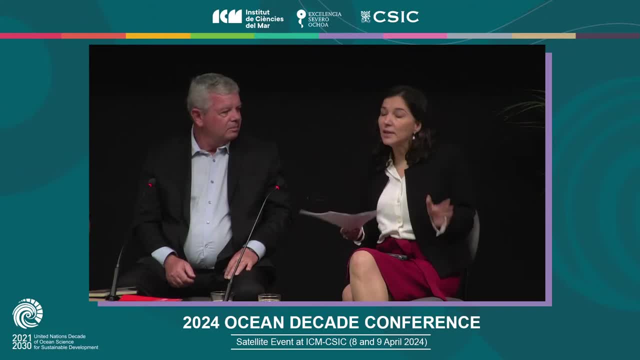 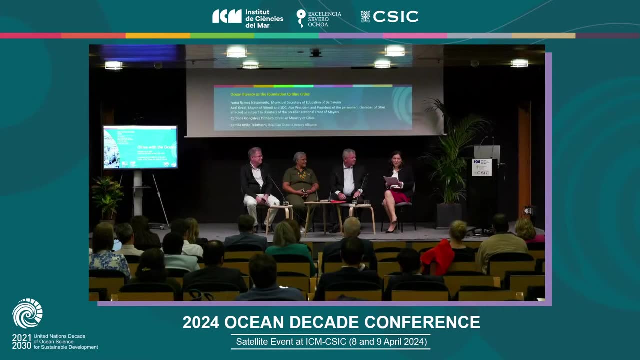 Challenges and must be built, and here we are doing it, We. it's one way of doing it. so thank you very much and we are open to every event like that and to link with local governments and Experts and the academia to work together. Thank You, Carolina, and with that we end this. 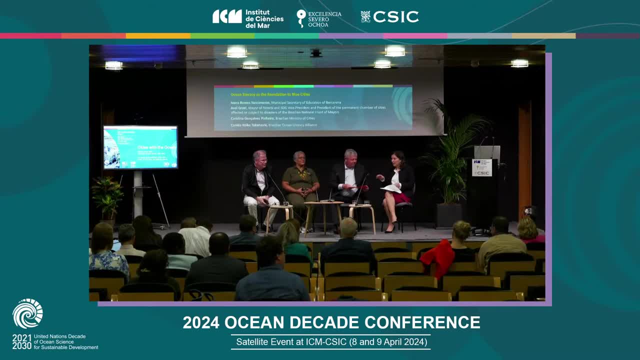 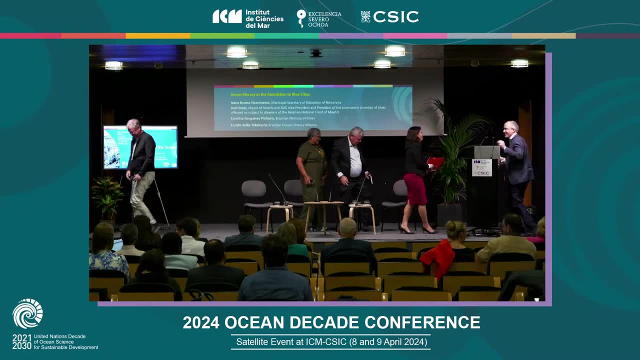 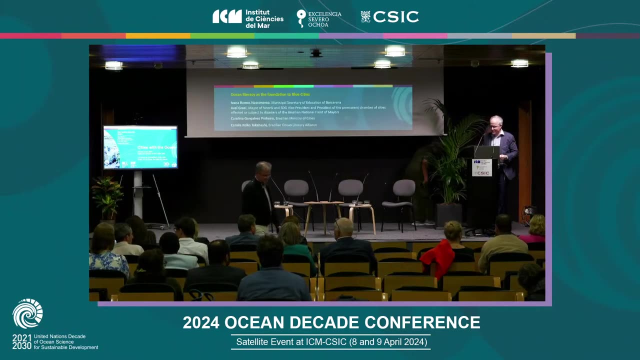 Session and just saying open to discuss with the seats, with the ocean platform as well. Thank you, thank you very much for your contribution and and this, these great synergies across Brazil at at city and national level. I'm afraid we're running quite late now, so 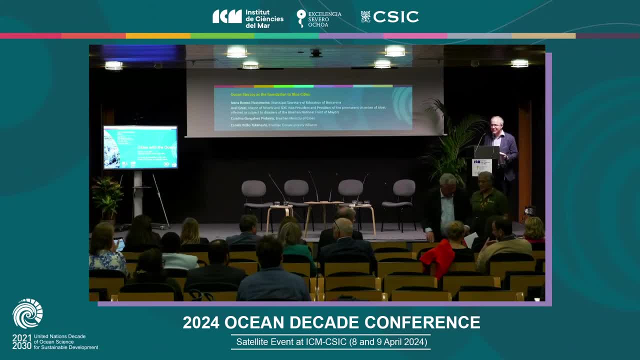 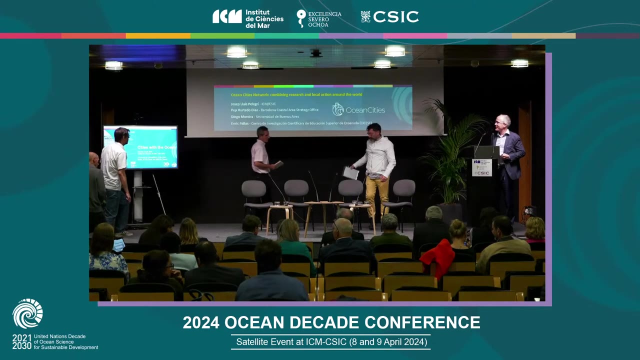 please ask the next speakers to really stick to their time or make it shorter if they want, but please help us finish on time. it's now my pleasure to switch to the Ocean Cities Network, a great initiative that started here at ICM and that will be 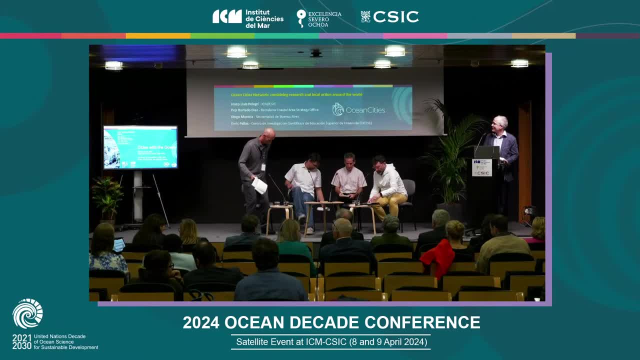 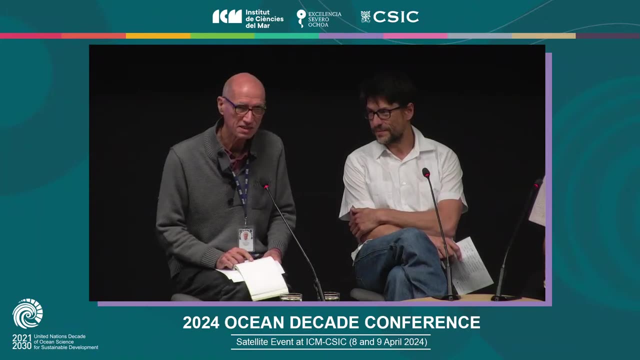 introduced to you by Joseph-Louis Pellegri. please, the floor is yours. Good afternoon. thank you very much, Olivier. well, it's a pleasure having you here and being able to share this initiative that started in June 2021. it's one of the 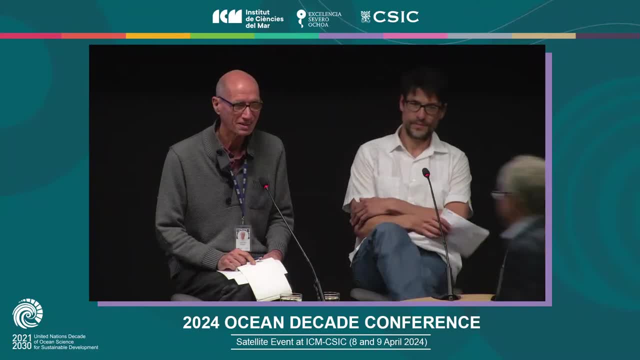 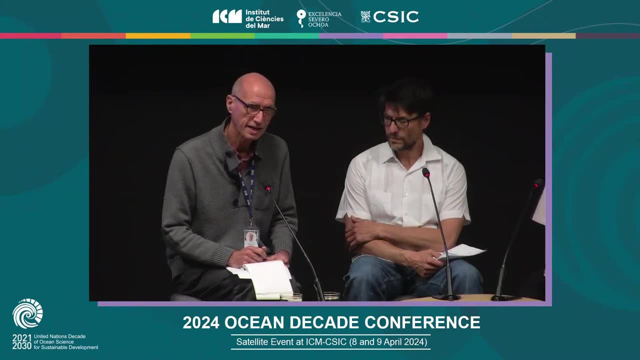 starting programs of the. thank you. it's one of the starting programs for the Ocean Decade, the, the, the, the. the motivation for the Ocean Cities Network is very much aligned of what speakers in the previous table explained. we really feel that any effective change has to come from coastal communities. 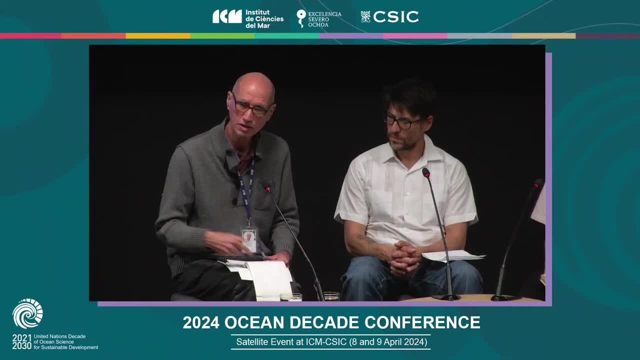 from the communities themselves, particularly from coastal communities that experience and are engaged with the, the urban ocean that is part of a global ocean. so from the very start we felt: ok, this is indeed an opportunity to experience the ocean in a fully integral way and trying to remove all sorts of barriers between a city that is disconnected with the ocean. 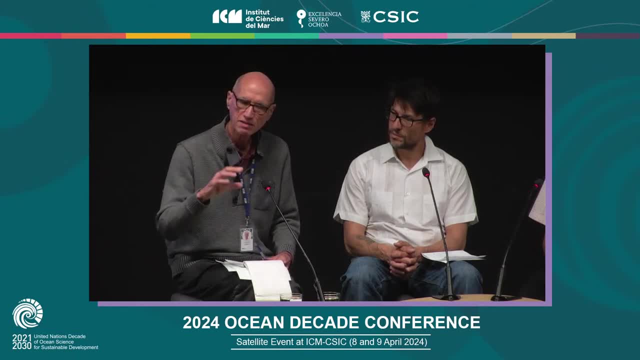 and trying to make this connection not only over the border, but also because of all the connections between cities, between cities and places, between countries and nations. and I'm trying to make this connection not only from the point of view as a global ocean, but as a global ocean and also as a global ocean connection. 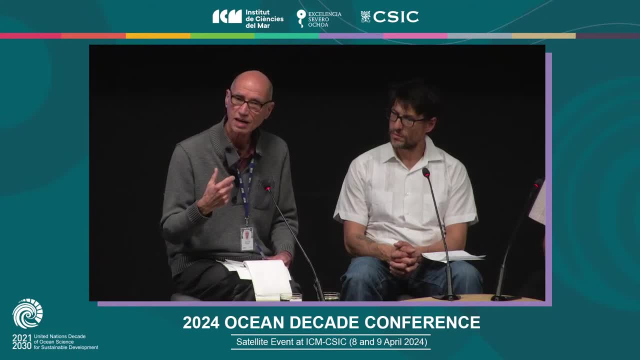 only with our mind, but also with our full possibilities, with our senses, with our intuitions, with our culture, with our traditions, and this is basically what motivated these Ocean Cities. And then the next step is to say, okay, people is who has to make the change, but what we? 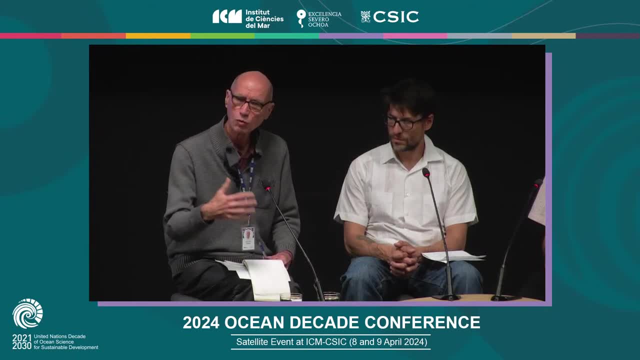 need is to share different vision, different ways of envisaging this connection with the ocean, And this is something that we can do both locally, and this is the starting point. so we have to make all local actors to talk together, to talk among them. so we have here scientists. 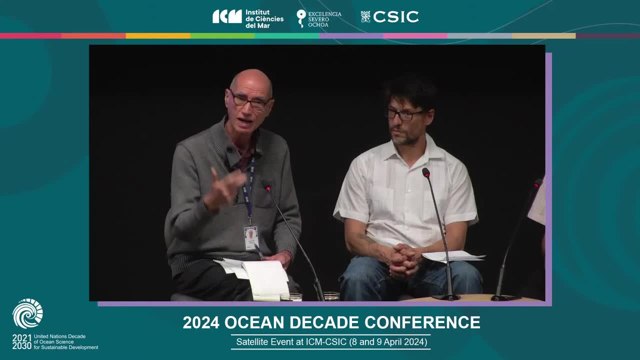 we have here the public administration, we have here stakeholders and we have the society or social actors to talk together and see the different points of view and then grow from these local strategies, these local conversations, this exchange of local perspective into regional, different points of view, how cities or communities from different places in one same region view. 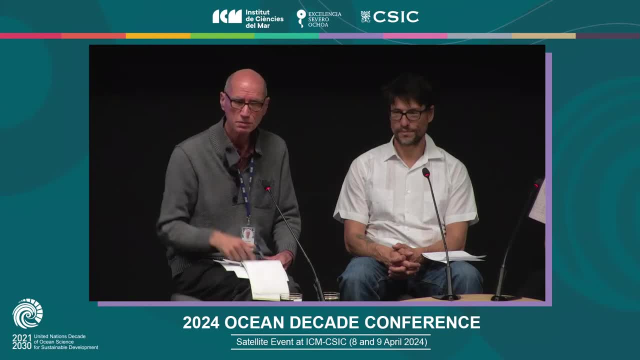 the situation And then sharing these views. So that's to reach globally and that's the motivation and we've been building and right now we have 20 partners belonging to this Ocean Cities Network from all continents, and here we have three coastal communities. 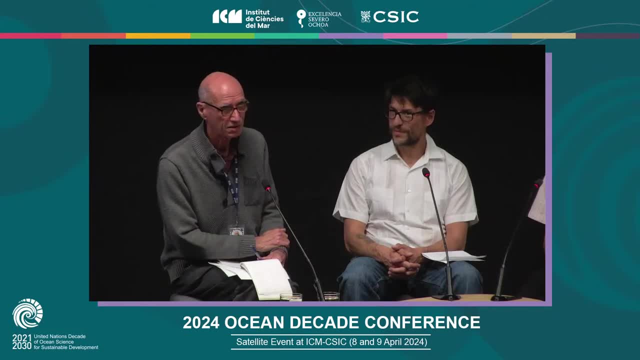 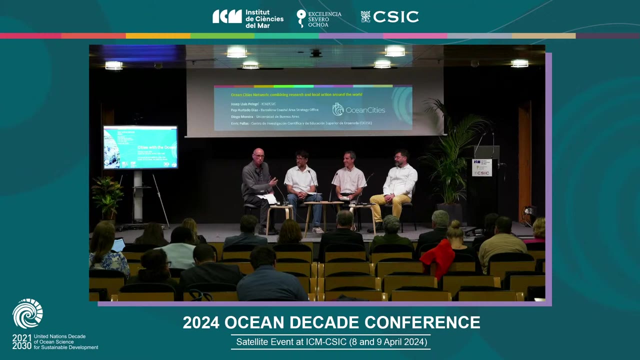 Enric Pallas comes from Ensenada, that's in Mexico, very close to the border of the US. Diego Moreira comes from Buenos Aires and Pep Hurtado is here from the city of Barcelona. I'll let them introduce briefly their institutions and what is their experience with making these. 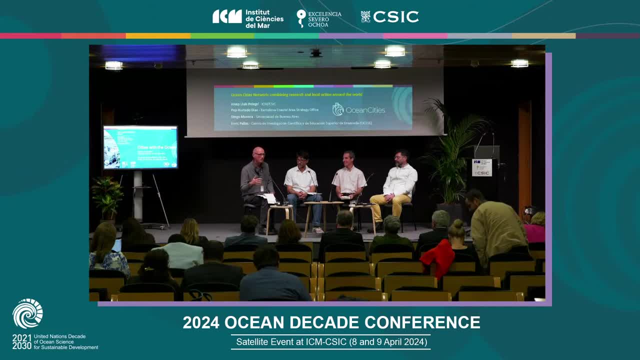 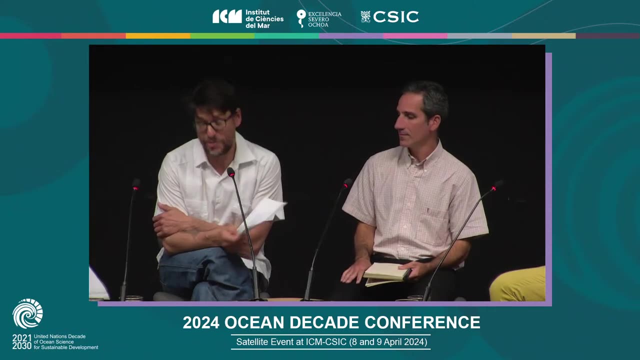 ocean cities. philosophy develop into a local and regional and global strategy. Please Enric yourself, Enric Pallas. Thank you very much, Jose Luis, for having me here and, as he said, I come from representing CICESE. 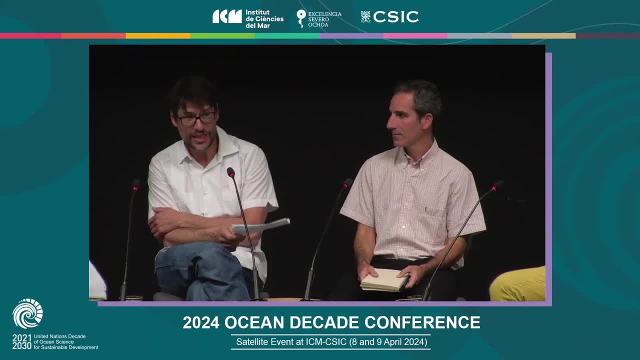 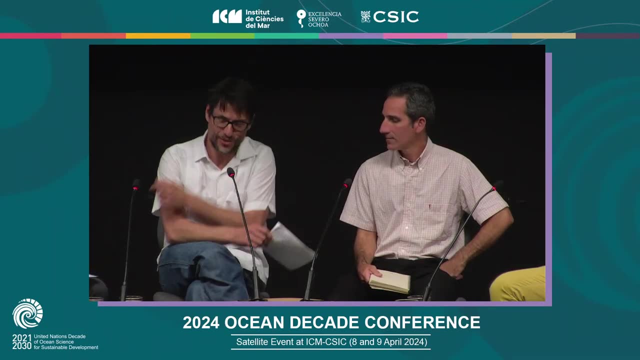 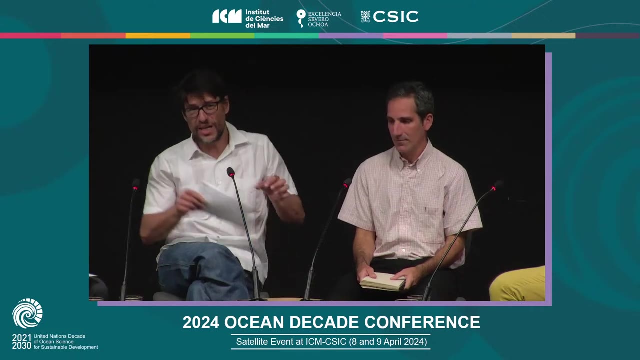 It's a research center in Ensenada, Baja California. This is located 200 miles south of Los Angeles, but we are in the Mexican side, of course, And it's a small city about 400,000 people, more or less, and we are inside a large bay. 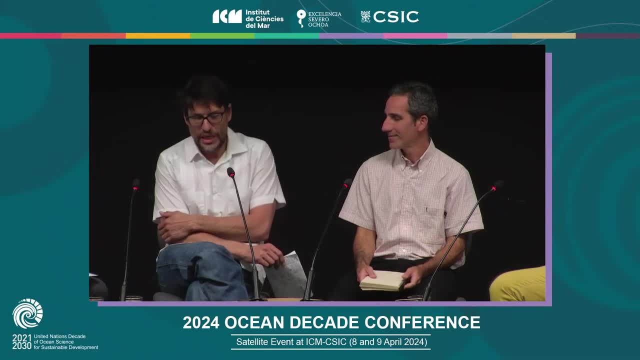 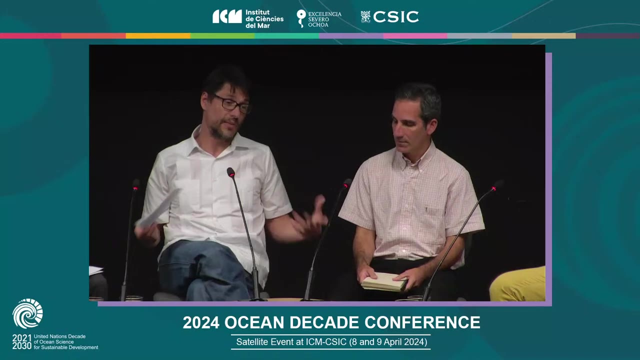 It's called the Bay of Todos Santos. Okay, So we are very happy that Jose Luis invited us, and last year we did many activities trying precisely to engage the population of Ensenada and showing them that they are living in an oceanic environment, because most of the people in Ensenada maybe does. 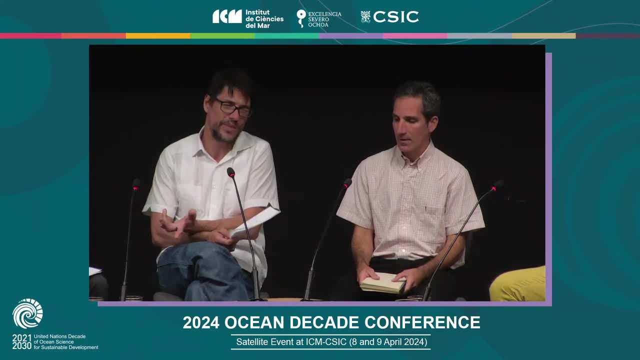 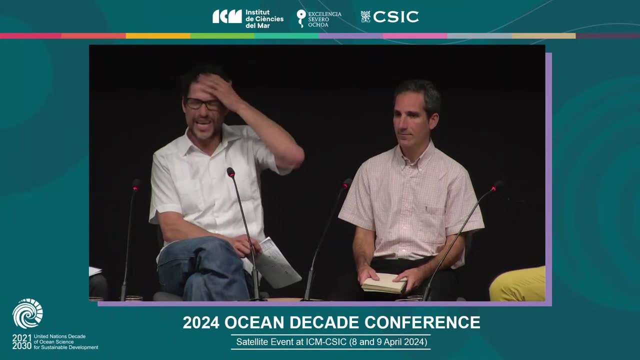 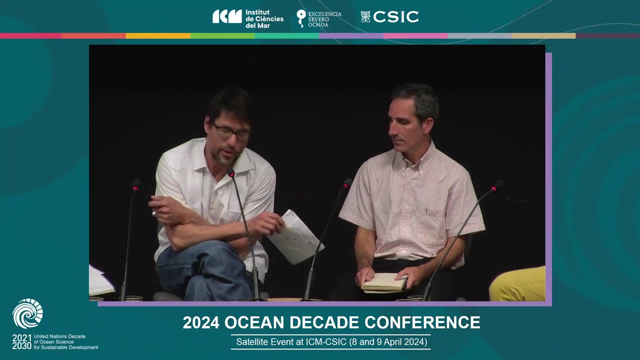 not use that much the ocean, the beach and the coastal environment. So we've been doing since January 2024.. Before we signed an agreement with the local government. I think this was a very nice quick start for all our activities and since then every month we're doing several activities. 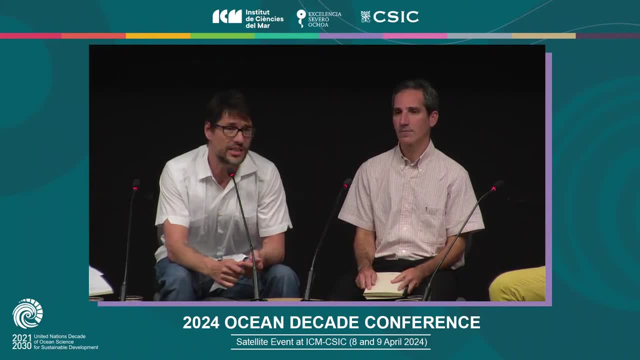 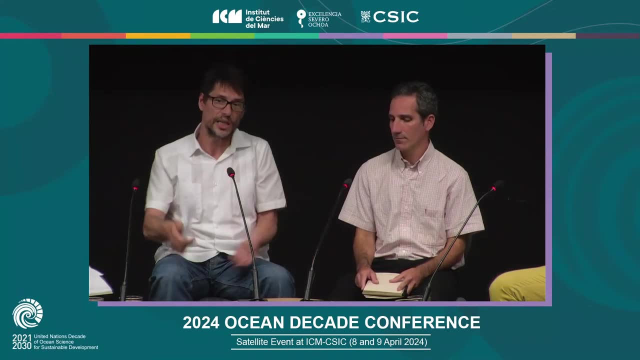 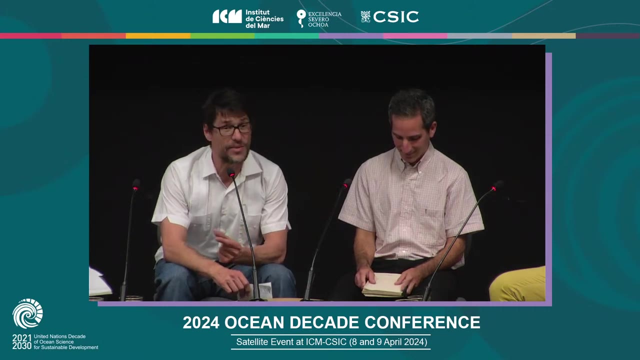 like, from artistic drawing contests to know how the population of Ensenada, what's the view of the population of the ocean? Even we did some food contests. There is a, Okay, There is a very local dish called ceviche, and it's made of raw fish with lemon and chili. 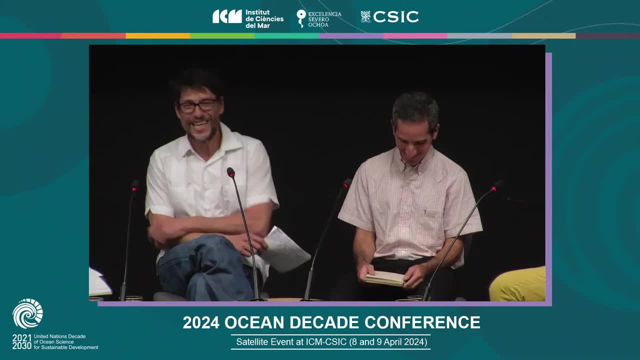 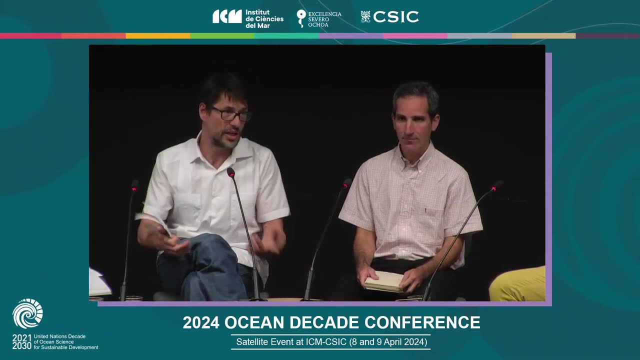 Of course, spicy in Mexico, like the spiciness, and this was a way to show the population how important it is to protect the fish and protect the fauna in the city, because it's a very important cultural dish, this ceviche. 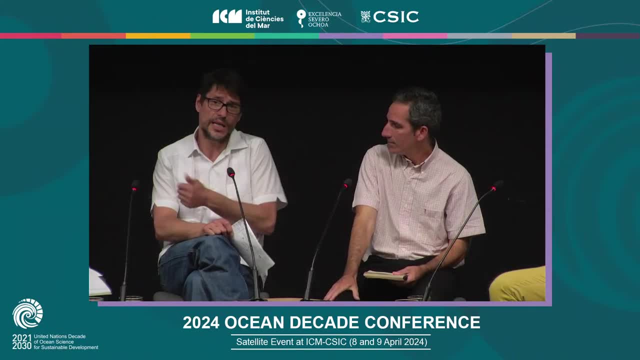 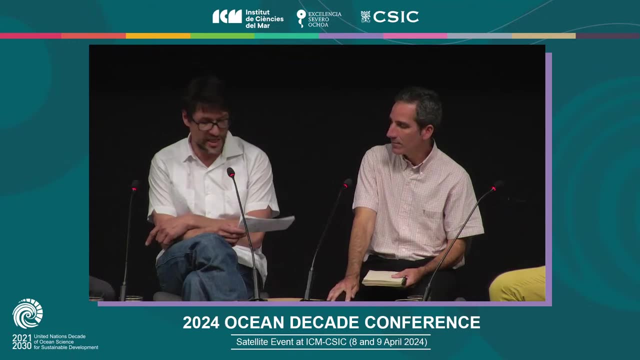 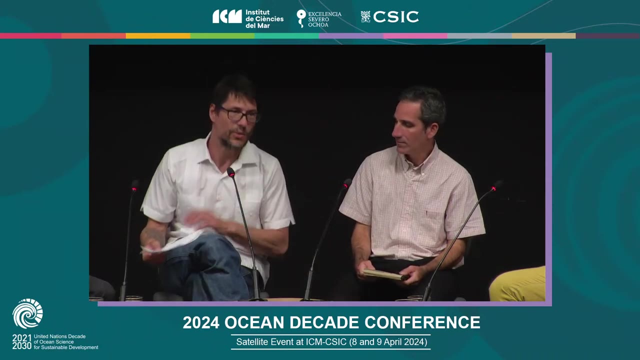 We've been doing a lot of activities of beach monitoring and plastic. We've been doing a lot of activities of beach monitoring and plastic monitoring, engaging the schools, high schools, different communities in the city and in between presentations, to tell the population why it's important to protect the ocean, why it's important to 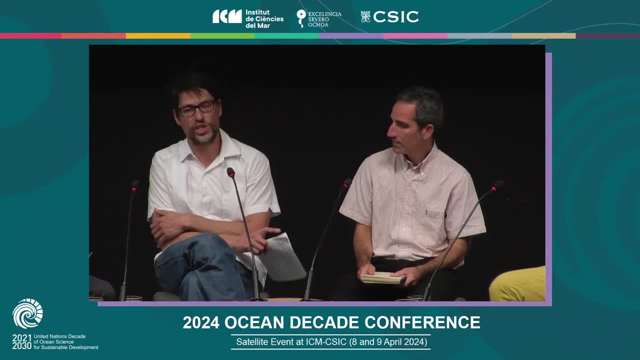 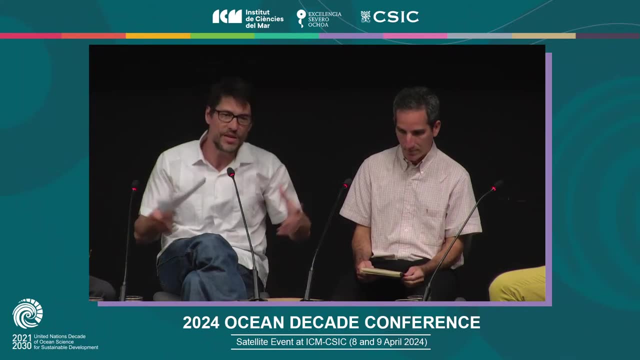 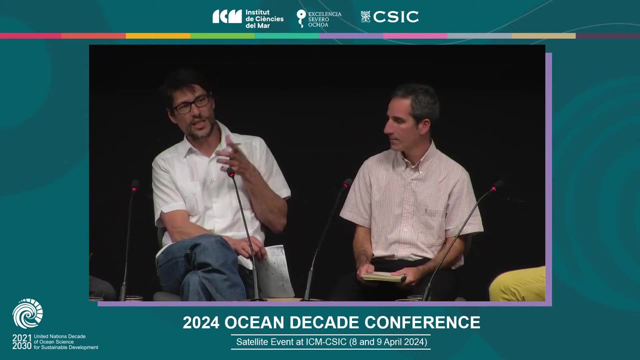 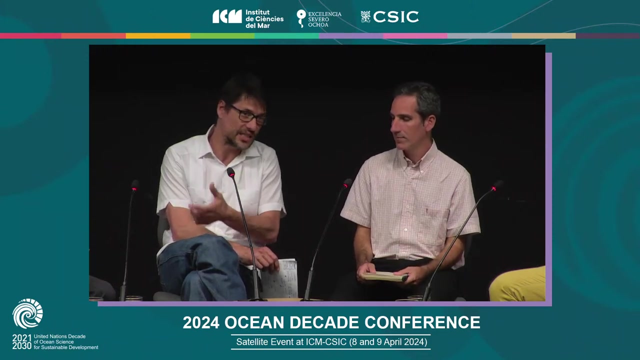 preserve and to conserve the ocean. One special activity that we're trying to become a program if you want. it's like monitoring the marine pollution. Specifically, we were interested in accounting for the plastic. It's a very actual topic- the microplastics and plastics. 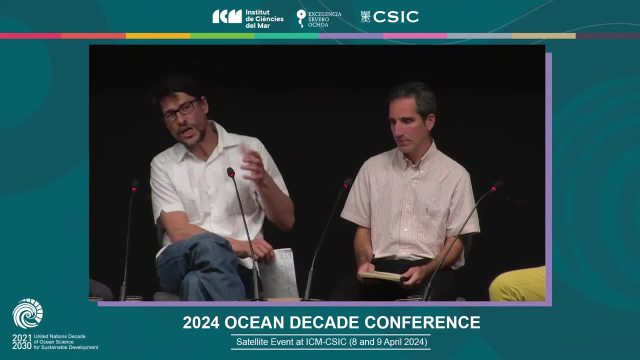 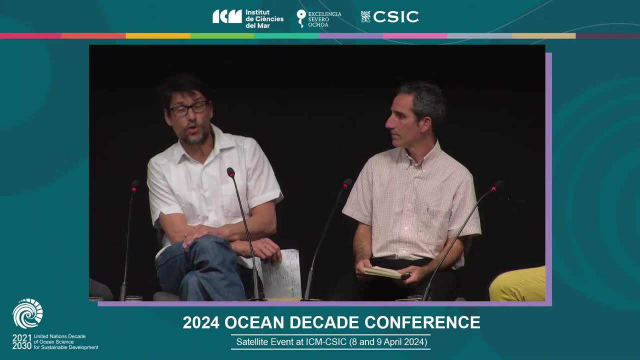 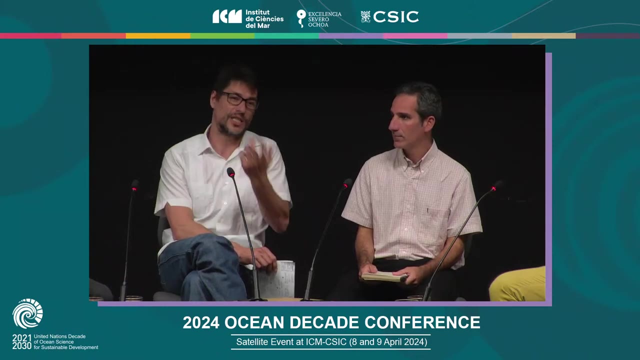 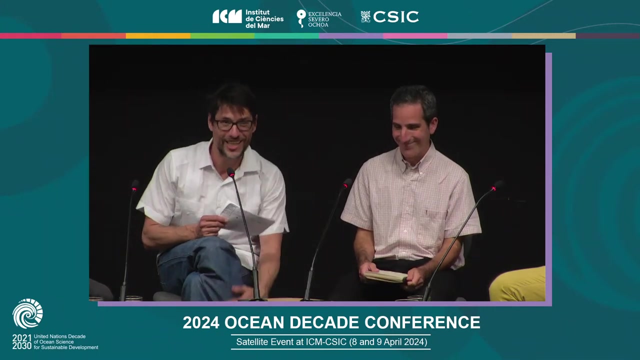 So our environmental approach was to study the turtles- sea turtles. And why the sea turtles? Because they are like ocean sentinels. They are very long-lived animals that are tens of years Like traveling with the large-scale currents, like the movie Nemo showed us. where the turtles 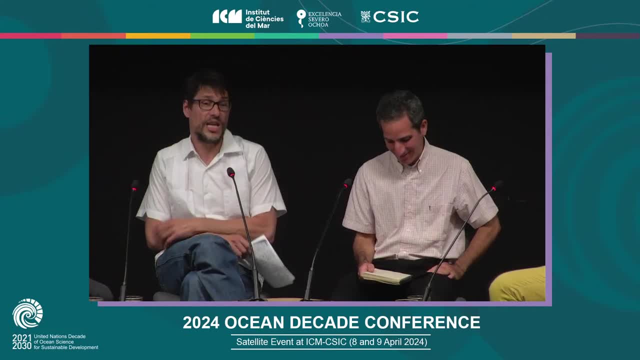 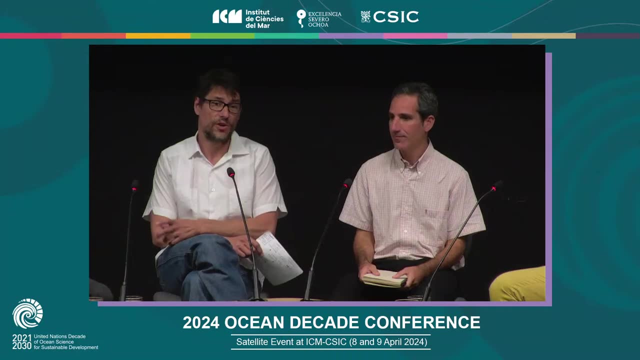 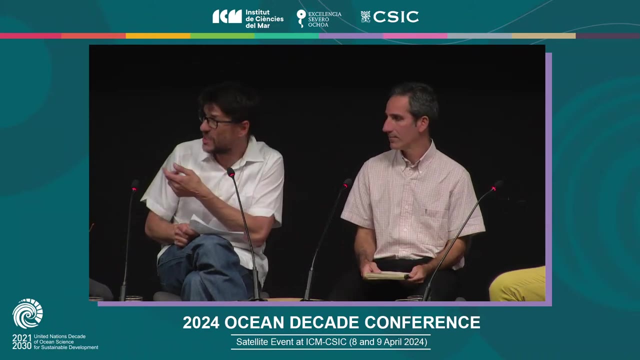 travel all around the ocean, So they are concentrating like plastics, And so we thought it was a very nice approach to see for the health status And we choose a specific place in Mexico. it was not in Ensenada, it was located in the 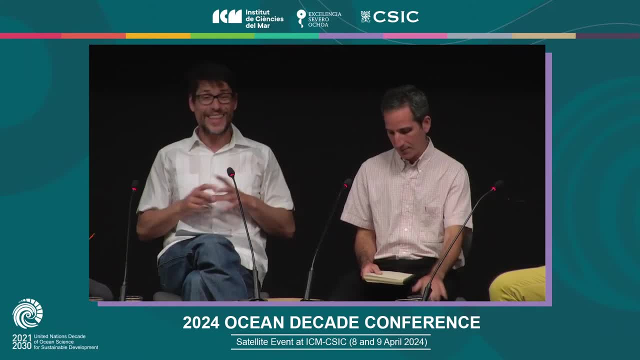 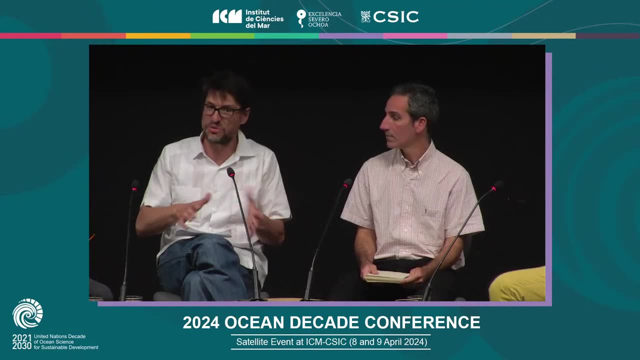 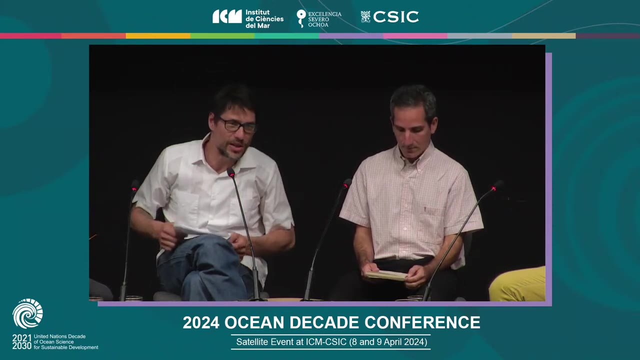 Gulf of California. It's okay, It's called Bahia de Los Angeles And we chose this site because it had a very low population. It has thousands of people, very low population, And also it's a pristine water environment, if you want. 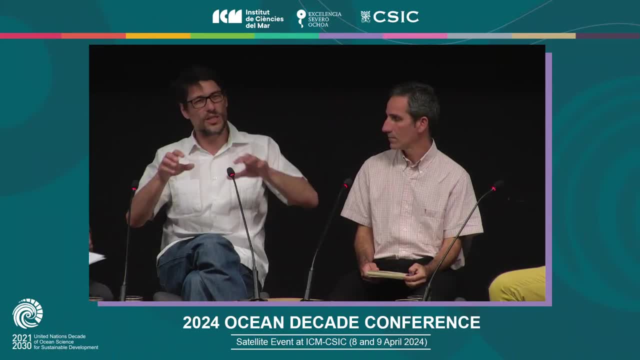 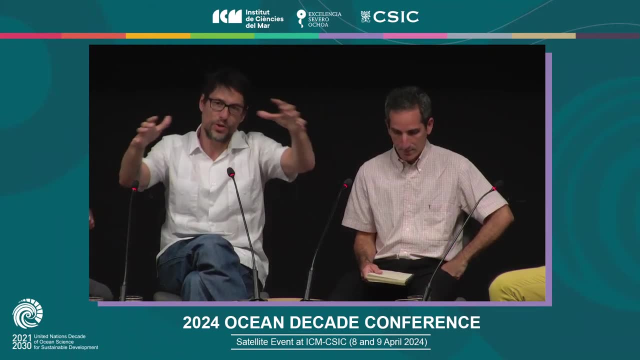 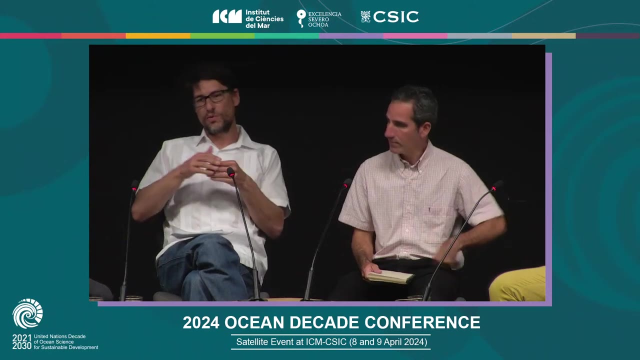 And the turtles were local turtles. These ones did not move much around, So they can tell us about the pollution of local pollution, regional pollution. So we just started with this program And we want to move it to Ensenada. But we just analyzed two turtles. it's a very small sampling. But well, in both of the turtles we found like around 24 microplastics per milliliter, like analyzing the shell, the fins and also fecal samples. So it's a pretty large amount, 24 microplastics. 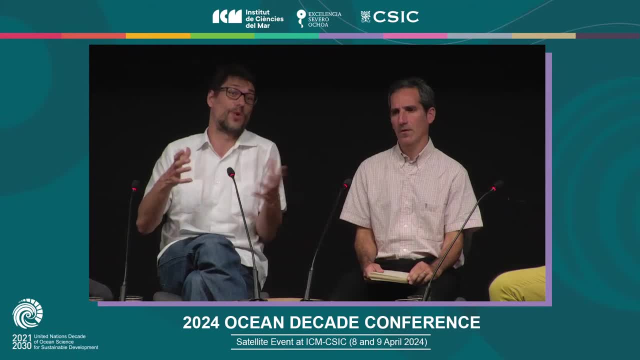 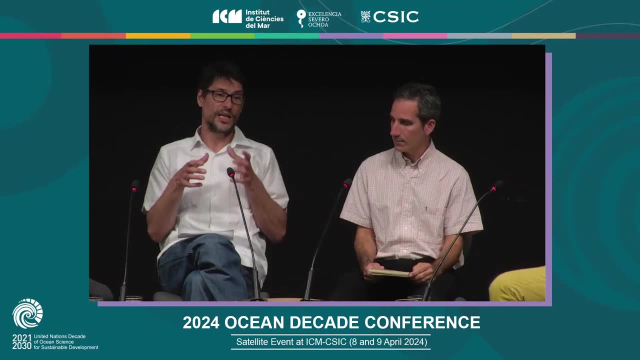 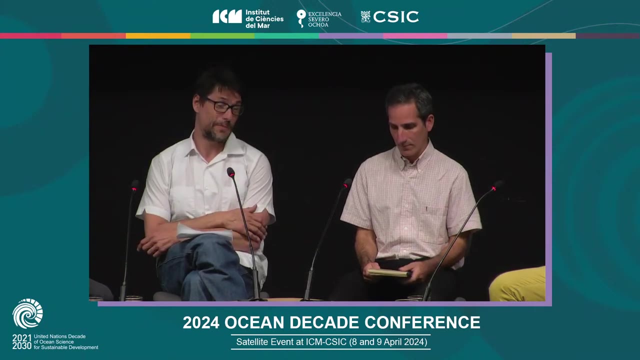 24 microplastics per milliliter, and in very clean waters, if you want. So we really don't know where to come from. these microplastics probably are not locally produced, but they come from remote regions into this pristine and low-populated bay. 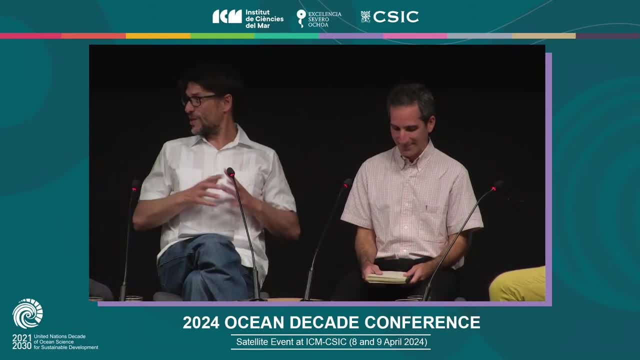 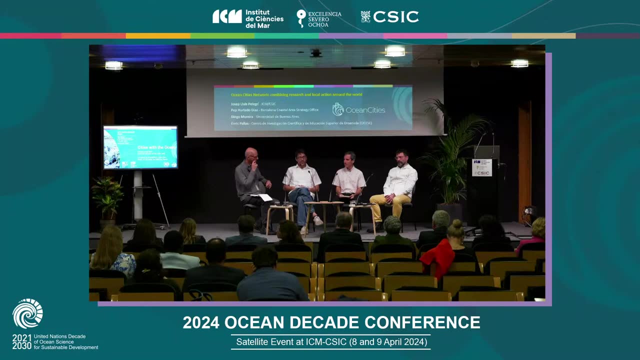 So we've been very active during this 2023, and we want to keep pretty much what our interest is to try to show them. Okay, Okay, Thank you. So we have a very nice bay and with a lot of fauna and flora, and this is very important. 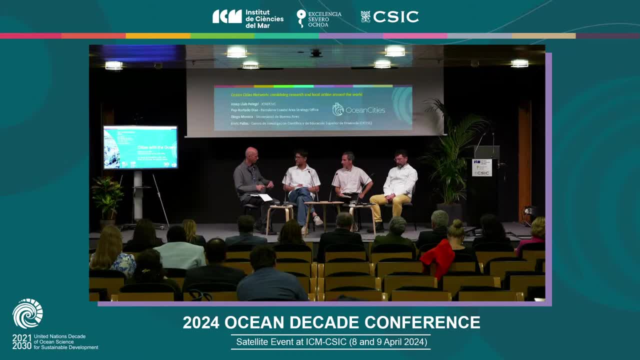 to preserve and to protect the bay. Yeah, Thank you, Thank you. Thank you, Enric. Thank you, Yeah, Okay, so we moved from a city in the Pacific open to large waves, with peculiarities, We moved to a city totally different. 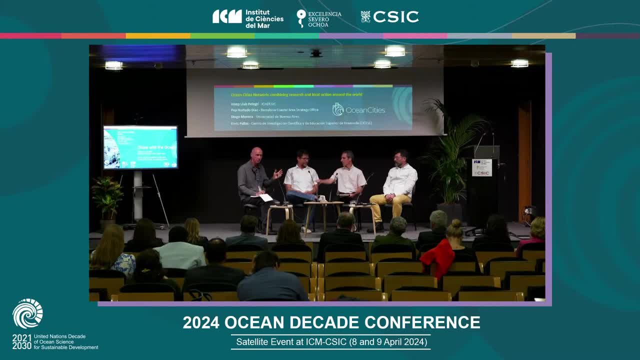 In a very large Rio de la Plata estuary with lots of sediments, in a way similar to the Amazons that we were seeing before, and people experiencing the ocean in a totally different way. So this exchange of ideas, it's really what drives and what builds the knowledge of this. 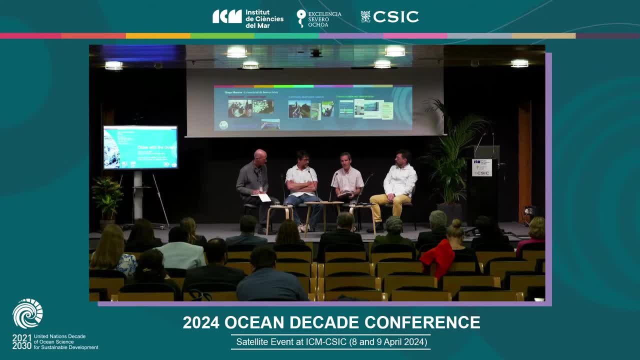 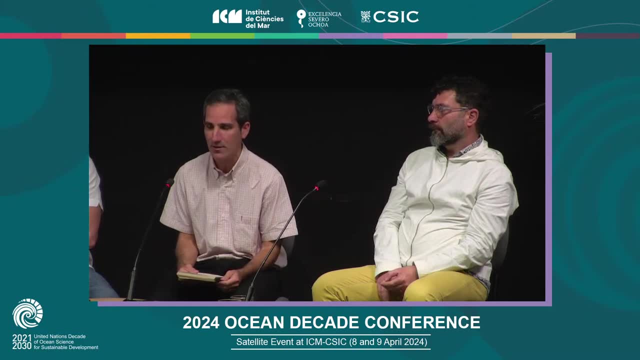 community. Thank you, Jose, please. Well, I'm Digo Moreira. I'm professor of the University of Buenos Aires and also a researcher in the CONICET, similar to the CSIC, And I will talk about some project that we have in Buenos Aires City, in the metropolitan. 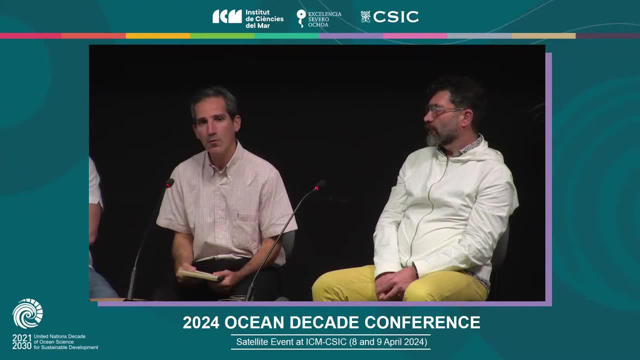 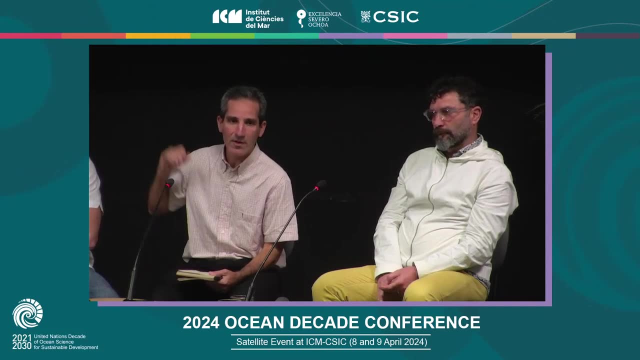 area of Buenos Aires City about flooding events. We suffer. this is very flat terrain so when it rains heavily we suffer a lot of inundation, of flooded events. We begin about 10 years ago. Yeah, now is a part of Ocean City Network- this anticipation of the flutes- and we work. 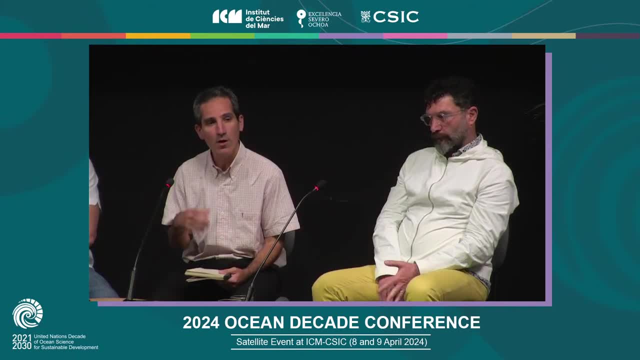 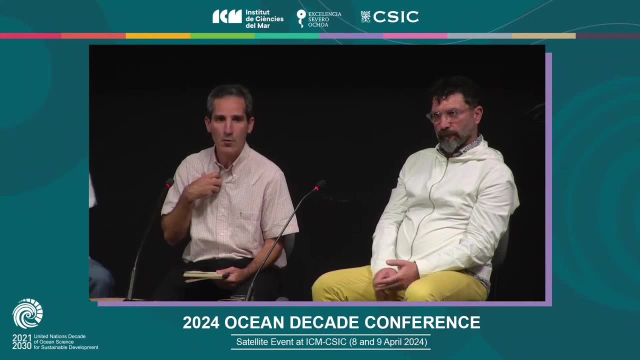 with the schools and the local community, constructing or co-constructing an early warning system centering the community. So we work with our National Weather Service, our National Hydrographic Service, the National Institution of Water and also the Geography Institute, and with the community, The community. 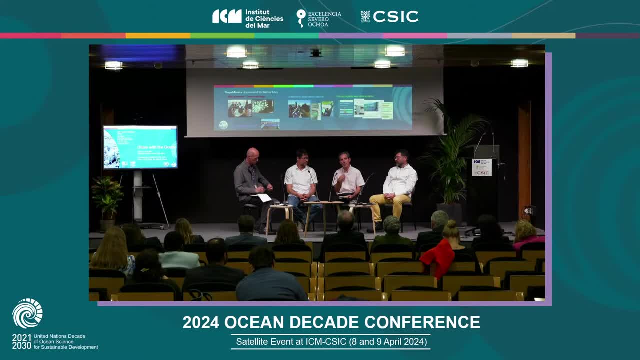 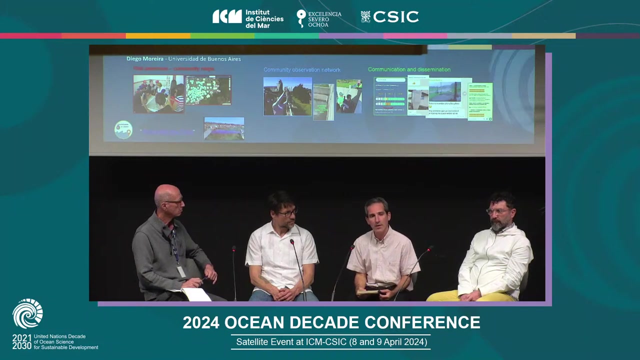 have a knowledge that we don't have in the research area. We begin with the symmetry of knowledge We go to with the community. they show us the terrain where the people live, where the people are more vulnerable or exposed to the flood events. We begin to measure or generate an observation system with the 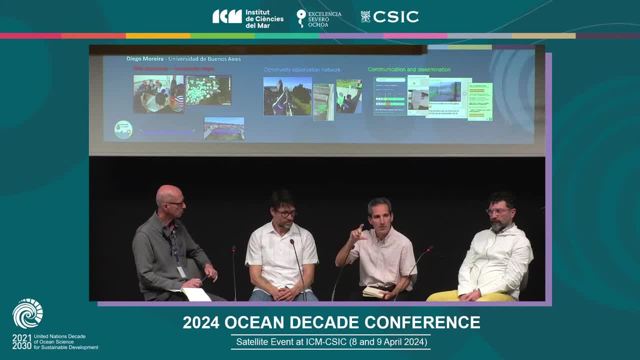 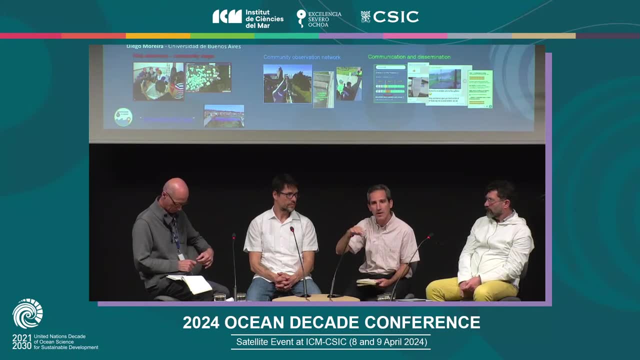 community with rain and gush. that is very simple to measure. in the community, with the school, So they measure the rain, and also with the rules in the rivers so they can measure when the river came out and the water begin to flood the houses. 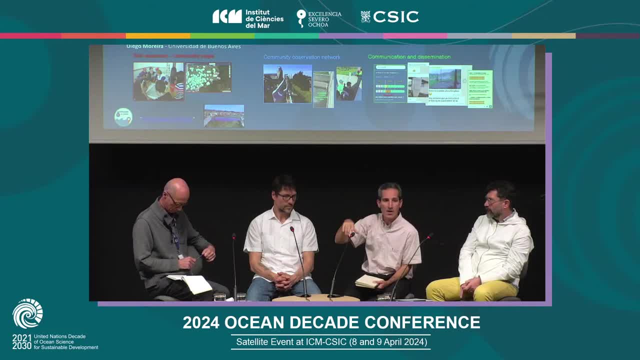 And then we share all the information in a WhatsApp group. The community participate, sending us a photograph and also the rules, the quantity of water that they measure in the rain and gush, And also the civil defense or civil protection work with us. We share this information and we 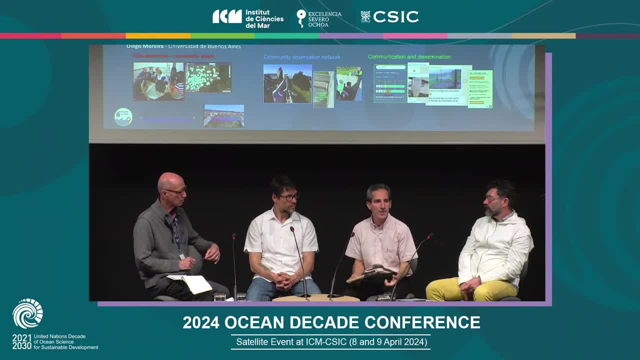 send this alert system to the community, They will be prepared to the events and also sharing the information that they collect. So I think, sharing this opportunity to share this kind of activities or program, it would be really nice to keep in touch with the other city, like Amazon citizens. 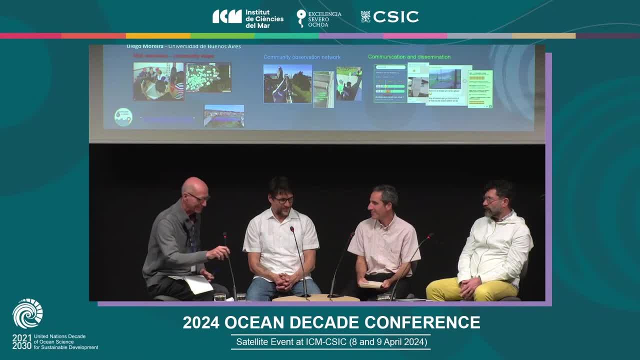 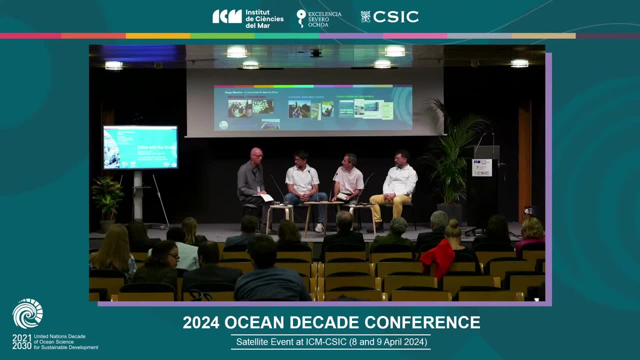 Juan. that's all, thank you. Thank you very much, Diego. So, along these lines, the key factor probably is to reach people so that they become really well-informed and they can both grow as a community and propose new ideas, And I think these ideas then can raise up as strategies. 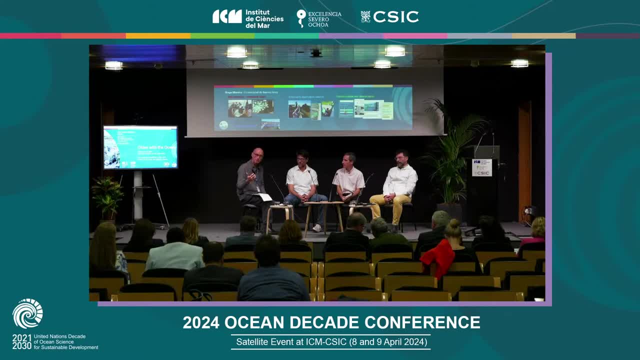 at mid and long terms that have to be undertaken by the administration and, in a way, also put pressure on the stakeholders, the companies, the corporations that are fully responsible of the evolution of our coast and our ocean, And I think that Barcelona is an excellent example. 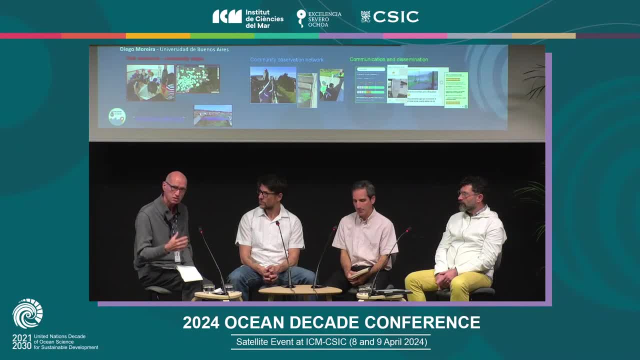 of this way of thinking, This way of acting? no, There's been for many years, particularly during the last years, but for many years there's been a high complicity, high engaging of the different actors, both from the local quarters. 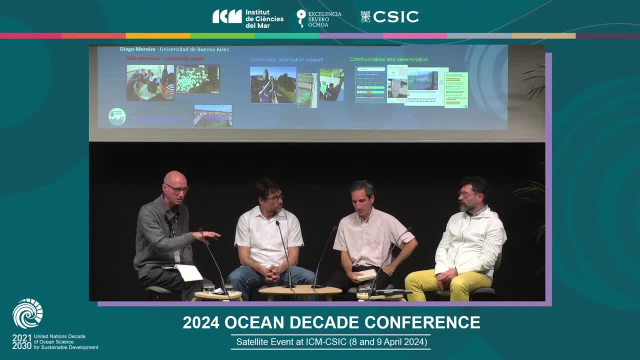 in the coastal communities, and the city hall has been endorsing and empowering all these social communities and engaging the scientific institutions and academic institutions in this process, And I think Pepi's the ideal person. But can you explain us a little bit how this has been? 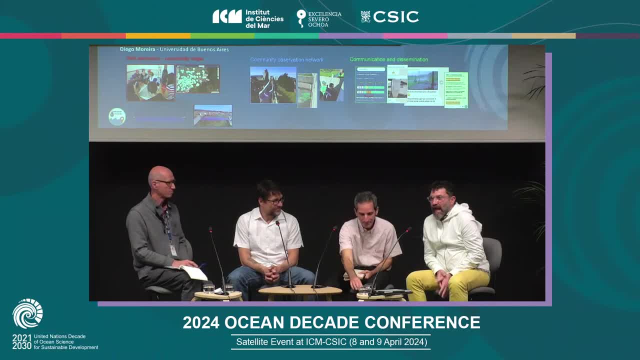 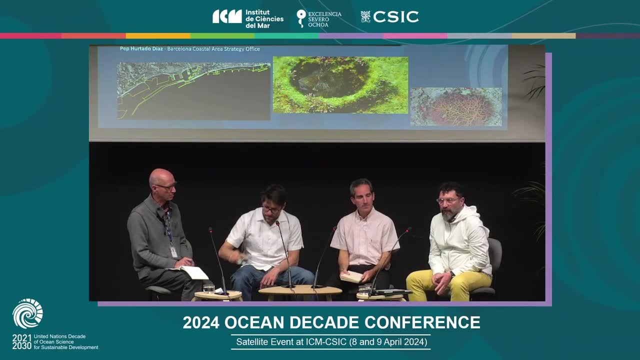 involved during the last years. Thank you, Josep Lluís. I am coming from the strategic coastal plan office on Barcelona And, as we heard before, knowledge, engagement, literacy is the concepts that we are working now. Barcelona city, The city council as a Mediterranean local corporation. 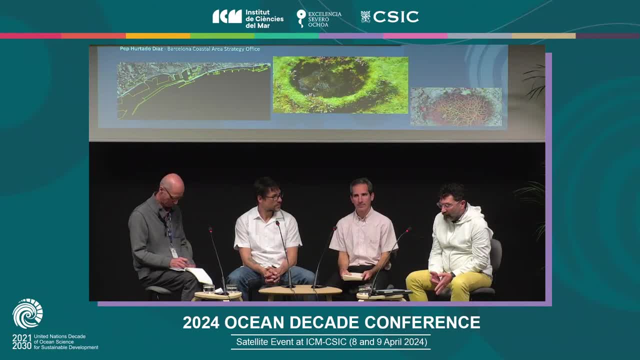 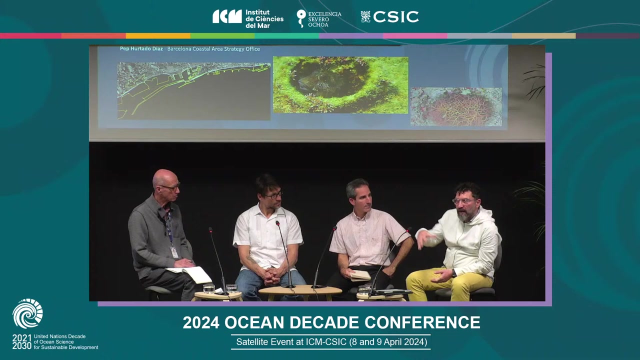 is Boston blue economy, capacity building, fostering innovation and adding value to the employment. And with a project, with the partnership with the Institut Ciencias del Mar that has hosted us, we are developing Mar de Ciencia, the sea of science. that is a project that will 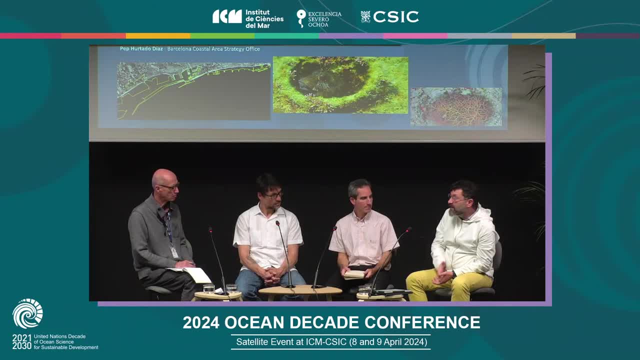 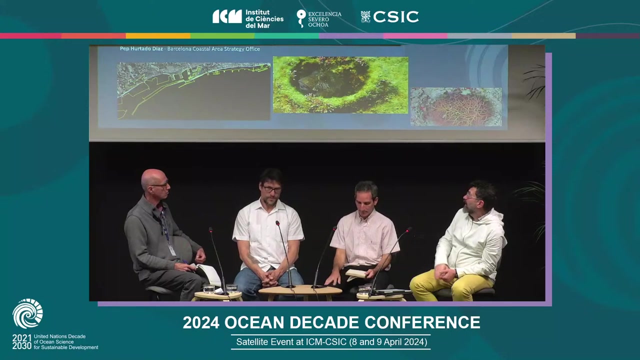 We do transfer knowledge to the, To the citizens of Barcelona, but not also from Barcelona, citizens also from the To the All the world, citizens of the world. As we can see on the pictures, Barcelona have had a big transformation from. 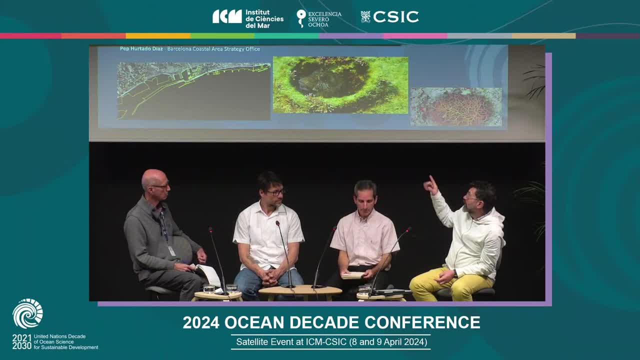 From, From, From the middle of the last century to the recent decades, because was built the front line with urban development that transform The coastline but also the seabed, And now in this seabed, in the seabed of Barcelona, 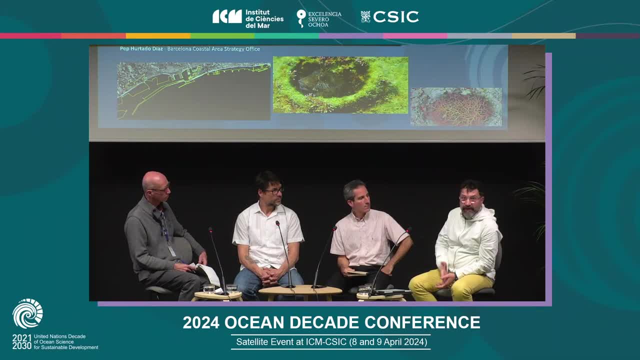 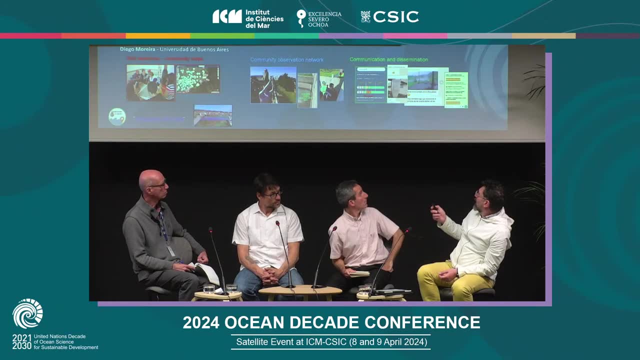 we are a lot of biodiversity, like you can see in these pictures. I'm It's only this one, okay? No, it's only No, it's, It's, It's, It's only Only one, Only one. 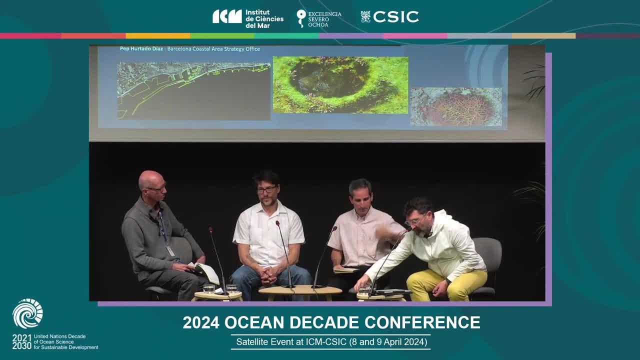 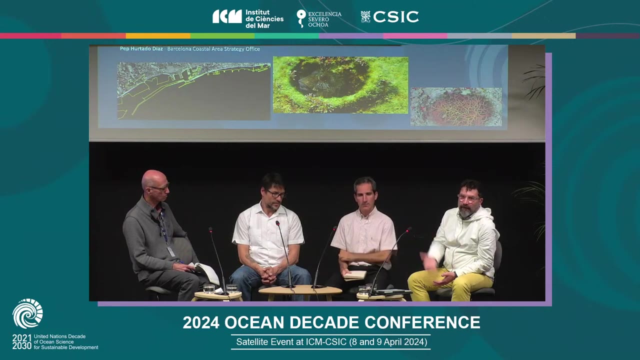 Only one. Yes, it's only one. Yes, Yes, I'm sorry. And from two decades we are transforming this coastal area to boasting to have a better environment and to transform the biodiversity of the seabed. Okay, well, I think this is basically what we want to explain. 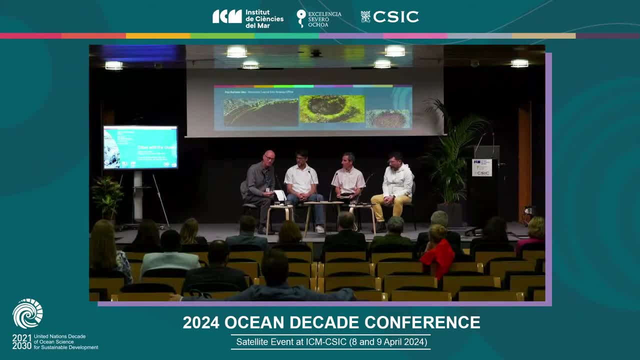 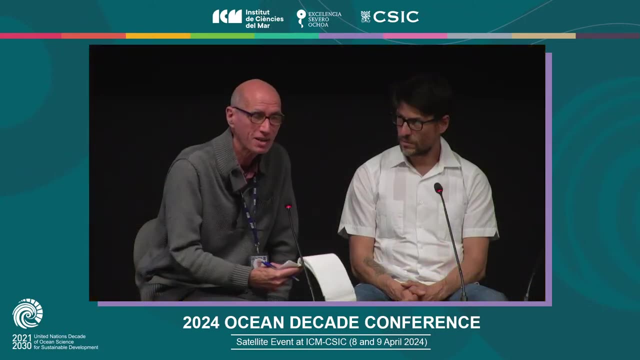 These are only a few examples. There are another many cities that are underlying this collaborative effort among locally, and then the idea is that we are sharing, we are connecting and we are building together this networking. Thank you very much, Thank you. 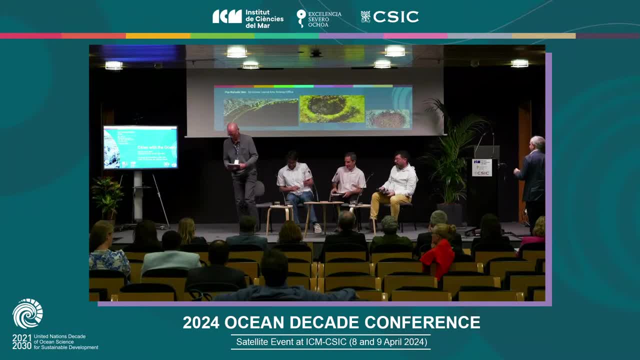 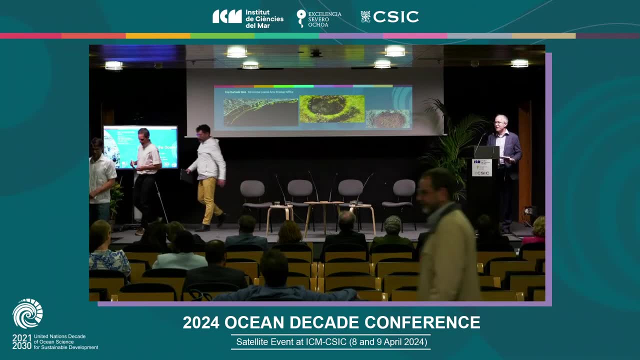 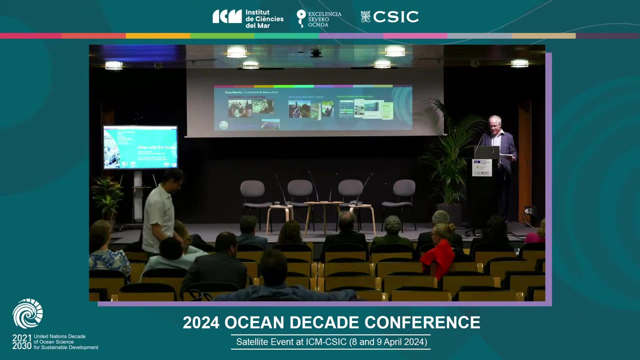 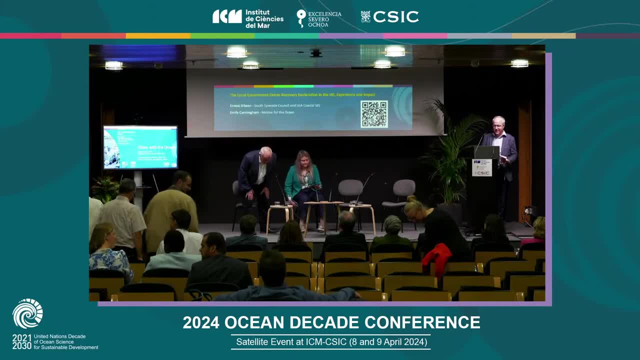 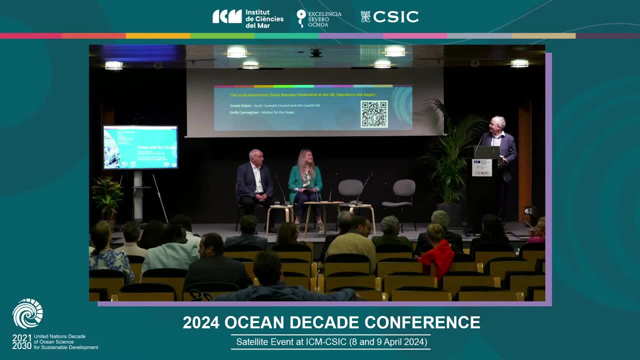 was initiated a few years ago by motion. Good morning, Good morning, Good morning for the ocean, and I am. it's my pleasure to to welcome Emily Cunningham and from motion for the ocean, as well as Ernest Gibson, counselor for South Tyneside Council. thanks a lot. thank you so. good afternoon everybody. as one of the 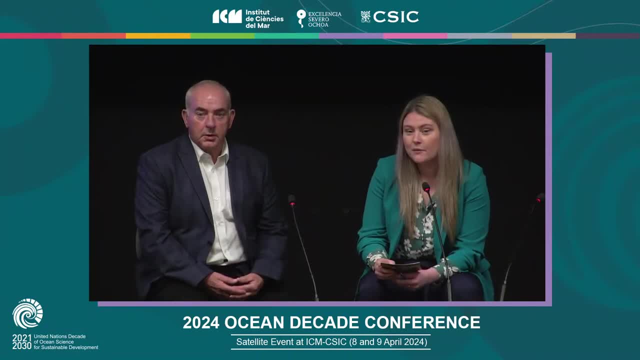 co-hosts of today's event. it's my pleasure to welcome you all and thank you all for giving up your time this afternoon. my name is Emily Cunningham. I'm an ocean conservation professional based in the UK and I'm a co-founder of the motion for the ocean. I'm honored to have with us today councillor Ernest. 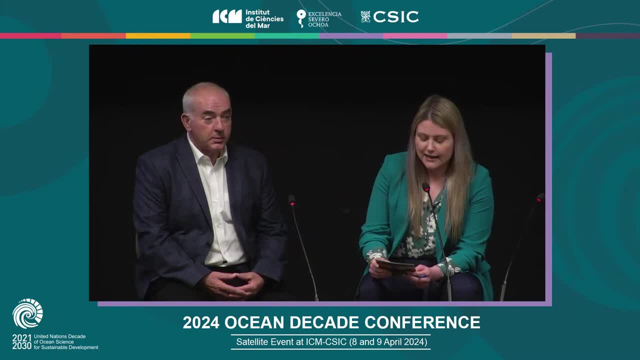 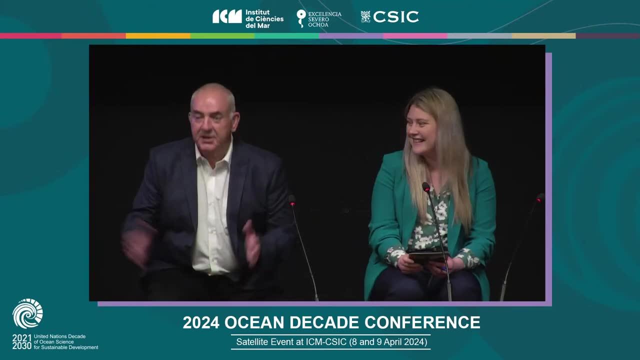 Gibson. so Ernest is the lead member for neighborhood and climate change at South Tyneside Council and also the chairman of the LGA Coastal SIG. I'll tell you a little bit about South Tyneside. I am a Geordie, by the way, so I come from the 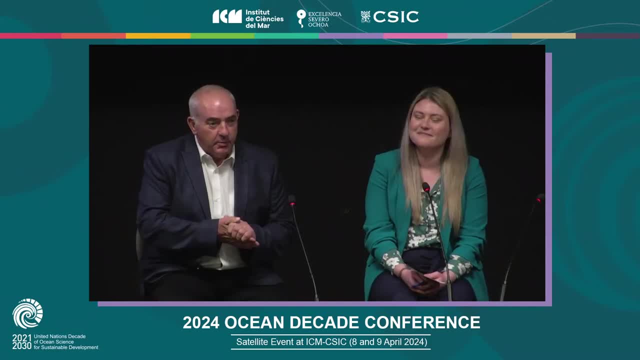 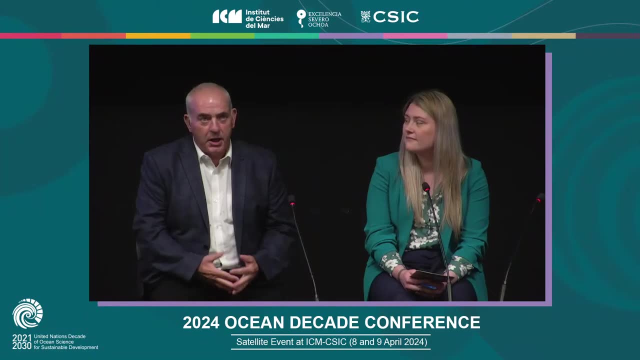 northeast of England. I was an ex coal miner. the area I come from was heavy ship. we built heavy shipping for three quarters of the world. we would produce lots of coals to London for the other power stations. so you can imagine what were. rivers in oceans were. 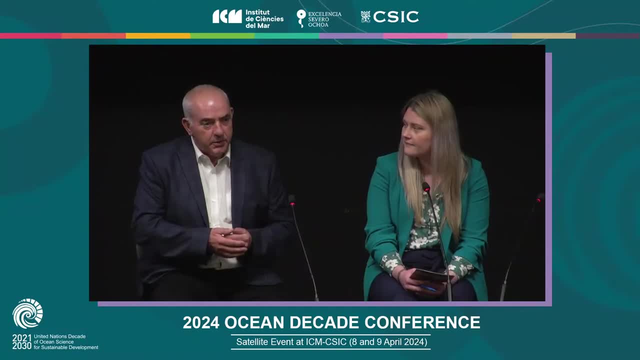 like what fish was starting to be depleted. pollution was quite heavy and we had to do something about it, and over the years, we were always looking at other ways, but the motion for the ocean came about, which give us the foundation stone, and it's all about building on this education. Education is the key to it. it's 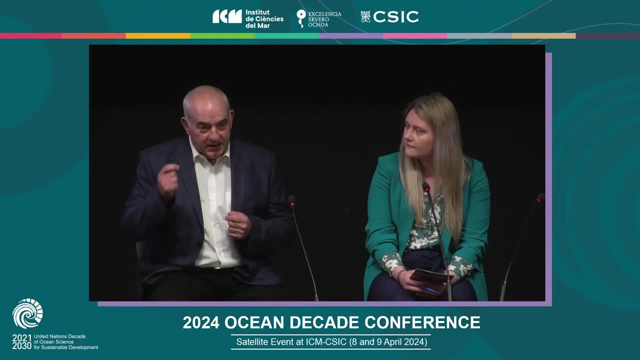 working with schools: it's in bed and policy is the key thing as well. policy within our local plans, policy within everything we do, from procurement to buying to employment procurement- we've got to look at and with embedding within that we have made the ocean for the motion, which is a very importantu. working with schools: it's embedding. policy is the key thing as well. policies within our local plans, policies within everything we do, from procurement to buying to employment procurement: we've got to look at. with embedding within 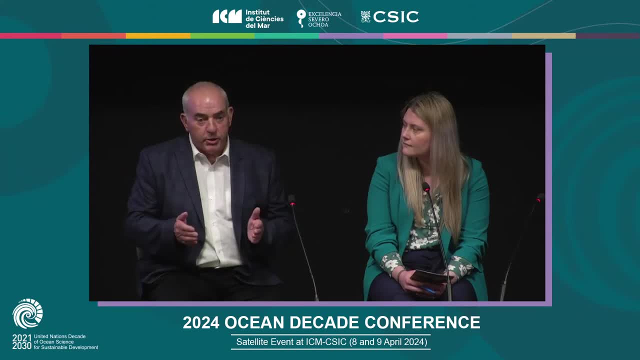 that we've got to look at it. with embedding within that, we have made the étienne for the, which is really cost effective. It costs the councils very little, with this being embedded in it, So as well as giving us a local perspective from South Tyneside, 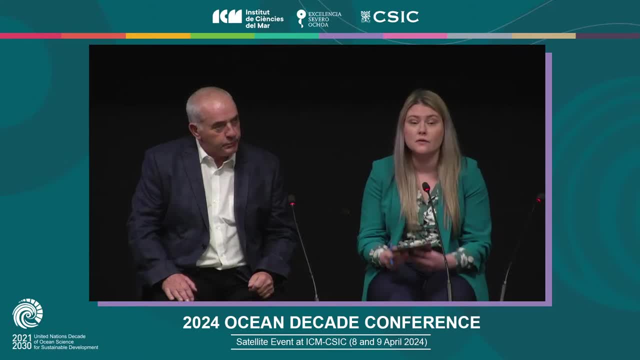 Councillor Gibson is also the chairman of a national coalition of councils, So 57 councils from all around England's coast. Together they cover 60% of the coast and 16 million residents. So this gives us this good balance of a local and a national perspective. 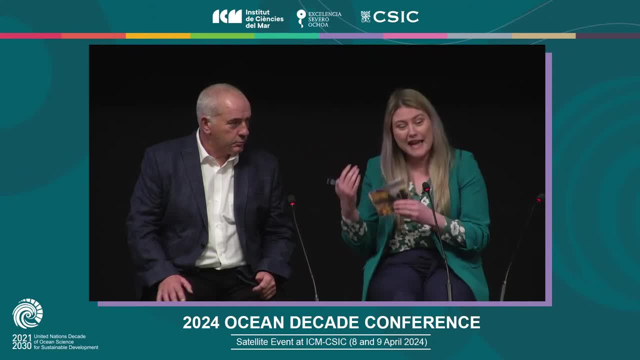 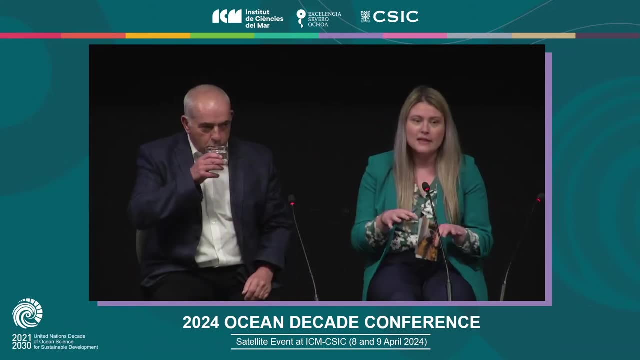 And to tell everybody a little bit about what the motion for the ocean is. so I'm a co-founder, together with Dr Pamela Buchan, who is here as well with us, And back in 2021, I was working leading the local government association special interest group. 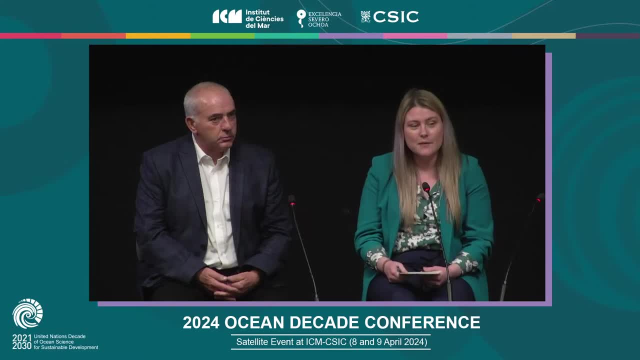 that Ernest is chair of. Pamela was a councillor down in Plymouth, which is on the south coast of England. She's also an expert marine social scientist And we were hearing from councillors that there was a real appetite to want to do something for the ocean. 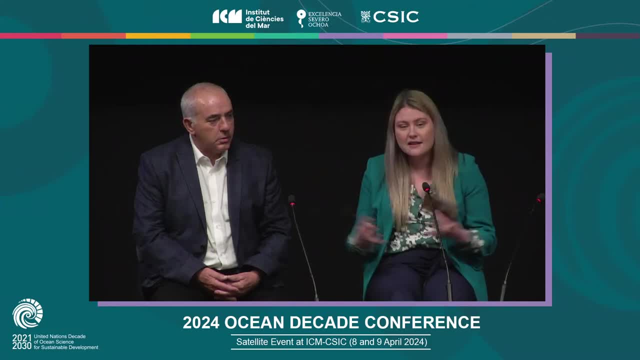 but they didn't necessarily have the knowledge or the capacity within the local government to make that change. And we'd seen how effective the climate emergency declaration had been for many local governments all around the world, And so we created an ocean recovery declaration- So like the climate emergency declaration, but linked to ocean health. 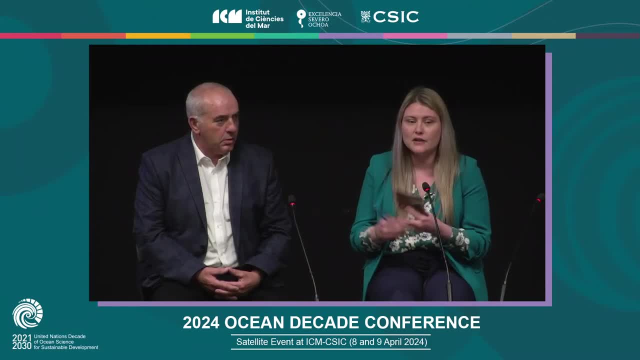 And so Pamela and I, and our colleague Nicola Bridge, who's an expert in ocean literacy, we created the motion for the ocean, the ocean recovery declaration, And we worked with experts in marine science and marine policy from all around England and created eight evidence-based commitments. 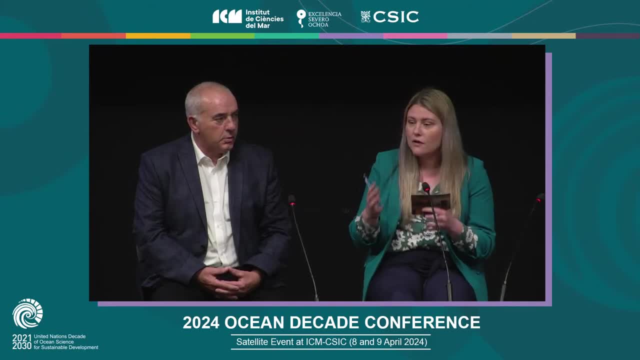 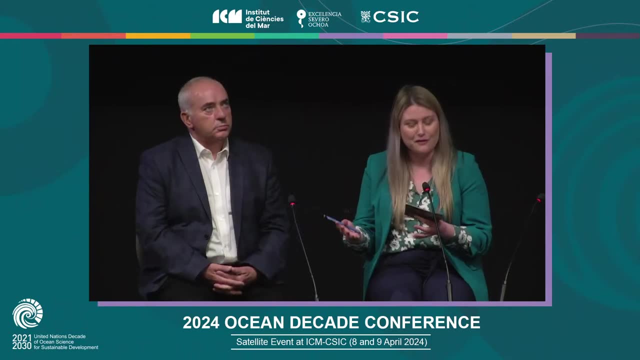 And that form. And that form becomes the ocean recovery declaration. So they're all the things that are within a local government's power, responsibility and privilege to take action for better or worse for the health of the ocean. The way to think of it is really: it's like a blueprint for local action for ocean recovery. 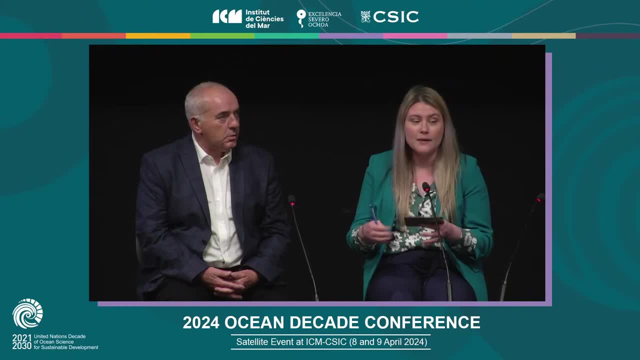 So it allows councils of all sizes to step up and take ocean action, meaningful ocean action- and also to grow ocean literacy locally. You'll hear us call it both the motion for the ocean and an ocean recovery declaration. It's called motion for the ocean because I'm sure that all the politicians know. 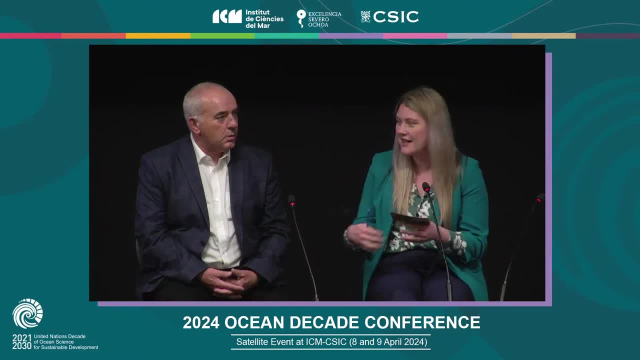 motion is the proposal that you put to council to get a change. So it got the nickname motion for the ocean, but it is a local government ocean recovery declaration. So Councillor Gibson was the third councillor to propose our motion for the ocean. 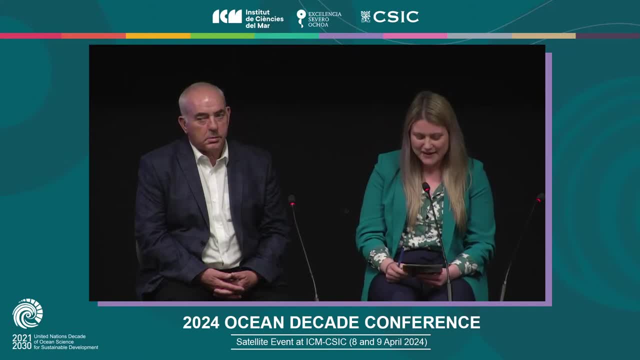 Pam was our first councillor to propose our motion for the ocean in Plymouth. Why did you feel, Ernest, that it was important to propose a motion for the ocean in South Tyneside? Why did you feel that it was important to propose a motion for the ocean in South Tyneside? 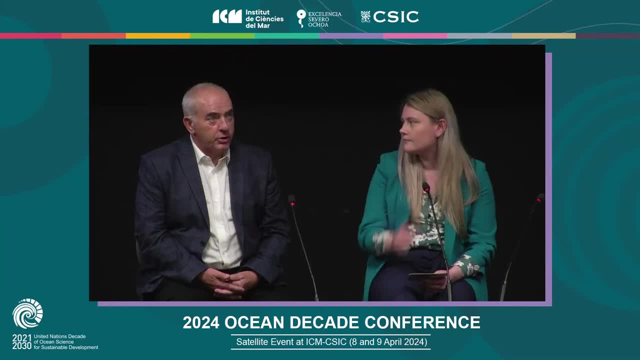 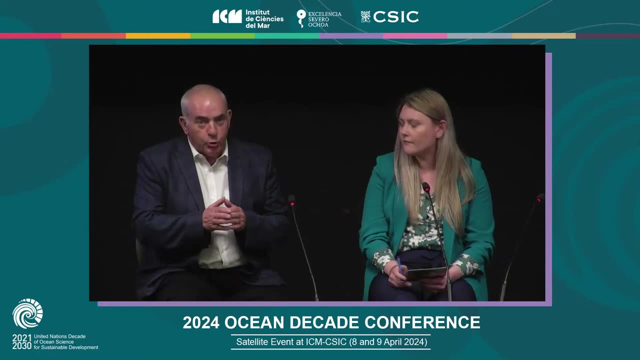 We felt that the motion for the ocean gave us, as I said before, the blueprint, the foundation to build from It put us in the right direction. People were talking about it, People felt safe with it within the community- You know, you go out- and everybody was saying: what's happened to our ocean? 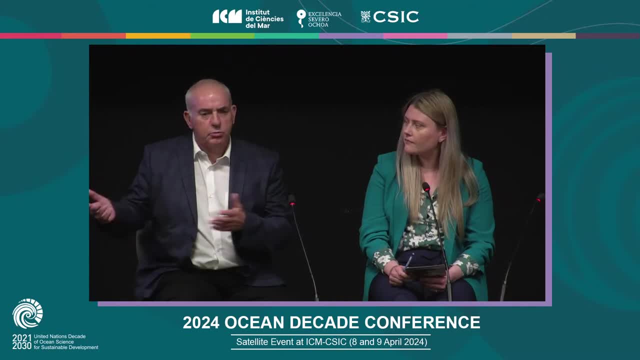 Why? What's happening with climate change? You know coastal erosion was affecting the local economy as well, So I had to do something. So this gives us the key to it, And it's about working with partners. It's not just one person can develop it. 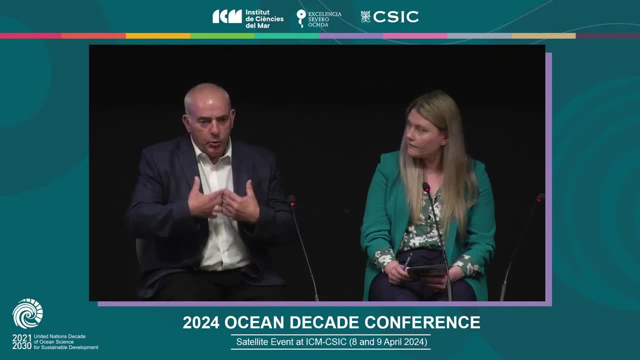 It's about everyone Within the local authority. we used to have one person who dealt with the ocean. Now you know, they said we'll have a team. We haven't got a team. now We've got everybody, because it's everybody's responsibility to deliver for the ocean. 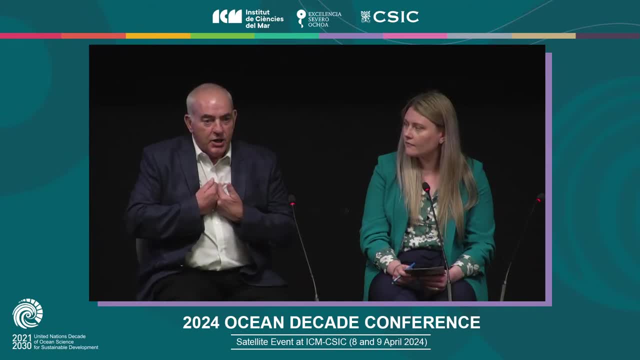 We'll work with local businesses. Local businesses come on board. Since this came about, everybody wants to be part of it. It's working with community groups. It's as you said. it's embedded in education and our curriculums within the schools. 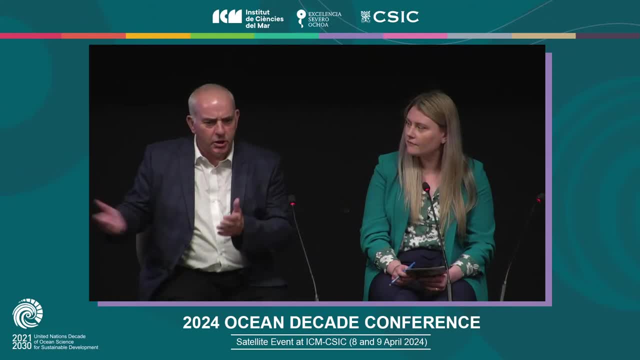 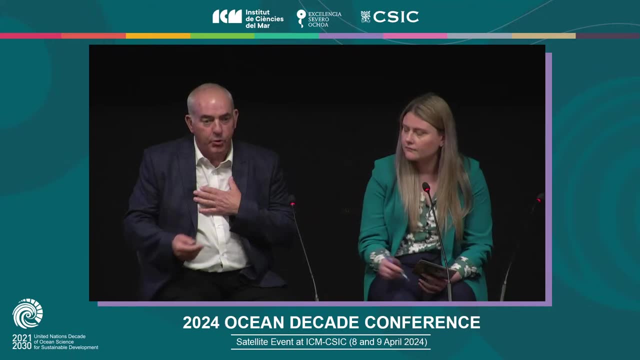 We have people in our coastline who live 100 yards from the beach. They've never felt sand between their toes. These are the kinds- some of it is through cultural differences- but they've never experienced it. So the ocean is a great healer. 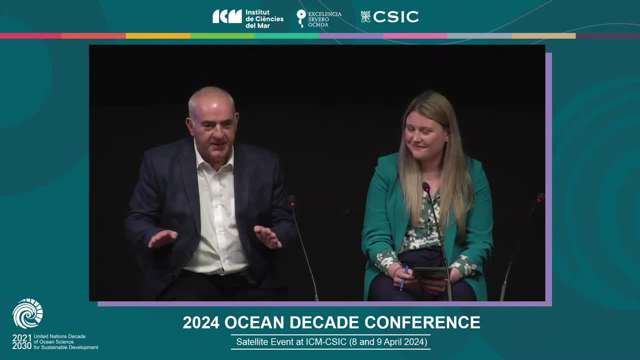 You don't need to go to the doctors for some medicine, for certain things You can go to the ocean. You know, my father died a few years ago and you felt, oh, you feel the world's falling apart. You go to the sea. 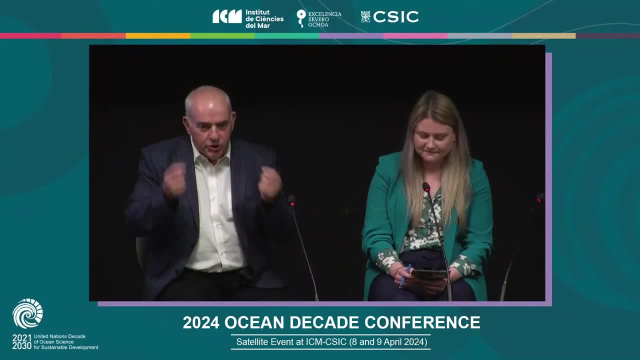 It's got healing powers. The sea, the ocean does help you in many ways. A lot of people I've spoken to who have health issues, they say you go there, you feel better. It's better than any tonic any doctor can give you. 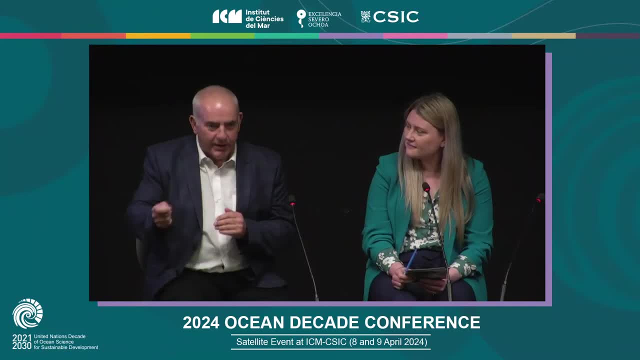 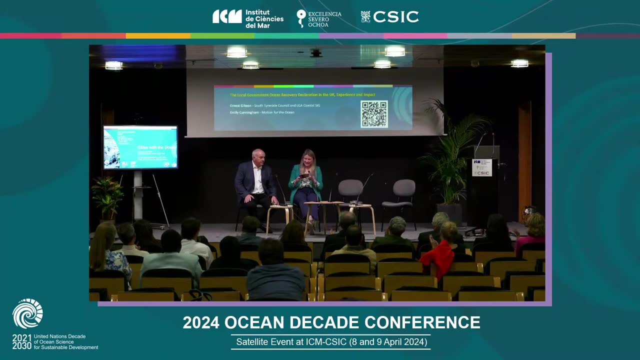 So this is why we need the motion for the ocean. We've got to get out there for a sustainable future. Thank you, I agree. Thank you So, Councillor Gibson, he was the third councillor to propose our motion for the ocean. 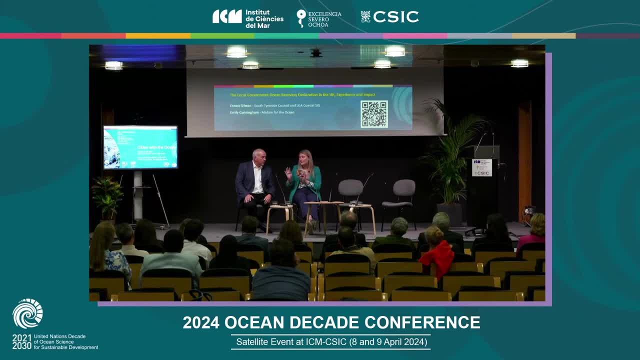 but he has been the loudest and longest champion, So I'm really grateful that he could join us here today. You were the third, but we've now got 27 councils from all around England and Wales who have made an ocean recovery declaration using our motion for the ocean. 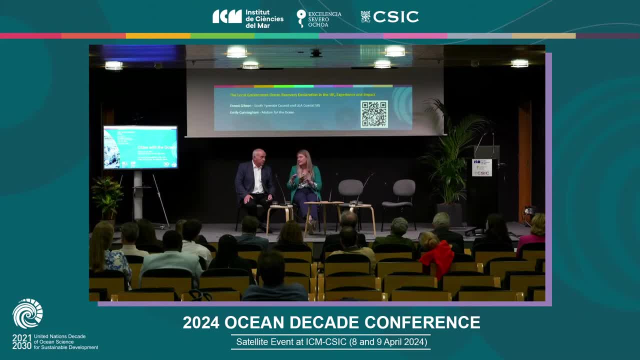 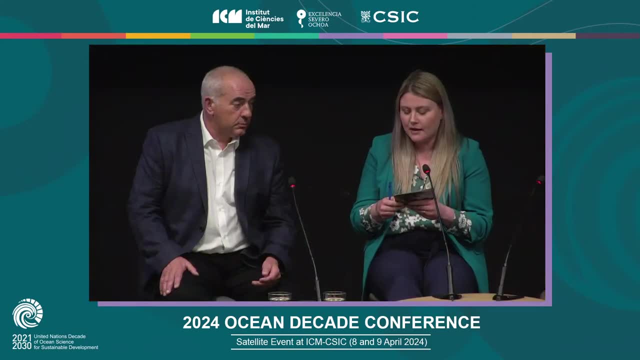 They're of all sizes, from little towns all the way to big cities. so Plymouth, Nottingham- Together they cover 4 million residents. So we're really excited at how it's gaining momentum. But as the chair of the LGA Coastal SIG, you have this national oversight as well. 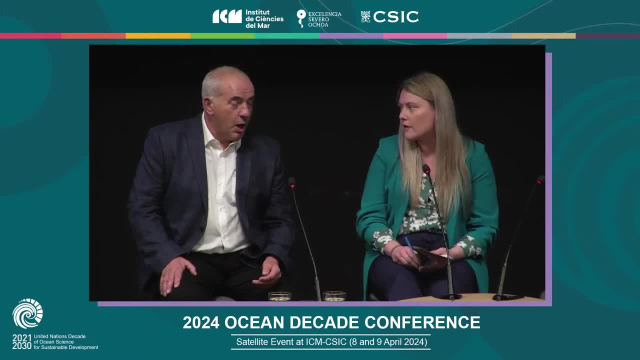 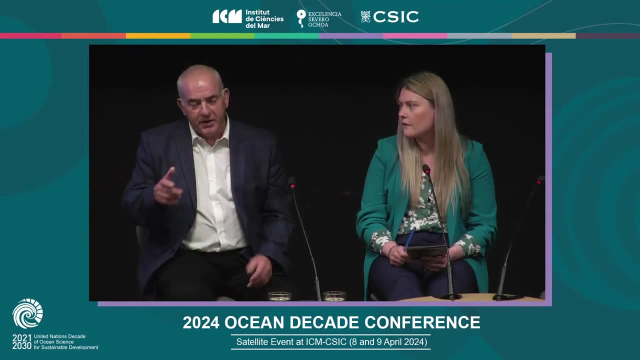 So what has been the feedback from other UK councils about the motion for the ocean? The feedback from other UK councils: some of them are positive. Some of them are very negative regarding it. Some of them are worried about cost, But I can reassure you, the cost is very minimal. 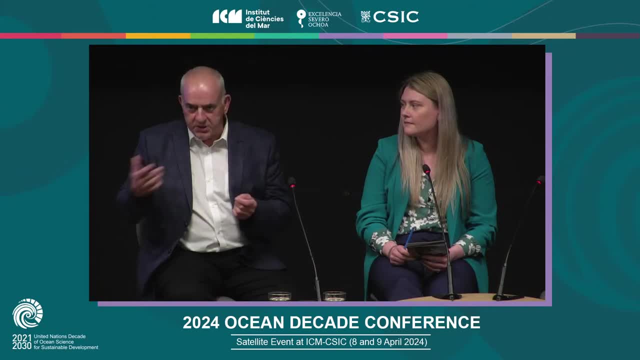 As I stated before, procurement exercise 106 money, as you have in England, which is when developers develop anywhere. they invest money for social values, but also into the community And this is where the money comes from. But with embedded into procurement, it's set in every policy. 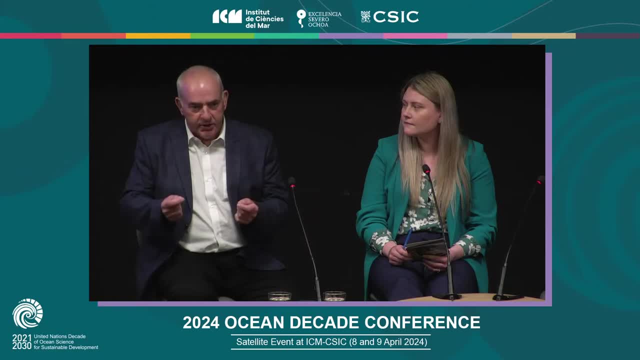 So, everything the local council does, we'll look at the environment, we'll look at the ocean, because it's become a major part. Tourism, because we've lost all this heavy industry. we need to bring people to the coastline, The coastline. 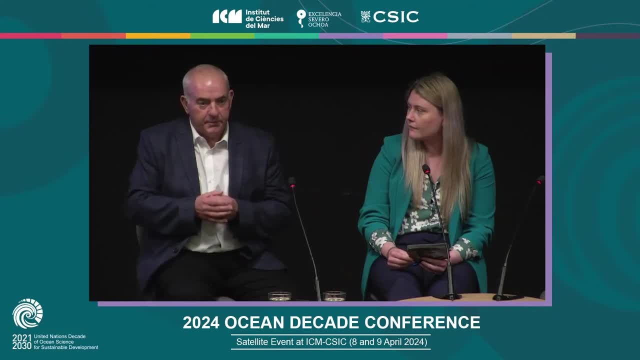 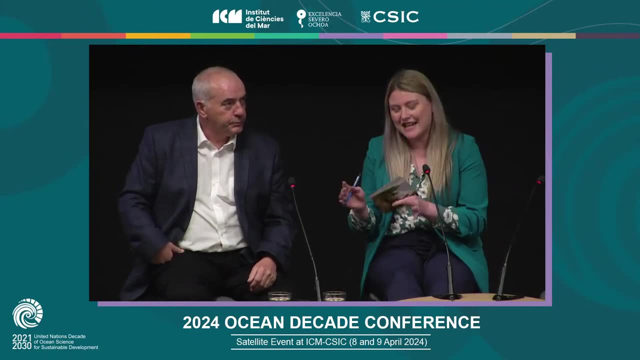 It's a place of work now for people. Tourism is the key, And so I think we got a lot of wariness around a potential cost. Is this another project? Is this going to need another team? But actually it's a culture change within a council of making the ocean everybody's responsibility. 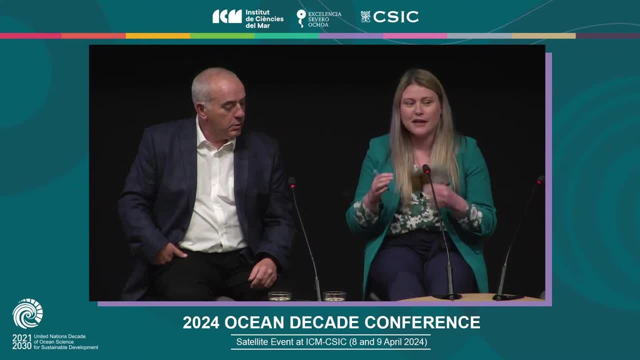 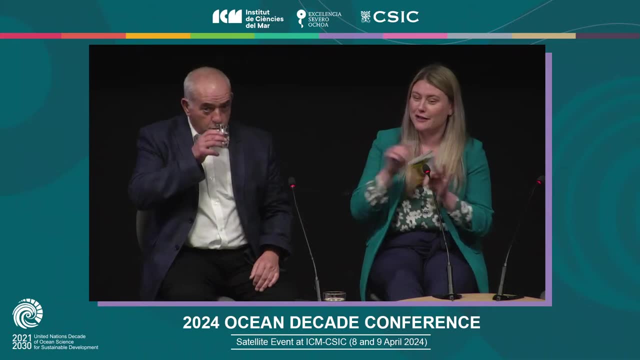 And quite early on we got approached by inland councils. So we had developed it thinking it would just be for coastal councils, And then councils right in the middle of England, which England's not that far from the ocean- if you're in the middle, 70 miles from the ocean. 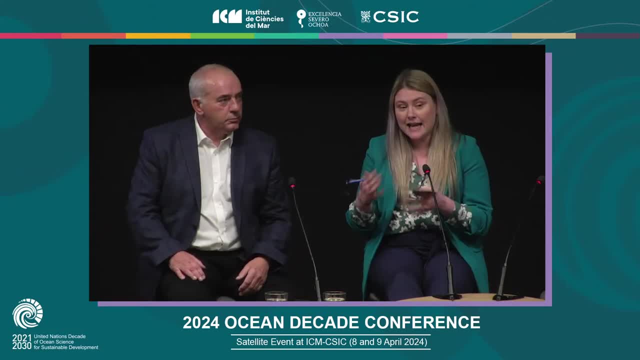 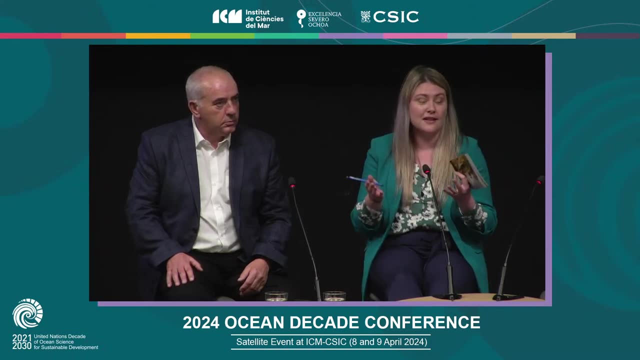 And we were getting in touch saying we want to do something. So we developed an inland motion for the ocean as well. So we have one which takes source to sea thinking, bringing ocean literacy to communities right in the centre of England Because, as we know, no matter where you live, you're affected by the ocean and you affect the ocean too. 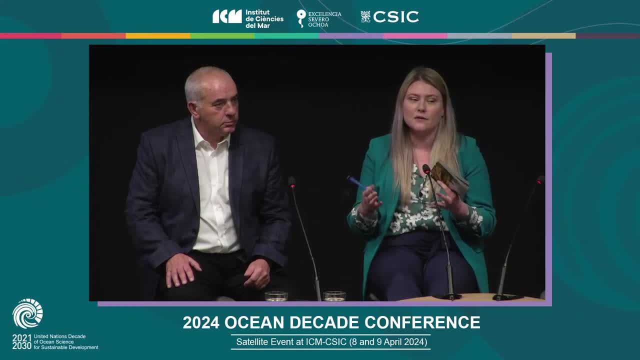 And so myself and my co-authors. we give free support to councils throughout developing it, So we try and make it locally relevant during the declaration process and then afterwards to help them implement it, Because we want to ensure this is more than just words on a page. 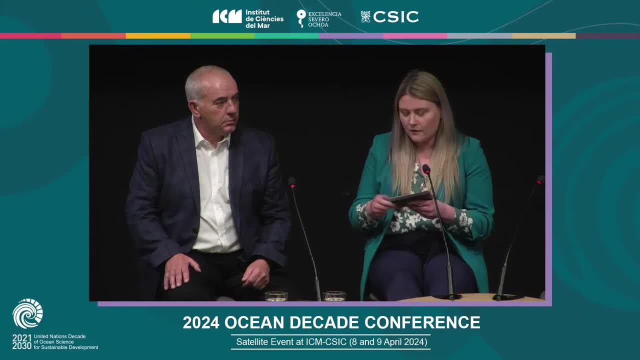 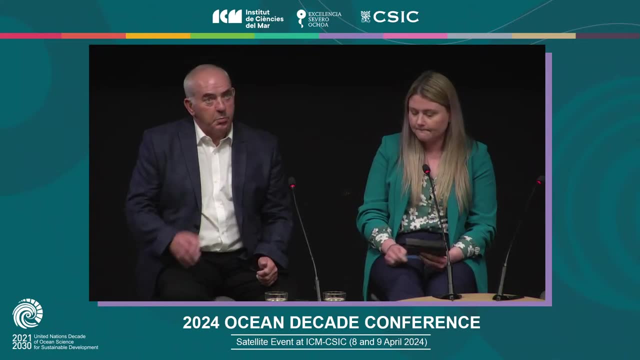 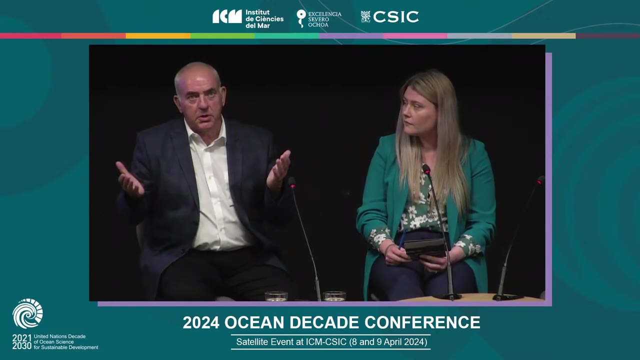 That it's actually meaningful action. And so, talking of action, what do you say? the most standout impacts have been in South Tyneside, The most standout impact with coastal erosion and the motion for the ocean. We've had a lot of fish depleted. 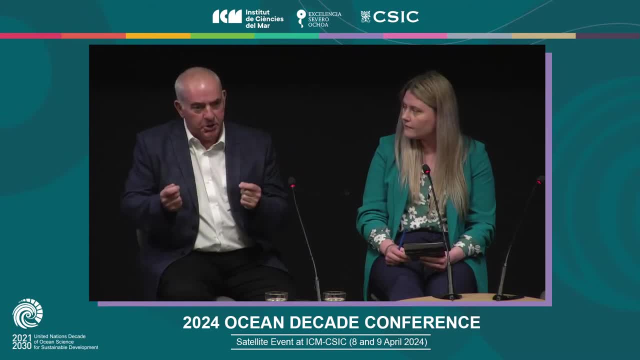 The stocks of our fish have depleted massively. We've had people complain about pollution, plastics, which is a main thing I heard somebody mention about fibres. They're not in the ocean Worldwide. we should be asking for washing machine companies or water companies to put filters on these washing machines which would prevent this. 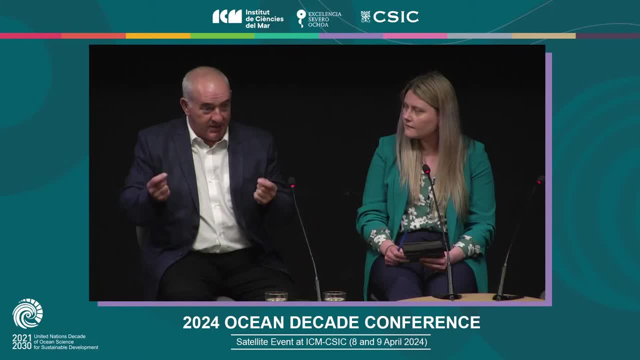 It would help. It wouldn't prevent it, but it's a step in the right direction. So have you found the motion since you've declared it? how has that benefited against those impacts? It's benefited massively, because what we've done is we've worked with the universities as well. 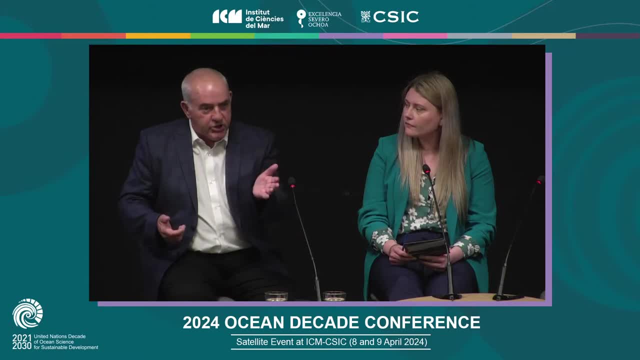 They've all came on board. It's the educational aspect Somebody mentioned about art In music. we've done the Blue Art Foundation, what was in the summer, And it was about artists' expression, how they feel about the ocean, And children came to see it. 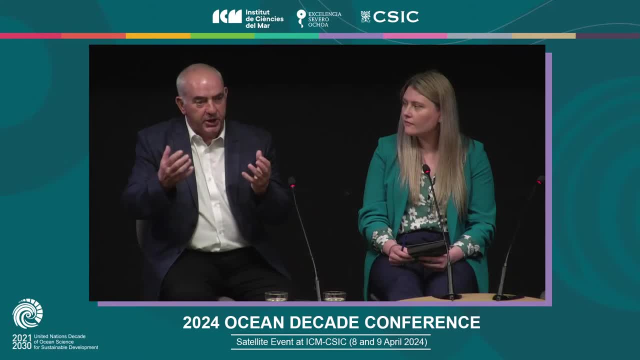 And it did. It was educational Just by looking at pictures. no words, just pictures- and it told you what the ocean was. It's part of our sustainability and the key for life. But there's a lot of investment can go into the ocean, but it's out there. 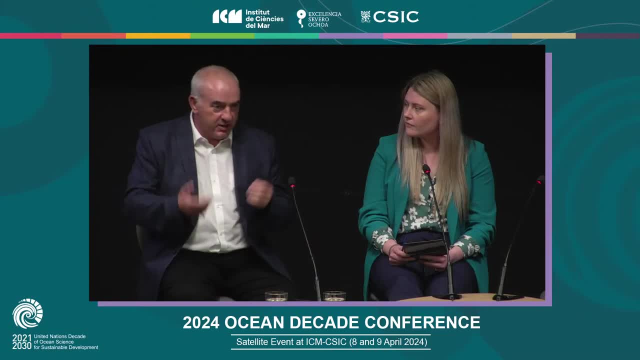 And it's skills You know. we could talk about the Green and Blue Agenda in South Tyneside. We have looked at that. We're bringing lots of prosperity jobs coming up with the ocean. We'll work with Seascapes, which looks at natural resources for habitats. 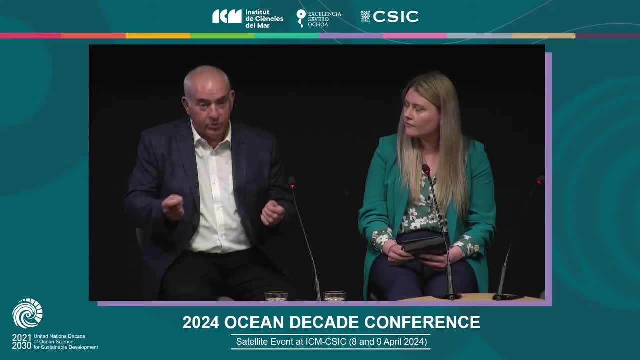 We're looking at Stronger Shores, which is natural-based solutions which they're working on, which could come in policy in a few years' time. These are the things we've looked at and we've pushed forward at. If the motion for the ocean wasn't there, we wouldn't have been doing that. 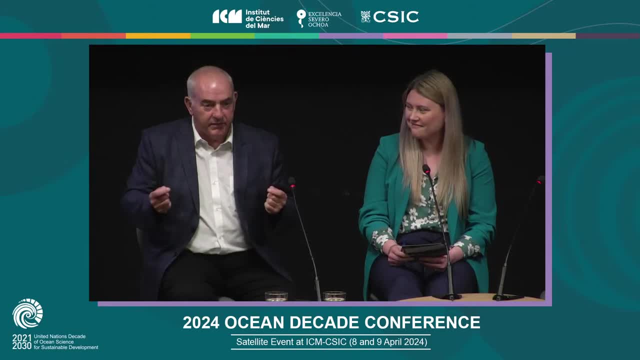 We would have still been twiddling my thumbs and thinking, oh, We need to think of a way forward, And this has helped us massively. And so in terms of what next? so we're trying to push this out across the UK. 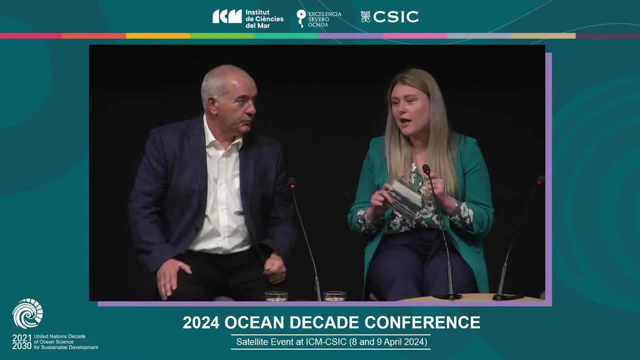 We've got a Welsh version in development, a Scottish version in development. We're very keen to push away from the British Isles as well, So if anybody's interested in working with us, we would love to take it international as well. I think the QR code is here. 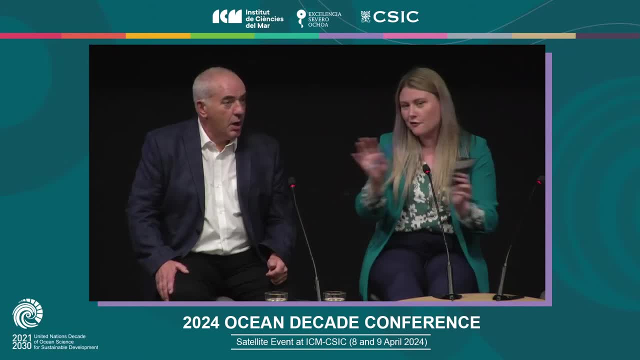 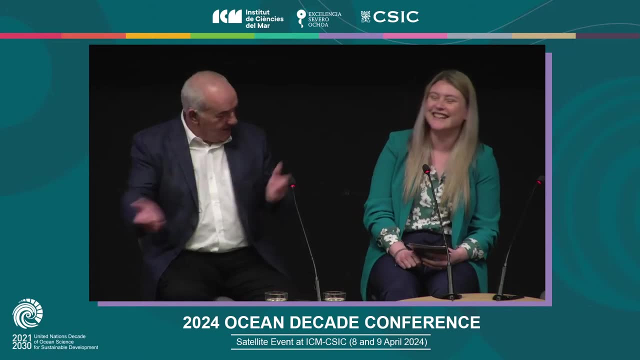 Or speak to us afterwards. Do you have a closing message for all the city leaders and people here today? To all the city leaders: take up the option, the motion for the ocean. It's free. Contact us, Not, Emily, or contact ourselves. 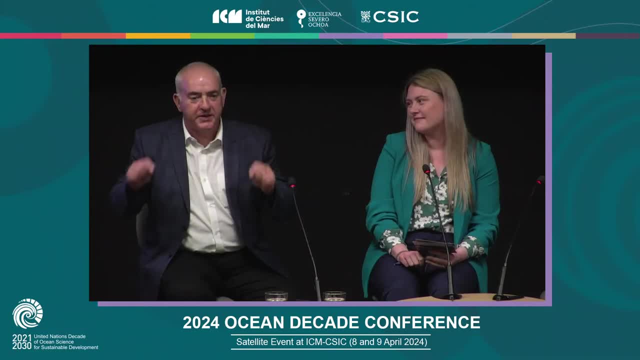 But think of embedding it in your procurement and work with your businesses, who will help you. The key is there, But the other message is we need dedicated coastal ministers around the world who are looking at the ocean, Because all our coastal towns are all unique and all have special needs. 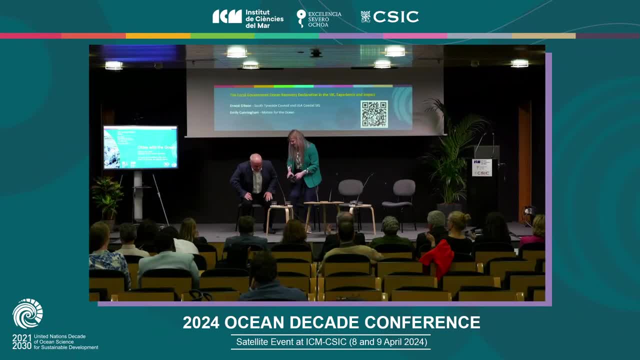 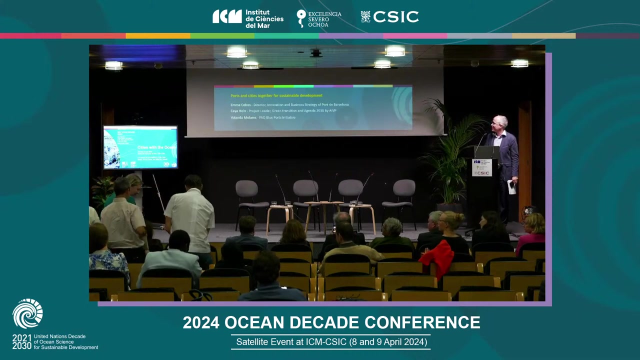 Thank you, Thank you, Thank you so much. We've already heard a lot from CEC. Let's now take a look at ports and how they also contribute and are key players of the sustainable development of coastal territories, And it's my pleasure to welcome now Emma Cobos, who is from the Port de Barcelona here. 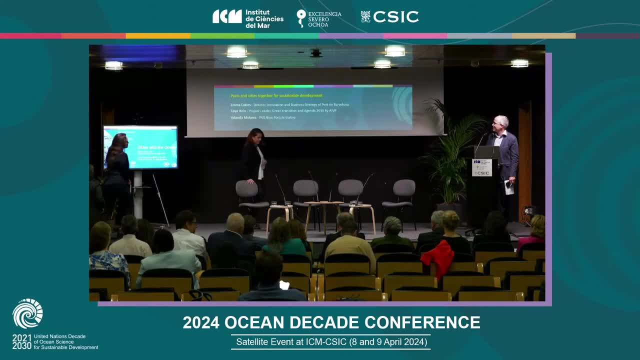 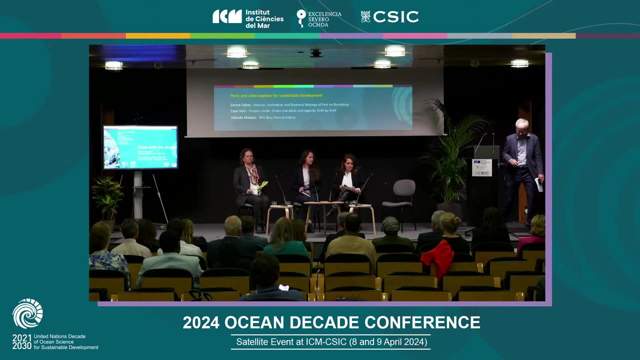 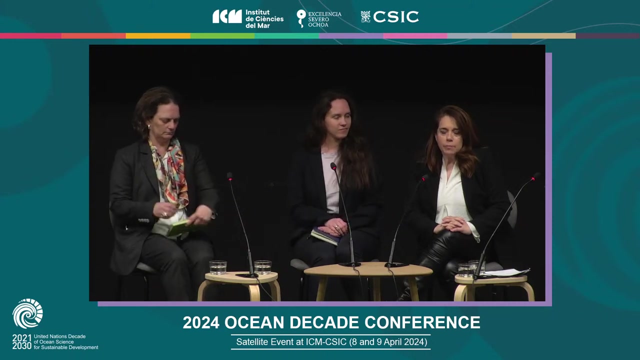 Director of Innovation and Business Strategy, Kaya Hein from the Association of Cities and Islands And Yolanda Morales from the FAO. Maybe we can start with Emma, All right? Thank you, Olivier. Good afternoon everyone, From the Port of Barcelona perspective. maybe I would like to speak more on behalf not only of the port, but also on behalf of the city. 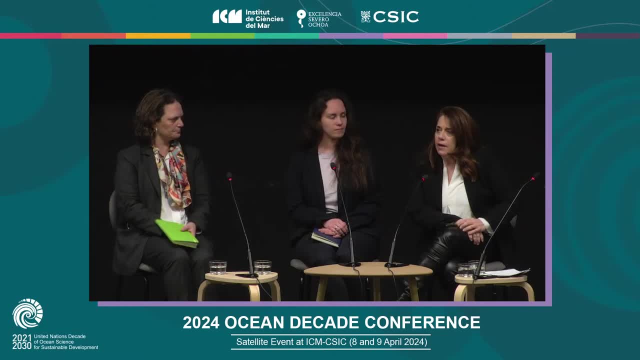 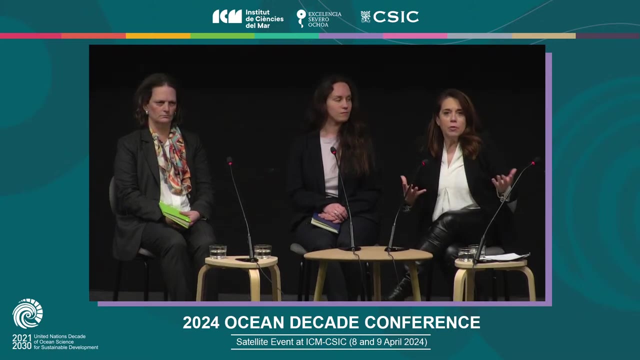 Thank you, Thank you very much. From a political perspective, I would like to speak on behalf of the city. We've had a blue economy strategy now in place for some years And we've been developing several projects, And I think this is for me, this is a strong statement. 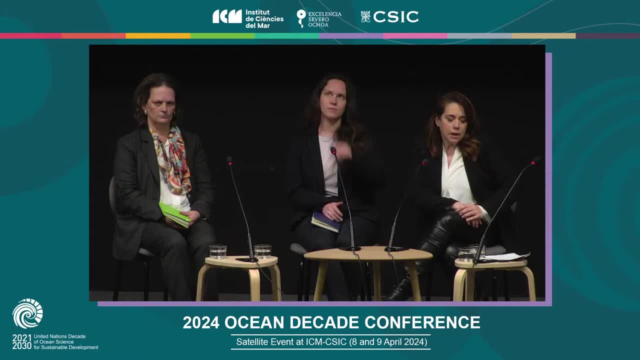 Because, no matter what political parties are ruling- the port or the city, or even the regional area, the Catalonia area, the Catalonian government- we have an understanding of how to do that And we have a strong commitment to do that. We have a strong commitment to do that. 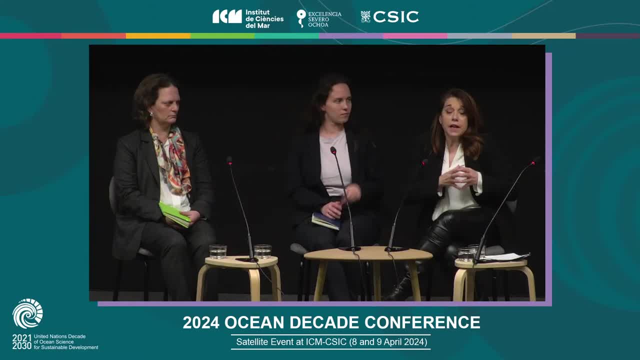 And I would like to speak on behalf of the city, Catalonia government. we have an understanding in blue economy And this is- I think this is a powerful thing. Actually, I think this is something we've been talking within the platform with Olivier for some time now. 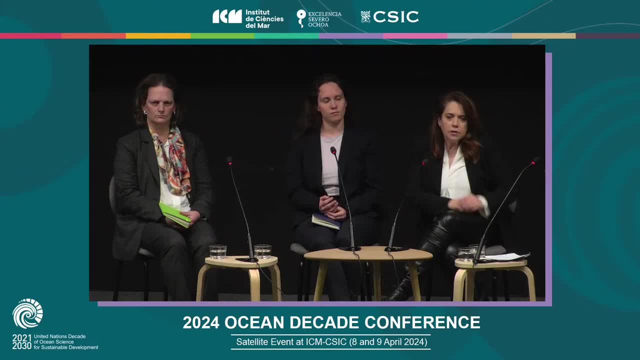 And I think this glue among these three main actors of the blue economy is very important for the Barcelona city and for the region, And maybe this is also part of why this event, this very relevant event of UNESCO, is taking place in Barcelona this week that I'm very proud of. 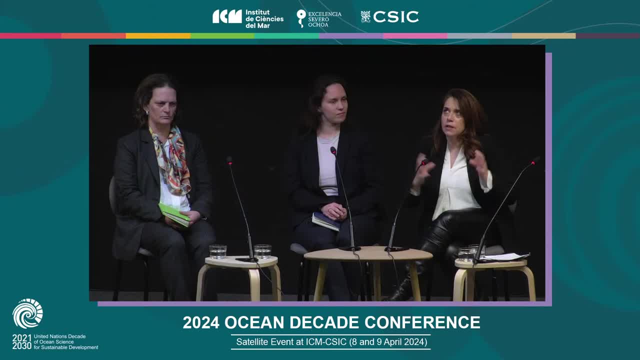 If I have to mention, maybe, a project that has brought us together, and it's a very small project, but I think it's easy to explain and it's very easy to see how useful that is. Not only is it very useful, but it's also very important to see. 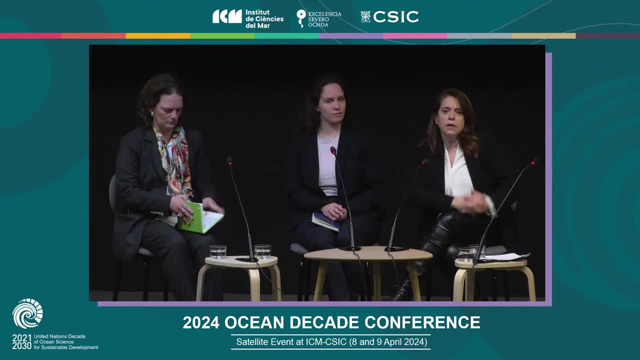 how useful that is. Not only is it very useful, but it's very important to see how useful that is. Not only is it very useful, but it's very important to see how useful that is, Not only for the port or for the city, but also for the. 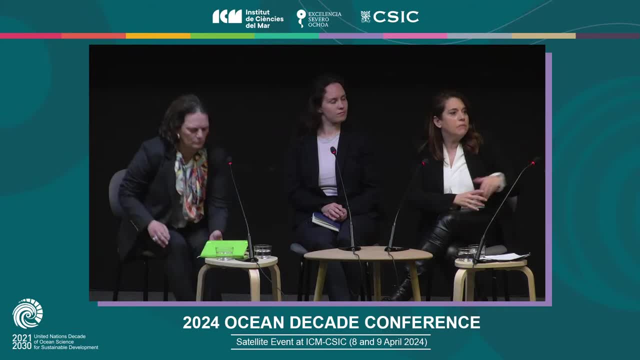 citizenship, because we cannot forget- and I think this has been very clear today- that we need to deliver a big message. We need to deliver outcome to the citizens. So this project we've been working on the port and the city, together with the EU commitment with- I think it's- 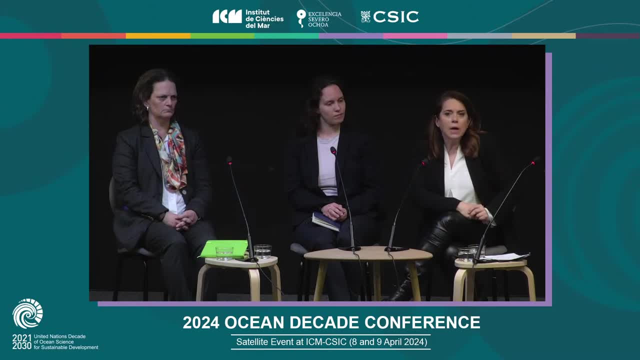 12 million euros of funding by the EU and 16 countries are involved. But basically the pilot has been going on in Barcelona is we have installed some sensors that are controlled on a satellite level to do an observing, forecasting and then simulation work over oceanographic issues. 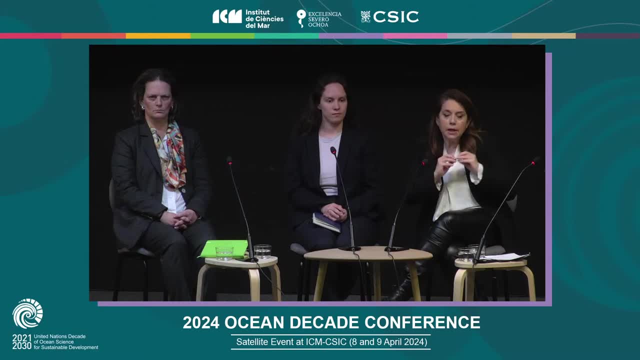 That means we're observing now, in a common platform with the city, sea tides, current and sea level In a framework of climate change. that is, for a city like Barcelona, really relevant And, as you all can imagine, the sea doesn't suddenly stop when. 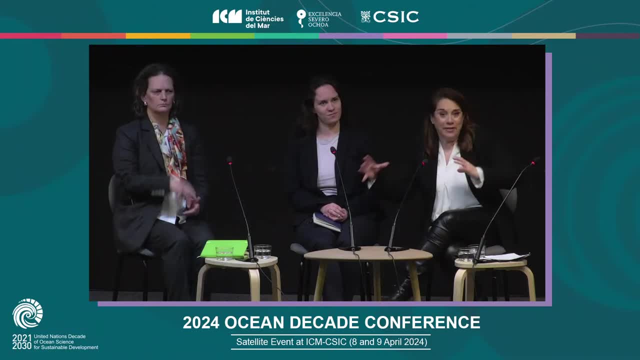 the port is over and starts another sea when the city starts on the coastline. That means we need to work together in such projects, observing the data, taking the data, sharing the data. Believe it or not, we share coastline, but we haven't shared. 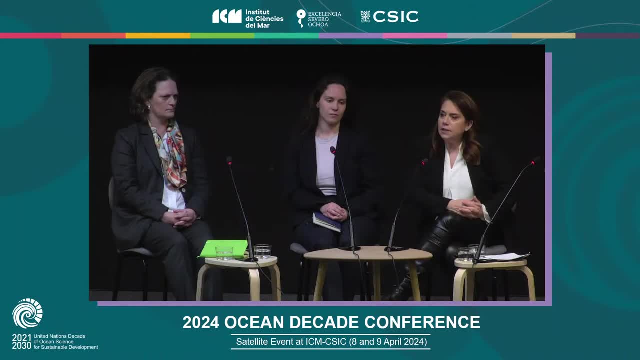 that data at this point. So, with this project, this has been a very enriching experience, And the OSPAC- this is how it's called- the OSPAC project allows us to do maintenance work when we have torrential rains in the Mediterranean. 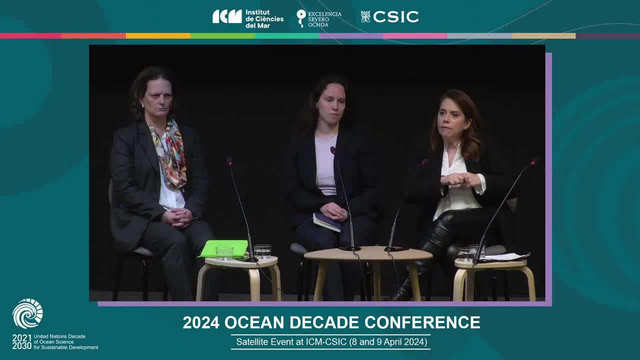 This is very often, Or when we have some sea level rising issues with our infrastructures, not only for the port, but also for the beaches within the city, It's quite important to have a platform like OSPAC. So this is a very small project, but I think it can illustrate how 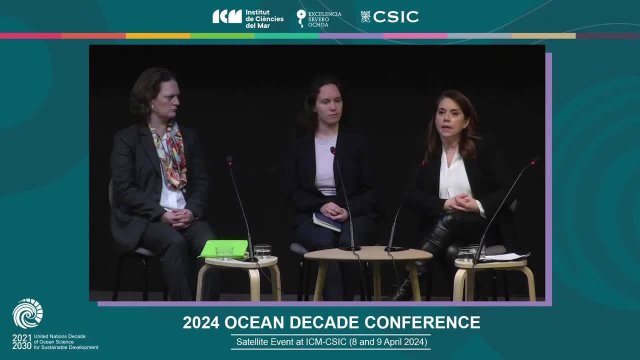 ports and cities can share and can go hand by hand in blue economies And I think it's really important to have that kind of sense of shared responsibility for the economy projects. Thank you, I will take the word now. So the AVP for any of you who are not aware of us, is the. 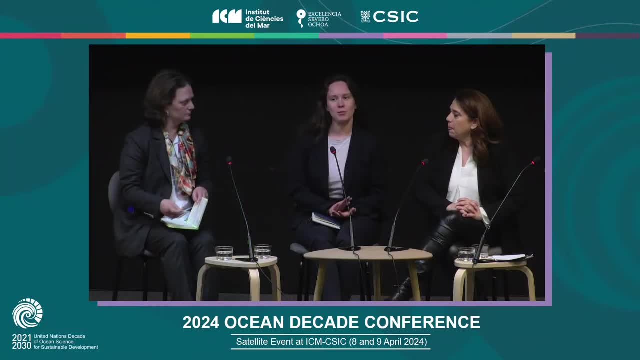 International Association of Cities and Ports, And I would like to highlight this again: cities and ports. It's one of the key messages that we really wanted to get across with the Cities, with Ocean platform is that all actors, all stakeholders who are linked to the ocean, especially 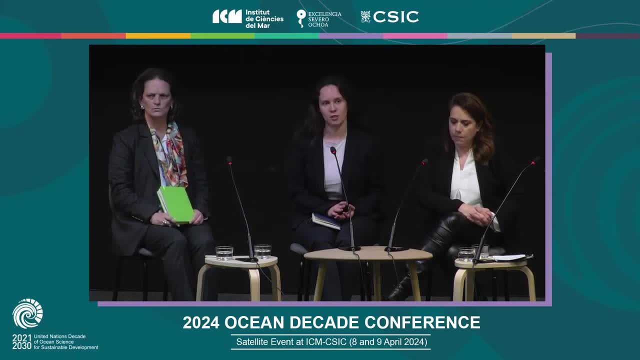 in cities or close to cities need to be at the table to discuss ocean literacy and ocean science. So, as Ms Kovos or Emma just very neatly explained, the port is also a huge actor in the city's relationship with the ocean. I think that we can all agree that, although we might not want, 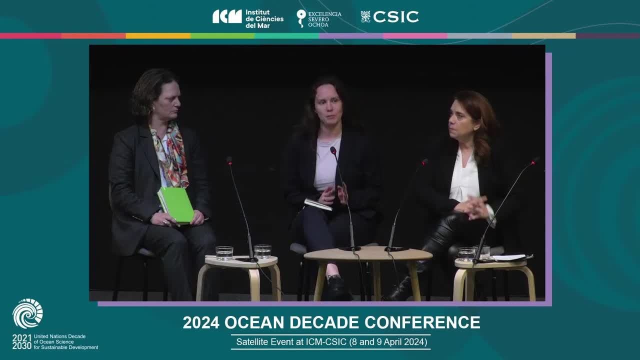 to hear it. port cities have historically been huge emitters. However, they also have the key to becoming very sustainable and drivers for a sustainable ocean. And then finally, of course, there is the ocean. It's bought into the rights of the economy for the 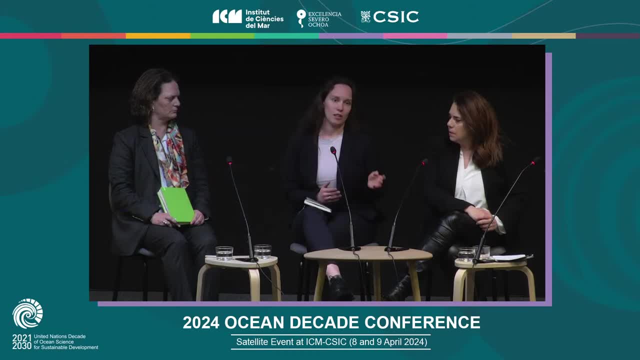 environmental protection of marine life and a lot of other aspects which are crucial. However, in order to do all this, ocean literacy and ocean science is key, So the AVP has encouraged our members, of which I see a few here- and interested in the platform. 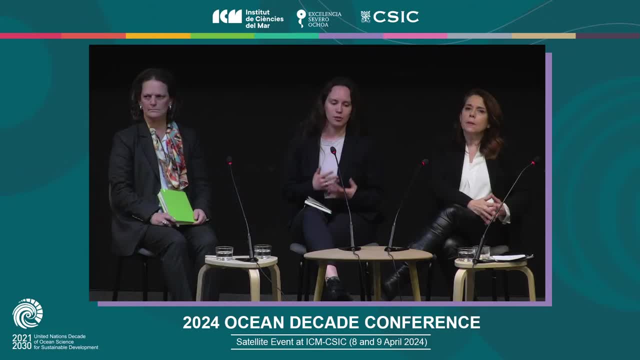 So I'm very happy To develop ocean literacy first of all in various ways. In theory, we have the agenda 2030, Biosphere and Museum, which is not under thecievel. It's a very important topic, So we have a set of recommendations. 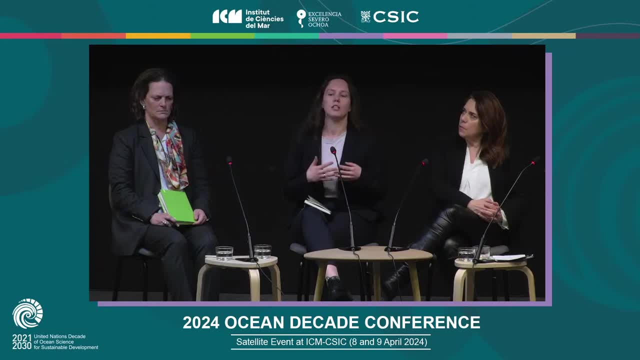 which is based on the UN sustainable development goals, in which the ocean literacy concept is inscribed in several manners: through governance, through human capital, which encourages training of your workers at all levels, and education and governance also in terms of including students and including research organizations in port cities, governance and as well as just in 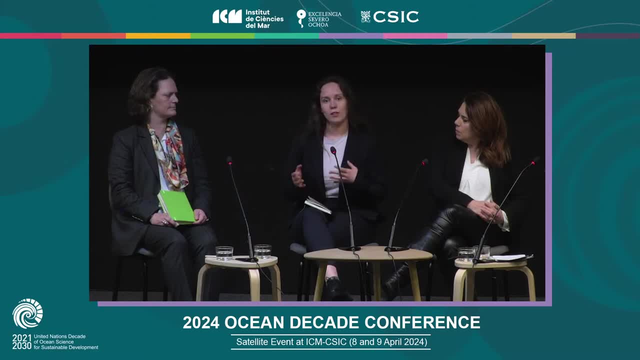 biodiversity and life quality, because in the end, those two are very much linked to anything that is being done, both on a decisional level, but also on an active level every day in a port and city. the second aspect is more in the practical sense, and it's through the port center concept, which has been taken up by 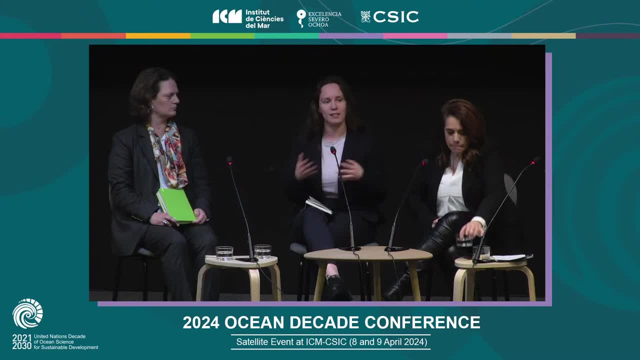 various members and is a concept shared by both the port and the city in a lot of cases, or in the ideal case at least. and in this, in this situation, the port and city come together in order to increase ocean literacy in their local context, for their citizens. so how is the ocean impacting the port and the city? how is 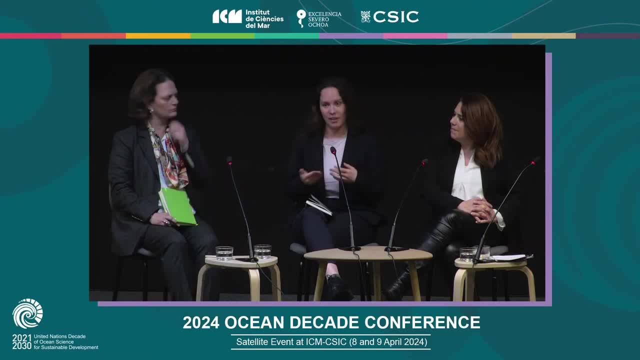 the port linked to the city? how is the industry linked throughout the port and city? so all these subjects which are key to understanding the ocean and how it impacts or is impacted by us and impacts us, are explained there, and it's a place also to discuss on how to move forward and how to advance. so this is one. 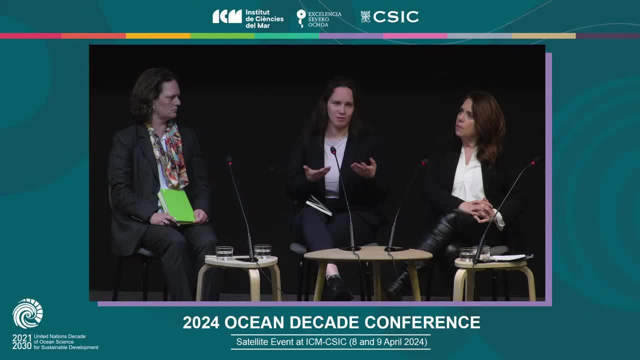 concept that we're very proud to have brought and to show the ocean literacy importance to us. the other is, on a more local and port authority level, to have courses which we- which we are proud to have as well- and which advance the ideas of understanding the linkages that I've just mentioned on a higher level, on how the policies. 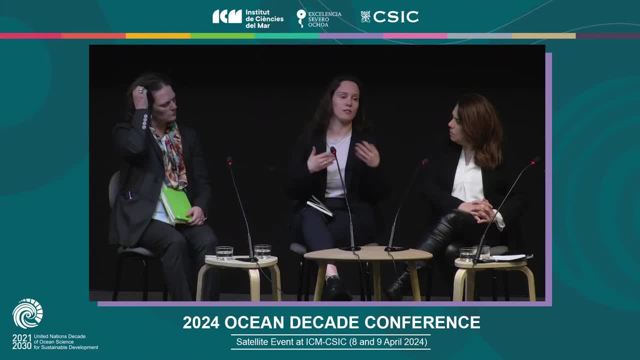 impact these on how the actions on day-to-day, but also in the visions for 2030, 2050 or whenever, can impact this as well. and on the second part which I would like to mention. I know I don't want to take up too much time, so I will. 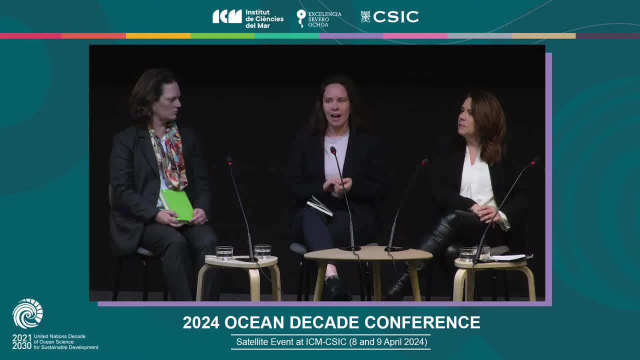 very quickly is that our members are very active in terms of ocean science and what we think the cities with ocean platform can really help- and this is why we're given our support- is the fact that, although our members are very active, it's often still quite locally and sharing these good practices. putting 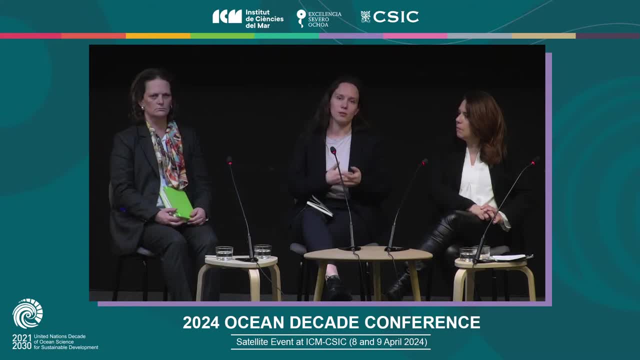 people in contact with the correct ocean science experts is very important. so we have various examples of Port of Barcelona- and the city of Barcelona are one- but various examples with innovation hubs where the ports and cities are together often to support innovation, especially maritime innovation, in terms of getting ocean science. that can really help in terms of decarbonizing, in terms. 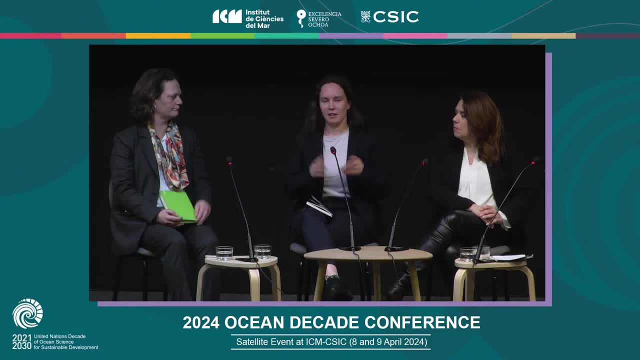 of deep polluting the ocean and and in various other ways. some, to just name a few, just name drop the Port of Lisbon, for example, and the city of Lisbon, Halifax, with the pier, all to see in Los Angeles, sorry, and many more that are currently not coming to mind, but I think it's important that we have that kind of 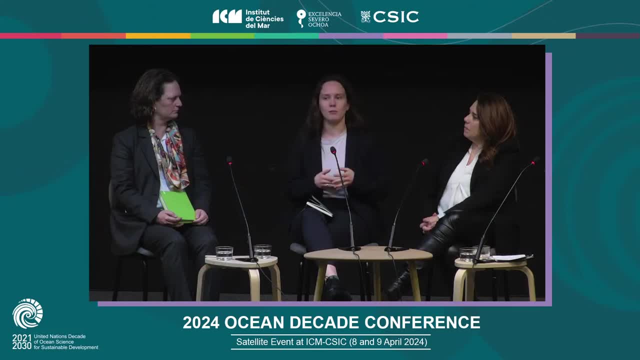 I don't want to take up too much time, so what I'm saying is: the city with the ocean platform really has a role to play here in bringing contact these key players from all over- not only the academics or not only the scientific community- with the port and city authorities, but also with the citizens. 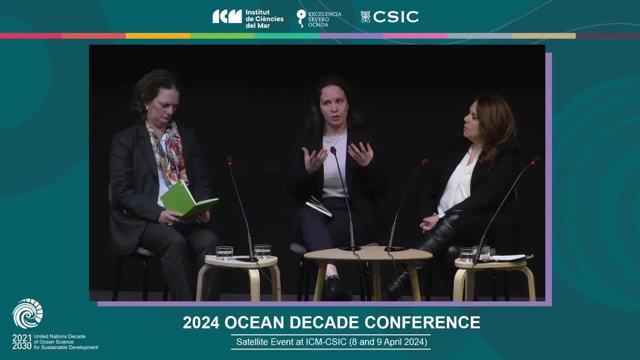 also with the workers, the with, with anyone really interested, because everyone has ideas, everyone who knows the impact that the ocean changes are going to have on them, and then also sharing those solutions so with the rest of the world. so I will now pass on the word. thank you very much. in my Gaia. 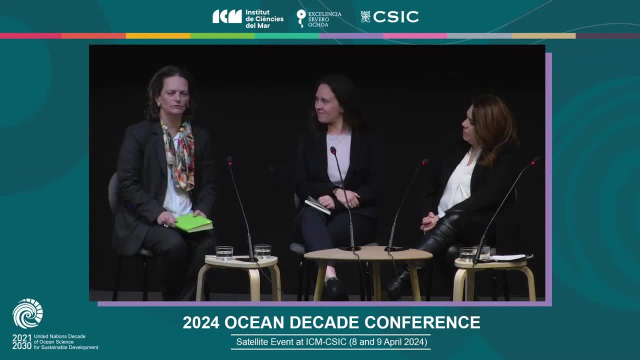 and and. well, I would like to present you on to tell you about the Blue Ports initiative, which is very much in a line with go to a port of Barcelona is doing, and it's very much aligned also on what a I've been doing, in fact I've been. 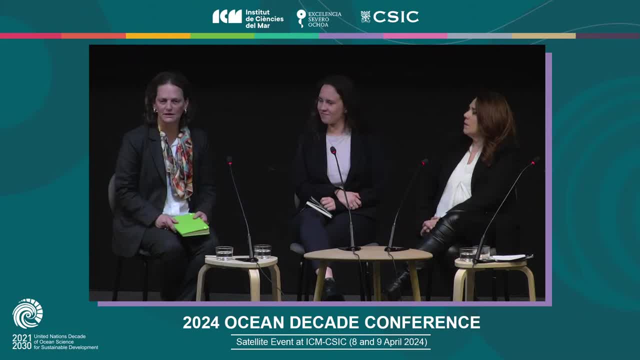 ourselves the Blue Ports initiative. we have been collaborating in many, many times and we've even done some, some activities together, and also Emma, I has has told. so we had the chance to have Emma in one of these, a workshop. we we've already prepared what the Blue Ports initiative is. well, the blue port 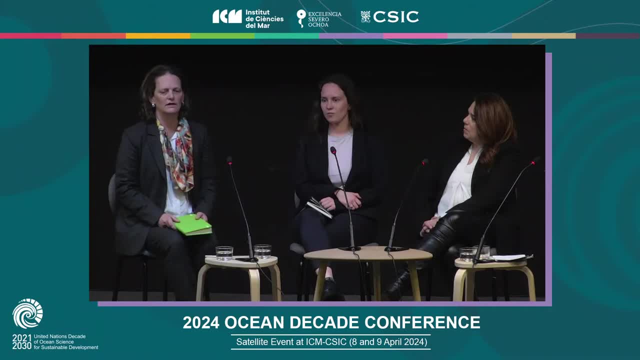 initiatives arises in more or less a 2018, 2019, as will say now, before pandemia, it was just before panamia, would have like two words now. it was just before panamia that in every year we were starting to think: okay, we have. 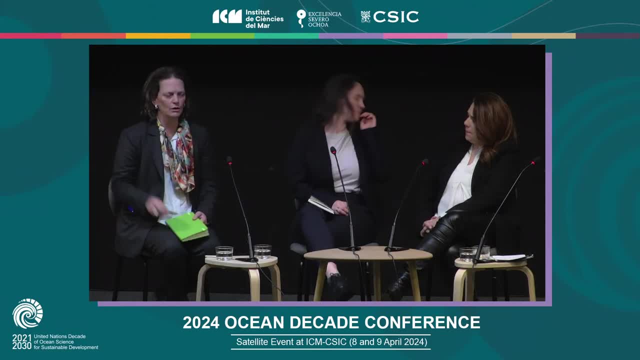 ports. we have fishing ports because of the climate change and also because of we are fao. we also have cities. there's an interaction in there, but also a beyond that interaction. imports have a big, big power, a big potential of creating value. creating value for itself. activate- and when you say for itself, you are saying without any doubt for the city itself. 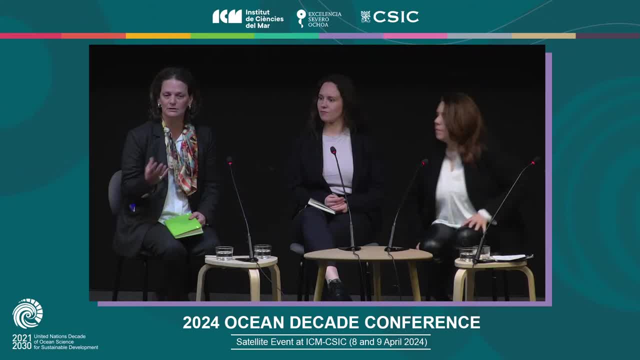 and it is a relationship that we cannot separate because we believe that is exactly the same thing- port and a city, whether the difference is. the difference is on the governance, yeah, on where the government is on. sometimes a well, sometimes not always- the governance of each of the entities are are different, but they should collaborate and work together and this is what 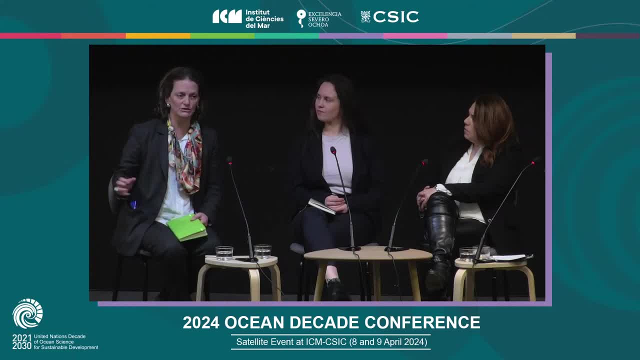 the blue ports initiative is about. it is about collaboration. it is about understanding how we can help road ports, fishing ports, to to be blue transform, as in fao we say, and how we can help them to understand what the role is in terms of environmental, social, economics and also governance. for that the blue ports initiative- nowadays we have the collaboration. 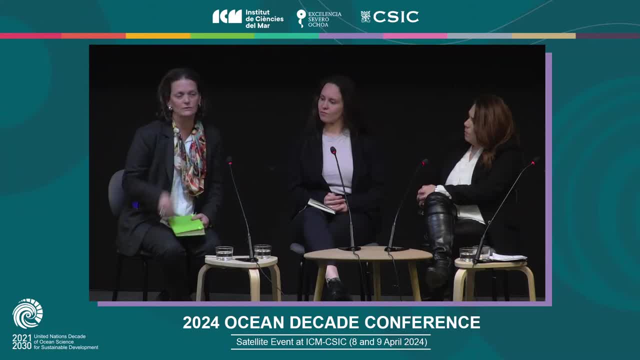 of in asia, vietnam. i'd like to name them because some of you of the countries are here today, but in in asia is a vietnam, indonesia, a thailand, philippines, china, korea, india and sri lanka. today in africa, we've got in morocco's collaboration and we also have a cabo verde. 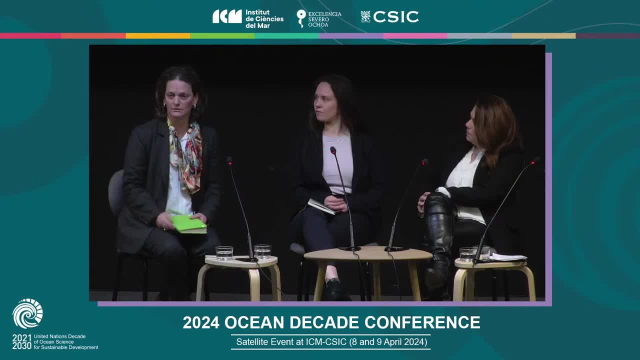 and kenya- and one colleague is here- and also a mozambique in america latina, in latin america we have central america, the seven countries through the sika region and also colombia, ecuador, peru and argentina. in the last we had brazil as well, so i hope that from today we continue having brazil. 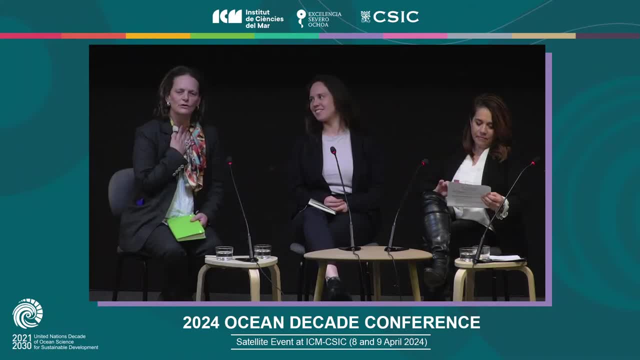 okay, what do we do there? what we do, first of all, is something that we believe it's very much in interesting is trying to understand and to learn from ports, from pc imports. what are they doing in terms of each of the in blue transformation on the agenda 2030 dimensions, and for that we do a. 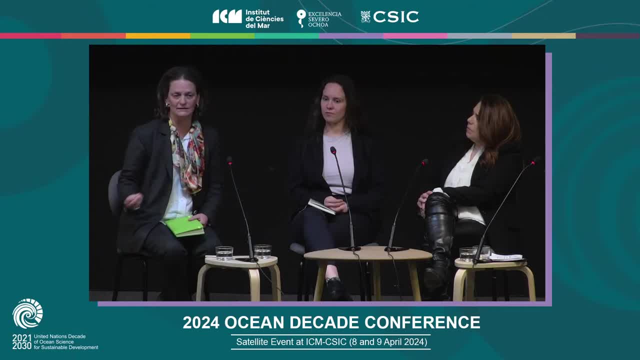 big effort on good and exchange of good practices. i will let you know some of them right now. the secondly is action. yeah, we need action, so for that we need tools. some of the tools are training, capacity building and also elaborating specific guidance that can help all of us. 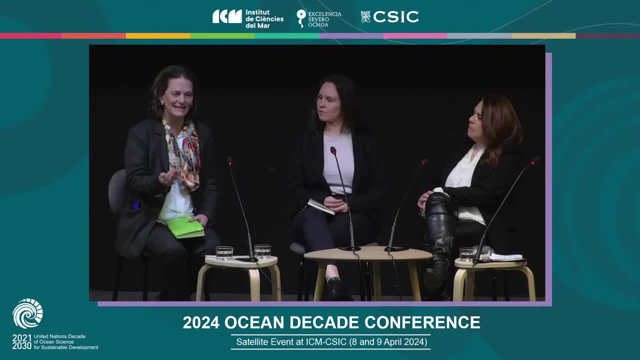 to follow the same roadmap. not to follow, not to do the same, but to follow a roadmap in terms of what we are saying these days, and then projects, projects and projects and and programs. it is very much important that we stop talking and we start doing actions. today is a very good 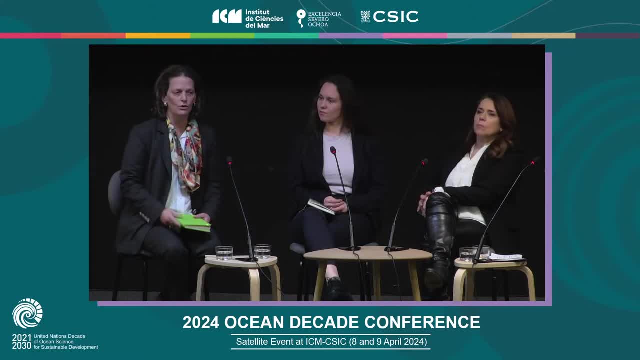 opportunity to learn from many actions, many projects that you all have shared, and i've compiled all of them because they are all very interesting, but what is more important is that we can learn from all of them and that we can learn from them, and that we can learn from them. 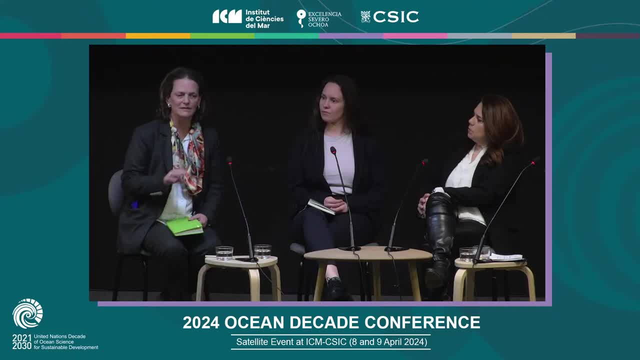 can establish schemes of collaborations. for that, science is essential, but is as important as a government, as important as a civil society, private sector and so on. science is important because we need to create baselines, we need to create and to generate knowledge which is based on something and 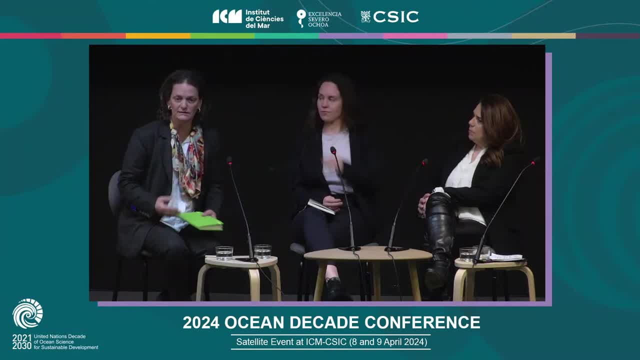 from that and on, we will be able to create wonderful things and to create and generate value, which is what we are looking for. we have three working groups and one of the working group is more concentrated on environment. yeah, an environment, the carbonization, we've already said- a preservation of biodiversity, just. 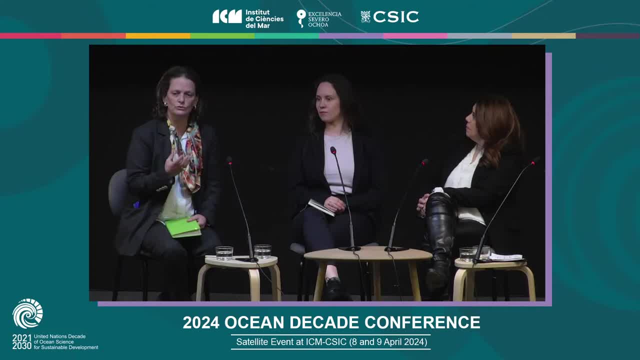 energy. i would like to take some examples just to to consider and to show how we can work all together. yeah, for example, if we take the, the biodiversity, the preservation of biodiversity, we can talk about civic restoration. for that we have some examples, like, for example, the port of 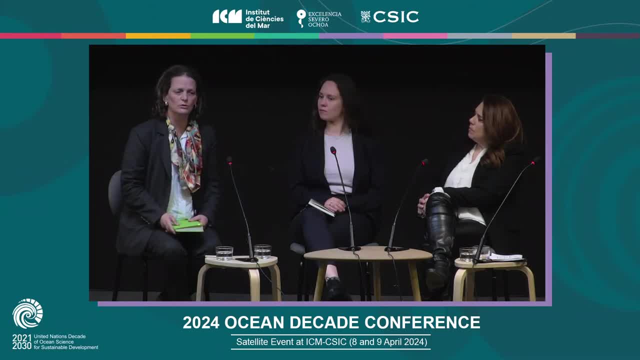 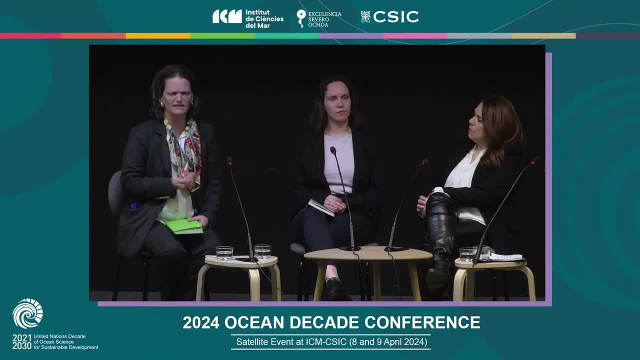 recovering the cvet, and not only to recover the cvet but also to show and to share the results with citizenships. but then, if we are talking about just energy, we can take, for example, the port of mauritius and learn from them how they are doing and implementing a specific plan on energy, on blue. 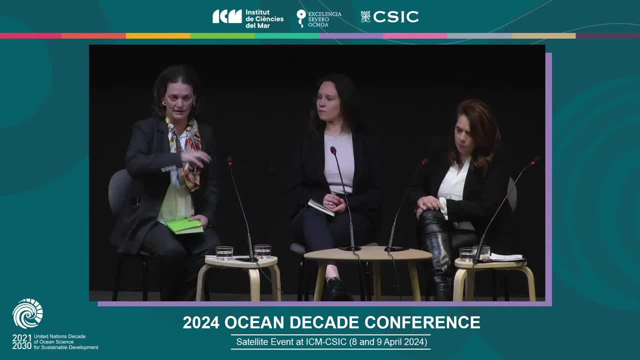 energy, both inland and also inline in terms of port operations, and working on that with the city, but also with the fishing fleet, in order to recover, to analyze a better ways of saving energy and to use non-fossil energy for the fishing sector, because we have four or five. 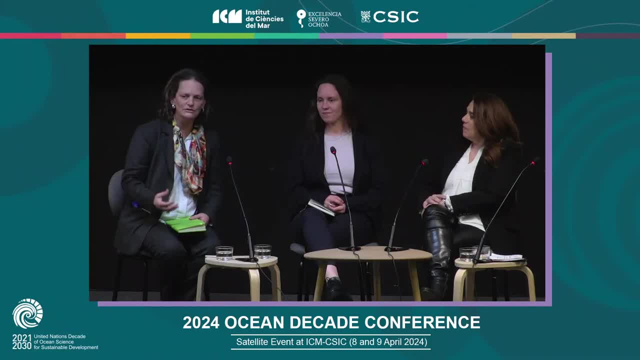 minutes i. i won't continue and just to encourage you to go through all the tools that are online and just to to create team, to continue working as a team, as, for example, this platform, to continue adding up. Nothing should step others, but complement. 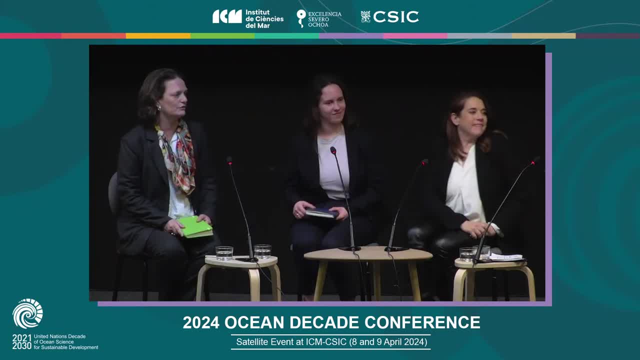 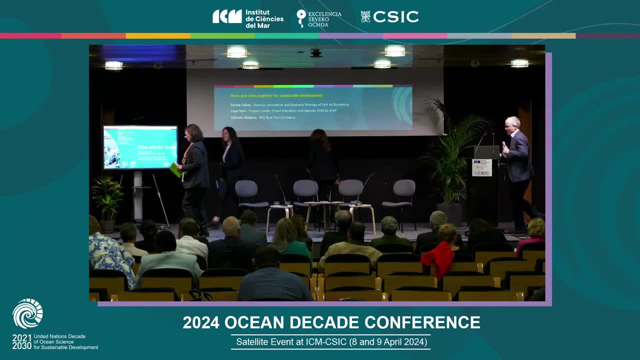 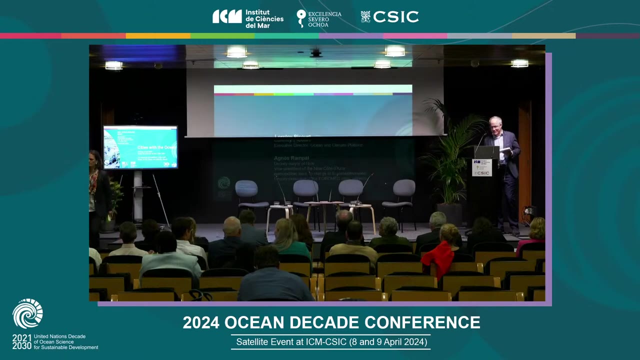 So thank you very much, Olivia, for this initiative, and to all of you. Thank you, Olivia, Thank you. We'll really need to run through the final part of our program today, so I invite Kate Strachan to join us. 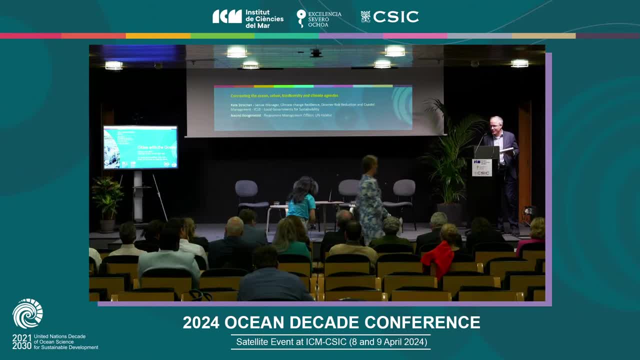 and she'll tell us about the connection between the climate, biodiversity and the ocean agendas. Please give us a brief presentation, Okay, so I'm gonna stick to my notes, so that can be brief and I can try and mix some stuff quickly. 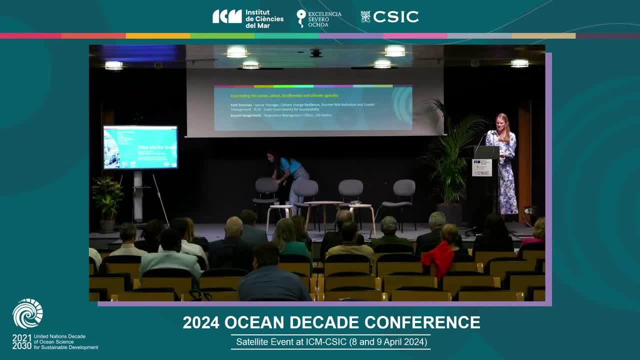 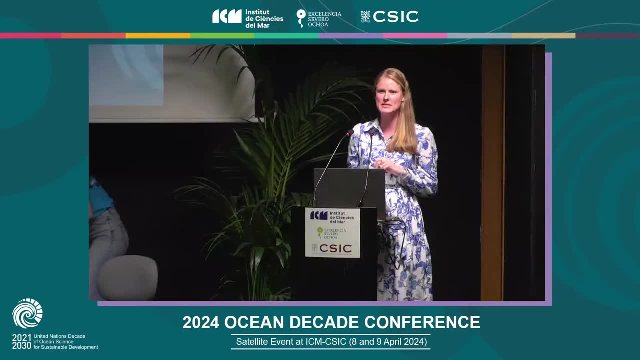 because I know everyone's getting tired, But I'd like you to sit there and just picture a world where the health of our ocean is intrinsically linked with the resilience of coastal cities, where the vibrant tapestry of marine life thrives alongside our marine life. 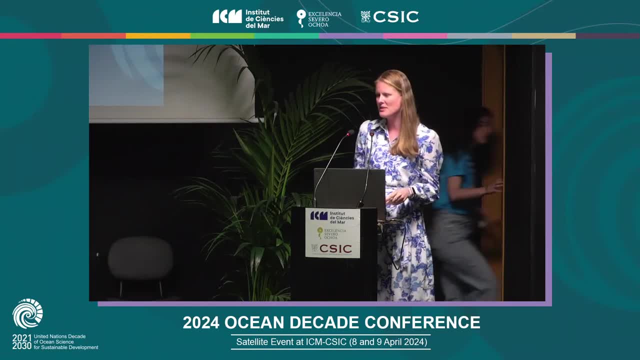 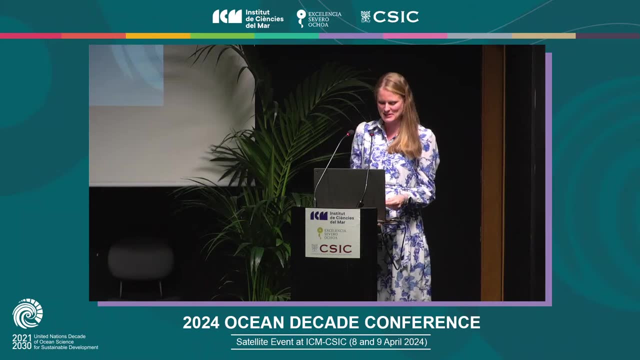 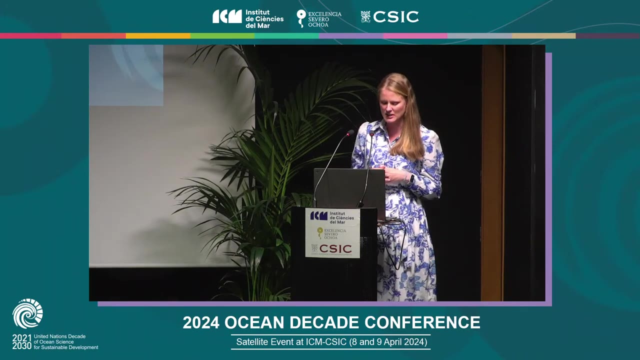 our thriving urban landscapes, And this vision is not a distant dream, but a tangible reality within our grasp. So today, as Olivia said, I stand here to illuminate that path towards this future, a future where climate change resilience, biodiversity preservation and ocean health. 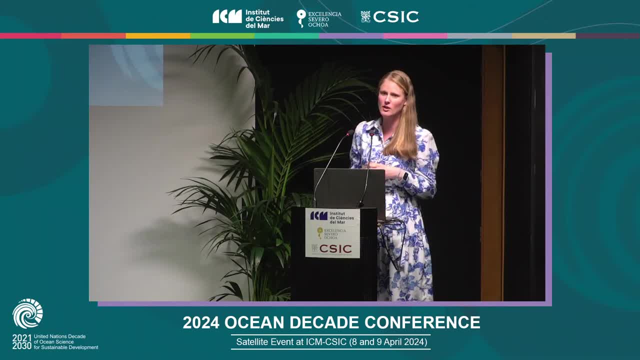 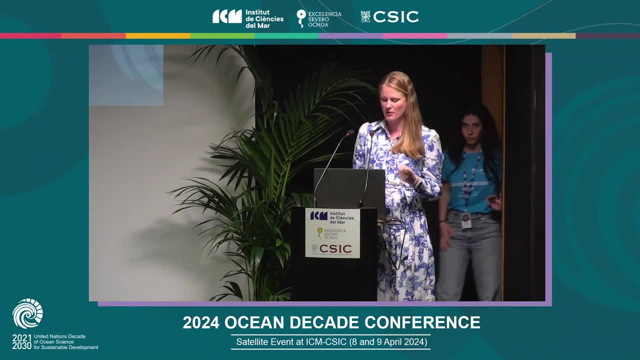 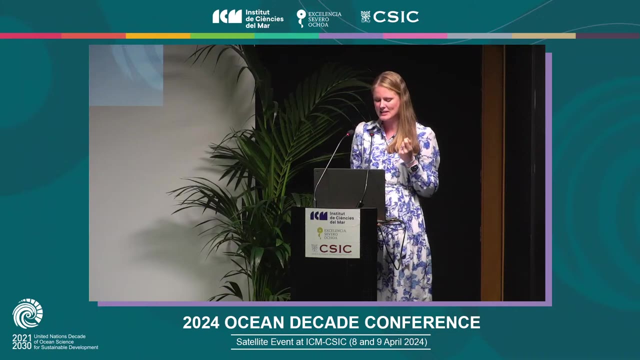 intertwine seamlessly, which is empowered by the pivotal role of our cities. The challenges we face from climate change, the relentless onslaught from climate change, the alarming decline in biodiversity- are not isolated phenomena, but crises that are interconnected and demand these integrated solutions. 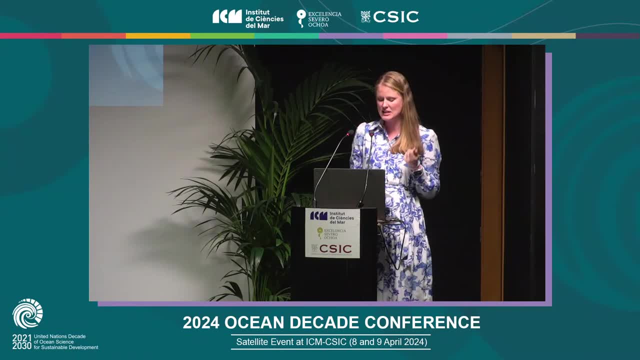 Our ocean, which is a vast resource, stands at the linchpin of this interconnectedness, regulating our climate, sustaining life and nurturing biodiversity. So it's imperative that we recognize the symbiotic relationship between climate change resilience, biodiversity and ocean health. 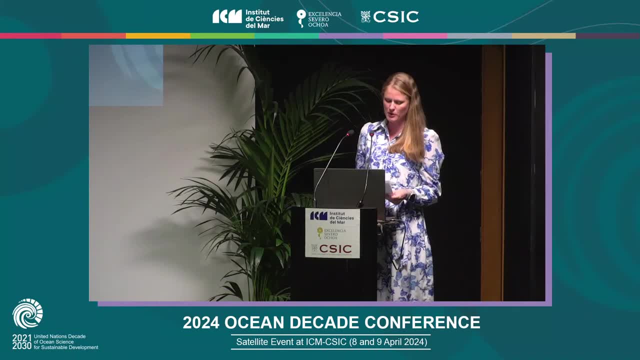 They're not different from each other, They're not different agendas, but rather they are pillars upon which our collective well-being stands. So we need to. we can't just address one aspect, but we need to address all three, integrated, using integrated approaches. 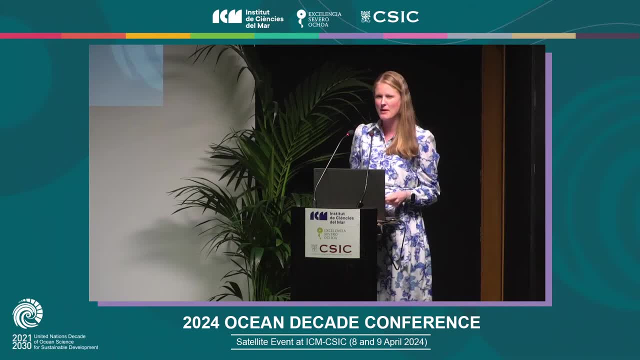 So empowering cities is not merely a matter of rhetoric, but a strategic imperative. And cities are at the epicenters of human activity, the engines of innovation and the crucibles of progress. They are where the battle against climate change and biodiversity will be won or lost. 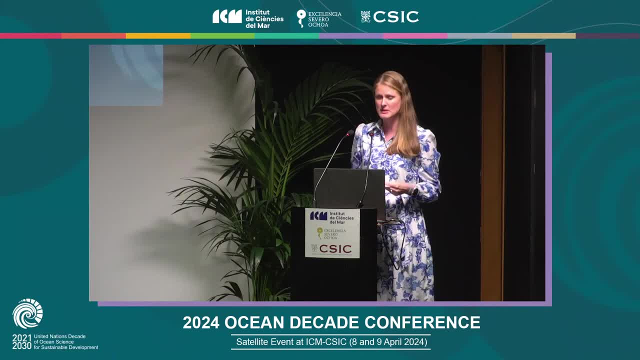 So for cities to fulfill this potential and be these agents of change, we need to ensure the necessary resources flow to them, And this includes finance, And we need to stop talking about resilience, but we need to ensure that there are concrete actions and investments. 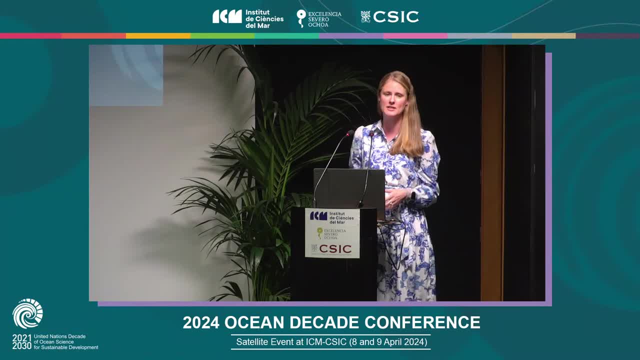 So this is where initiatives and platforms play a huge part And, just to just to put this out there, highlight one is, for example, Cities with Nature, which exemplifies this ethos of collaboration and collective action, With over 300 cities from 75 countries and. 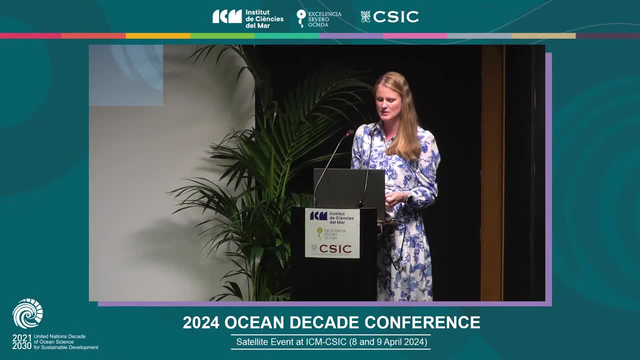 25 partners. Cities with Nature serves a testament to the power of solidarity in the face of adversity. It provides a platform for cities to unite in their commitment to harmonize urban development with nature conservation, fostering resilience and sustainability. So cities like Kochi, Barisiccia, Melbourne. 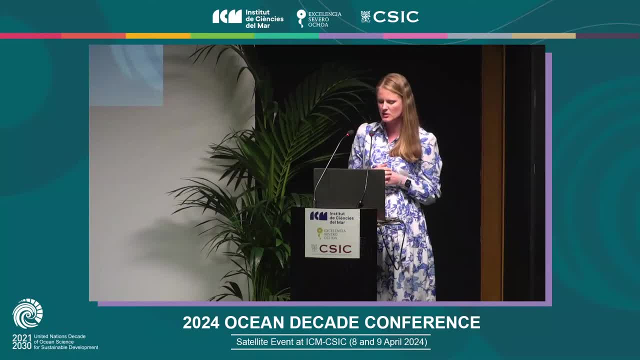 and the city of Cape Town, just to name a few, have already embraced this ethos, making commitments to protect their marine ecosystems and promote coastal resilience. They understand that the health of our ocean is not just a matter of stewardship, but is really about well, as a prerequisite to the 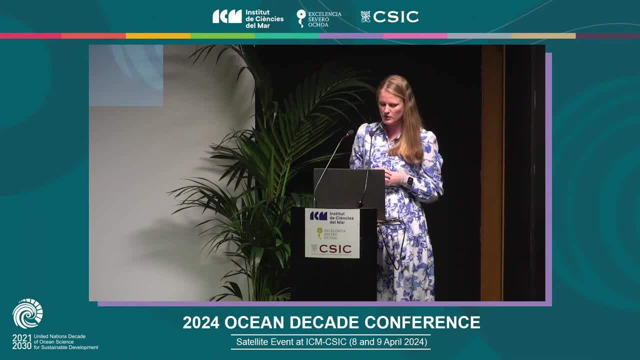 prosperity of their citizens. So, yeah, I'm not going to go into details about Cities with Nature, but these platforms play a key role in also ensuring that cities uphold these commitments and report on these commitments annually. So, for example, Cities with Nature is used for cities to 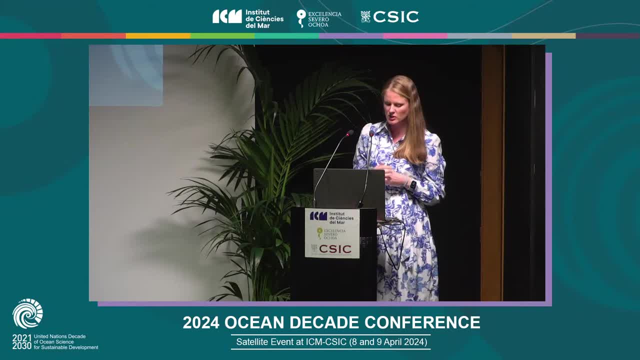 report on the convention of biological diversity, decision 1512, and as well as their commitment to implementing, for example, the Kunming-Montreal global biodiversity framework, as well as the national biodiversity policies. So these are what platforms can be used for and, yeah, as we stand here today and we look to the future, we must 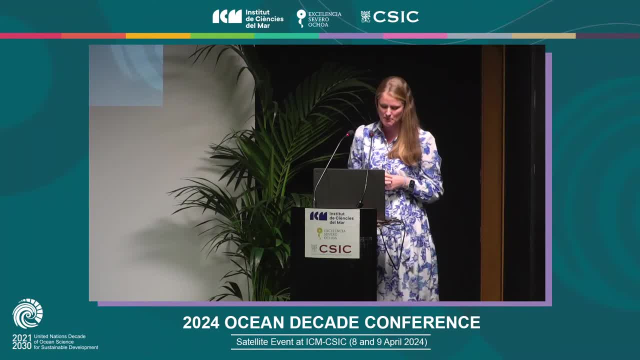 seize the opportunities that are presented by upcoming events, and i'm thinking of the cbd cop 26, as well as the world water forum, the world urban forum, as well as unoc cop 30 next year, as these gatherings, yeah, they offer a really crucial platform for dialogue and collaboration. 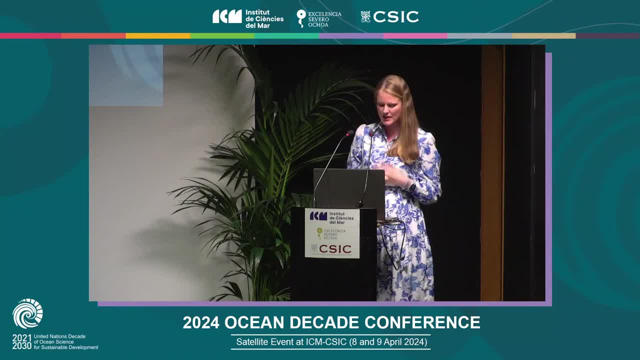 where innovative approaches to climate resilience, ocean health and biodiversity conservation can be shared and amplified. but beyond these speeches and declarations that come out of such events, we must ensure that these commitments made translate into tangible actions on the ground. it's not enough to set ambitious goals anymore. we must provide cities with the tools and resources. 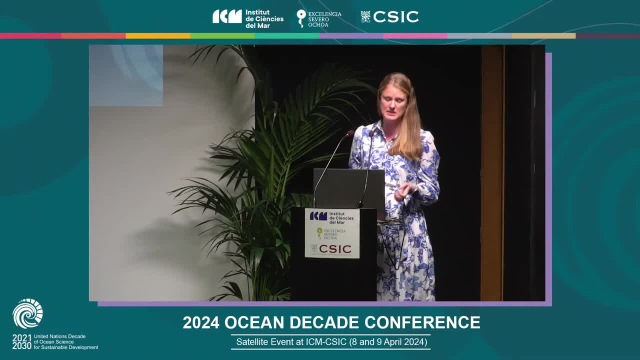 and the support they need to achieve these goals and make them reality. so, from nature-based solutions to innovative infrastructure, the possibilities are limitless, and we need to empower cities to lead the charge towards a more resilient and sustainable future. we pave the way for a world where humanity and nature coexist in harmony, so today, i ask that we stand together in solidarity. 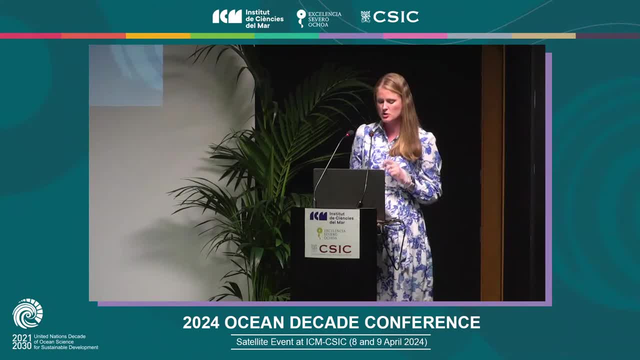 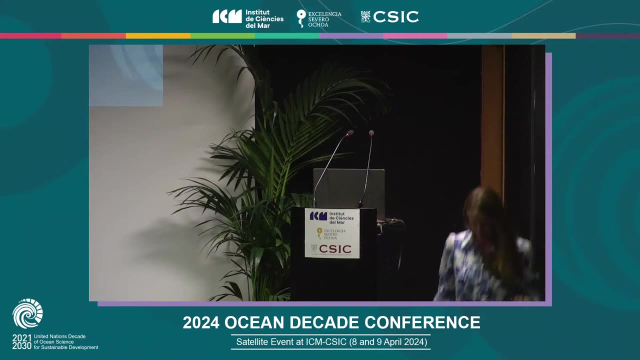 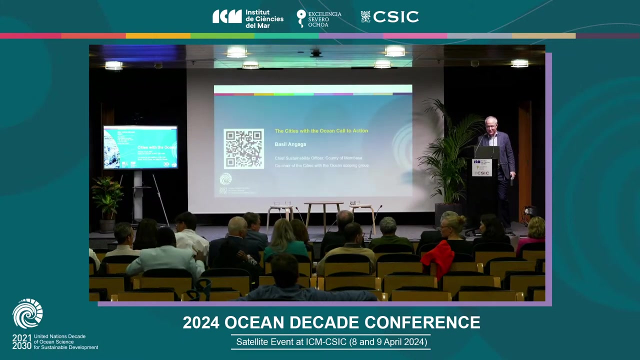 united in our commitment to safeguard our oceans, preserve biodiversity and build climate resilient cities to their together, we can turn the tide on climate change and chart a new course towards a bright future, a more sustainable future for all future generations. thank you very much, kate. uh, now we'll we'll switch to uh basil angaga. i must say that 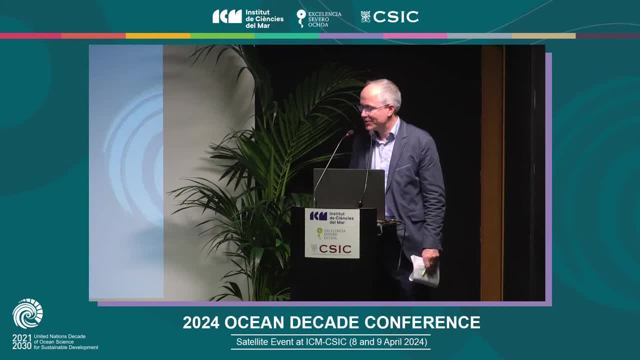 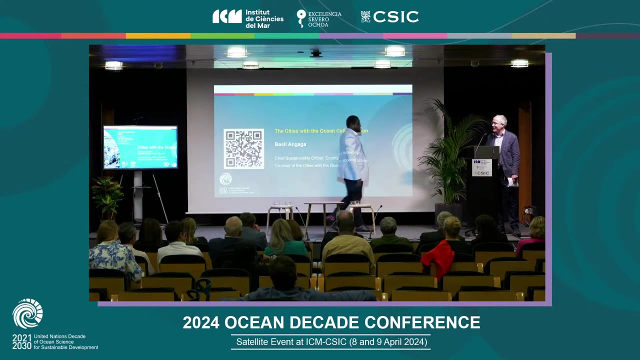 beyond. beyond being the chief sustainable sustainability officer of the county of mombasa, basil has been a great co-chair of the scoping group for the cities with the ocean platform and he'll give you a very brief introduction to the, to the call to action that has been drafted by this group and you can find: 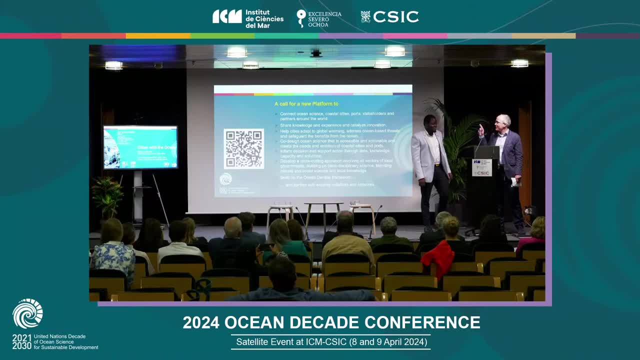 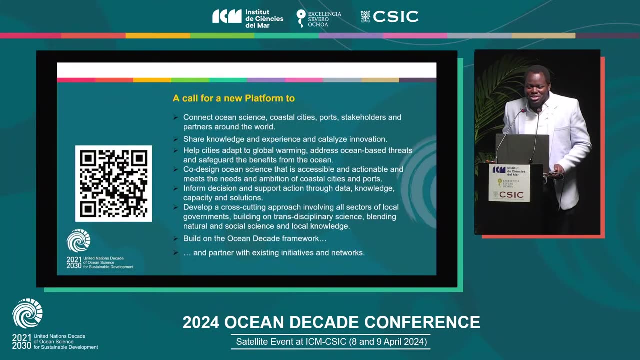 this, this call to action, using the QR code that is on on this slide. thank you, perfect. thank you, Olivia and all of you, for the commitment that you've shown since we started the process of setting up this platform, today that we are formally launching this call to action. I come from a tiny city in the Western 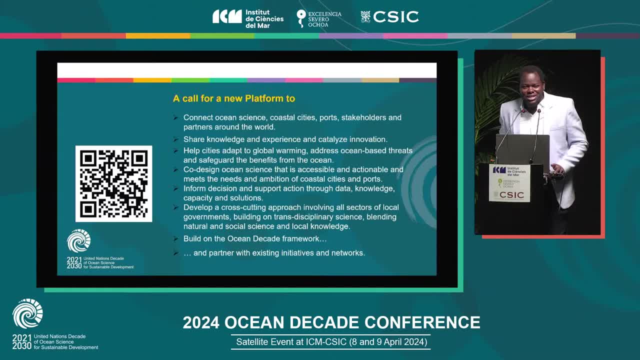 Indian Ocean, a city called Mombasa in Kenya, just 225 square kilometers, with a population of around 1.2 million people and, because of urbanization, we have a floating population of about 2.5 million people. and we have a floating population of about 2.5 million people and, because of urbanization, we have a floating 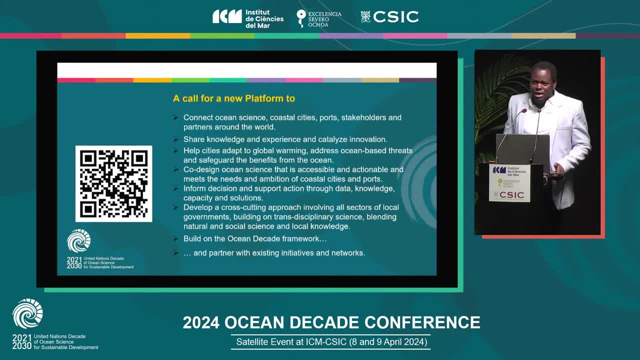 population of about 2.5 million people and, because of urbanization, we have a daily of around half a million people that also come to Mombasa and interact with our city and our ocean, and that is why, when we got this opportunity to come and coach at this process, we were really excited. first, for the continent of 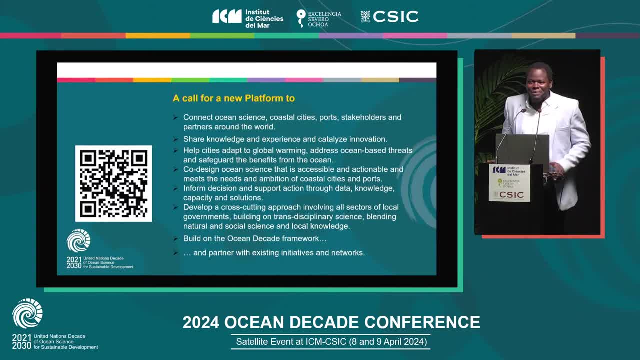 Africa because, as you can see in the room, yeah, so, so. so we say: do it's also part of advocacy to rally the rest of the continent to all also acknowledge and be a part of some of these processes? so Mombasa is leading on behalf of the continent and we hope that this would be an opportunity for the 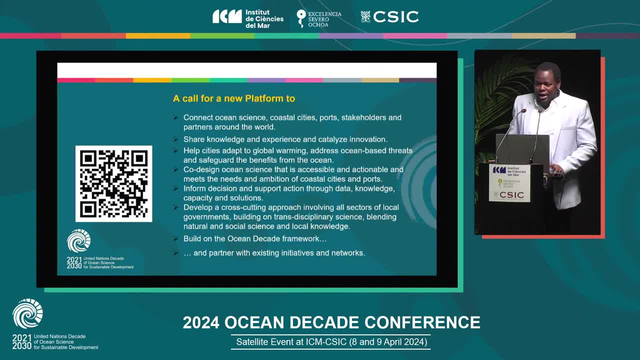 rest of the continent to also come and be a part of this platform. so the platform that we're launching today, based on the collaborative effort and work that we went through together with you to create an ambition that would unite this two crucial communities- on one side, cities and ports, and on the other, the science- 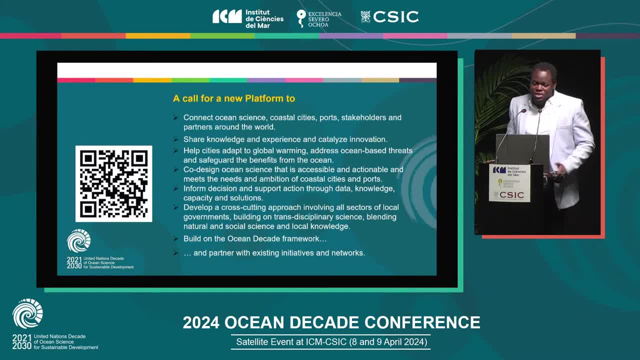 community and the decade actions to just come together and support the sustainable development of our cities. we hope that this platform would, of course, enable all of us to share knowledge and experiences and catalyze innovation and what has been happening here through the through the past couple of years, but I just want to say that we are moving out. 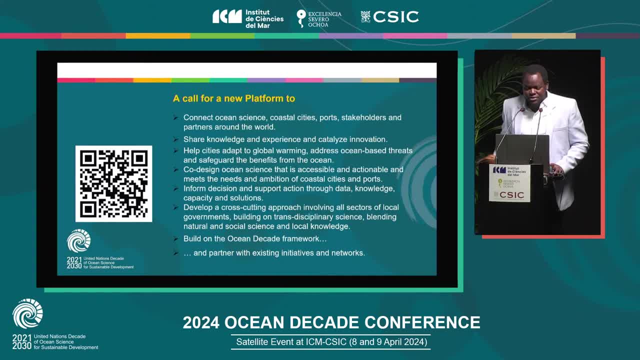 the day is what we envision that would happen with this platform. you see a panel and different players coming in together: scientists, city experts, national government players also coming together to just see how to generate and share a lot of religion. they are speaking here. I could see a lot of similarities with our. 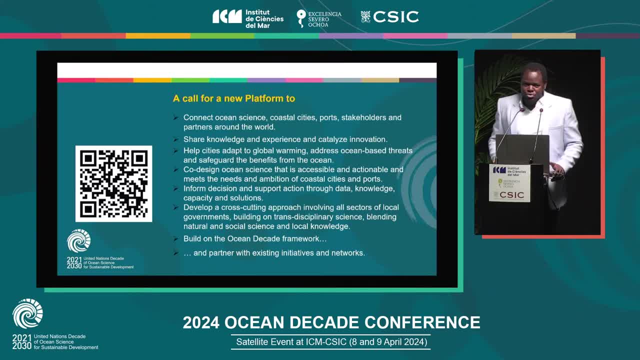 from Brazil to to Bacarana and and, and to Portugal and to all these other cities. so it's a platform that will enable us to share these experiences, so that we also don't get into the risk of maladaptation of maybe some strategies and solutions, because there are people who've experienced them and we're 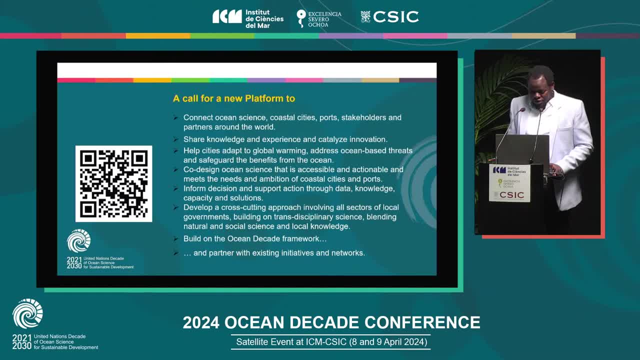 learning from those experiences to build better solutions. and also, more importantly, is the challenge of climate change and the risks associated with it that our cities are become more vulnerable to. so we believe that this platform would help cities adapt and, of course, protect and safeguard the ocean, because we are looking at the ocean as a hotbed of 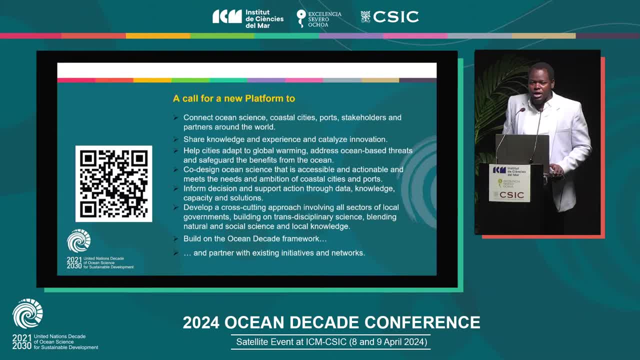 you know of the climate crisis and, of course, we are looking at the ocean as a hotbed of solutions, for climate change could be blue carbon solutions and strategies that could be adopted as well to help these cities become more adaptable to this, the changing climate- and, most importantly, is the opportunity to 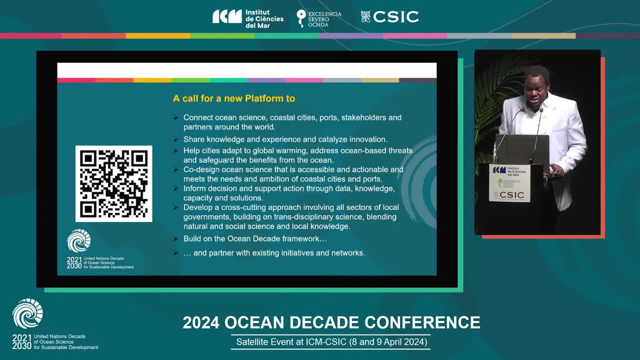 co-design the science that would be more accessible and actionable to these cities. one fun fact that I must also say is that Mombasa is home to the president of IPBS, dr David Obura, and until we read that in the news, we're like: oh so a city hosts such important scientists. they generate a lot of. 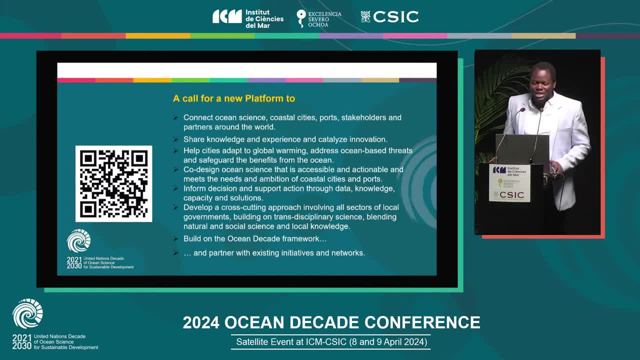 knowledge for the world and we don't take that knowledge as a city. so it's an opportunity to also welcome the science community to come and, of course, help cities or City officials, who are naturally not only the scientists but the people who are actually contributing to the development of the science community. so I'm sure that you'll see that. 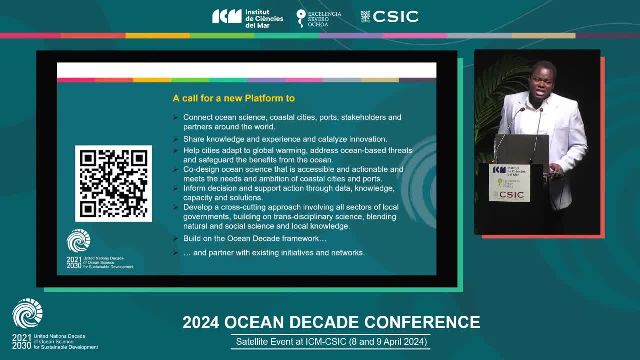 Thank you, ocean scientists to get to understand and appreciate this science when it is generated in collaboration with them. then they're able to see and and also on up to the kind of solution of suggestions that are coming out of those particular processes, but also to inform decision and and for this city to. 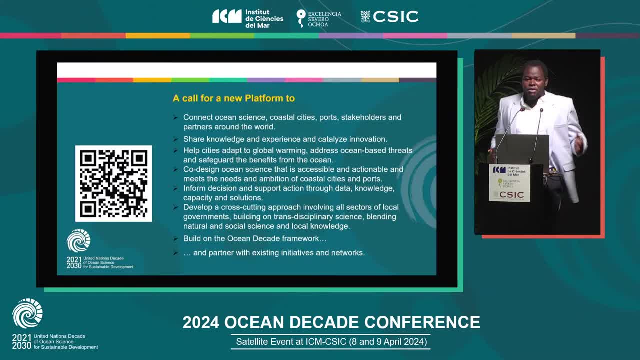 develop sustainably, then that development has to be influenced by data, and and this data will come from science. so so it's also an opportunity to inform these decisions that us, that cities, are going to make, and to also challenge cities to adopt some of this evidence-driven suggestions that are: 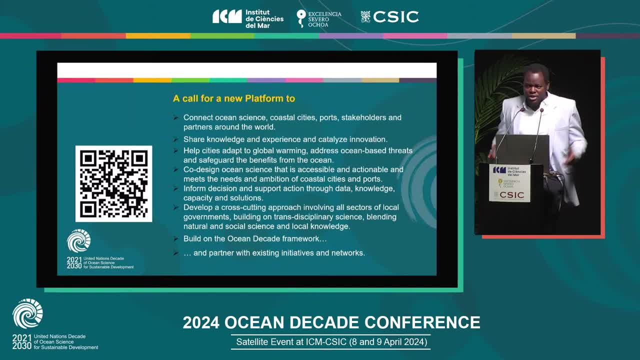 coming from from the science communities and to ensure that development, and this is also data-driven. and then we also hope- and this is very important because this, this is a multi stakeholder or a cross-cutting approach. it's going to be transdisciplinary and- and if you check the room, you'll find- 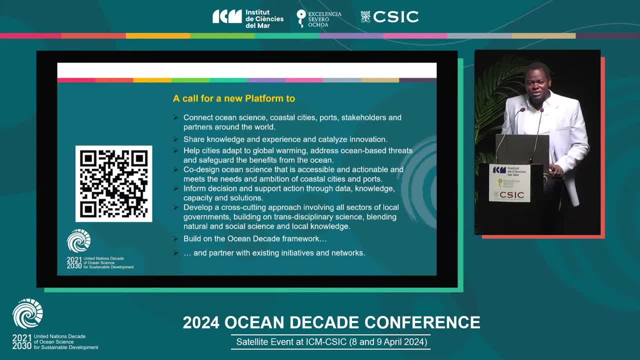 scientists from from different domains, and this is the core of this, of this platform, that we are able to leverage the different expertise that we bring to ensure that you know, we support this coastal community. it is to interact better with the ocean and, most importantly, also leveraging on 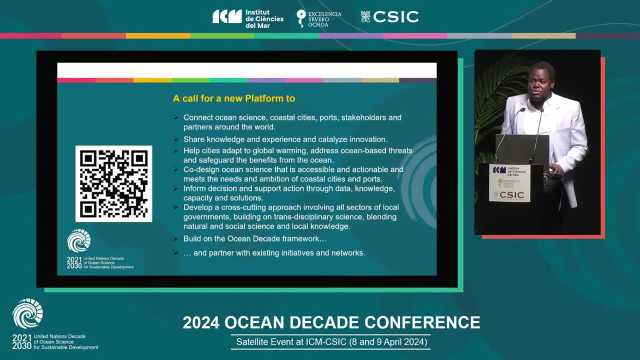 local knowledge, because some of these indigenous communities have also lived with the ocean for a long time and and we have to find a way of mainstreaming some of the knowledge that they've held over the over those decades of interacting in the ocean and also getting to pass them on and 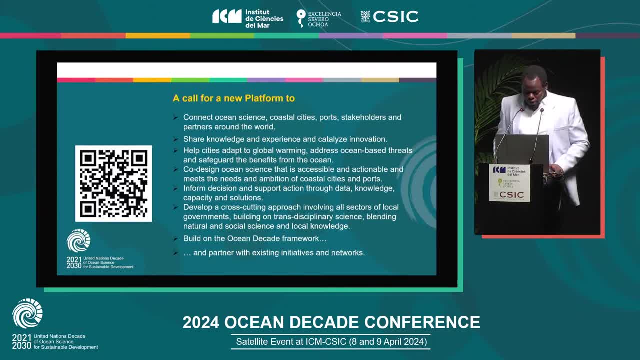 to have it influence the science as well, and then the platform will build on the ocean decode from work, the kind of challenges that we are, the city is focusing on. of course, there are naked challenges as well, and not to duplicate what are the networks and initiatives already doing, but to find synergies and 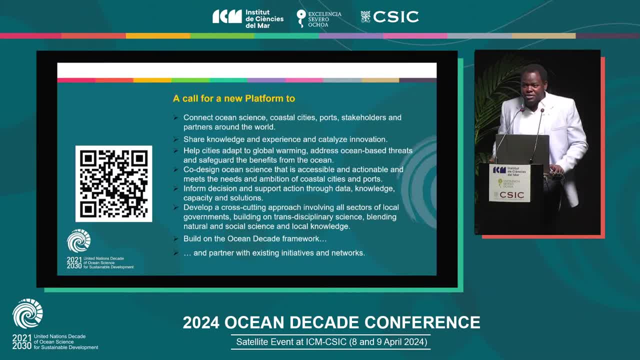 ways through which we can partner with initiatives like maybe now, equally- and I will just make a quick note that the work that we are doing with this is three times bigger and that is because of the work that we are, that we, what the ports are doing, and and the foul blue port initiatives as well, and others to 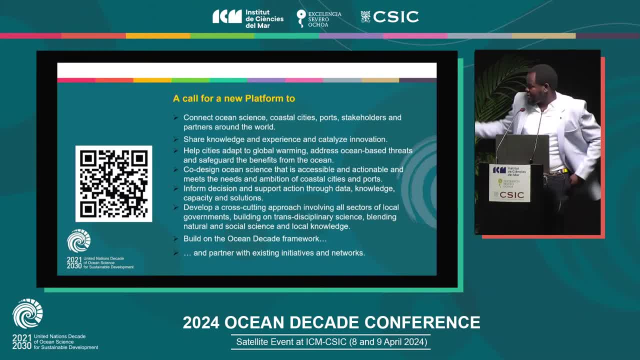 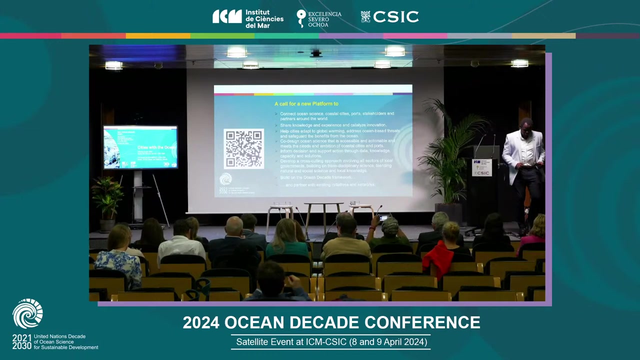 just ensure that we get to build synergies and not to duplicate our work. that has been done, so the call to action is: live on that keyword code. you can access it there and it's now open to more cities and more partners to join and cleaner, healthier and a more productive ocean for all. thank you, so thanks Brazil. 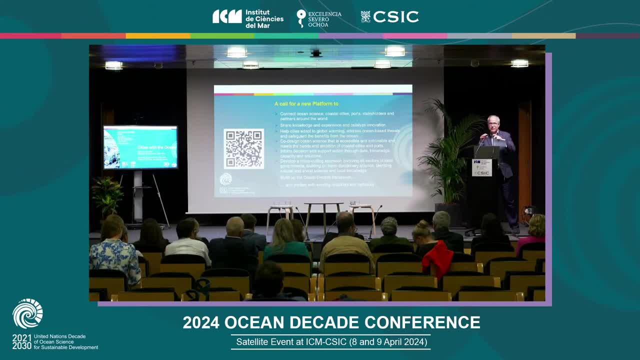 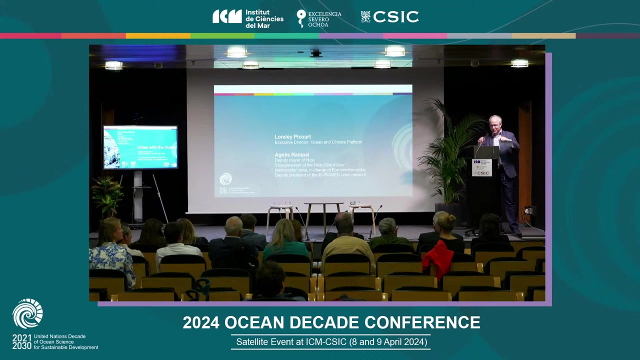 our last speakers for for today. as we're here already looking at the next steps and the the UN Ocean Conference next coming next year, I'd like to invite Lorelie Picourt and and Agnes Rampal, who is the representing today, the mayor of Nice, Mr Christian Estrosi, and she's vice president of the Nice, Côte d'Azur. 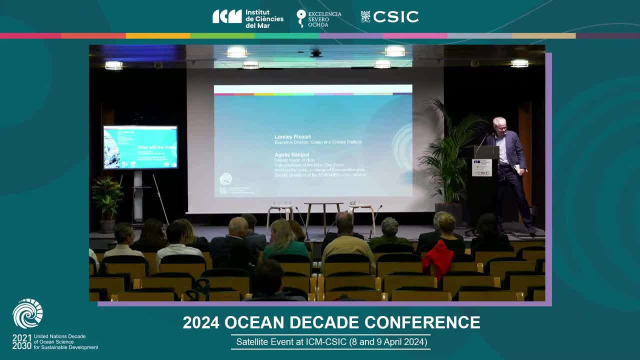 metropolitan area. thanks, thanks a lot. good afternoon. don't worry, I speak very fast, so we'll be good. as mentioned, I'm Lorelie Picourt, the executive director of the ocean and climate platform, which is an international network from civil society organizations working at the interface between science and policy. so how do we boost, as Kate was saying, the 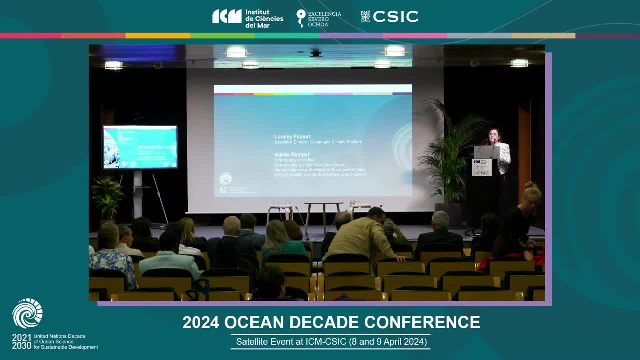 relationship between ocean climate and biodiversity. first of all, please allow me the courtesy of thanking our hosts, IOC, UNESCO. it's a privilege to be here. it's great to kick start the year also with Barcelona, to kick start this with you guys. so we've heard a lot today about the 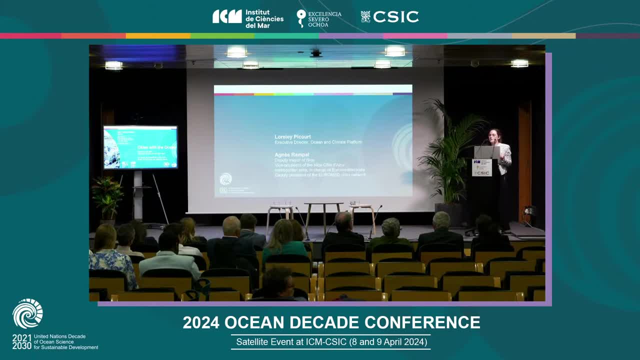 international climate and sometimes very complex relationship that cities have with the ocean. and we know that our coastlines are changing rapidly, that we may reduce and we have to reduce- our greenhouse gas emissions, but sea level rise is here to stay, so we need to start anticipating our reactions. how do we adapt coastal 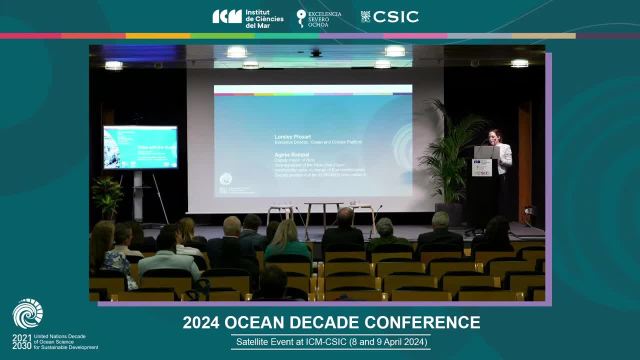 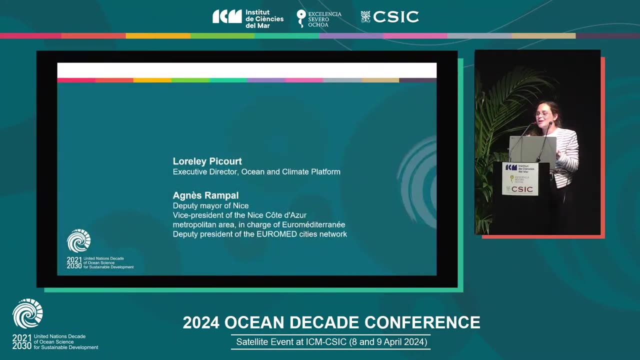 cities to the impacts of rising sea levels. well, we need to genuinely develop adaptation pathways that are rooted in firm scientific knowledge and that respond to economic, social and economic challenges, and we need to start working on ways to address these global and environmental imperatives. this is actually why the ocean and climate platform launched about four years ago, a 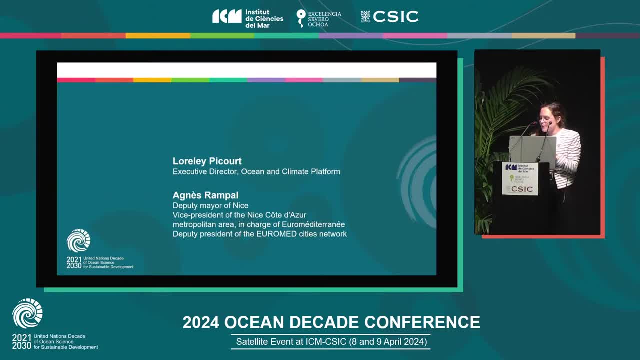 project called cities, and the idea was really to facilitate the development of adaptation strategies to support coastal cities threatened by sea level rise in three main ways. the first one was to collect and disseminate knowledge, knowledge that we already have. how do we make it accessible and sharing? experiences: you know what happens in Western Africa may be different than what happens in the Pacific, but how do we learn how to make it accessible? sharing experiences: you know what happens in Western Africa may be different than what happens in the Pacific, but how do we learn how to make it accessible? sharing experiences: you know what happens in Western Africa may be different than what happens in the Pacific, but how do we learn? learning how to make it accessible, sharing experiences. you know what happens in Western Africa may be different than what happens in the Pacific, but how do we learn? learning how to make it accessible, sharing experiences. you know what happens in Western Africa may be different than what happens in the Pacific, but how do we learn? 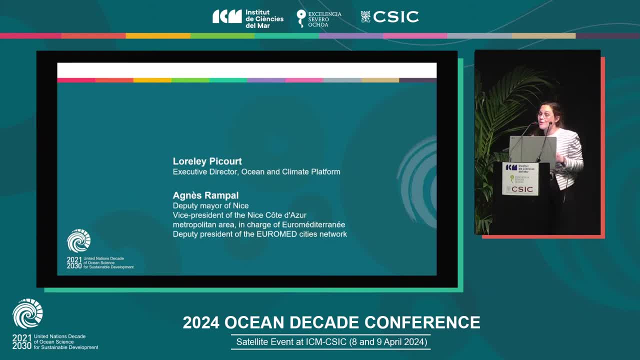 from each other's experience, and how do we build this solidarity that we've heard from each other's experience? and how do we build this solidarity that we've heard from each other's experience? and how do we build this solidarity that we've heard about so much today? and finally, how do we 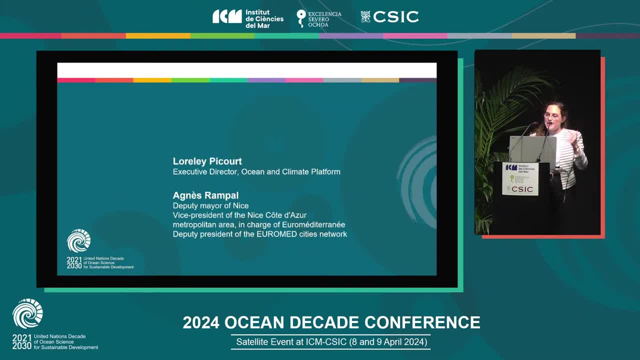 about so much today? and finally, how do we about so much today? and finally, how do we advocate for greater action at the local advocate for greater action at the local, advocate for greater action at the local, national and international levels, over the national and international levels, over the. 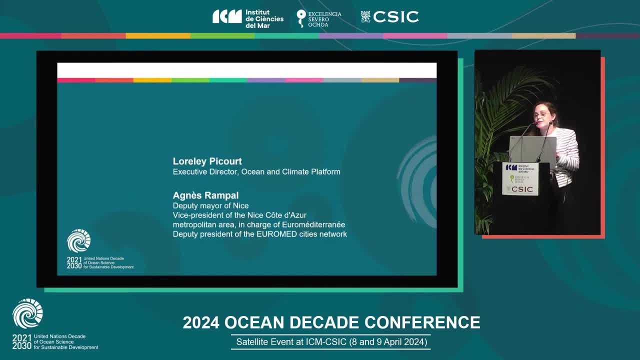 national and international levels. over the last three years, we have mobilized. over last three years, we have mobilized. over last three years, we have mobilized over 250 stakeholders across the globe. we've 250 stakeholders across the globe. we've 250 stakeholders across the globe. we've organized a number of workshops. we have 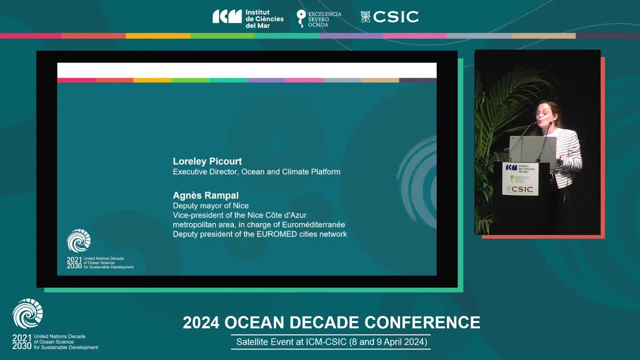 organized a number of workshops. we have organized a number of workshops. we have launched a city's declaration that was launched. a city's declaration that was launched. a city's declaration that was signed by over 50 mayors from Jakarta to signed by over 50 mayors from Jakarta to 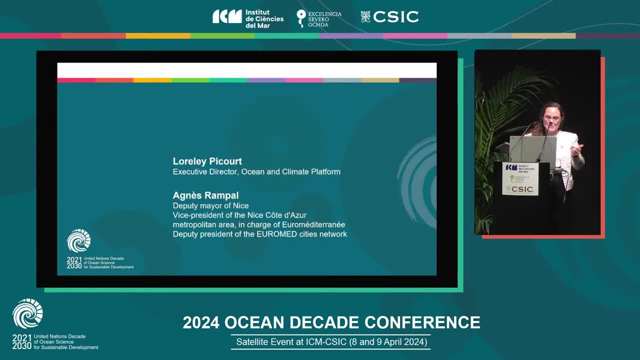 signed by over 50 mayors, from Jakarta to Lagos, as well as my two genius here in Lagos, as well as my two genius here in Lagos, as well as my two genius here in the room and our friends from nice of the room and our friends from nice of. 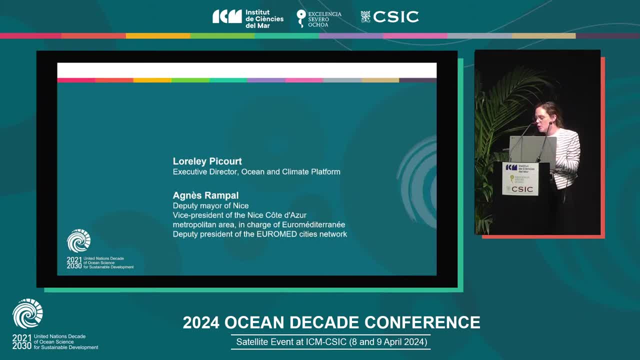 the room and our friends from nice. of course there is political leadership and course there is political leadership and course there is political leadership, and we need to continue emphasizing this in. we need to continue emphasizing this in. we need to continue emphasizing this in our global efforts to boost political 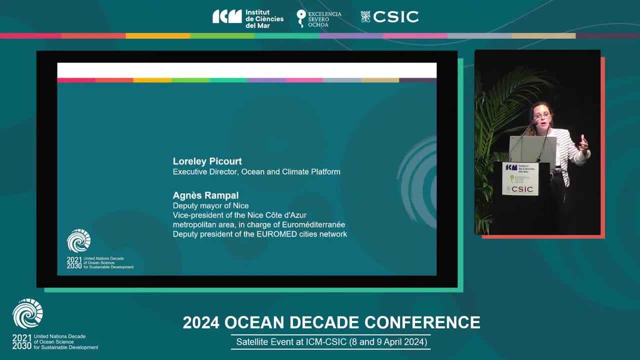 our global efforts to boost political, our global efforts to boost political leadership. we have launched these policy leadership. we have launched these policy leadership. we have launched these policy recommendations as well last year, at the recommendations as well last year, at the recommendations as well last year, at the one polar summit in in Paris. that was. 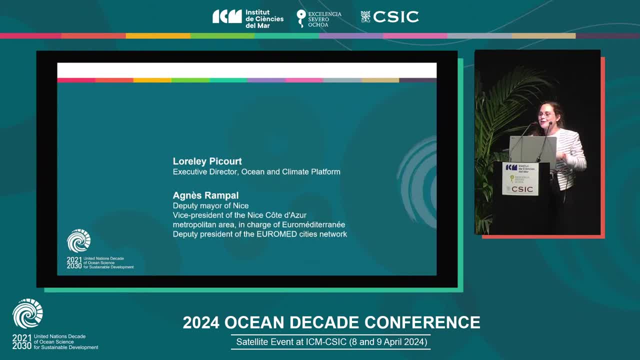 one polar summit in in Paris. that was one polar summit in in Paris that was supported by many organizations in the, supported by many organizations in the, supported by many organizations in the room. here again, IVP equally. and many room. here again, IVP equally. and many room. here again, IVP equally. and many, many friends of the platform focusing on 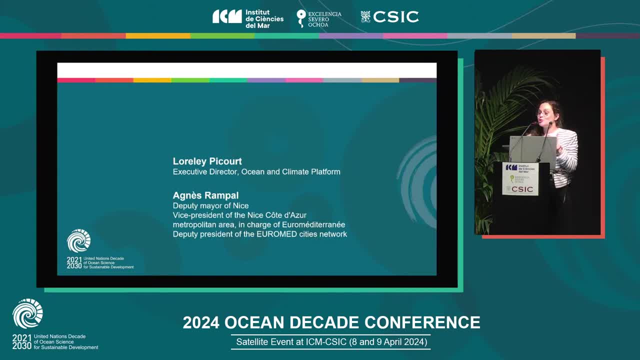 many friends of the platform focusing on, many friends of the platform focusing on priorities. there are solutions, knowledge priorities. there are solutions, knowledge priorities, there are solutions, knowledge, social justice as well as finance, and social justice as well as finance, and social justice as well as finance, and we'll hear a lot about this in the next. 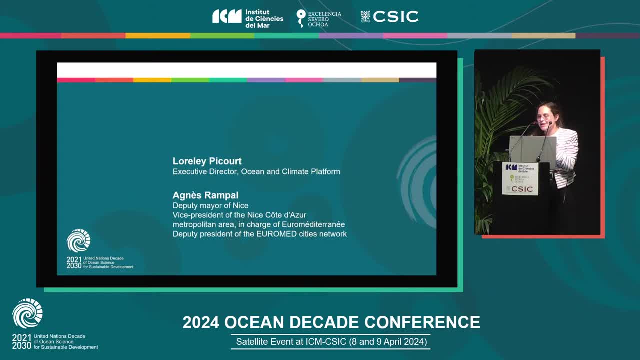 we'll hear a lot about this in the next. we'll hear a lot about this in the next few days, so I won't get into it. but one few days, so I won't get into it. but one few days, so I won't get into it. but one key takeaway here is that there's no 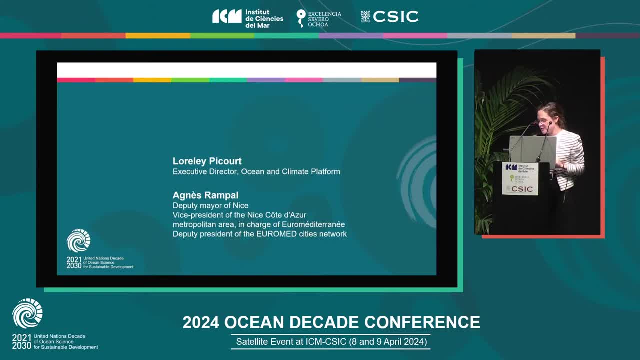 key takeaway here is that there's no key takeaway here is that there's no one-size-fits-all solution. we need to be one-size-fits-all solution. we need to be one-size-fits-all solution, we need to be context-specific and we need to break. 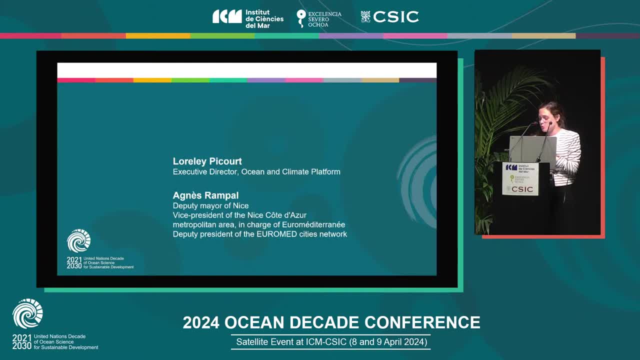 context-specific and we need to break context-specific and we need to break away from reactive short-term and away from reactive short-term and away from reactive short-term and protection-based responses to design, protection-based responses to design, protection-based responses to design, long-term adaptation strategies that are 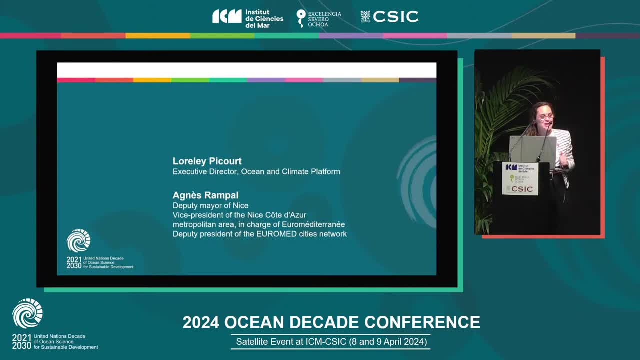 long-term adaptation strategies that are long-term adaptation strategies, that are tailored to local conditions. so, in the tailored to local conditions, so in the tailored to local conditions, so in the spirit of genuinely, you know boosting spirit of genuinely, you know, boosting spirit of genuinely, you know boosting this political leadership. we're now 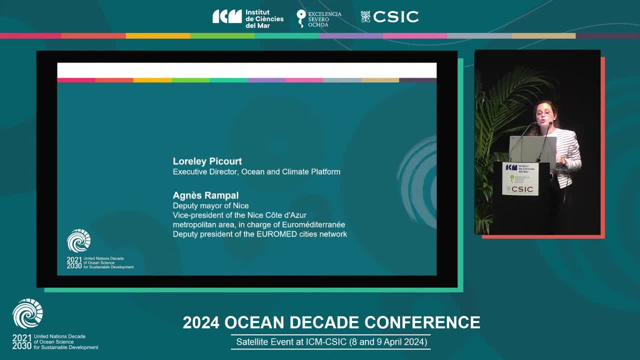 this political leadership. we're now this political leadership. we're now sailing towards 2025 and the next UN sailing towards 2025 and the next UN sailing towards 2025 and the next UN Ocean Conference that will take place in Ocean Conference that will take place in. 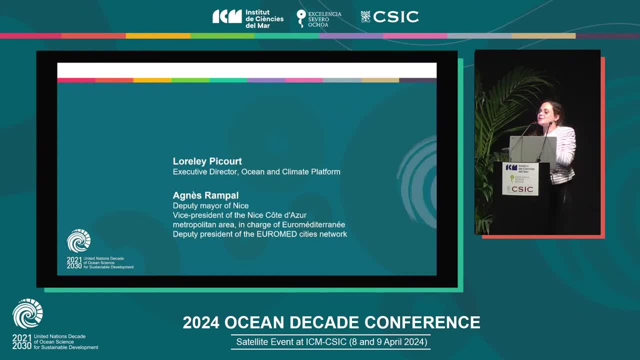 Ocean Conference that will take place in Nice, and our hope is to take the city's Nice, and our hope is to take the city's Nice and our hope is to take the city's initiative one step further with the initiative. one step further with the initiative, one step further with the launch of the ocean rise and resilience. 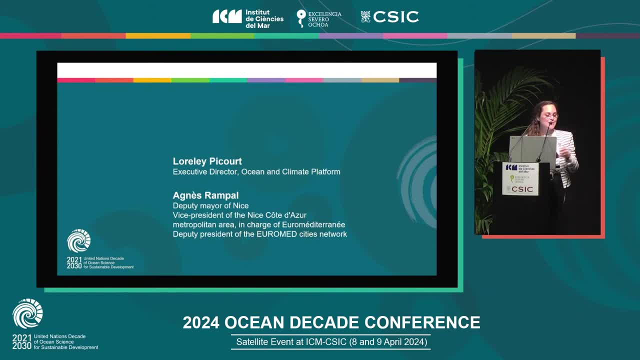 launch of the ocean rise and resilience. launch of the ocean rise and resilience coalition, under the great leadership of coalition, under the great leadership of coalition, under the great leadership of our friends from nice and mayor Christian. our friends from nice and mayor Christian. our friends from nice and mayor Christian is Tracy. so, without further ado, 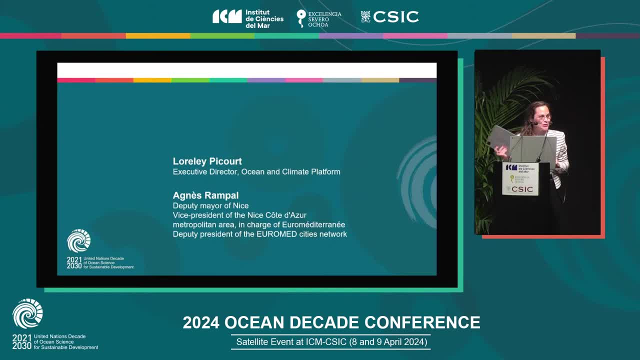 is Tracy, so without further ado, is Tracy, so without further ado, it's my very good privilege to invite. it's my very good privilege to invite. it's my very good privilege to invite Agnes Rompel to invite to announce the. Agnes Rompel to invite to announce the. 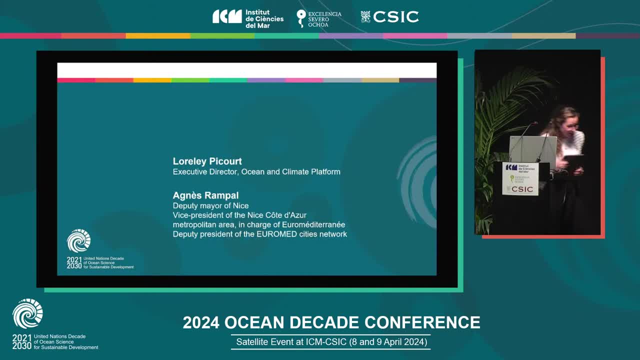 Agnes Rompel, to invite to announce the rest of the of the great work that we'll rest of the of the great work that we'll rest of the of the great work that we'll be doing together. thank you, thank you be doing together, thank you, thank you. 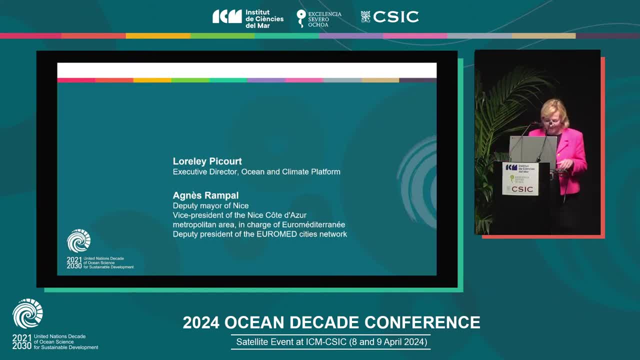 be doing together, thank you. thank you, Lorelei, my English is not so good. Lorelei, my English is not so good. Lorelei, my English is not so good. excuse me on behalf of Christian. is. excuse me on behalf of Christian. is excuse me on behalf of Christian. is Rosie, mayor of nice. president of the. 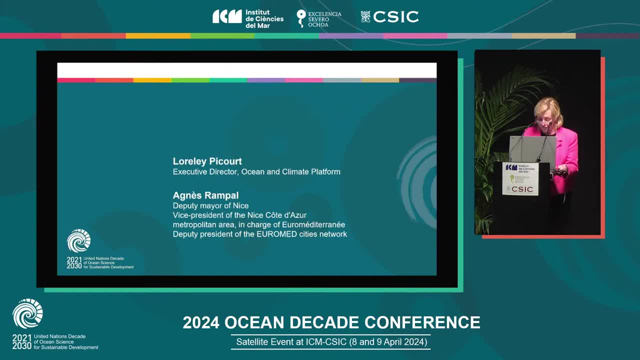 Rosie, mayor of nice. president of the Rosie mayor of nice, president of the metropolis of nisco dazur and president metropolis of nisco dazur and president metropolis of nisco dazur and president of the French South region. I would like 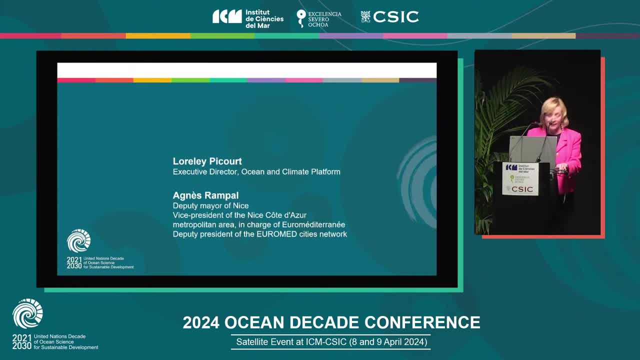 of the French South region, I would like of the French South region. I would like to thank you for this invitation to, to thank you for this invitation to, to thank you for this invitation to participate to your important meeting, participate to your important meeting, participate to your important meeting cities with the ocean, city and ports. 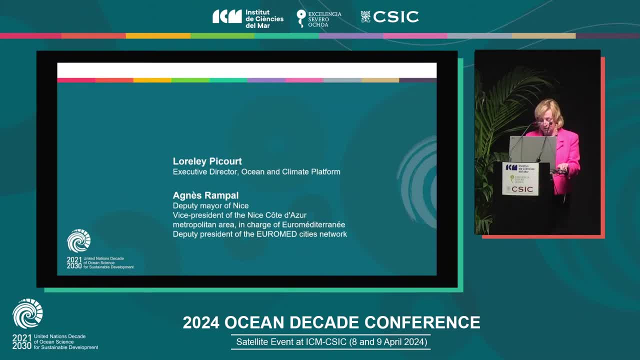 cities with the ocean city and ports. cities with the ocean city and ports: perspectives and connecting City Ports perspectives and connecting City Ports perspectives and connecting City Ports and the ocean are essential for all of, and the ocean are essential for all of, and the ocean are essential for all of us, especially coastal city. we need to. 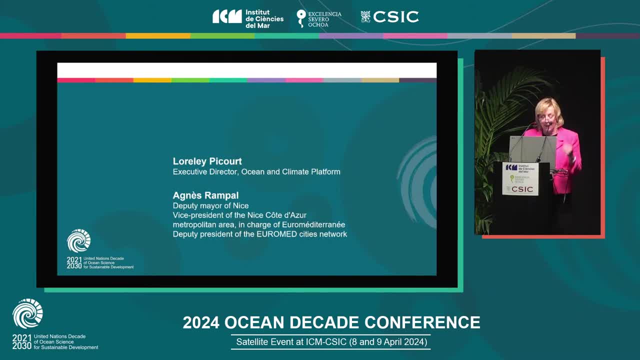 us, especially coastal city. we need to us, especially coastal city. we need to federate initiatives in order to make to federate initiatives in order to make to federate initiatives in order to make to make public policies converge for a make public policies converge for a make public policies converge for a better future and to pave the way of a. 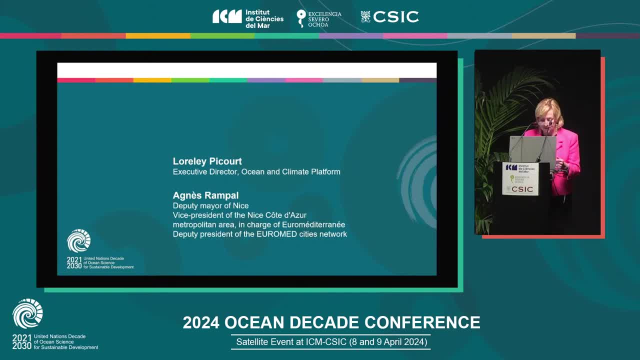 better future and to pave the way of a better future and to pave the way of a successful adaptation of our cities. we successful adaptation of our cities, we successful adaptation of our cities. we all, especially on the Mediterranean Sea, all especially on the Mediterranean Sea, all especially on the Mediterranean Sea, have been or will be hit by violent and 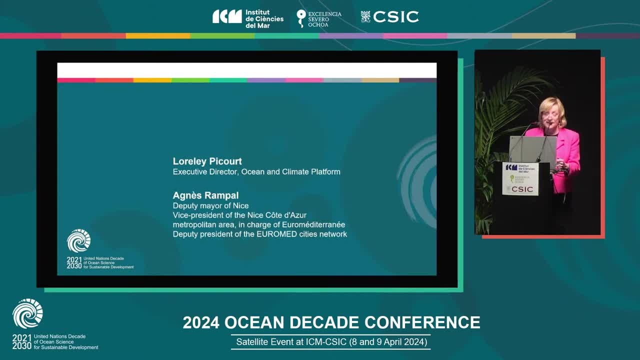 have been or will be hit by violent and have been or will be hit by violent and extreme weather events. extreme weather events, extreme weather events, sea level rise and a growing number of sea level rise and a growing number of sea level rise and a growing number of city will be affected by the coastal. 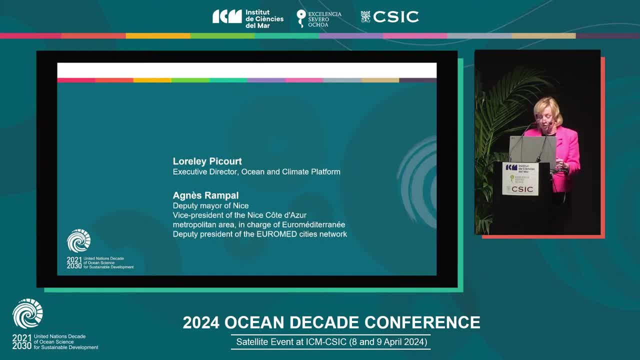 city will be affected by the coastal city will be affected by the coastal erosion. all these phenomenon are the erosion. all these phenomenon are the erosion. all these phenomenon are the result of climate change, and that's why result of climate change and that's why result of climate change, and that's why we need to act now, collectively and in a 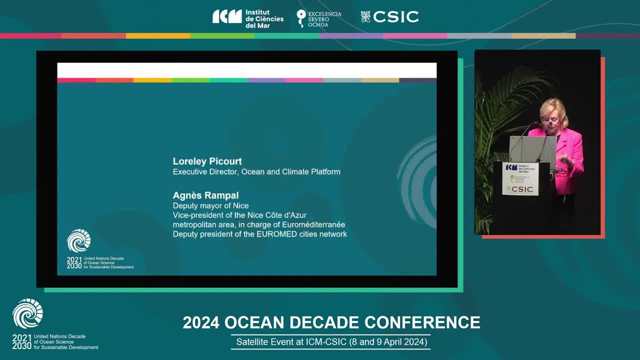 we need to act now collectively and in a. we need to act now collectively and in a convergent way to adapt our territories- convergent way to adapt our territories. convergent way to adapt our territories. our work today has been rich and still. our work today has been rich and still. 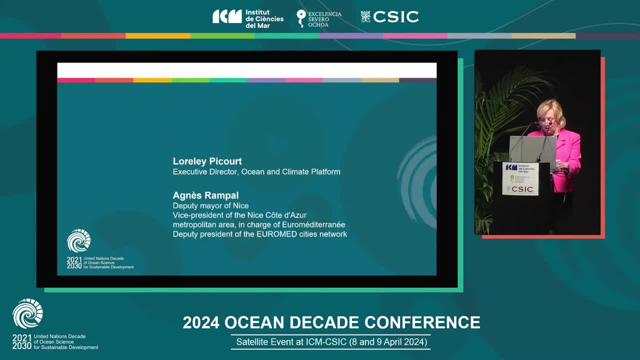 our work today has been rich and still stimulating. a lot of example have been stimulating. a lot of example have been stimulating. a lot of example have been very inspiring for all of us. we need to very inspiring for all of us. we need to very inspiring for all of us. we need to aggregate diverse actors, cities, port. 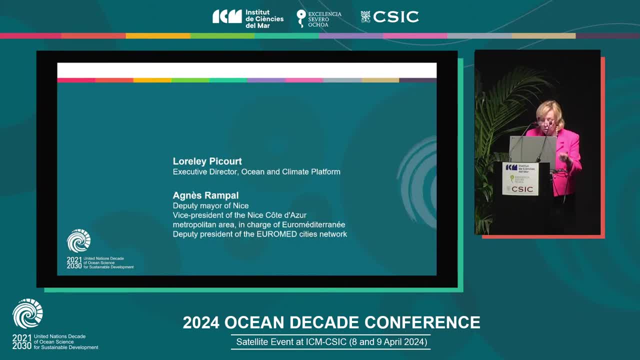 aggregate diverse actors: cities- port. aggregate diverse actors: cities: port- United Nation institution- non United Nation institution. non United Nation institution. non governmental organizations. ocean governmental organizations. ocean governmental organizations. ocean science for the agenda of 2030 by the science. for the agenda of 2030 by the. 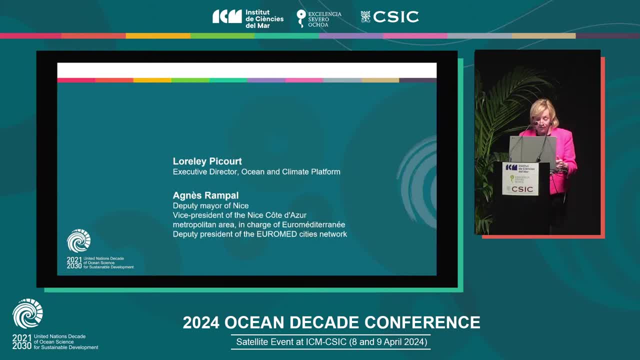 science for the agenda of 2030 by the AI VP and the FAO blue port initiative. AI VP and the FAO blue port initiative. AI VP and the FAO blue port initiative. as it has been underlined by the. as it has been underlined by the. 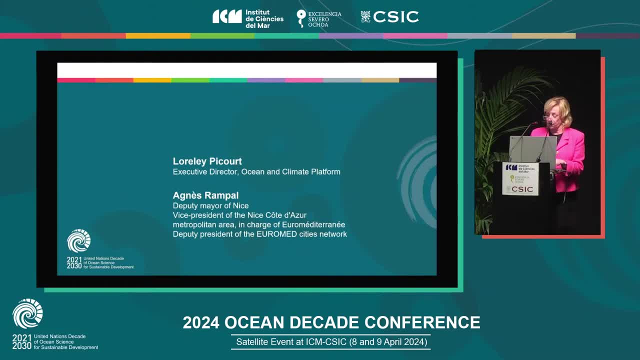 as it has been underlined by the roundtable port and city together for roundtable port and city, together for roundtable port and city, together for sustainable development. but we need to sustainable development, but we need to sustainable development, but we need to connect communities and agenda as it is. 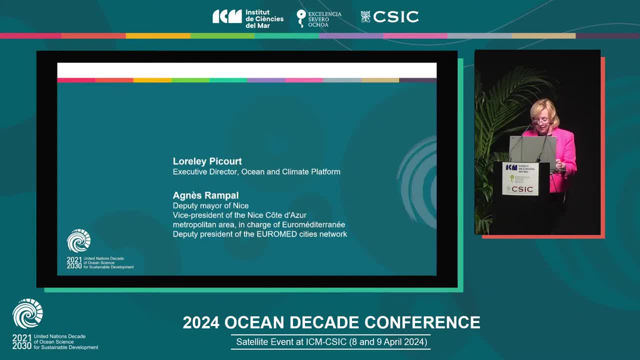 connect communities and agenda as it is. connect communities and agenda as it is. be at it as excuse me. it has been. be at it as excuse me. it has been. be at it as excuse me. it has been revealed by the roundtable gathering. revealed by the roundtable gathering. 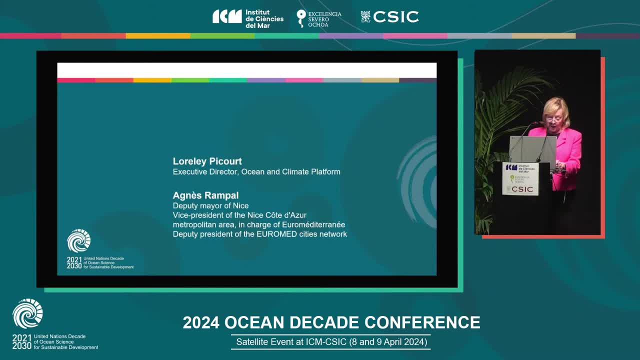 revealed by the roundtable gathering. representative. the United Union Habitat representative. the United Union Habitat representative. the United Union Habitat. ICLA ICT with nature and DCC CR. so ICLA ICT with nature and DCC CR. so ICLA ICT with nature and DCC CR. so some facts are well known in the world. 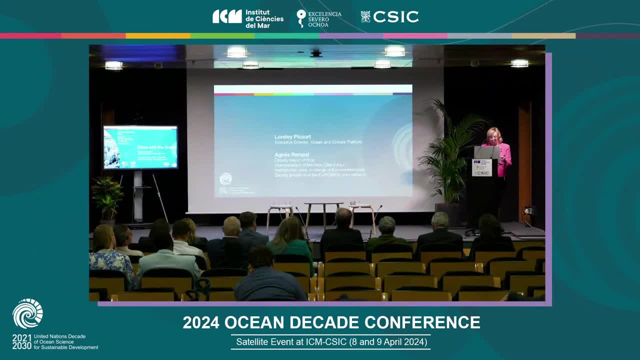 some facts are well known in the world. some facts are well known in the world today: 900 million people are living next today. 900 million people are living next today. 900 million people are living next to the sea, at less than 10 meter above to the sea at less than 10 meter above. 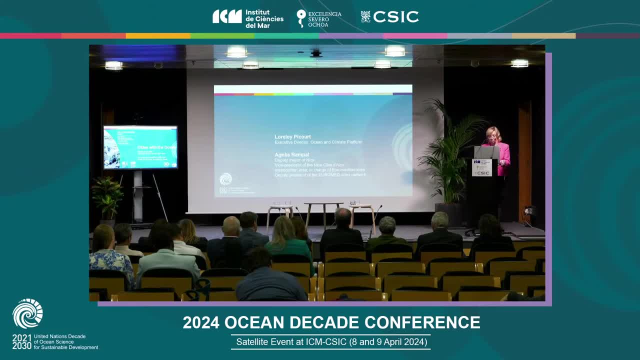 to the sea at less than 10 meter above the sea level and according to the the sea level. and according to the the sea level. and according to the fourth IPCC report, the sea level could. fourth IPCC report- the sea level could. fourth IPCC report- the sea level could rise from 30 centimeters by 2050. and. 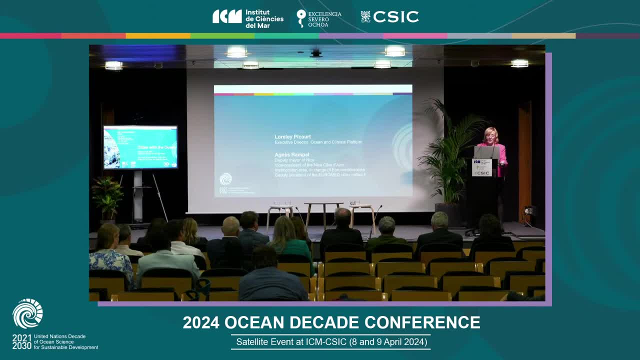 rise from 30 centimeters by 2050. and rise from 30 centimeters by 2050 and even by one meter by the end of even. by one meter by the end of even. by one meter by the end of the even. by one meter by the end of the century. this is a reason why President. 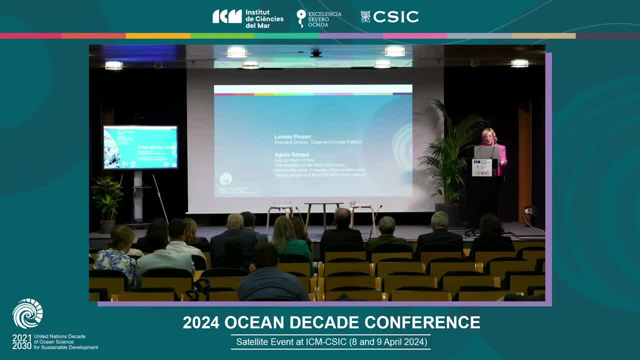 century. this is a reason why President century. this is a reason why President Macron asked our mayor, Christian is Macron, asked our mayor, Christian is Macron, asked our mayor, Christian is Rosie, to create a coalition of coastal Rosie, to create a coalition of coastal Rosie, to create a coalition of coastal city and regions across the sea hosting. 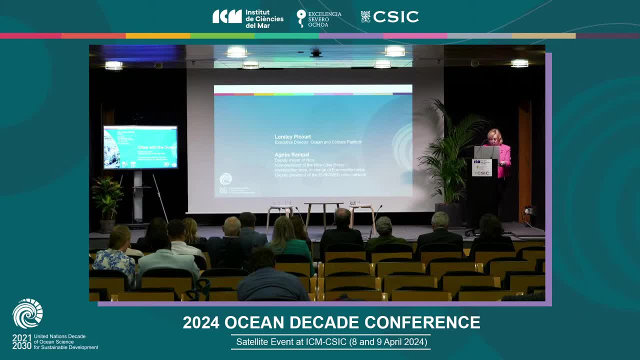 city and regions across the sea, hosting city and regions across the sea, hosting over 1 billion people. this coalition, over 1 billion people, this coalition, over 1 billion people, this coalition will be found in nice alongside the will be found in nice alongside the will be found in nice alongside the Enoch conference, the 7 of June 25. this. 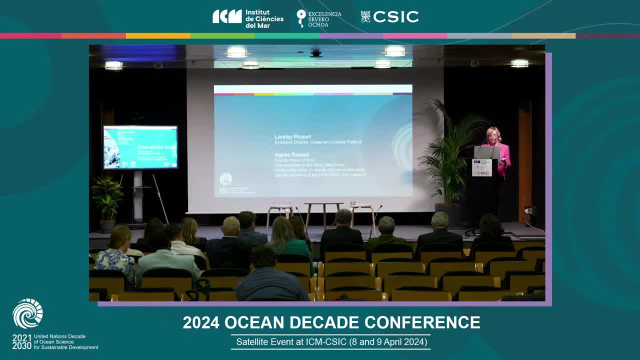 Enoch conference, the 7 of June 25. this Enoch conference, the 7 of June 25. this coalition should act, coalition should act, act, coalition should act, act on the Enoch conference, the 7 of June 25. this coalition should act on the Enoch conference, the 7 of June 25. this coalition should act around three main axes: scientific: 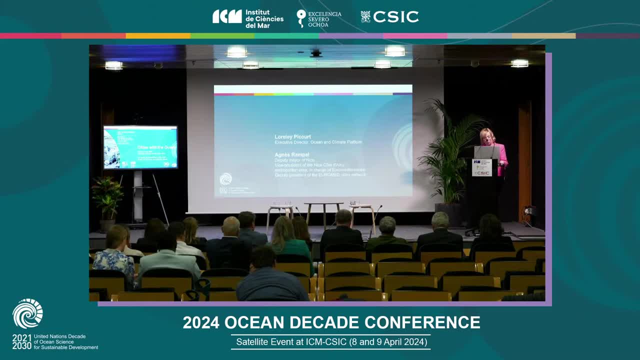 around three main axes. scientific- around three main axes: scientific cooperation, finance, finance cooperation, cooperation, finance, finance cooperation, cooperation, finance, finance cooperation. and institutional and decentralized and institutional and decentralized and institutional and decentralized cooperation between coastal cooperation, between coastal cooperation between coastal territories. a special event concerning the territories. a special event concerning the. 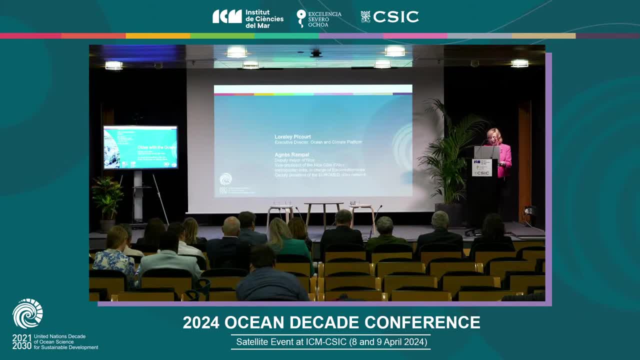 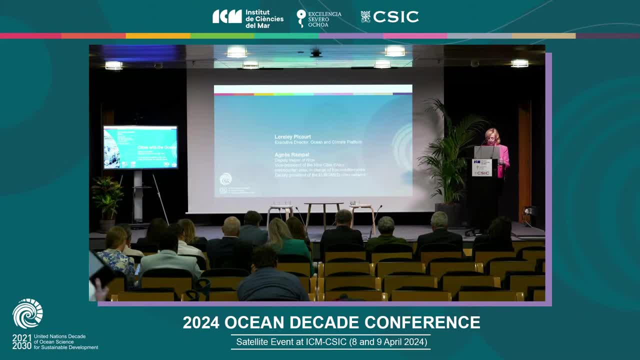 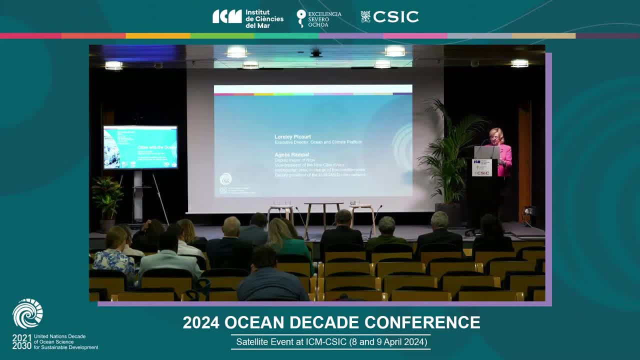 before start, the Enoch sweet nice, as a major role to play in mobilizing, major role to play in mobilizing, major role to play in mobilizing Mediterranean cities on a global scale. Mediterranean cities on a global scale, Mediterranean cities on a global scale. until then, they are still open question. 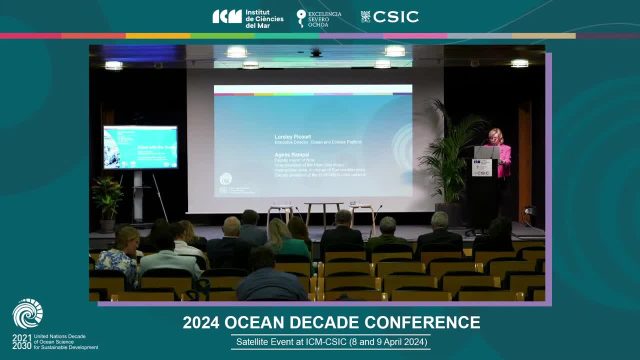 until then, they are still open question. until then, they are still open question to work on in order to contribute to, to work on, in order to contribute to, to work on, in order to contribute to this coalition, we need to think about a. this coalition, we need to think about a. 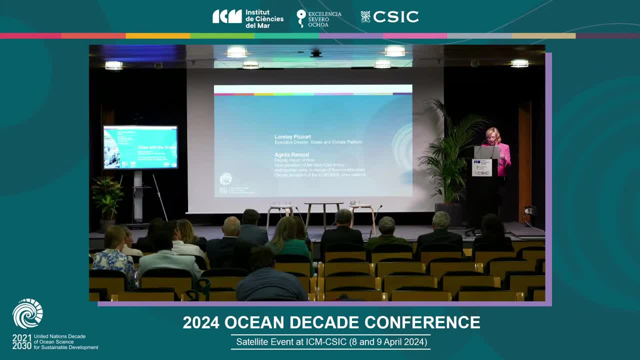 this coalition. we need to think about a tool that collect data, making it freely. tool that collect data, making it freely. tool that collect data, making it freely accessible for all city, within the accessible for all city, within the accessible for all city, within the coalition, coalition, coalition. we need to think about a mechanism to pull public and private. 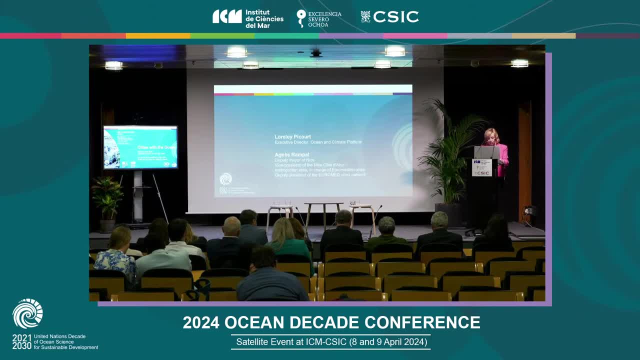 we need to think about a mechanism to pull public and private. we need to think about a mechanism to pull public and private resources to assist cities and region resources to assist cities and region resources to assist cities and region in financing their adaptation effort in in financing their adaptation effort in. 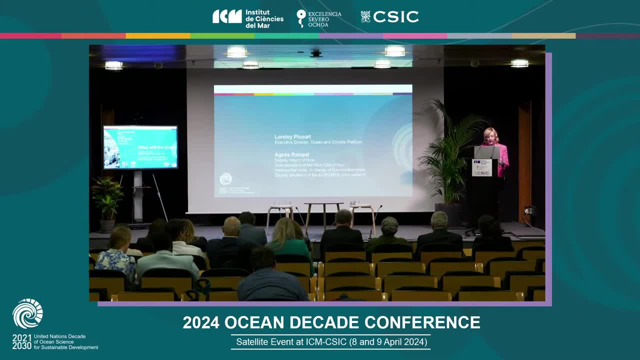 in financing their adaptation effort. in this regard, the work that has been this regard, the work that has been this regard, the work that has been engaged by the entire governmental ocean, engaged by the entire governmental ocean, engaged by the entire governmental ocean ocean Commission in the of the UNESCO. 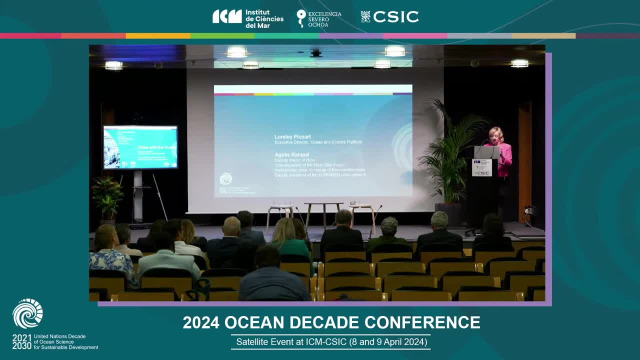 ocean Commission, in the of the UNESCO ocean Commission, in the of the UNESCO, alongside all of you present here today, alongside all of you present here today, alongside all of you present here today, is paving the way, is paving the way, is paving the way for gathering innovative solutions to 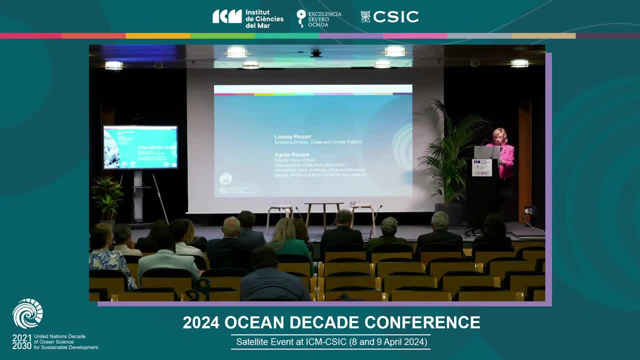 for gathering innovative solutions to. for gathering innovative solutions to better understand and protect the ocean. better understand and protect the ocean. better understand and protect the ocean. as you say: one ocean, ten years ten. as you say, one ocean, ten years ten. as you say, one ocean, ten years ten. challenges I would like to offer you one. 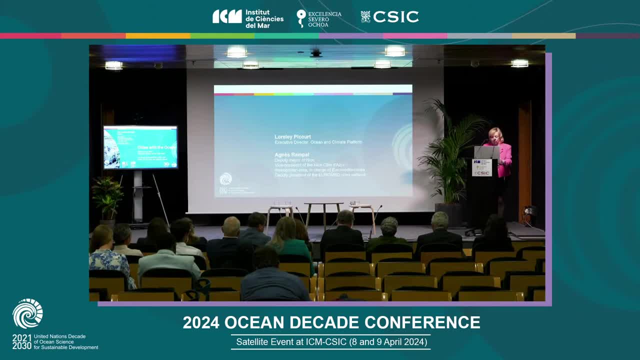 challenges. I would like to offer you one challenges. I would like to offer you one more challenges. challenge- let's join us. more challenges. challenge- let's join us more challenges. challenge: let's join us with Lorelei. let let's join our forces with Lorelei. let let's join our forces. 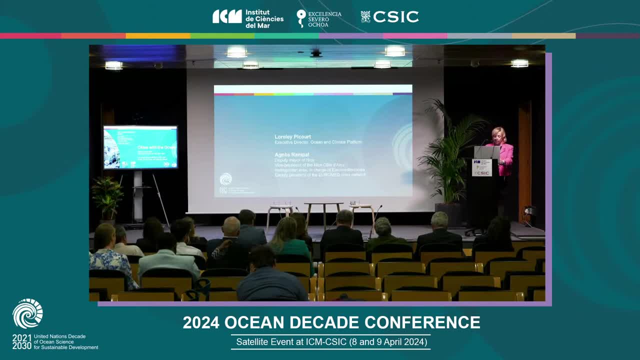 with Lorelei, let let's join our forces and please participate to our coalition and please participate to our coalition and please participate to our coalition. project to our, the next you know. project to our. the next you know. project to our, the next you know, conferencing, conferencing. 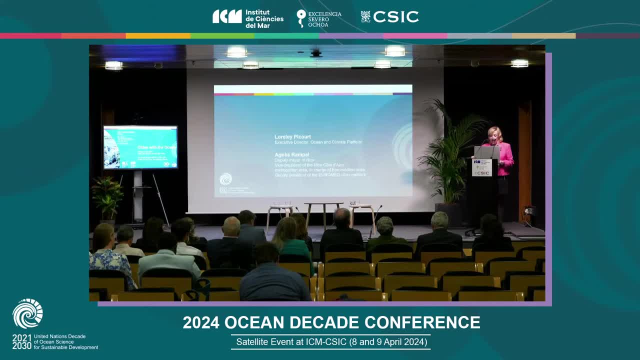 conferencing: conferencing in 2025, at the time where the in 2025, at the time where the in 2025, at the time where the multilateralism is in crisis. we believe multilateralism is in crisis. we believe multilateralism is in crisis. we believe it's still possible to invent a. 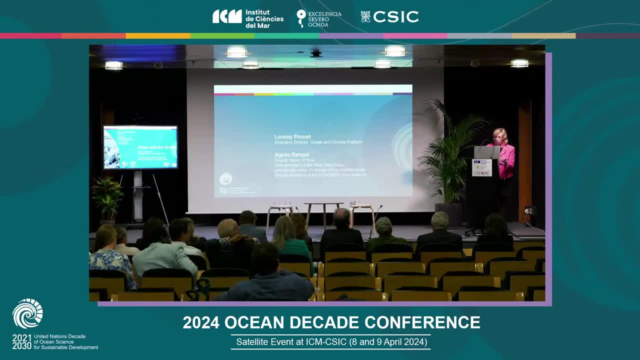 it's still possible to invent a. it's still possible to invent a multilateralism of territories, where multilateralism of territories, where multilateralism of territories where leader of coastal city and regions could leader of coastal city and regions could leader of coastal city and regions could communicate and share at their own scale. 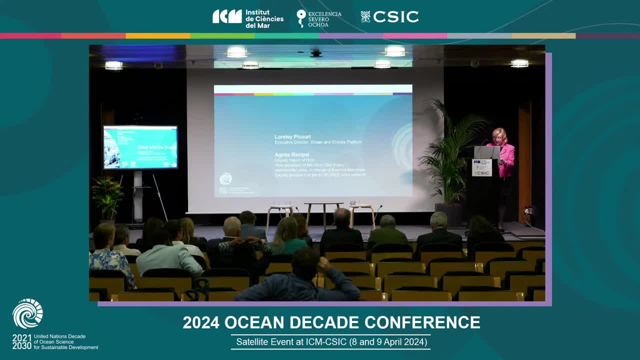 communicate and share at their own scale. communicate and share at their own scale. the mayor and the leaders of the coastal. the mayor and the leaders of the coastal, the mayor and the leaders of the coastal cities and region are the first to cities and region are the first to. 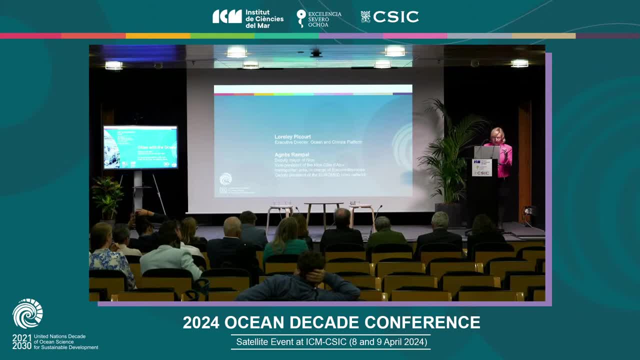 cities and region are the first to face the consequences of clear climate, face the consequences of clear climate, face the consequences of clear climate change, but, but they are also the first change, but, but they are also the first change, but, but they are also the first able to act to adapt their city. we need 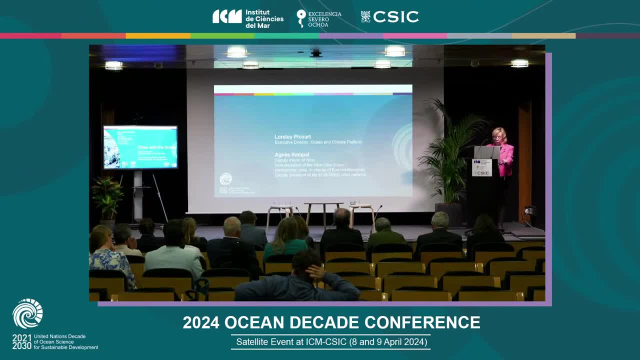 able to act to adapt their city. we need able to act to adapt their city. we need you to take part of our working groups, you to take part of our working groups, you to take part of our working groups and to support us with your expertise, and to support us with your expertise. 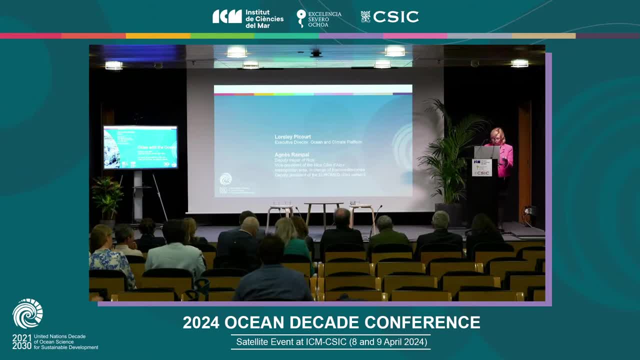 and to support us with your expertise, your energy, your passion and your, your energy, your passion and your, your energy, your passion and your ambition for the construction of this ambition. for the construction of this ambition, for the construction of this coalition, we have to act now for the 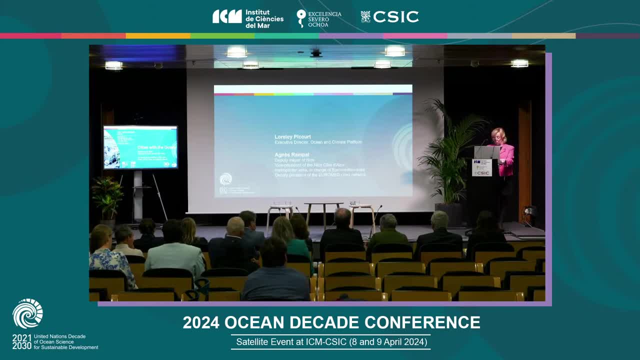 coalition. we have to act now for the coalition. we have to act now for the future of future, of future of our coastal territory, which are the our coastal territory, which are the our coastal territory, which are the future of our children. thank you very. future of our children. thank you very. 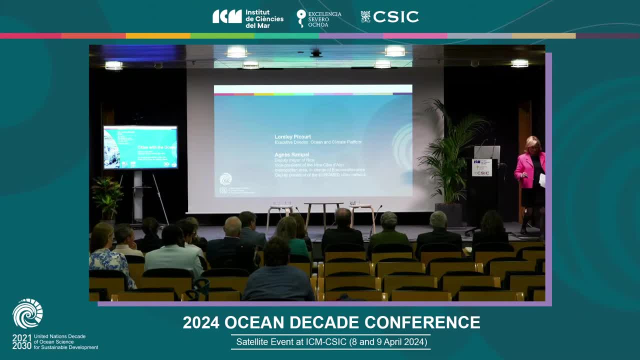 future of our children. thank you very much. thank you very much, mrs compel and it's. thank you very much, mrs compel and it's. thank you very much, mrs compel, and it's now time to close this, this event today. now time to close this, this event today. 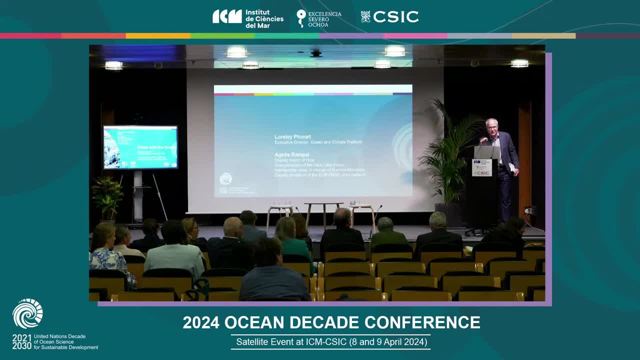 now time to close this, this event today, and, and I'll let Allison Clausen tell, and, and I'll let Allison Clausen tell, and, and I'll let Allison Clausen tell you the very final words: thank you you, the very final words, thank you you, the very final words, thank you. thank you very much, Olivier, and I am. thank you very much, Olivier, and I am thank you very much, Olivier, and I am going to quickly because I know we're going to quickly, because I know we're going to quickly because I know we're also testing the, the patience of our, also testing the, the patience of our. 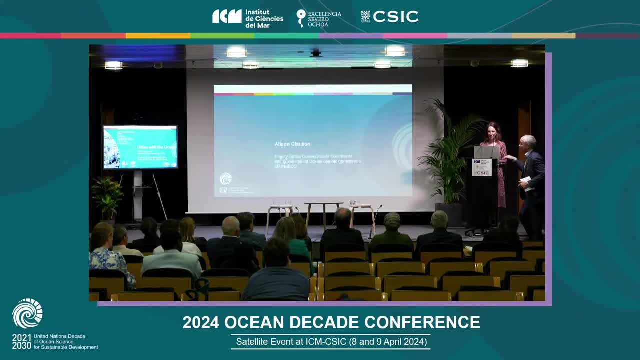 also testing the, the patience of our audio-visual crew. so thank you very much, audio-visual crew. so thank you very much, audio-visual crew. so thank you very much for staying with us till the end, but for staying with us till the end, but for staying with us till the end. but I'd really just like to say some closing. 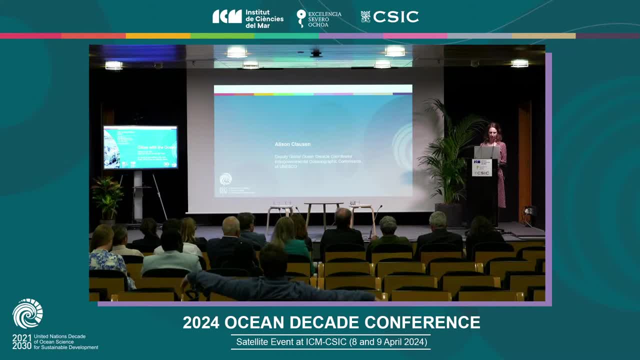 I'd really just like to say some closing. I'd really just like to say some closing words and echo Vita Helgeson the IOC words. and echo Vita Helgeson the IOC words. and echo Vita Helgeson, the IOC executive secretary, and expressed our executive secretary and expressed our 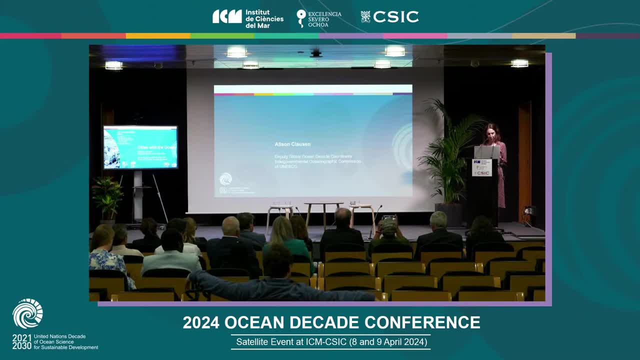 executive secretary and expressed our deepest thanks to the members of the deepest thanks to the members of the deepest, thanks to the members of the cities with the ocean scoping group, who cities with the ocean scoping group, who cities with the ocean scoping group, who have worked so hard to draft a 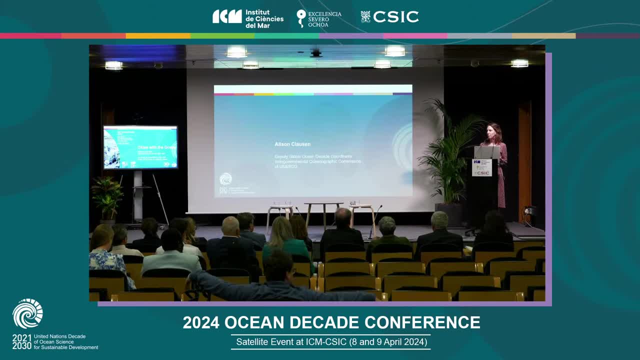 have worked so hard to draft a. have worked so hard to draft a comprehensive and inspiring call to comprehensive and inspiring call to comprehensive and inspiring call to action. it's been a really important action. it's been a really important action. it's been a really important step in clarifying the ambition of this. 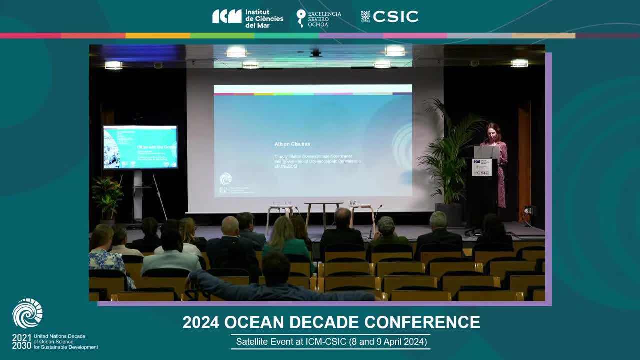 step in clarifying the ambition of this step in clarifying the ambition of this platform that we hope is going to have, a platform that we hope is going to have, a platform that we hope is going to have a great future, moving forward and bring on great future, moving forward and bring on. 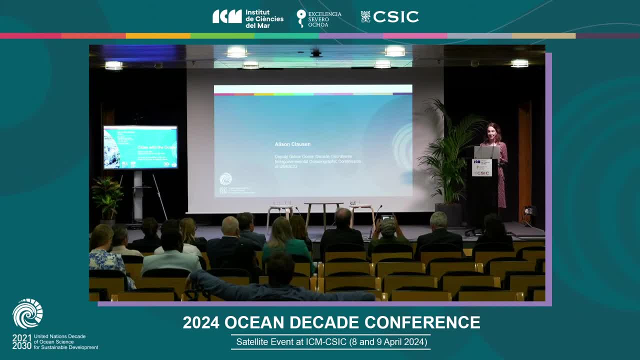 great future, moving forward and bring on many new partners. the ocean decade, many new partners. the ocean decade: many new partners. the ocean decade conference that starts in probably a two conference. that starts in probably a two conference. that starts in probably a two in a too short a time for many of us is 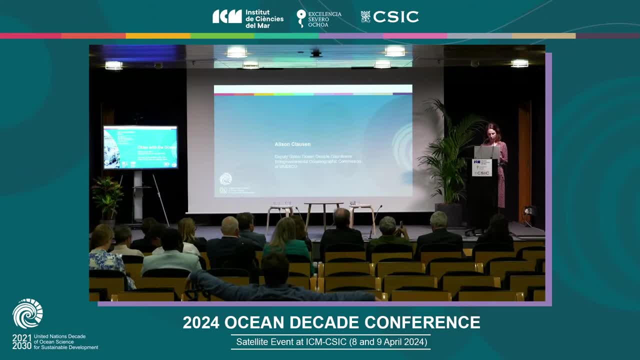 in a too short a time for many of us is in a too short a time for many of us is going to focus on defining the strategic. going to focus on defining the strategic. going to focus on defining the strategic ambition of the ocean decade for each. ambition of the ocean decade for each. 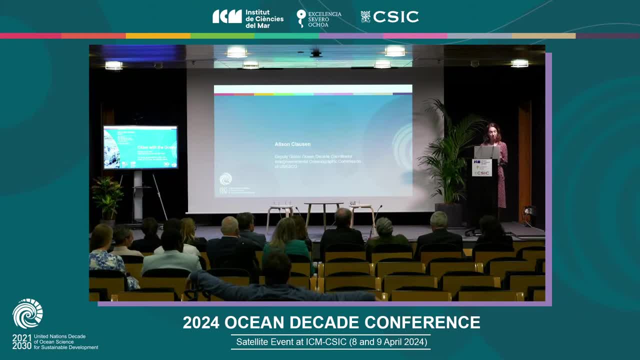 ambition of the ocean decade, for each challenge at a global level, and between challenge at a global level, and between challenge at a global level, and between Wednesday and Friday. that's going to be Wednesday and Friday. that's going to be Wednesday and Friday. that's going to be what we're talking about. a lot is looking 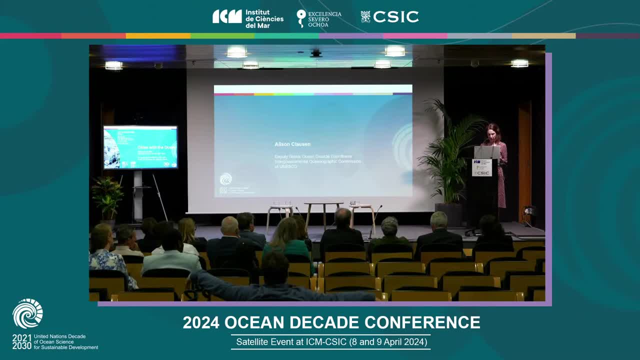 what we're talking about a lot is looking at the challenges in turn, but at the challenges in turn, but at the challenges in turn, but also looking across those challenges and also looking across those challenges and also looking across those challenges and helping to look at that strategic. helping to look at that strategic, helping to look at that strategic ambition, and that's why, of course, as ambition, and that's why, of course, as ambition, and that's why, of course, as we've heard this, new cities with the. we've heard this, new cities with the. 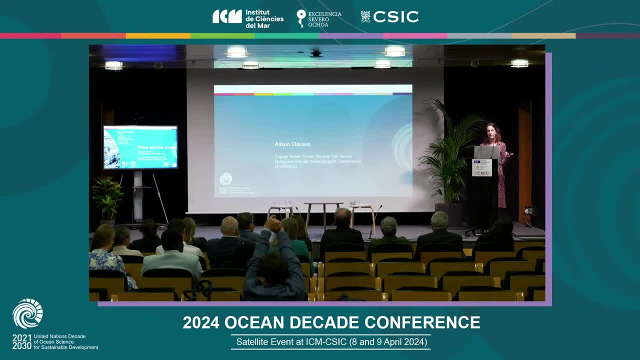 we've heard this: new cities with the ocean platform is so important. because ocean platform is so important, because ocean platform is so important, because it's going to help us complement this. it's going to help us complement this. it's going to help us complement this work and take it from that global global. 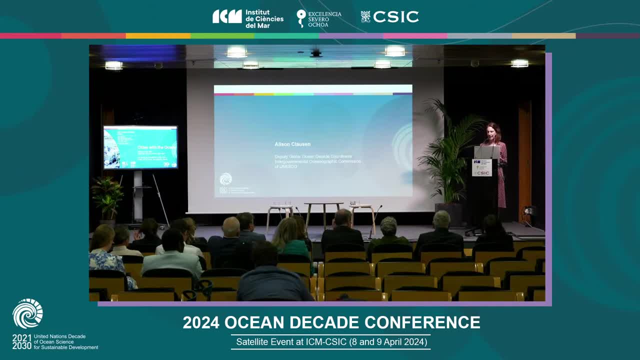 work and take it from that global global work and take it from that global global level to a level where most of the level, to a level where most of the level, to a level where most of the action is is really happening, but of action is is really happening, but of 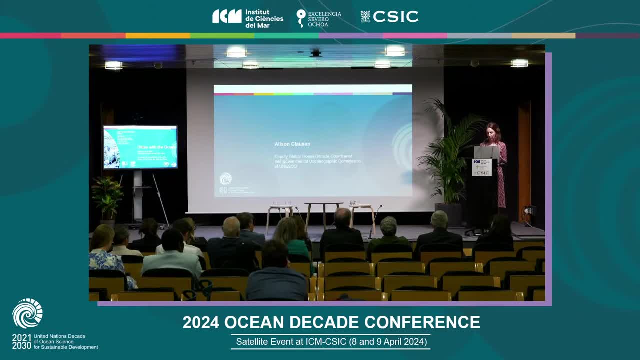 action is is really happening, but of course we can't do this alone. we need to course we can't do this alone. we need to course we can't do this alone. we need to do this within the ocean decade, do this within the ocean decade. do this within the ocean decade framework with the decade collaborative. 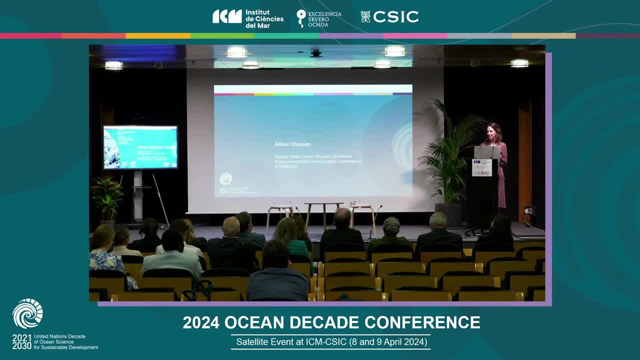 framework, with the decade collaborative framework, with the decade collaborative centers, the coordination officers, the centers, the coordination officers, the centers, the coordination officers, the national decade committees, many of you national decade committees, many of you national decade committees, many of you whom are represented here today, and we whom are represented here today, and we 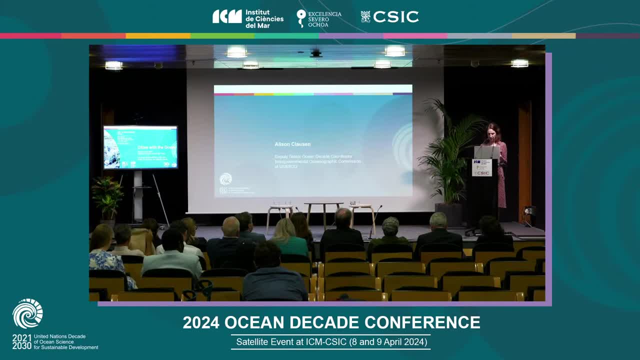 whom are represented here today, and we also need to develop strong synergies. also need to develop strong synergies. also need to develop strong synergies with existing networks and initiatives, with existing networks and initiatives, with existing networks and initiatives, and help connect the dots and strengthen and help connect the dots and strengthen. 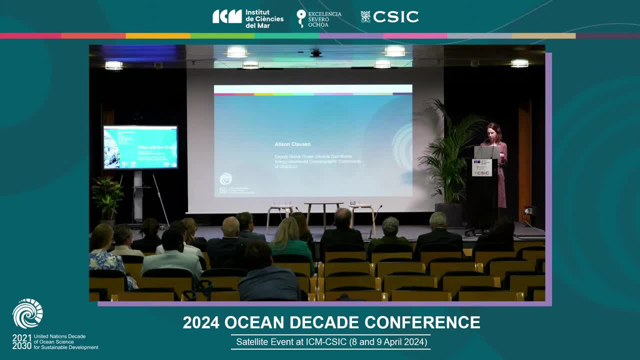 and help connect the dots and strengthen these. so an equally important task for these. so an equally important task for these. so an equally important task for the platform will be to map and engage. the platform will be to map and engage. the platform will be to map and engage with existing initiative and networks. 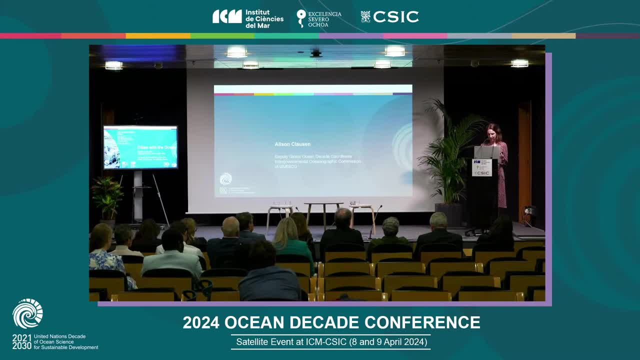 with existing initiative and networks, with existing initiative and networks, and we've we've heard from many of them and we've we've heard from many of them and we've we've heard from many of them here today. I'm really delighted that key here today. I'm really delighted that key. 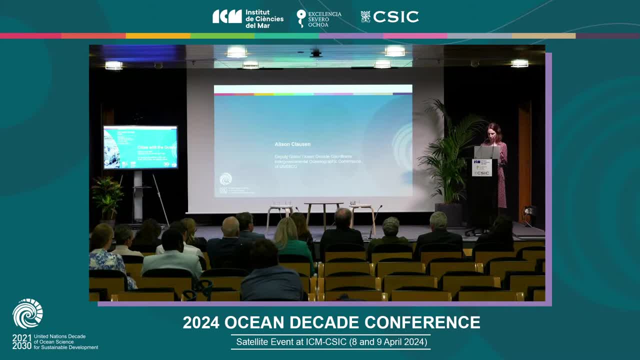 here today. I'm really delighted that key partners have shown their interest and partners have shown their interest and partners have shown their interest and joined the scoping group for you from UN. joined the scoping group for you from UN. joined the scoping group for you from UN habitat, equally to FA, blue ports, AI VP. 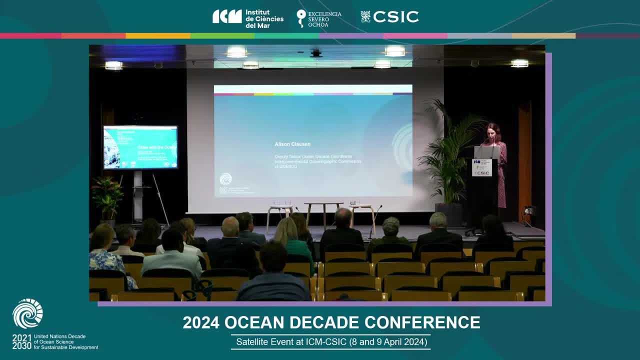 habitat equally to FA blue ports, AI VP. habitat equally to FA blue ports- AI VP. and this partnership will, of course, and this partnership will, of course, and this partnership will, of course, expand over time and will move from this expand over time and will move from this expand over time and will move from this common ambition to collaborative action. 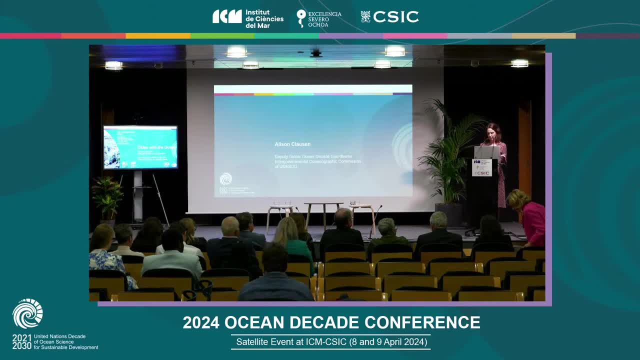 common ambition to collaborative action, common ambition to collaborative action. these synergies are going to determine. these synergies are going to determine. these synergies are going to determine how the platform can best be organized, how the platform can best be organized, how the platform can best be organized, structured and resourced. and I would like 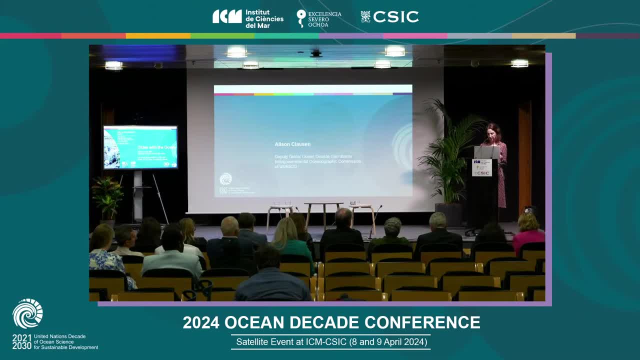 structured and resourced and I would like structured and resourced and I would like to re-emphasize that if I OC UNESCO is to re-emphasize that, if I OC UNESCO is to re-emphasize that, if I OC UNESCO is the implementing agency of the ocean. 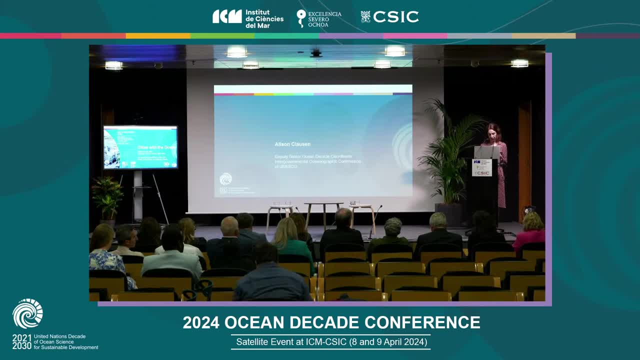 the implementing agency of the ocean. the implementing agency of the ocean, decade has initiated this platform and decade has initiated this platform and decade has initiated this platform and and worked and supported the- the scoping, and worked and supported the- the scoping, and worked and supported the- the scoping group, as it's moved forward. we're really 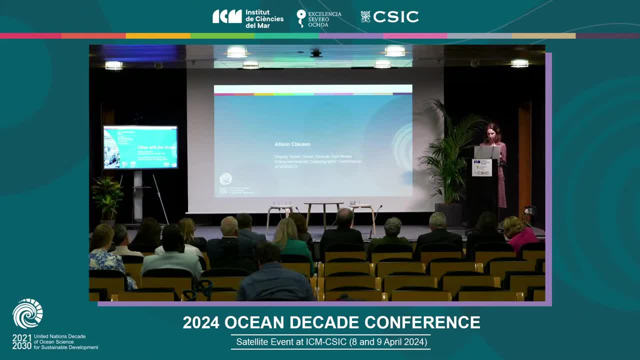 group as it's moved forward. we're really group as it's moved forward. we're really looking to two partners and welcoming looking to two partners and welcoming looking to two partners and welcoming partners to host resource and activate partners to host resource and activate partners to host resource and activate it, so it really does become a common a. 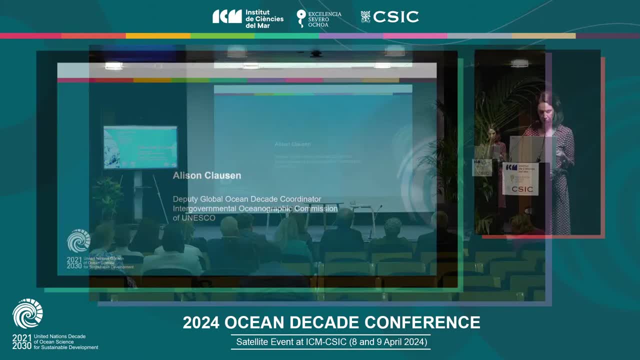 it so it really does become a common a it so it really does become a common, a common work and a common group, and we common work and a common group, and we common work and a common group and we can have a strong consortium to deliver, can have a strong consortium to deliver. 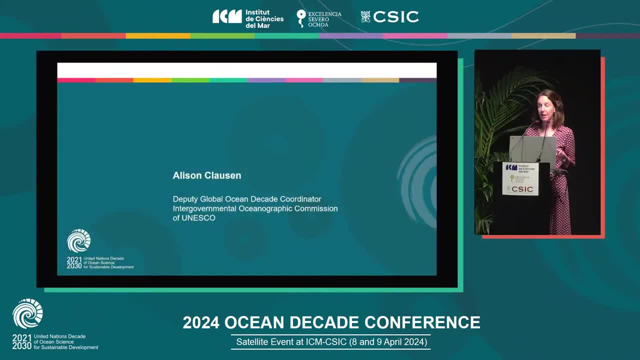 can have a strong consortium to deliver the ocean science we need for the. the ocean science we need for the. the ocean science we need for the coastal cities and ports. we want, so I. coastal cities and ports. we want so I. coastal cities and ports, we want so I call on all of the partners to to. 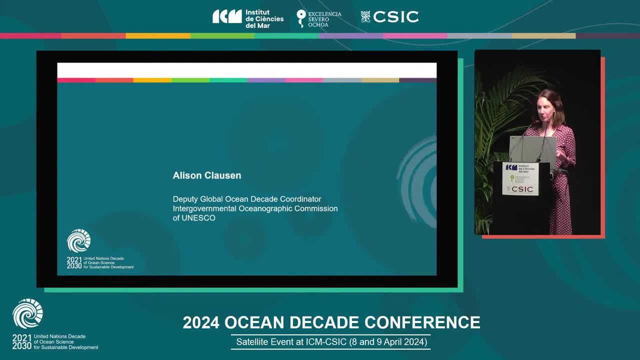 call on all of the partners to to call on all of the partners to to contribute to this collective effort and contribute to this collective effort and contribute to this collective effort. and we're always standby, ready to have. we're always standby ready to have, we're always standby ready to have discussions to see how we can best work. 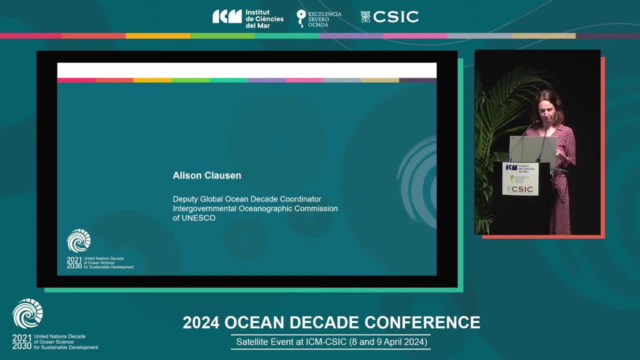 discussions to see how we can best work. discussions to see how we can best work together, as we've just heard from from together. as we've just heard from from together. as we've just heard from from from the previous speakers. one of the from the previous speakers, one of the. 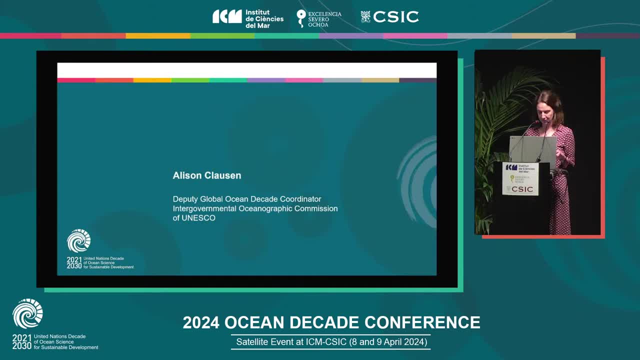 from the previous speakers. one of the next major steps on the ocean agenda is: next major steps on the ocean agenda is: next major steps on the ocean agenda is the UN Ocean Decade Conference in just the UN Ocean Decade Conference, in just the UN Ocean Decade Conference in just over a year in nice, and where we're 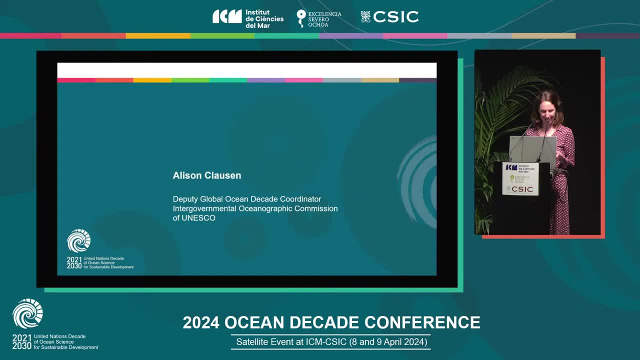 over a year in nice, and where we're over a year in nice and where we're looking forward to working with the, looking forward to working with the, looking forward to working with the municipality of nice with Lorelei and municipality of nice with Lorelei and municipality of nice with Lorelei, and colleagues, to ensure that the ocean with 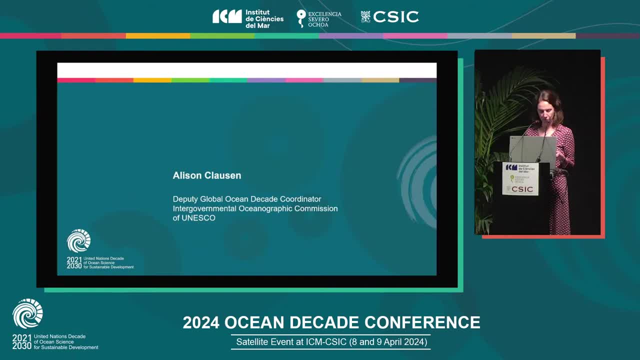 colleagues to ensure that the ocean with colleagues, to ensure that the ocean, with the city's platform as well, integrated, the city's platform as well integrated, the city's platform as well, integrated with the ocean rise and resilience, with the ocean rise and resilience with the ocean rise and resilience. coalition and summit, because there are 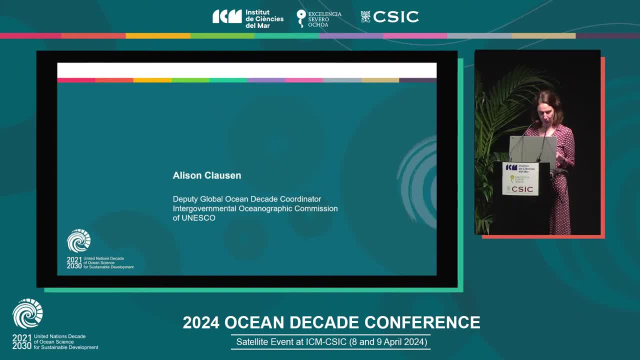 coalition and summit, because there are coalition and summit, because there are obviously a large number of synergies, obviously a large number of synergies, obviously a large number of synergies. and again we can be stronger by working, and again we can be stronger by working, and again we can be stronger by working together. so with this, I thank you again. 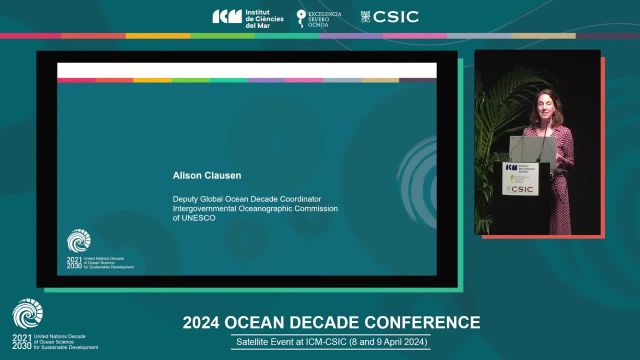 together. so with this, I thank you again together. so with this, I thank you again to all the members of the scoping group, to all the members of the scoping group, to all the members of the scoping group, to all our speakers today, to the, to all our speakers today, to the. 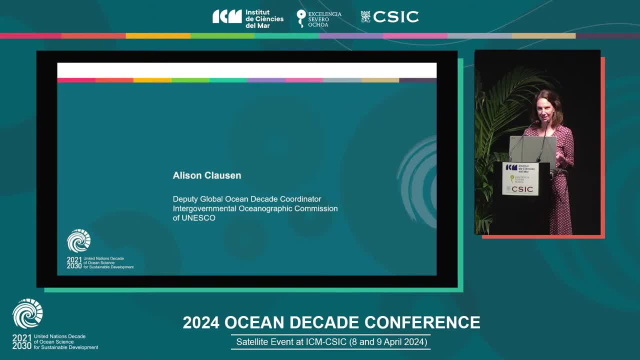 to all our speakers today, to the audience here today, of course to ICM for audience here today. of course to ICM for audience here today, of course to ICM for for hosting us in this, in this, for hosting us in this, in this, for hosting us in this, in this magnificent venue. I wish you all a. 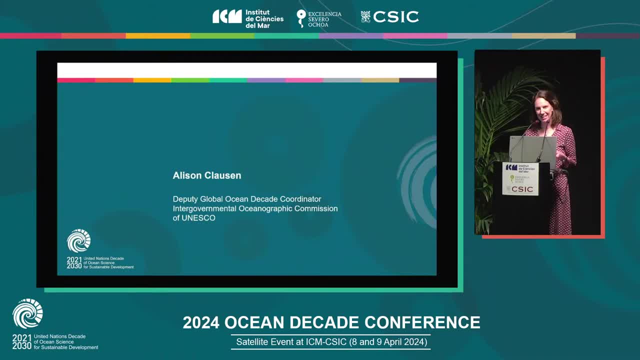 magnificent venue. I wish you all a magnificent venue. I wish you all a wonderful ocean decade week. look wonderful, ocean decade week. look wonderful, ocean decade week. look forward to seeing you at the ocean, forward to seeing you at the ocean, forward to seeing you at the ocean decade conference starting on Wednesday. 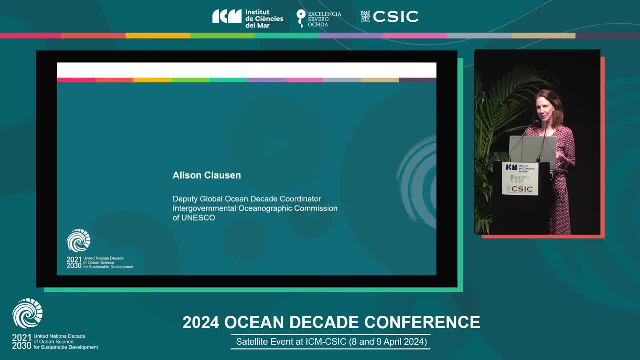 decade conference starting on Wednesday. decade conference starting on Wednesday. and look forward to continuing the and look forward to continuing the and look forward to continuing the collaboration on coastal cities in the collaboration on coastal cities in the collaboration on coastal cities in the framework of the ocean decade. thank you. 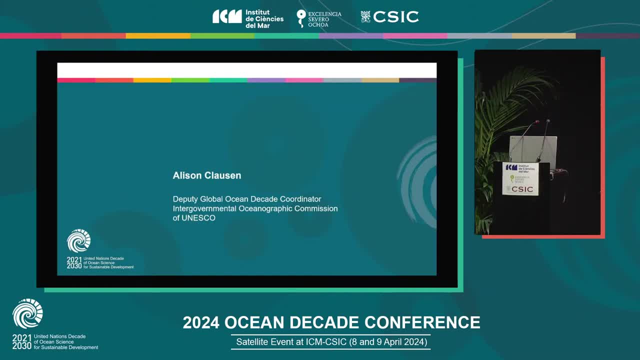 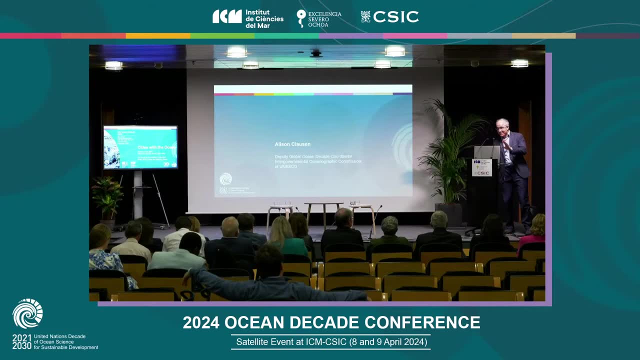 framework of the ocean decade. thank you. framework of the ocean decade. thank you very much, thank you. the the event is is closed, but thank you. the the event is is closed, but thank you. the the event is is closed, but I, before leaving, I just want to invite. 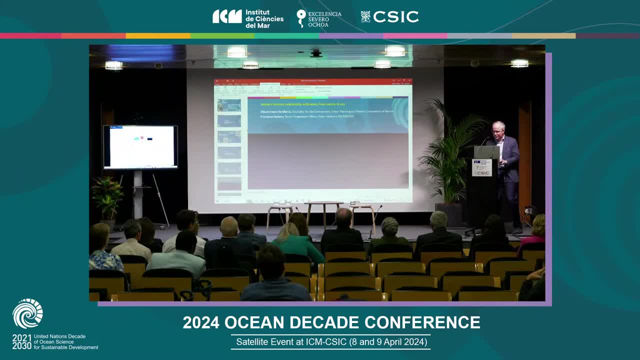 I before leaving, I just want to invite. I before leaving, I just want to invite. invite our speakers and members of the. invite our speakers and members of the. invite our speakers and members of the scoping group to move to the to the scene. scoping group to move to the to the scene. 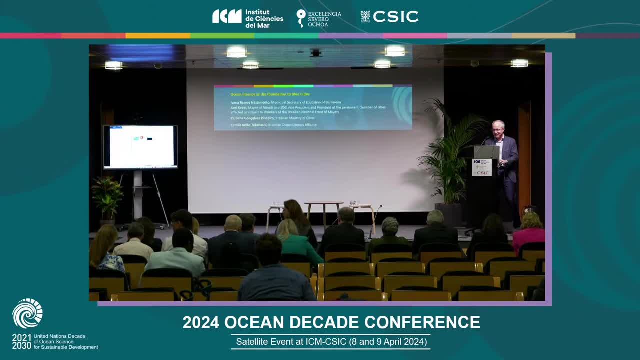 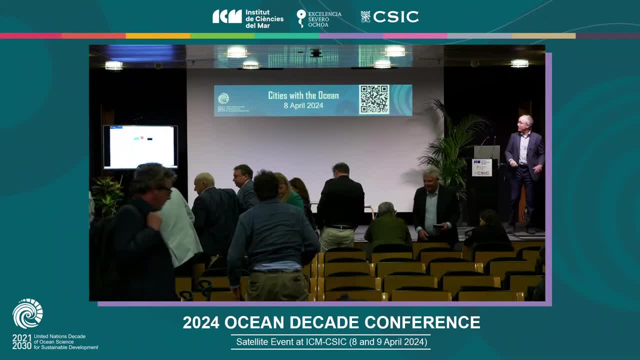 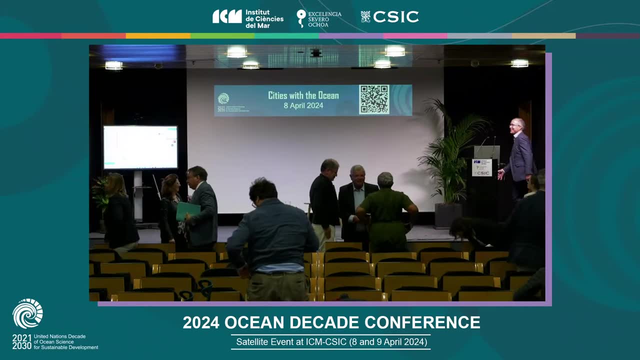 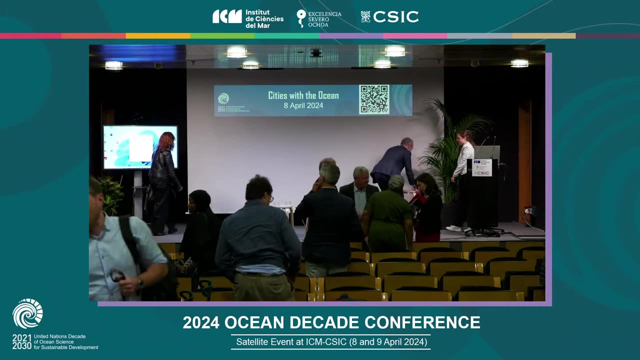 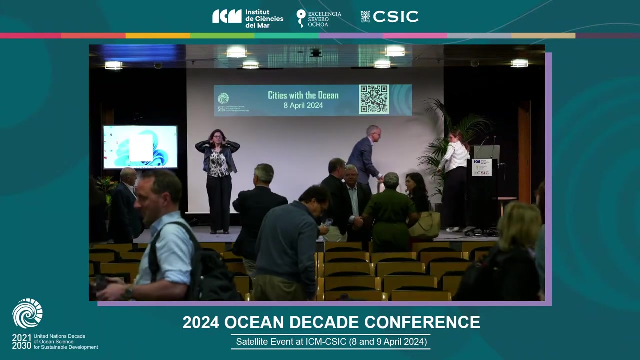 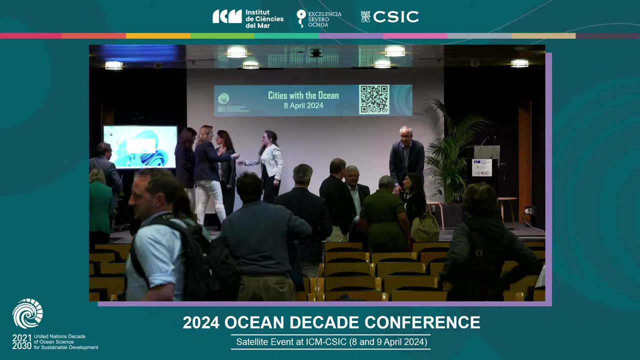 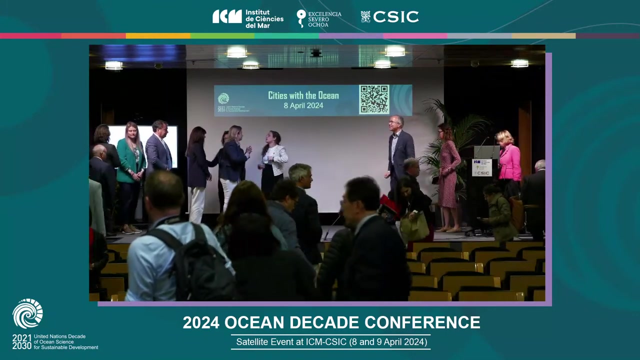 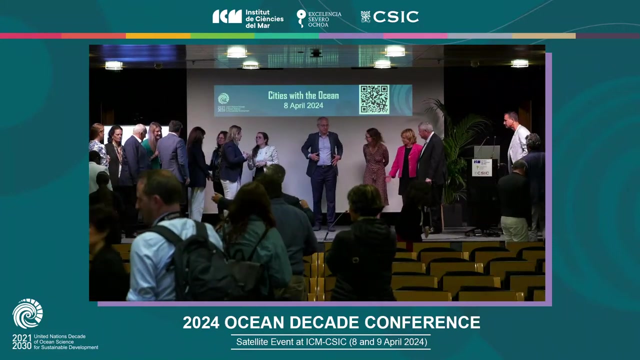 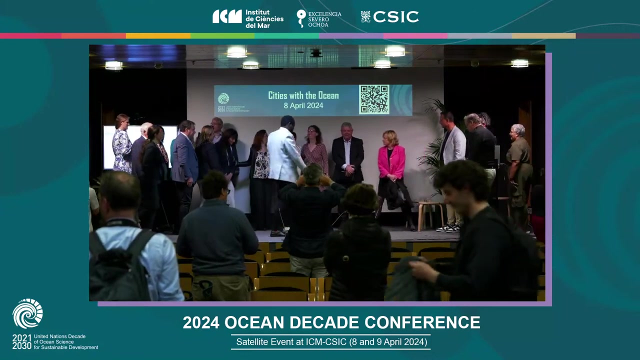 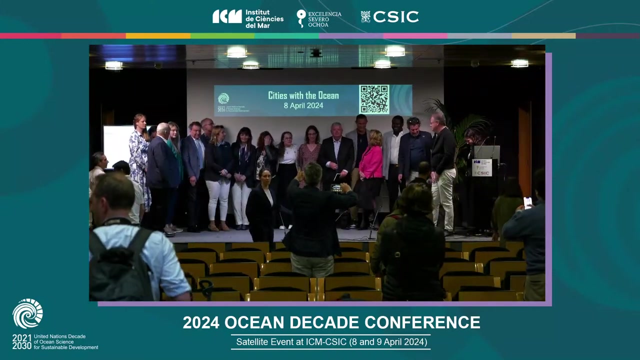 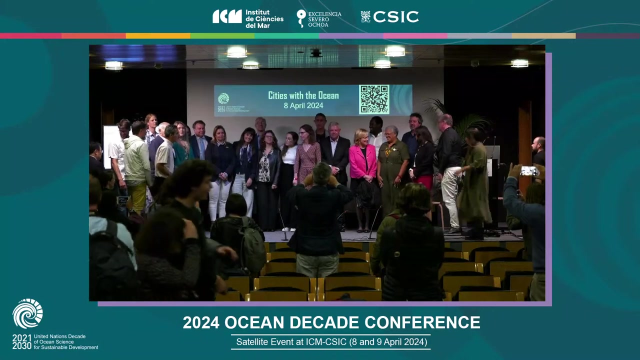 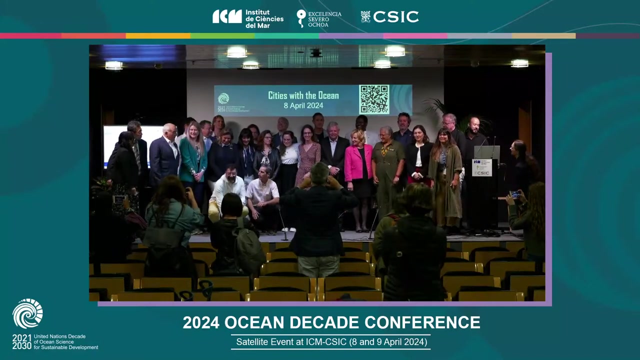 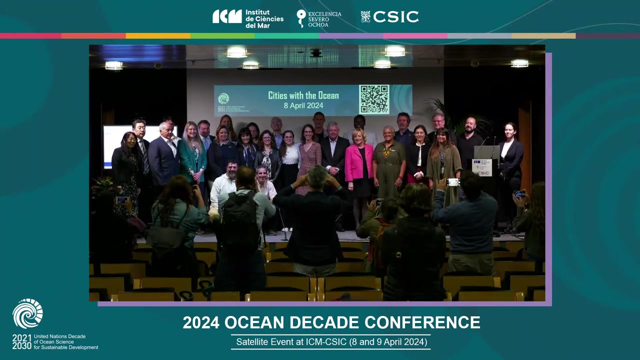 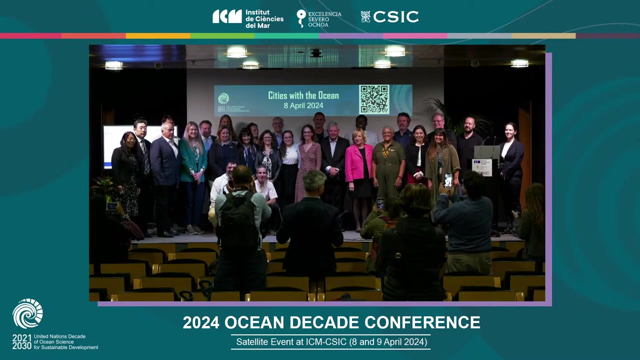 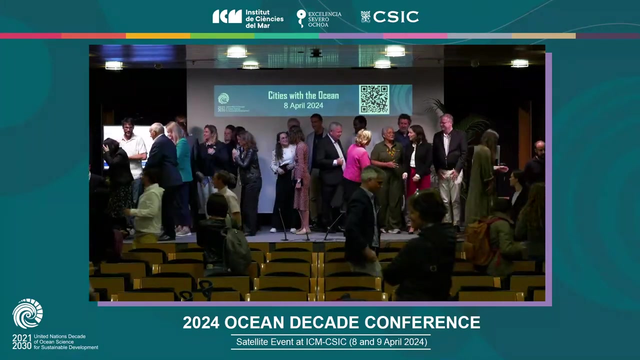 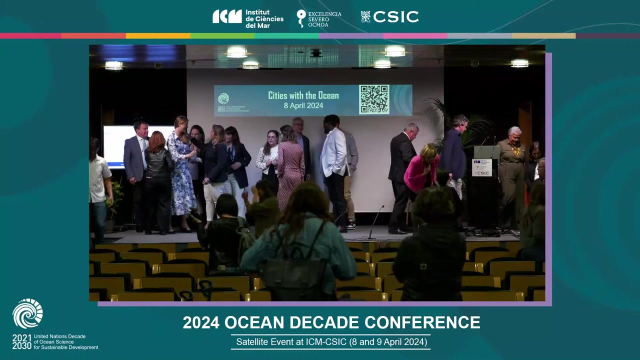 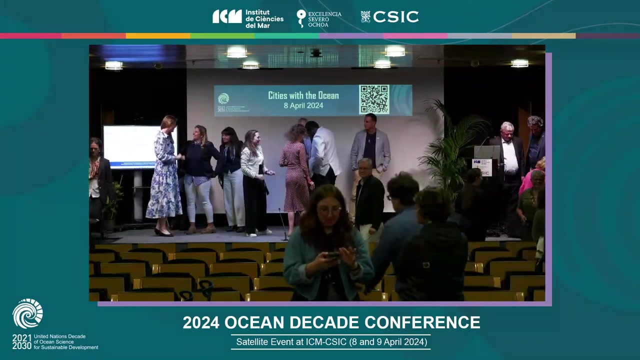 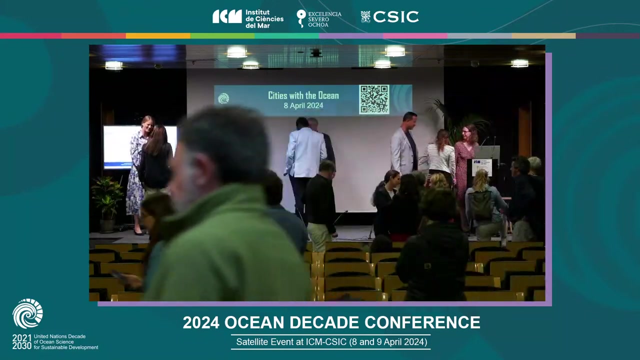 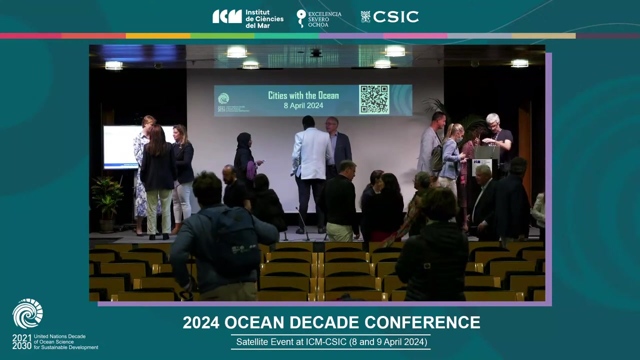 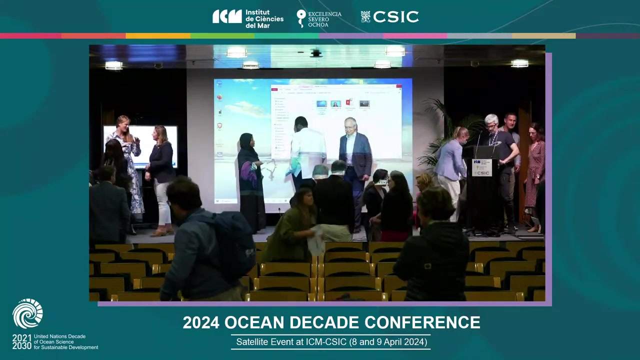 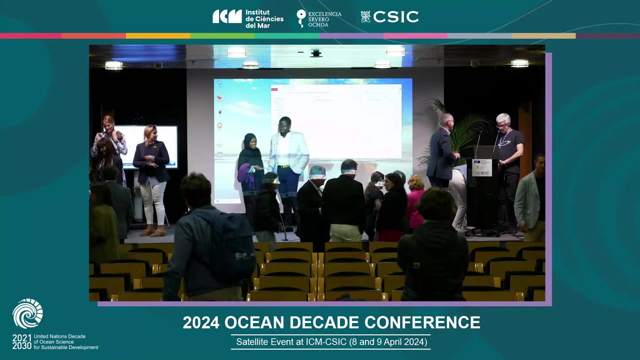 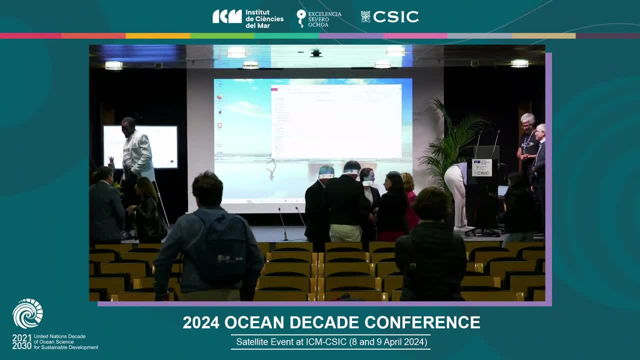 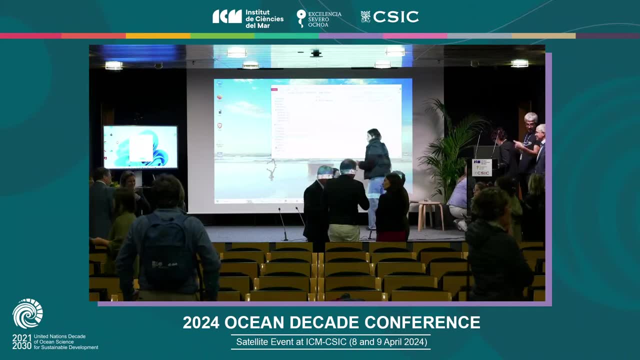 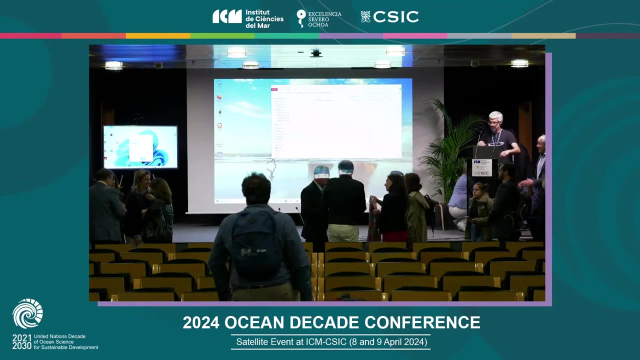 Yeah, Yeah, I pushed as much as I could, Yeah, but then we don't have breaks. The people who's working inside don't have any breaks. You have to set the new communication, new tool, translators. Okay, Thanks a lot for your support. 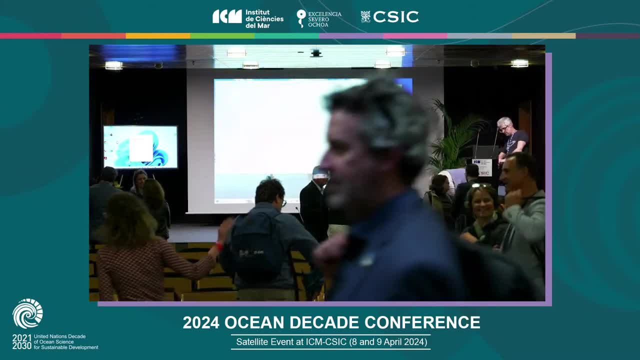 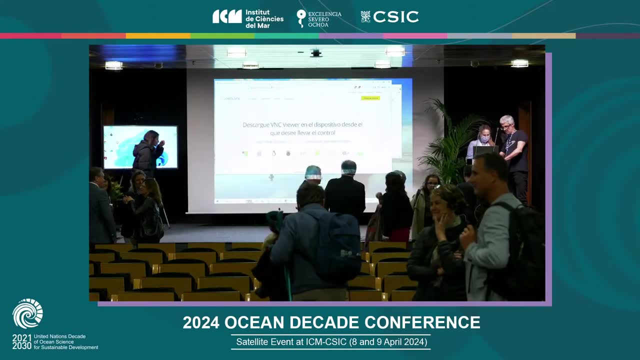 Look, here you have it. Here you have the add-on. Okay, It's active. okay, Now I'll cover this one if you want me not to see it? Yeah, because I'm going to the Gmail. If you put the drive, I'll give you my.